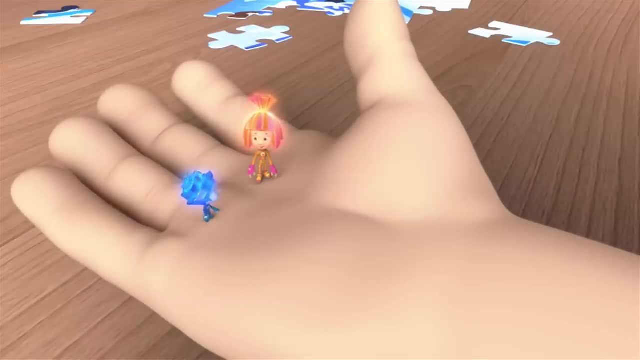 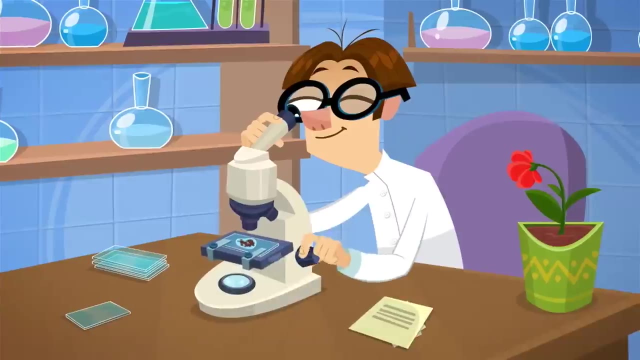 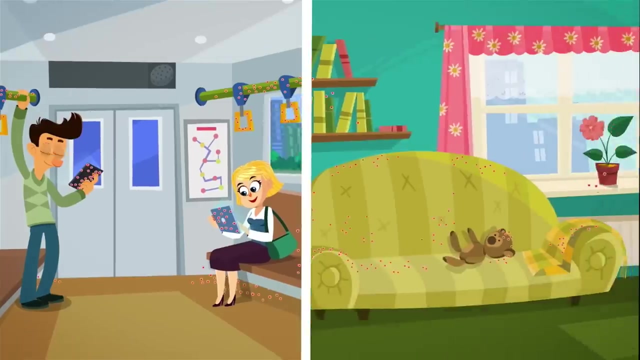 He's got a microscope We can take a look at some germs. Germs or microbes are such tiny creatures we need a microscope to see them, But they live everywhere: In the earth, the water, throughout the air. They're on everything, even on us. 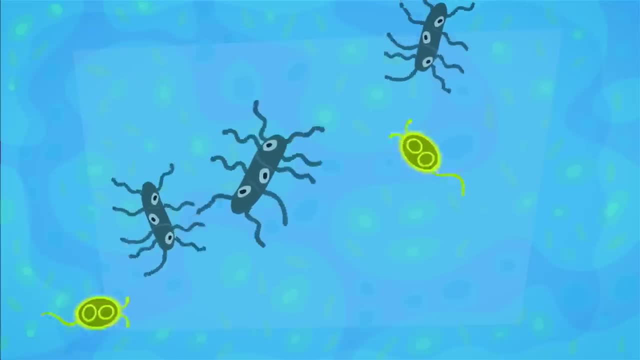 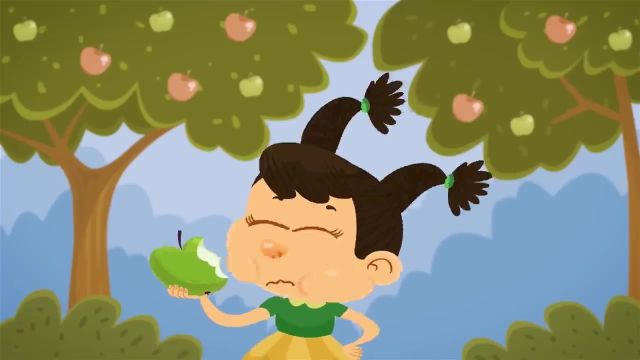 Some microbes are able to move around with the help of filaments or tails. Lots of microbes are harmless, but there are some dangerous ones too. If they get inside of you, through your nose or your mouth, they could end up with a sore throat. 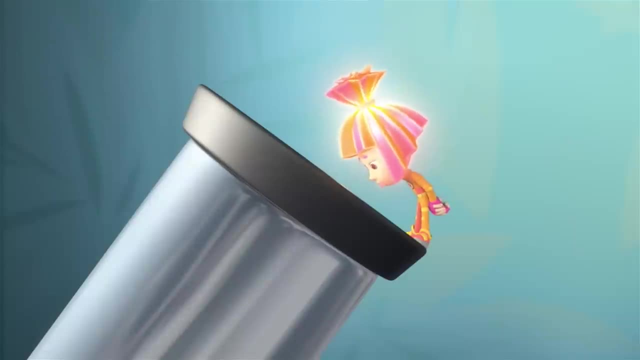 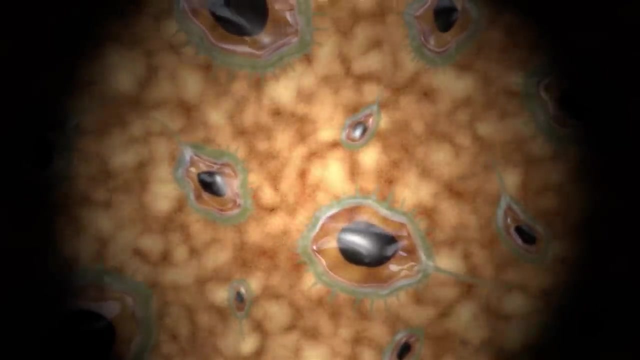 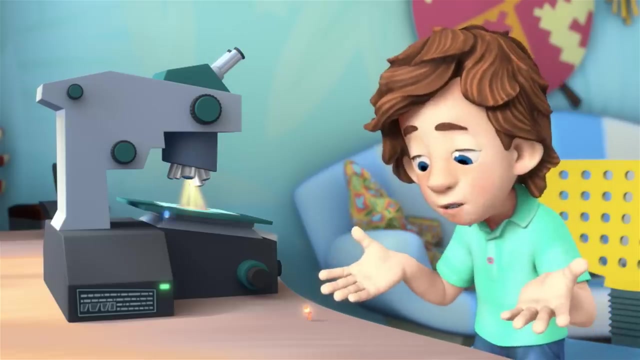 or a stomach ache. Turn it a little more. Stop Now. take a look, It's horrible. Hey, let me take a look. Wow, they're so scary. Hang on, Do I really have germs like that living on my hands too? 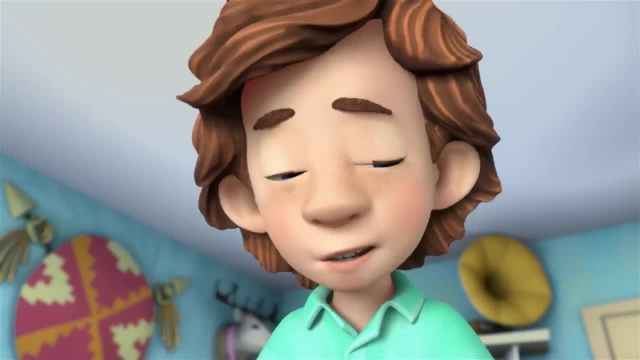 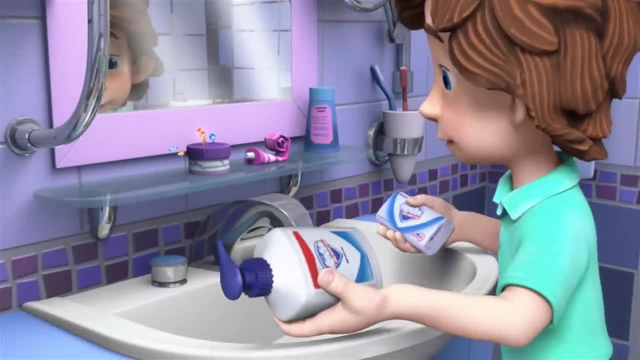 You got it, But I washed them uh, seven times With soap. I use soap to get rid of germs, not just water. So which soap should I use? Either This one, that one. They are both antibacterial. 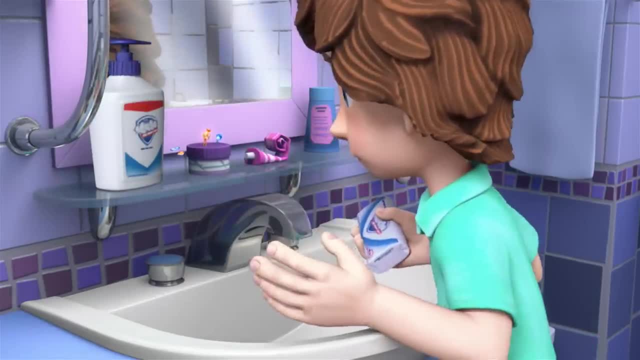 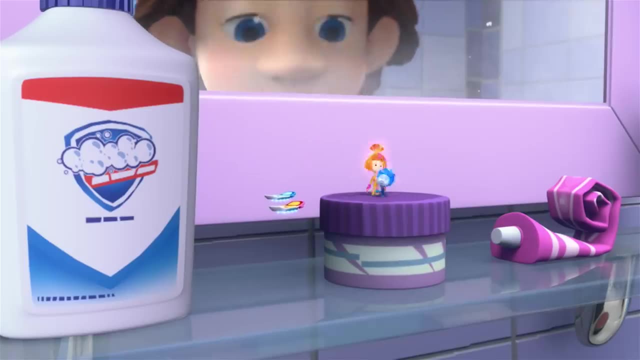 so they kill bacteria. And what about germs? Will it kill them? Of course, Bacteria is just another name for germs. They're the same thing. Wash Tom Thomas. give me a drop of that liquid soap. I want my hands to be real clean. 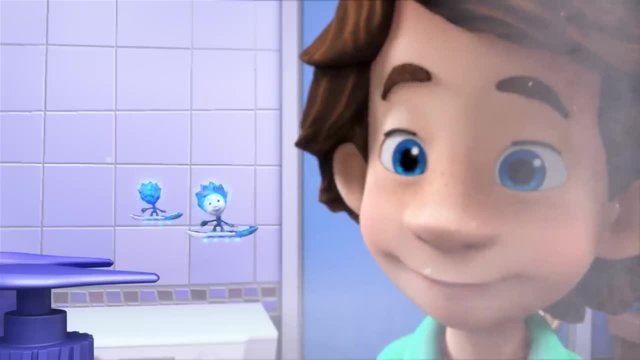 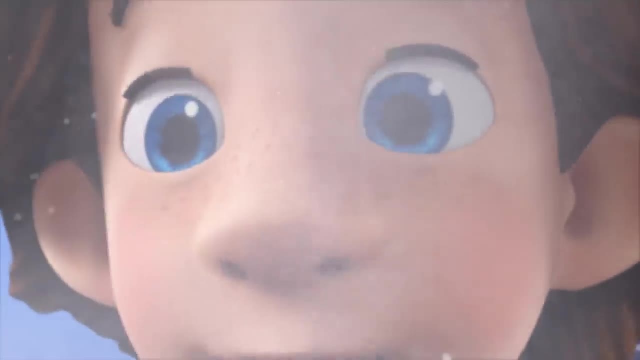 Good job. That's the spirit, Hooray, Let's go put that puzzle together. All right, but doesn't it have germs all over it And they're on the soccer ball? What are we gonna do? I think we should clean them with soap. 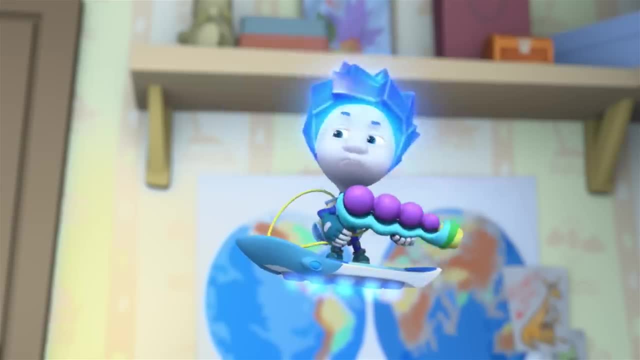 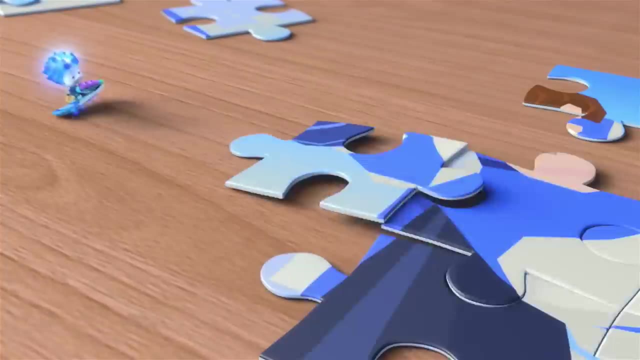 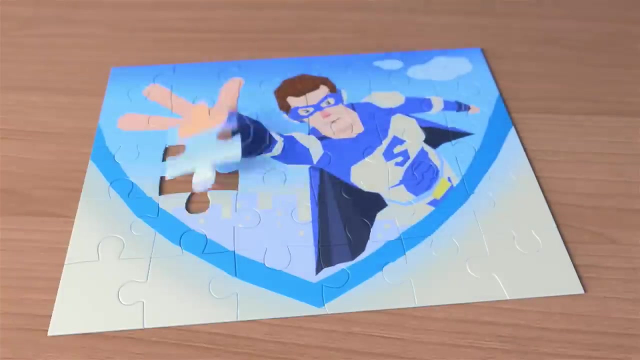 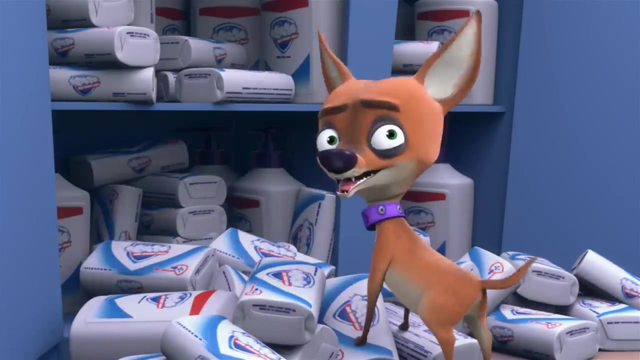 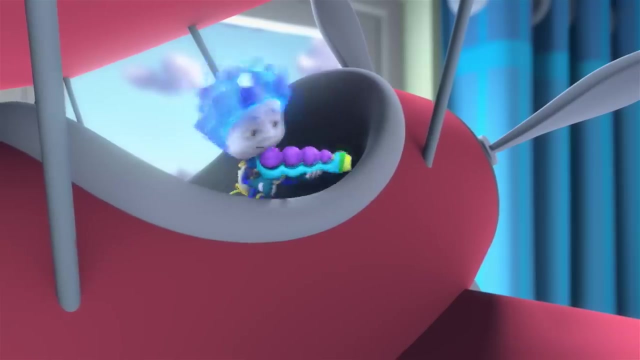 No, clean the whole room. You're right, I can't do that. I don't feel like doing it. I'm gonna go get some more soap. Oh, You're right, I'm gonna get some more soap. All right, let's go. 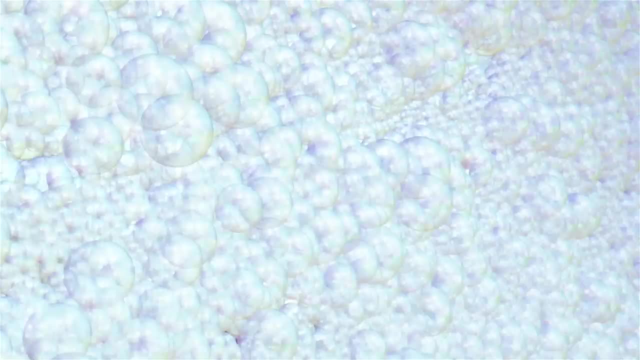 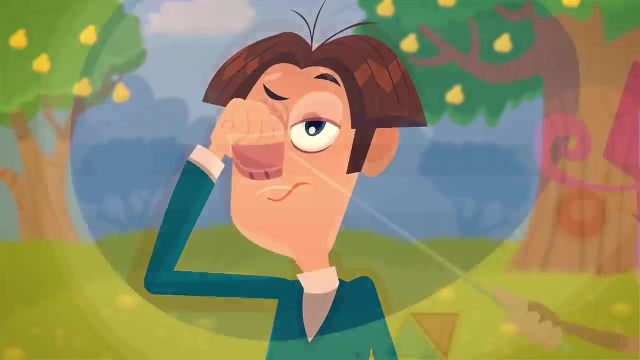 We're going to go get some more soap. I'm gonna go get some more soap. We're going to get some more soap. We're going to go get some more soap. We are surrounded by millions of invisible microbes, including those that can cause an illness. 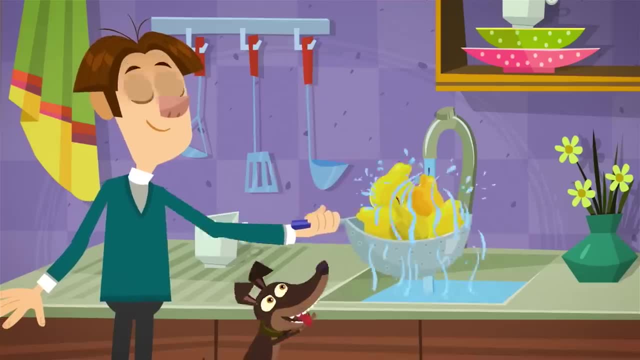 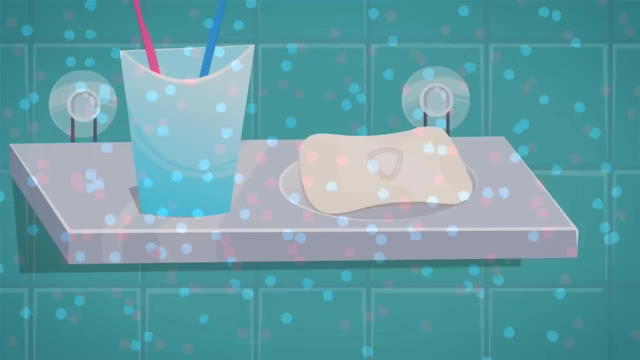 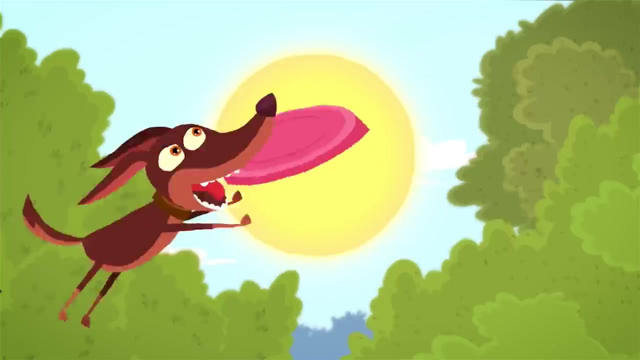 But there is no need to be afraid of them if you follow these simple rules- only washed fruits and veggies. keep your home clean and wash your hands very well with soap, preferably an antibacterial one, and every day. antibacterial soap protects you for a few hours after it's been washed off. it not only cleans your 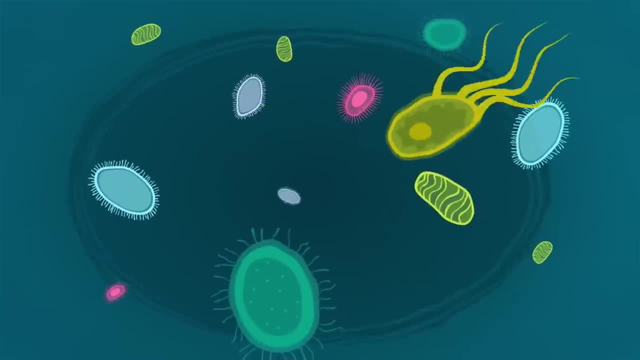 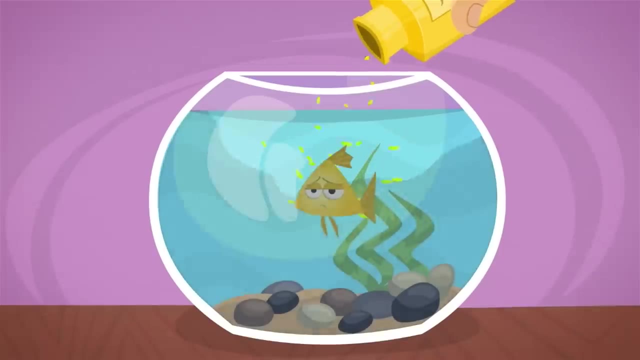 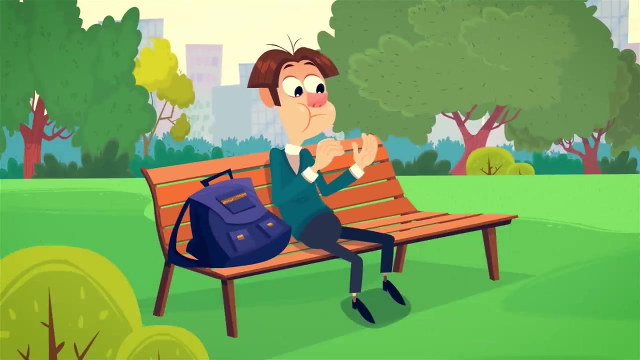 hands, but also stops germs from reproducing. there are useful microbes too. some bacterias can be added to milk to make yogurt and cottage cheese. others are used for purifying water. even inside of humans are a lot of useful bacteria that help their bodies digest food. 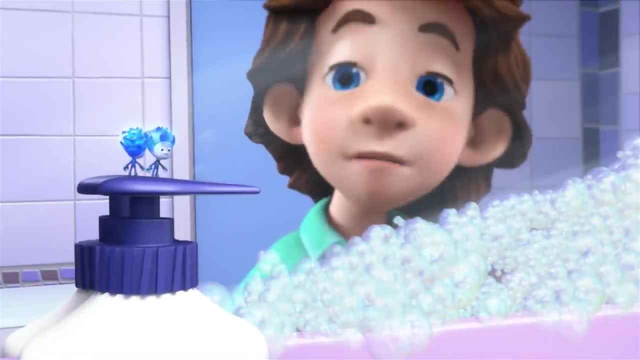 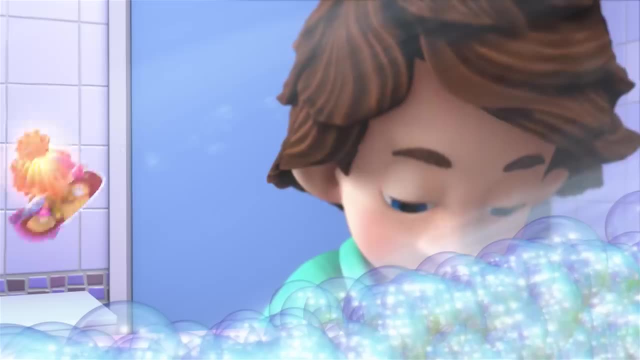 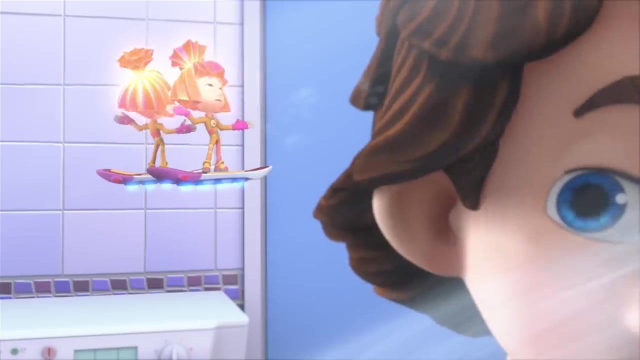 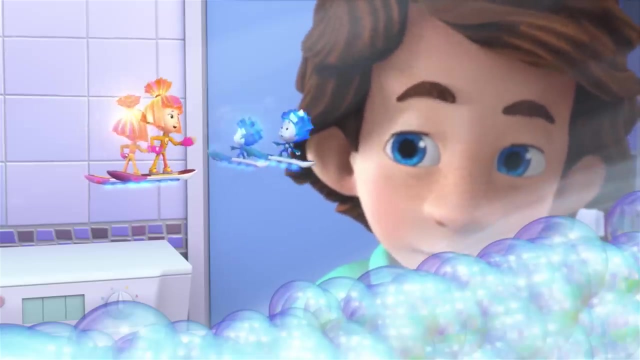 Nolik, what do you think? are there microbes living on the soap? I don't know. we should wash that too, just in case. washing the soap with so, so there won't be any germs on it. you gotta be joking, listen. rid of all the microbes is impossible and unnecessary. you just need to protect. 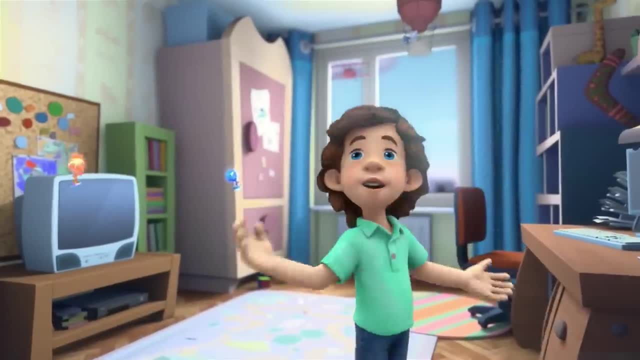 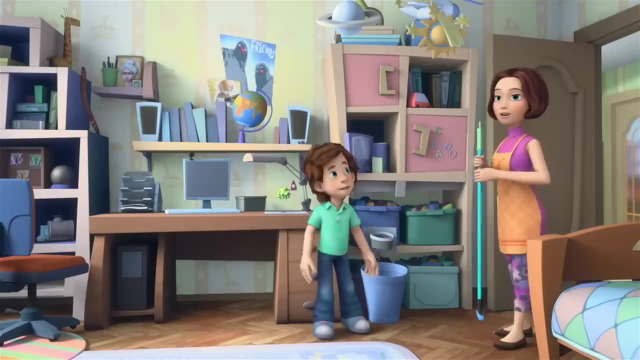 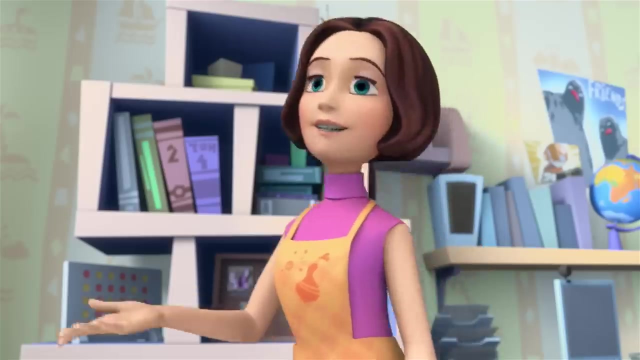 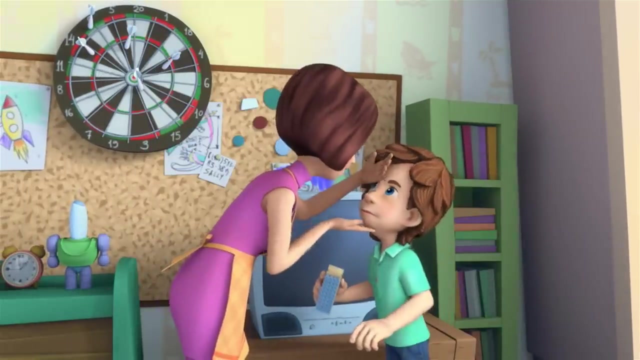 yourself from the bad ones. bacteria gone, Tom Thomas. I need a minute so I can mop your room, but I already washed it. what a good boy. the tables sparkling. oh, just look how clean it is in here. great job, what's going on? nothing, you're not sick, are you? no, Tom Thomas, you did a great job in here. only you're taking. 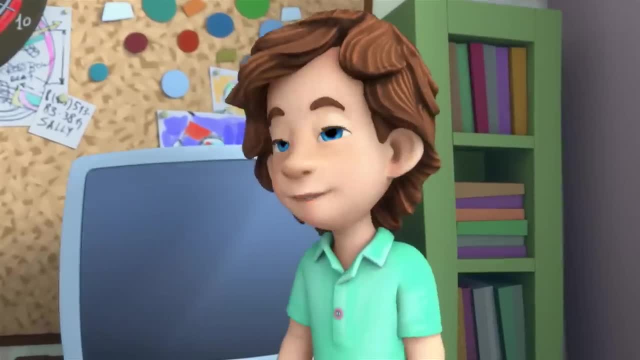 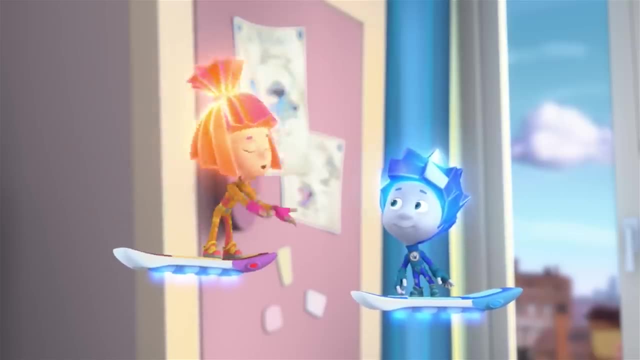 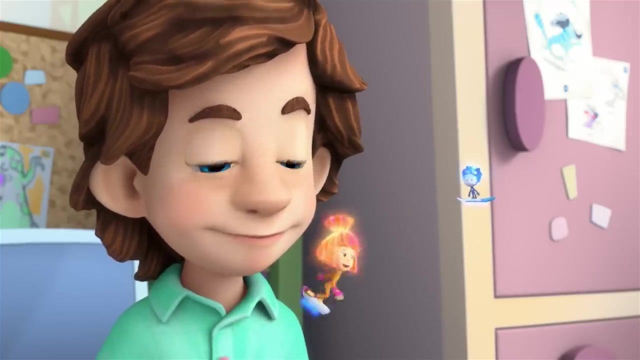 this cleaning way too far. understand? I've got you and do you get it me? get what? that the most important thing is to make sure you wash your hands with soap. okay to the germ fighters: making the world safer, one less term at a time. the iron, the iron. 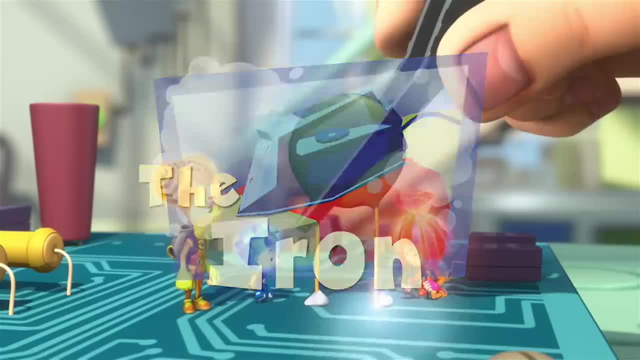 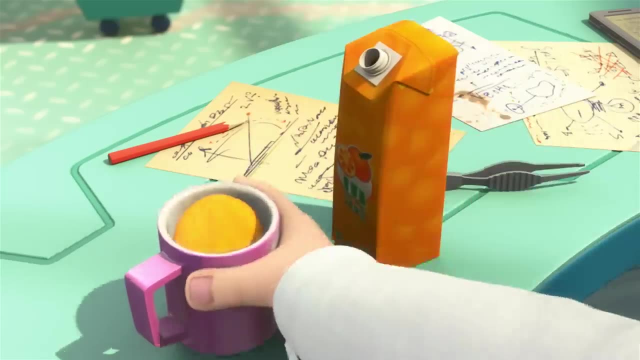 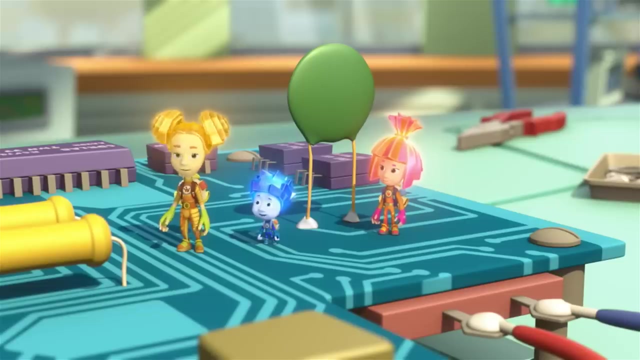 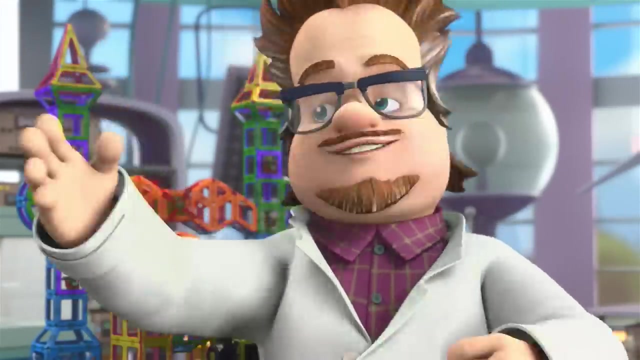 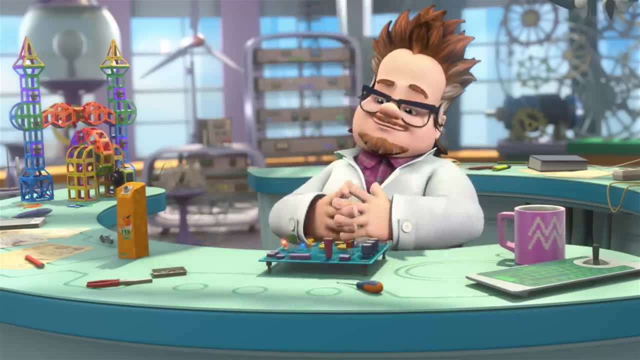 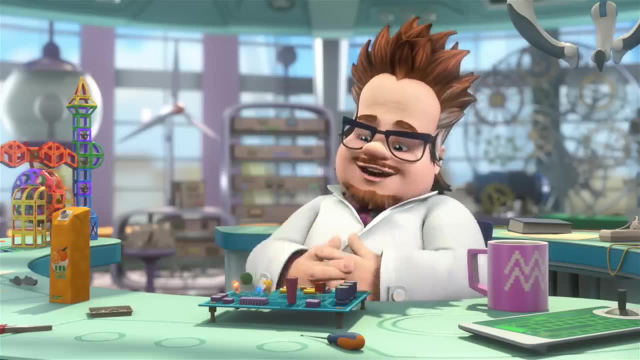 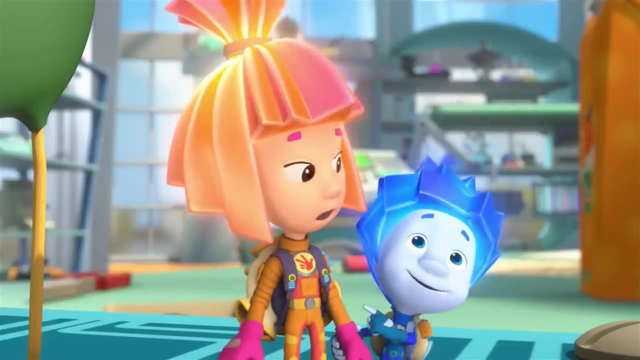 too modest, but fair and well-deserved. Wow, and you're getting it to you. Well, yeah, only sure when you found out I don't, you would meet your magicians. will they show it on TV? why, of course class. and during your speech, can you say hi to me and me, and me and sipka right say something like this I'd like to send. 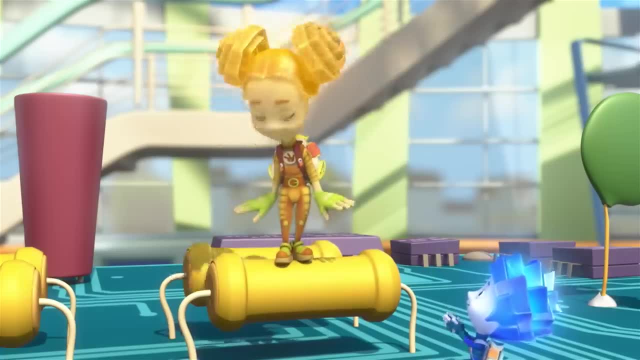 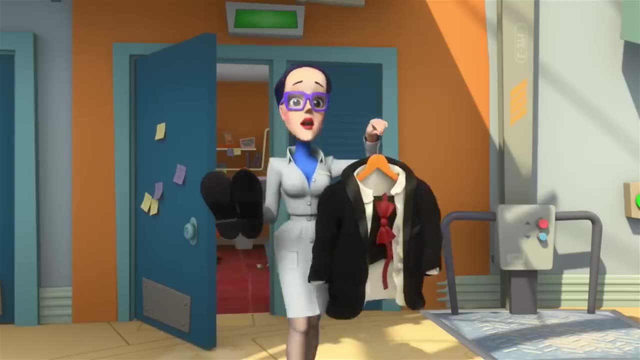 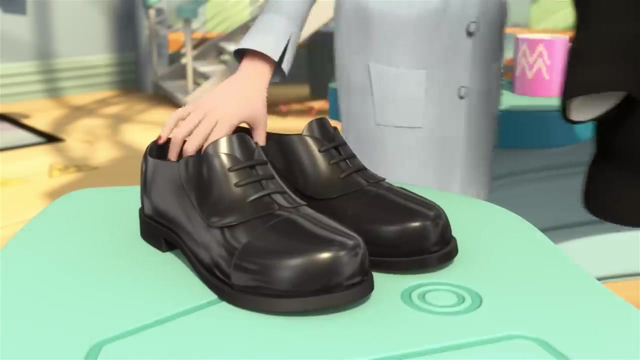 a big shout out to all my fixie friends. oh, that's a great idea. that way everyone can know about fixies. professor, you genius, didn't I see an iron in here earlier? mm-hmm, huh, oh. oh. come on, Elisa, there's no need for that, I'm not going. 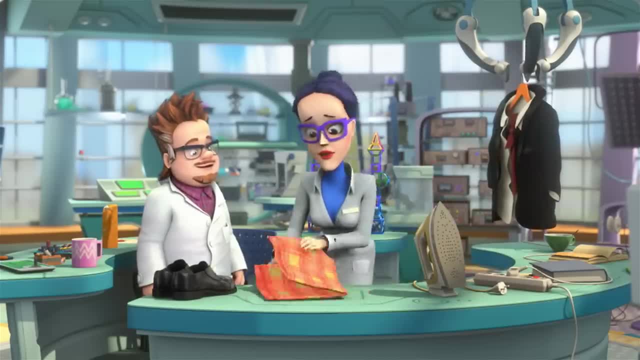 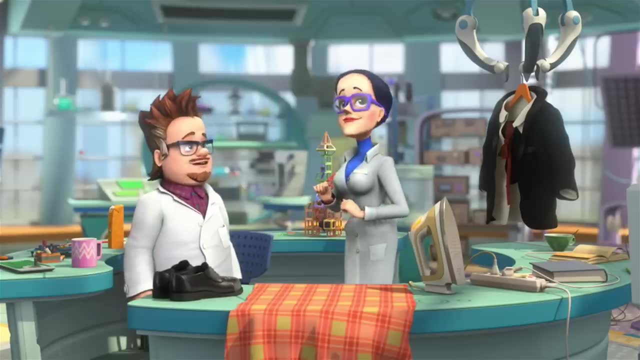 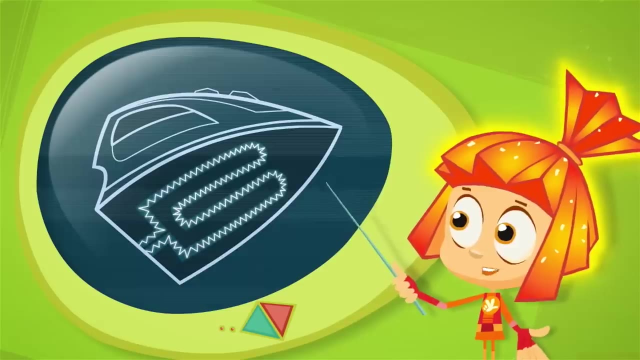 to argue with you. you have to look just perfect, otherwise everybody is going to think that I don't take care of you. first we'll let the iron warm up and then I can iron your suit. the most essential part of an electric iron is called the heating coil. it's hidden inside the iron soul plate. when the iron 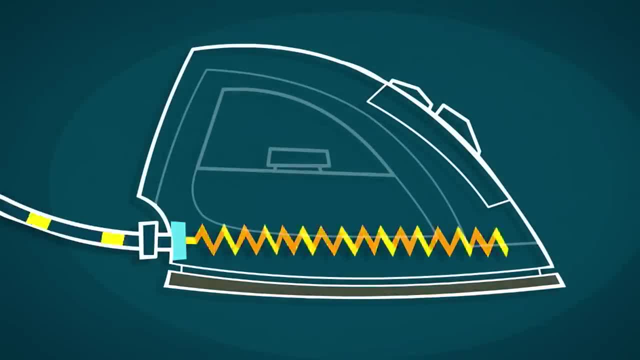 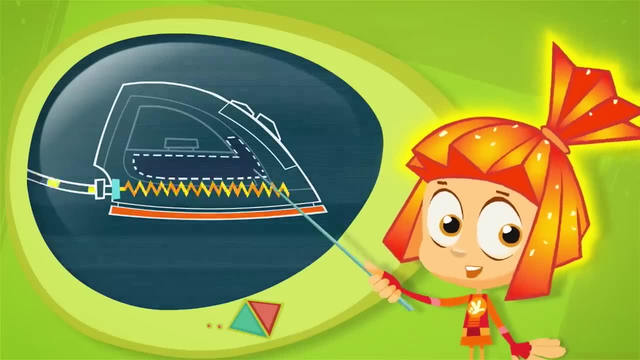 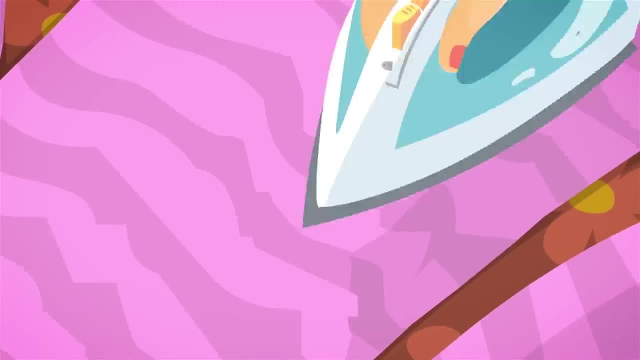 is plugged into an electrical outlet, the coil gets hot and heats up the soul. people use a hot iron to remove the wrinkles from their clothing. irons also have a water container. when the water gets hot, it turns into steam. steam comes out through the holes in the iron sole, making it even easier to remove. 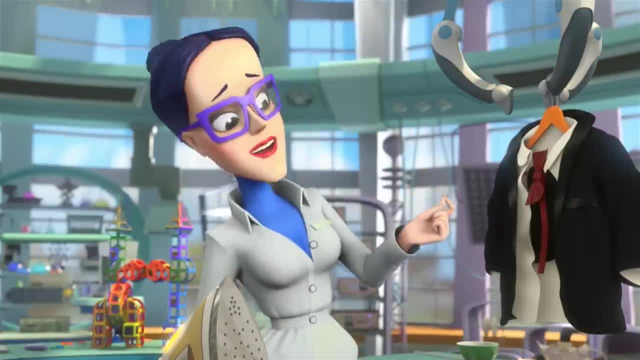 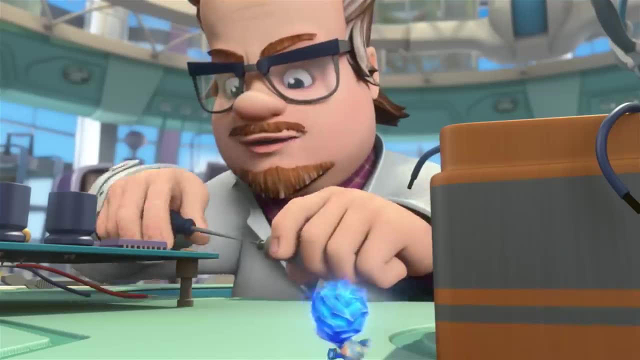 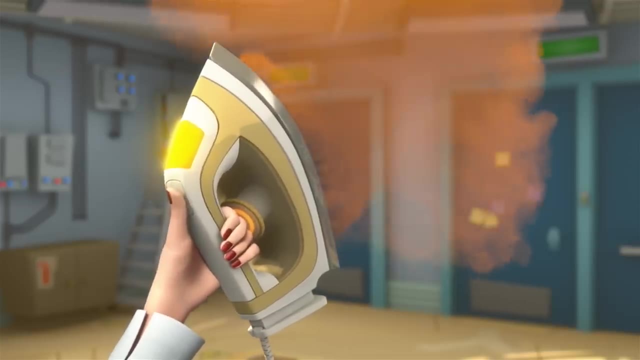 wrinkles. well, well, this sure is hot. all that's left to do is pour some water into it. professor, this is water, right? yeah, yeah, it's water. no, wait, wait, wait, it's not water. It's not water. Then what is it? Well, it's uh juice. 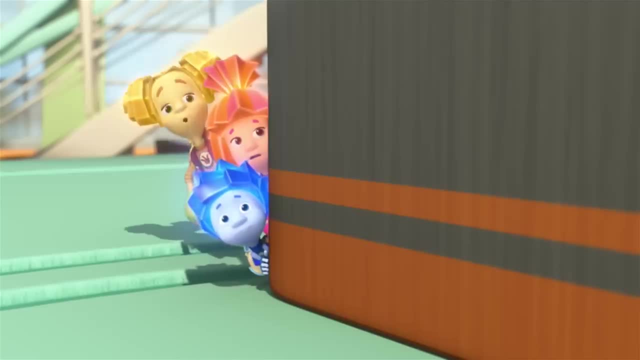 Juice, Yeah, juice, Oh no, The poor iron won't last Cute And it smells like crud. I broke the iron. It's awful. No, no, no, no, no, Elisa, Don't be so upset. 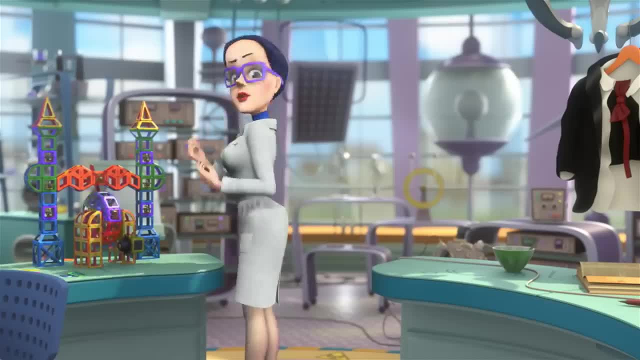 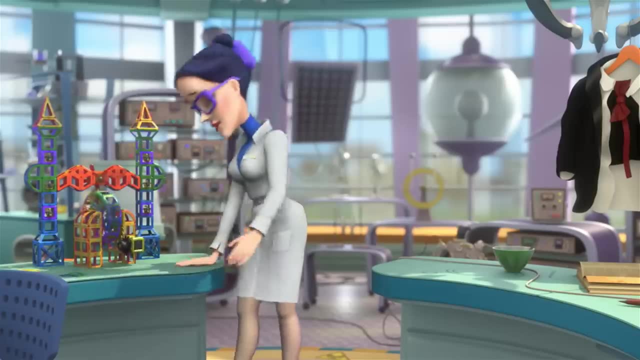 Don't be so upset. It's the genius of the year ceremony and you'll be in a wrinkled suit in front of the whole country. Oh, I won't survive. Elisa, hang in there, Be careful, Be careful. 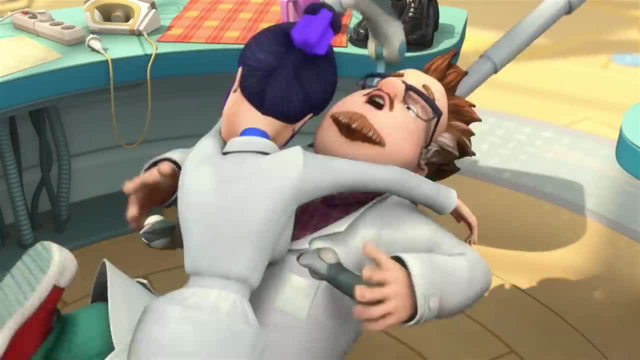 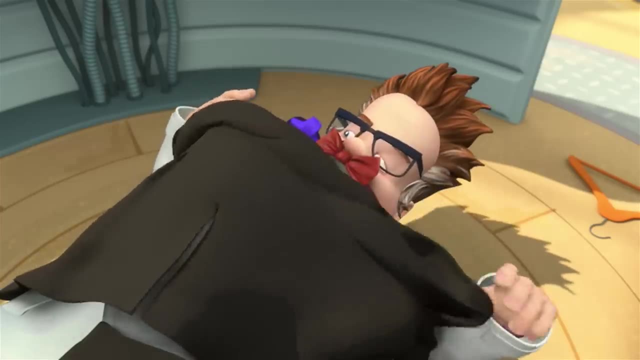 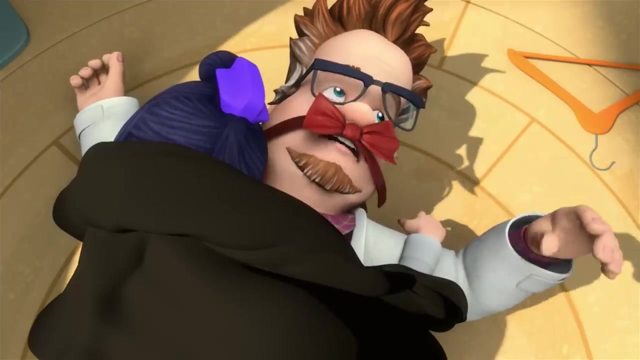 Elisa, Elisa, Professor, you're genius, Are you? all right? Couldn't be any better. We're going to go fix that iron for you And while we're doing that, you go fix Elisa. That would be great. 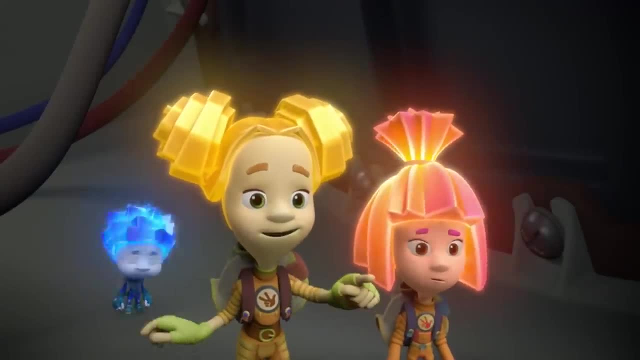 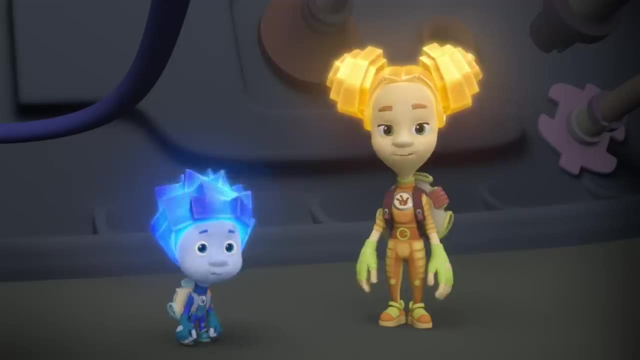 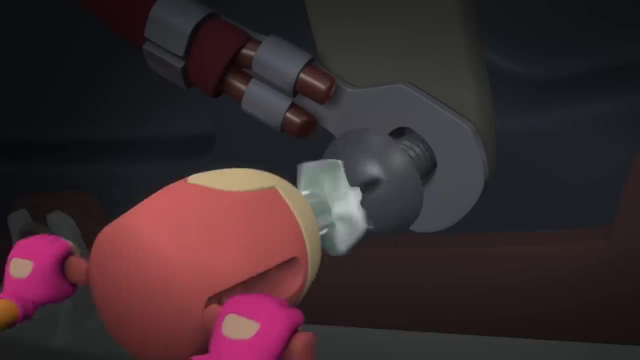 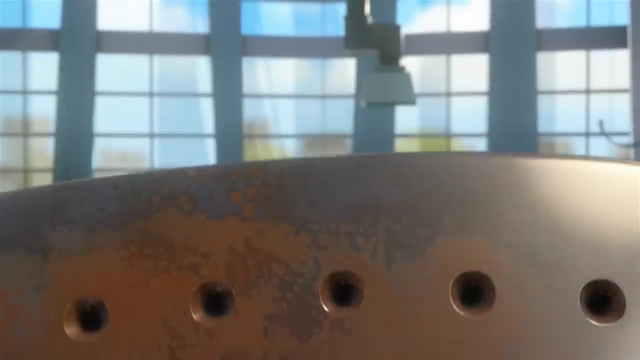 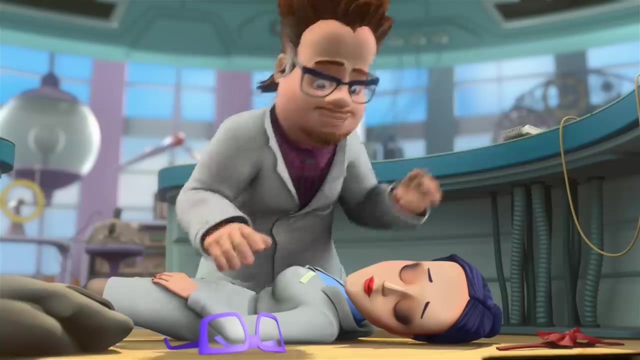 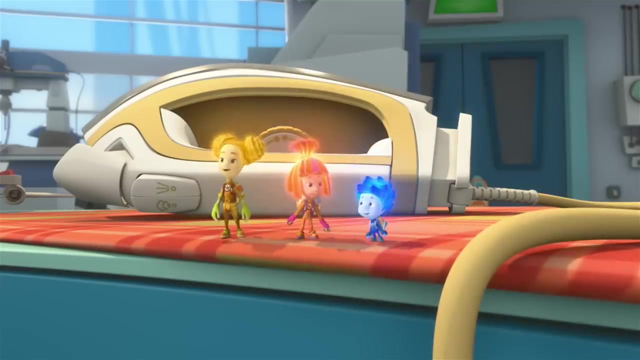 Look over there, I'll fix the contact. You and Nola can scrape that burnt juice off the iron. Mm-hmm, Mm-hmm. Elisa, Elisa, please wake up. We did it. your iron is fixed. 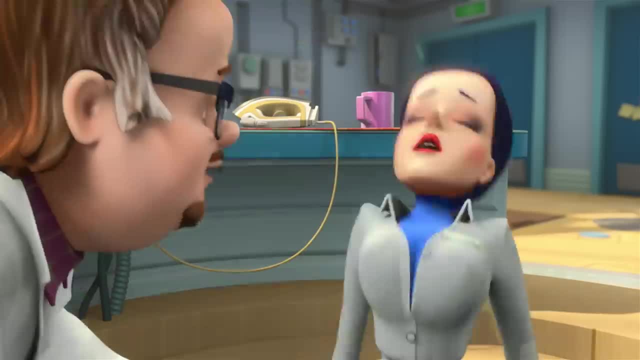 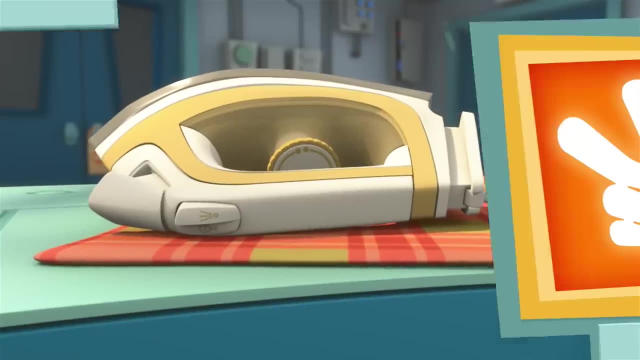 Elisa, you should see the iron, it's working. What? And I'm just lying around here? I have to hurry where's the iron And your suit? Wrinkled clothing is not very beautiful, And that's why, since ancient times, 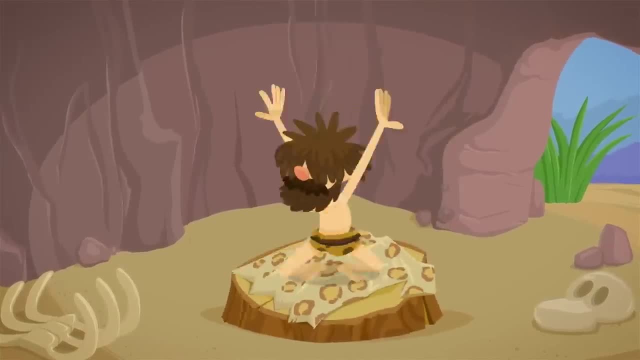 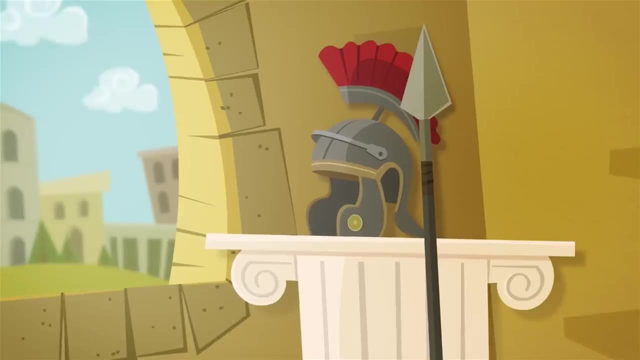 people have been trying to find different ways to get rid of wrinkles. For example, long ago, people would put their wrinkled clothing under a heavy flat rock. In ancient Rome, people used to beat their crinkled garments with a metal hammer. 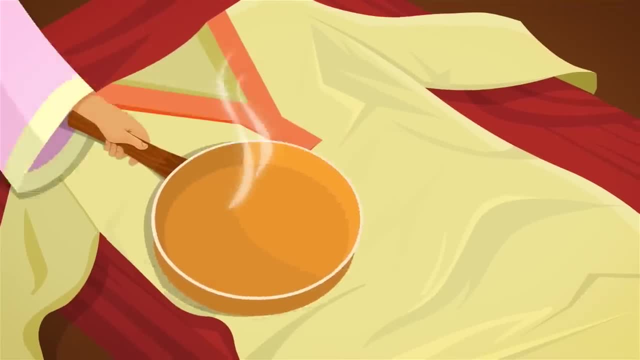 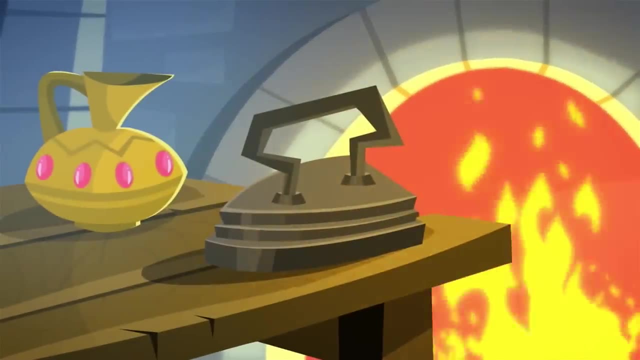 And in China, fabric was ironed with hot frying pans. Irons with a shape like what is used today appeared during the Middle Ages. They were made out of cast iron and needed to be heated up on a stove before they could be used. 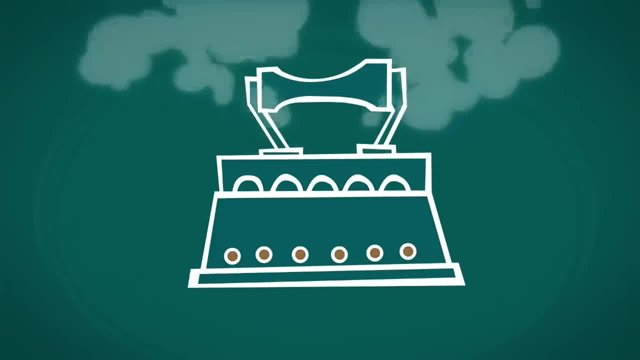 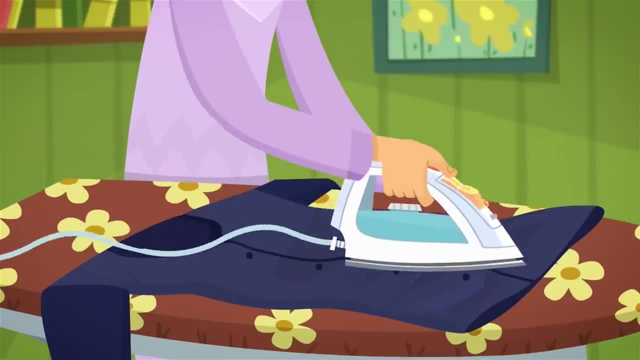 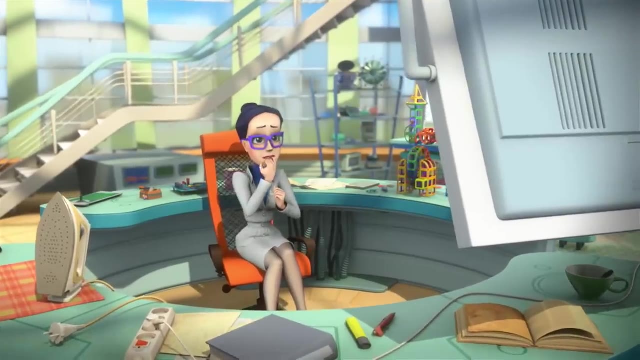 Later, people came up with irons that were heated by putting hot coals inside, And finally, in the 19th century, a convenient electrical iron was invented and has been used ever since. And the prize for Genius of the Year goes to: 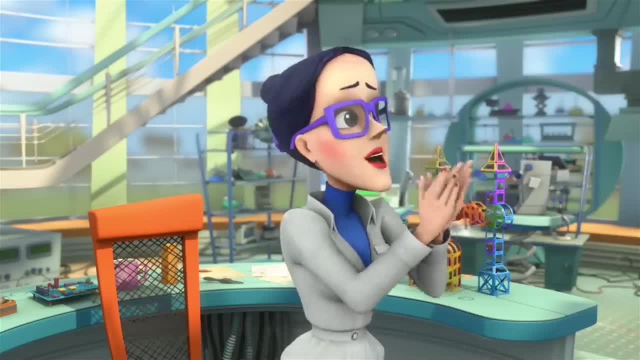 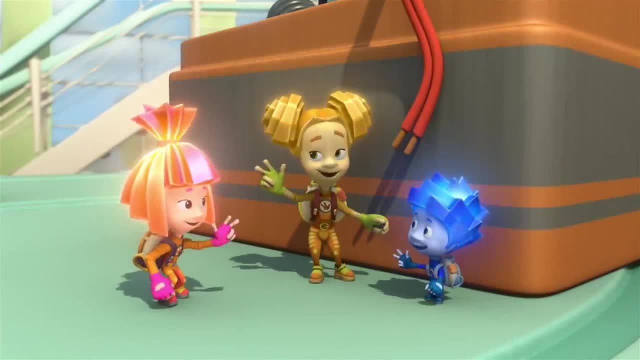 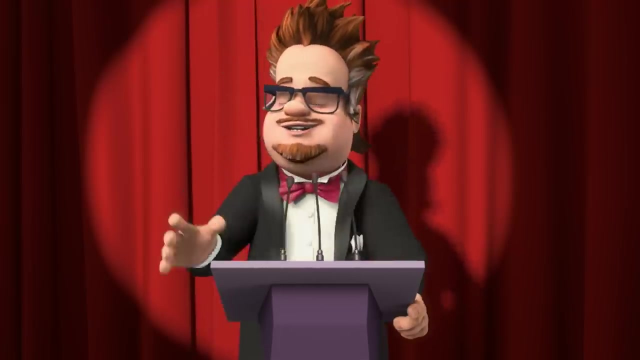 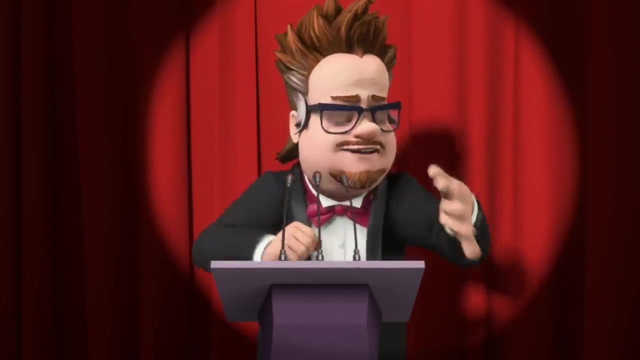 Professor Eugenius, Bravo, Bravo, Professor, Titties, Titties. I thank you, I give my sincerest thanks to you And may I take this opportunity to send my greetings to Fix, Uh, Uh, To all the Fixers. 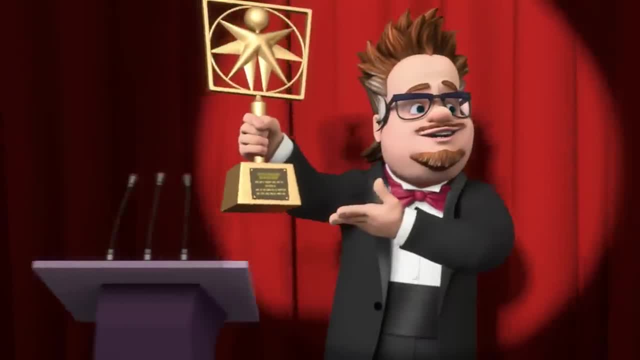 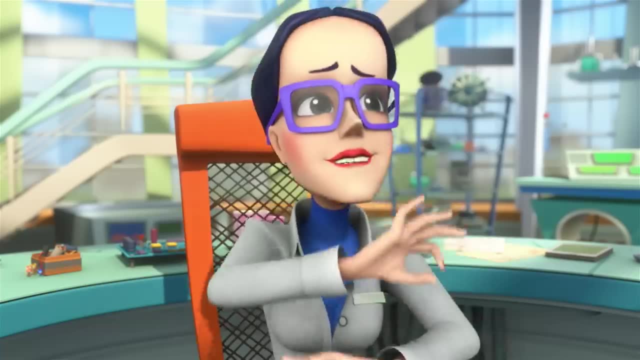 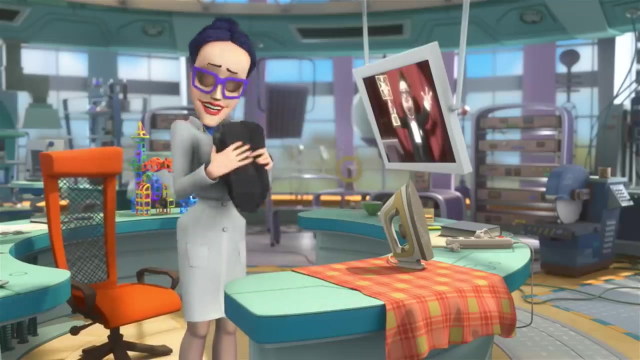 S-S-Sists, just give me the prize. Oh, that was quick thinking, Brilliant, He is just astounding. Perfection from head to toe. Huh Well, practically perfect, Ha-ha-ha-ha-ha-ha. 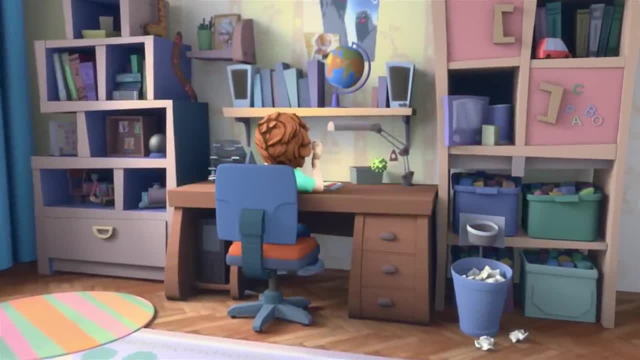 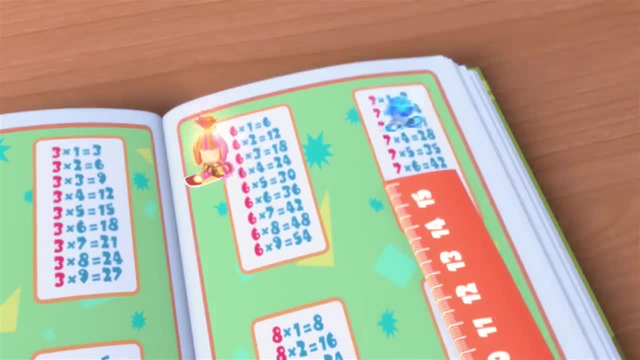 Vitamins. Seven times five is thirty-five. Seven times six, Um, uh, wait a sec. Uh, It's uh. Tom Thomas, are you ready For what? For our walk, Did you forget? Oh yeah, 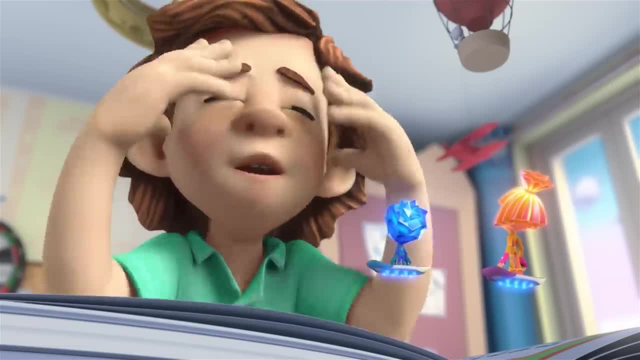 I'm having such problems with my memory. I keep trying to memorize this table, but I can't. If you want to improve your memory, you need vitamins, Vitamins. Well, How's it going, Tom Thomas? Not well. 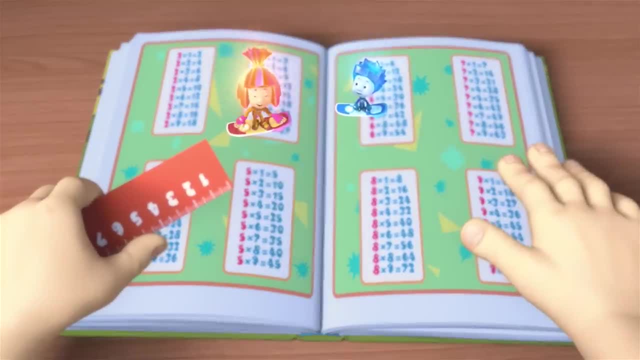 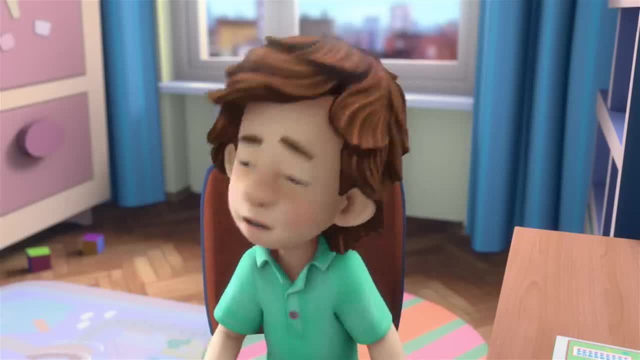 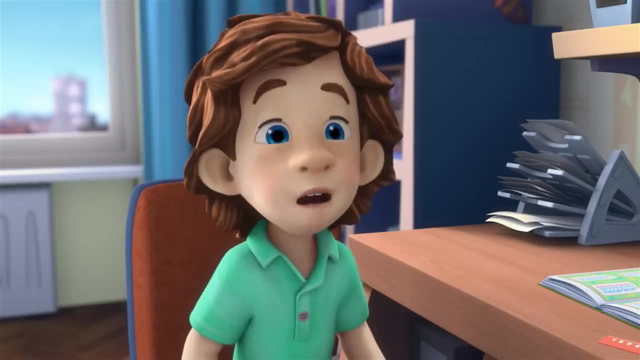 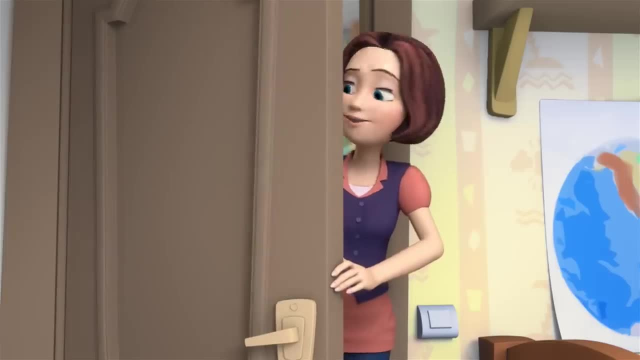 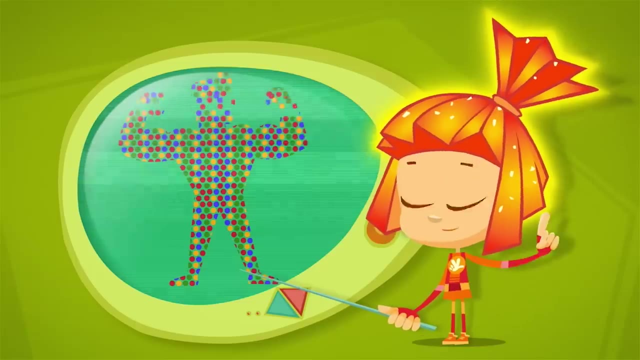 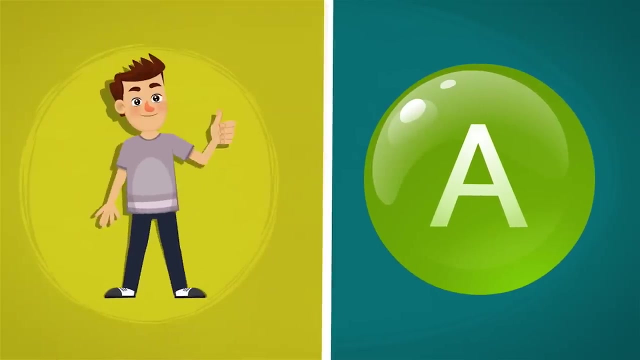 Shh, just a school friend. Well, all right. Vitamins are very important for people's health, even though you don't need much of them. For instance, vitamin A is necessary for good eyesight and normal growth. Vitamin C helps keep you from getting sick. 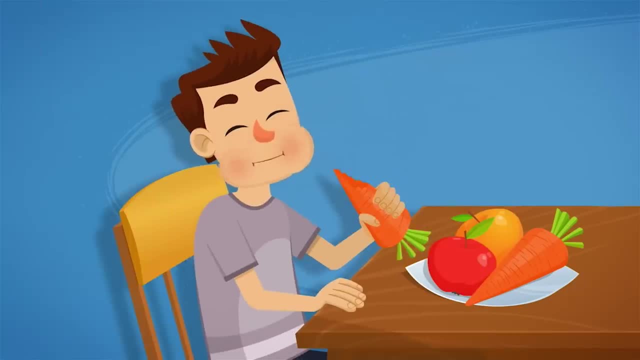 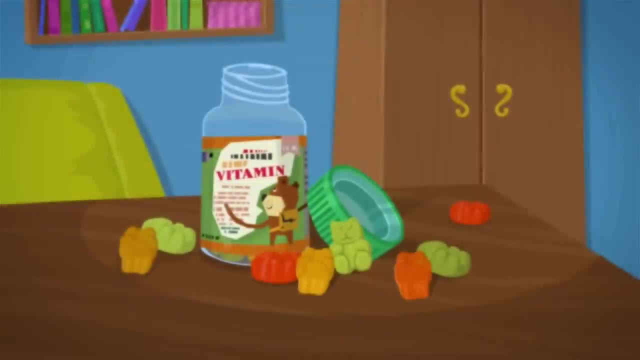 Vitamin D makes your teeth and bones look younger. Vitamin C- Vitamin D. Vitamin C- Vitamin D. Usually people get the vitamins they require from a diet of fruits, dairy vegetables and other healthy foods. But if someone still isn't getting the vitamins their body needs, then doctors recommend taking special vitamin pills. 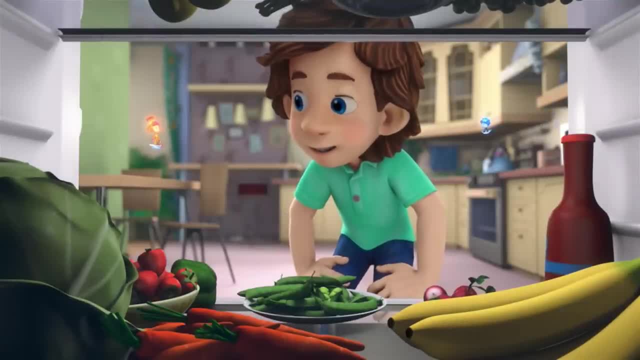 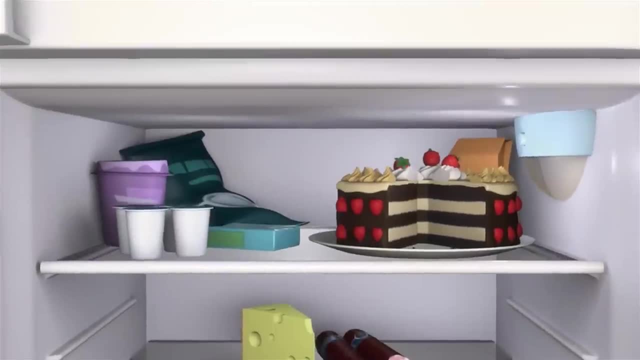 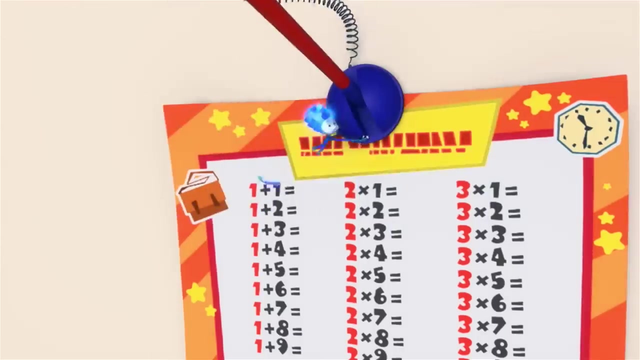 Alright, take out some vegetables and some fruit And some berries. They have a lot of vitamins too. Forget about it. We're strengthening your memory with vitamins. And you've studied the multiplication table at the same time. Alright, then There are three cherries in each pile. 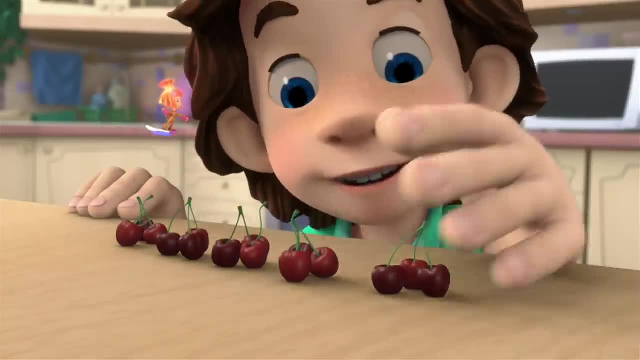 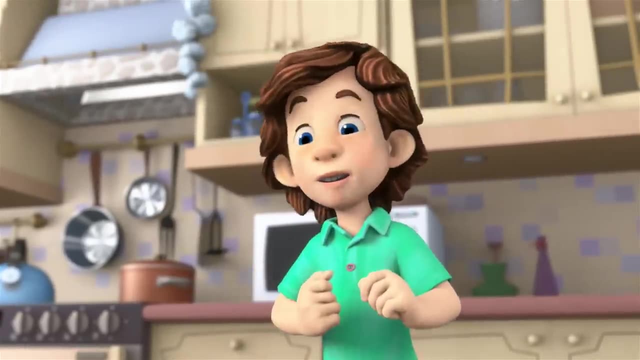 Tom Thomas eats five piles. Go on, eat, eat. So here's the question: How many cherries did Tom Thomas eat all together? I don't know What'd you say. I said I don't know. Try counting those pits then. 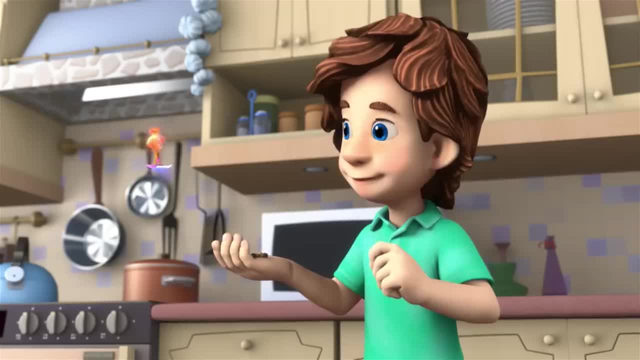 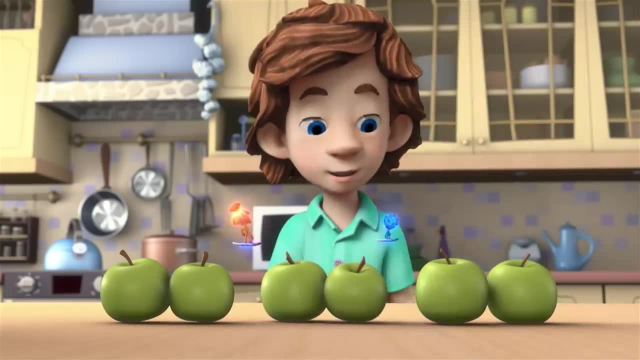 Huh, Fifteen, That's right, And that means that three times five equals fifteen. Now try my problem: Tom Thomas ate three pairs of apples. That's easy. The answer's six. I just couldn't find more apples for that one. 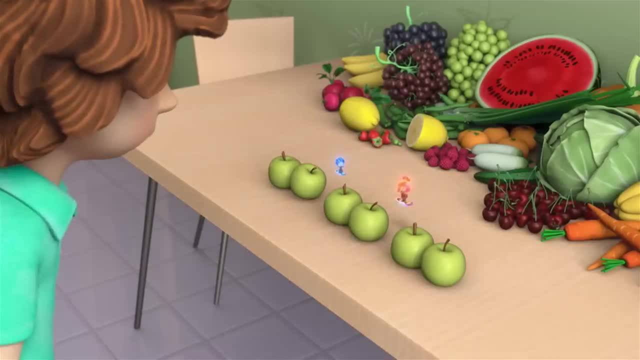 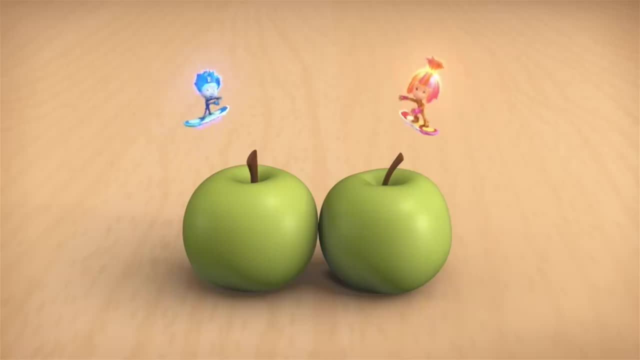 Tom Thomas quit slacking off. To get this problem right, you have to eat the apples. They have vitamins, I know, But if I eat these do I get a stomachache? You have to eat with a stomachache. That's a good idea. 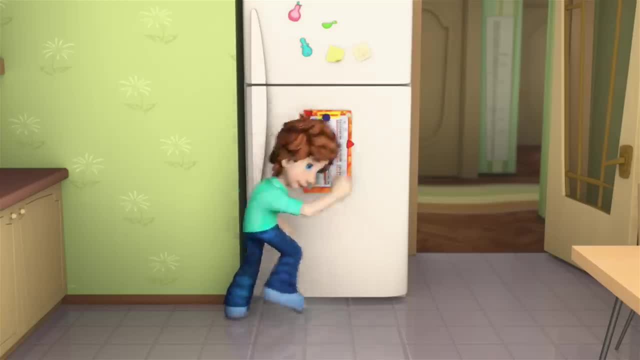 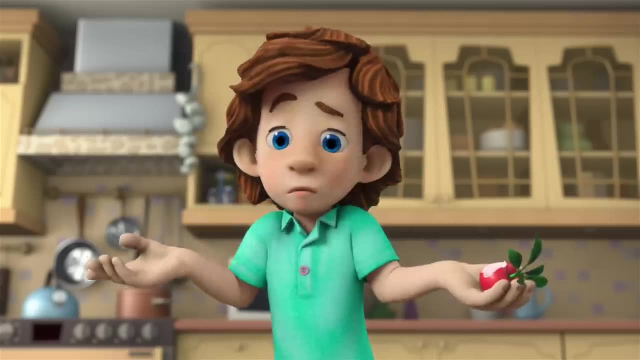 That's great, Tom, You've got it. Tom, I'm not sure about you, but the only way you can do this is to eat those from Tom's bowl. You can't eat a whole, whole plate of apples. You gotta eat them in one bite. 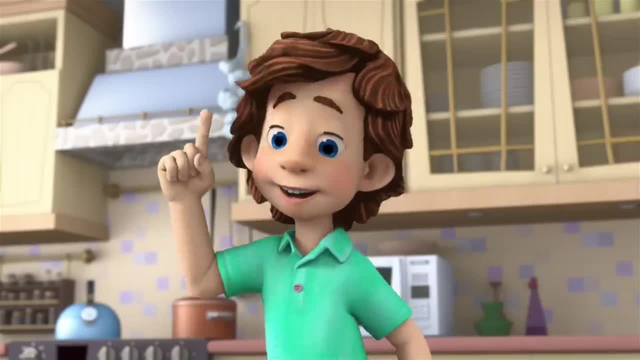 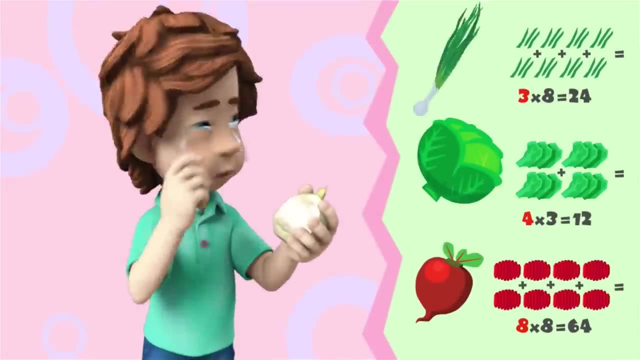 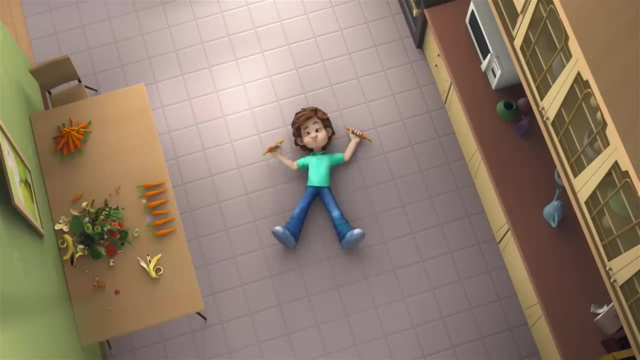 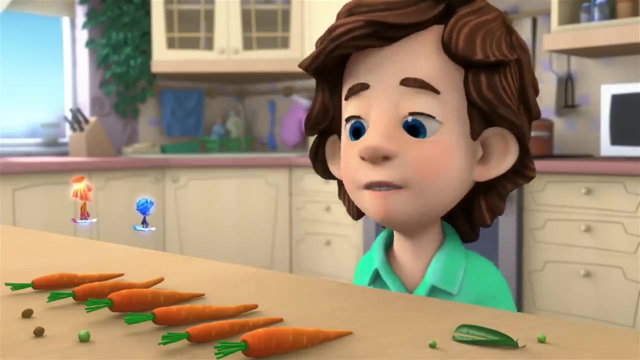 Go on. So how many cherries does Tom have? Ten, Ten, Ten. That's all I can't eat anymore. Keep eating. They have vitamins Anyhow. we don't have enough carrots for me to learn how to multiply by nine. 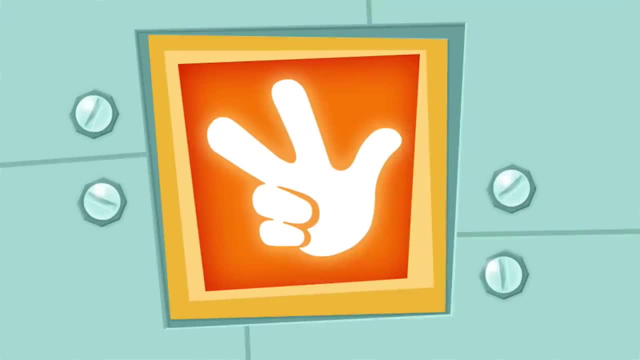 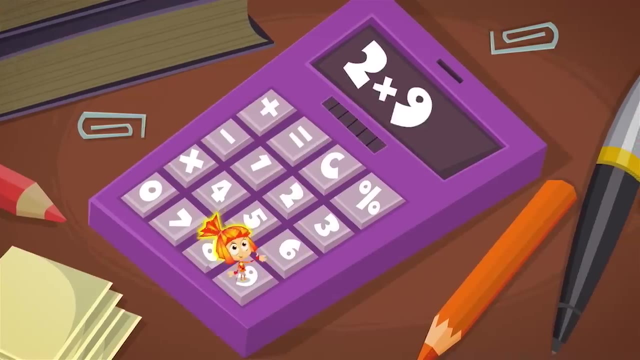 All right, then I'll help you To multiply two by three. all you need to do is just add three twos together. It's much harder to multiply a number by nine. That takes too much time to add. That's why at schools, they want you to memorize the table. 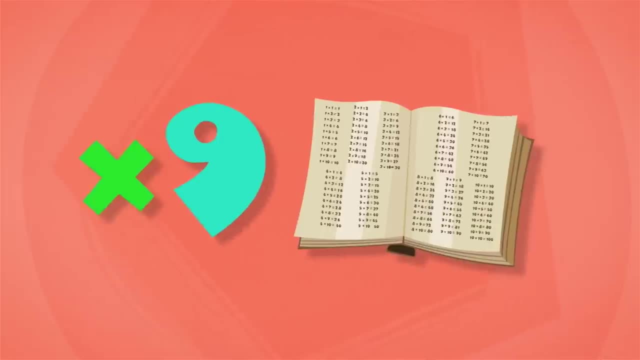 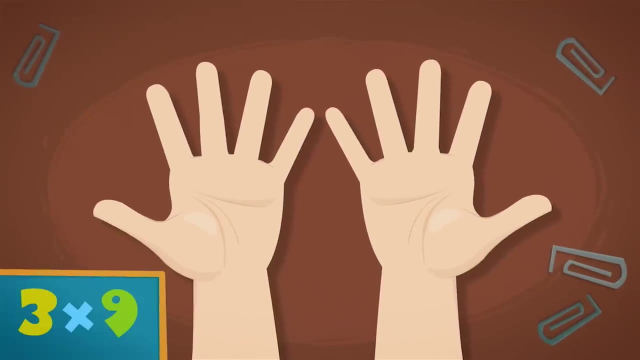 But there's a simple way to multiply by nine without the table or a calculator. Let's say you need to multiply the number three by nine. Put your hands face up in front of you Now, find the third finger from the left and bend it down. 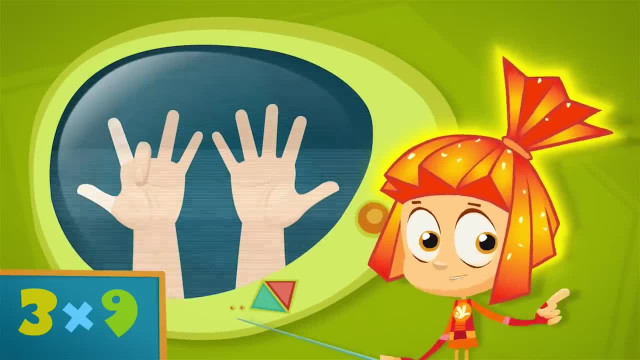 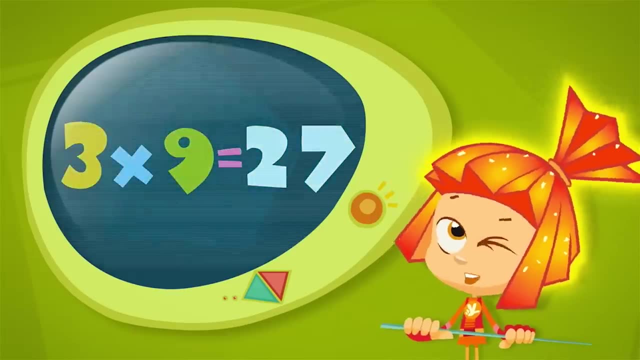 So what do we see? There are two fingers to the left of the bent finger and seven fingers to the right. Two and seven, Seven means that the answer is twenty-seven. You got it. Great, Let's do another problem. What is seven times nine? 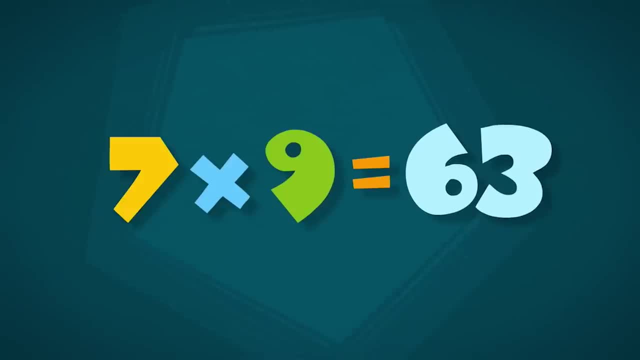 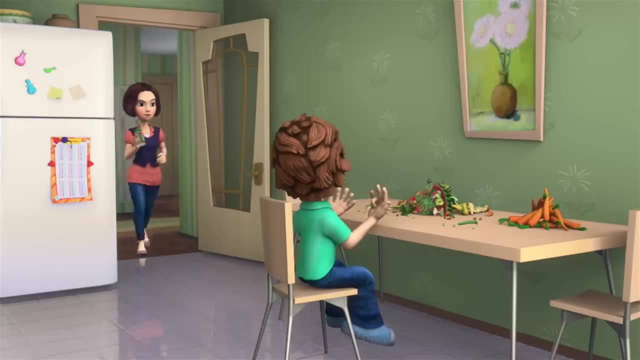 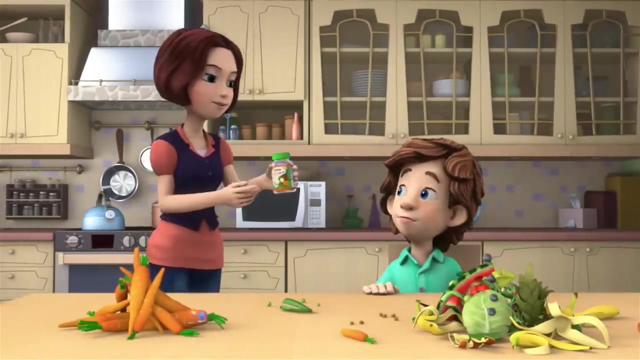 Here are six fingers and here are three. That's right. The answer is sixty-three. Tom Thomas, did you eat all of that? But you're the one that told me you need to eat vitamins. That's why I got these vitamins for you. 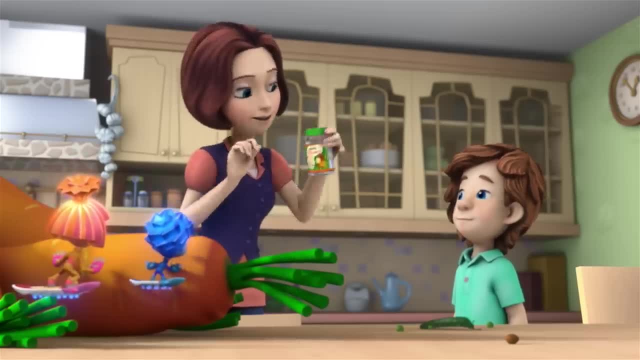 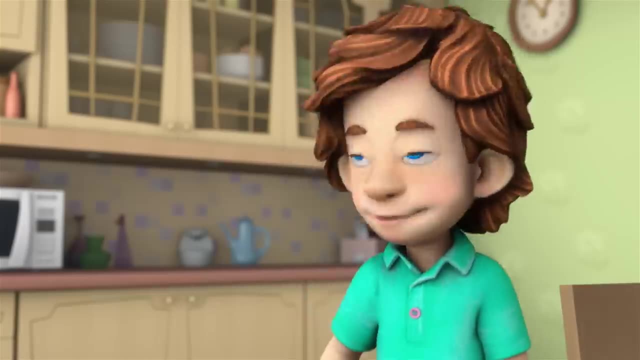 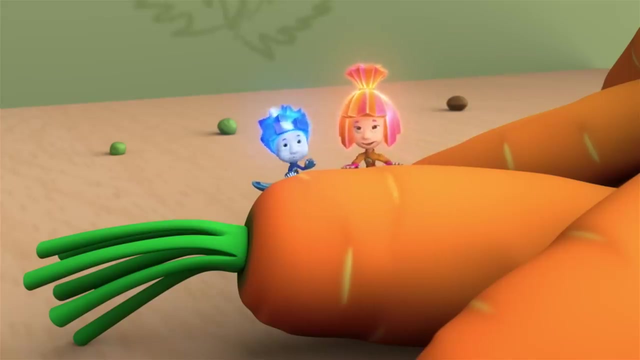 That little? What do you mean? Little? There's enough in this bottle for a month. Go ahead, try one. They're very good for you. They taste good too. Right, Better than an onion Or a radish. 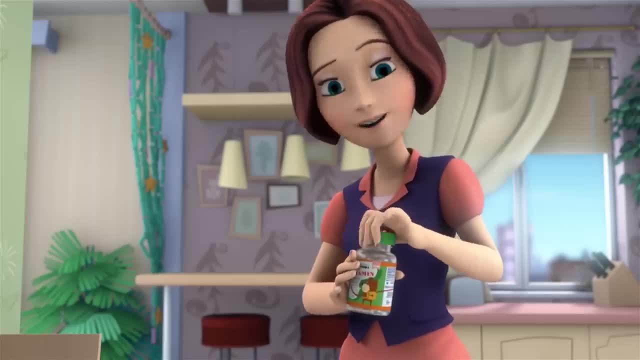 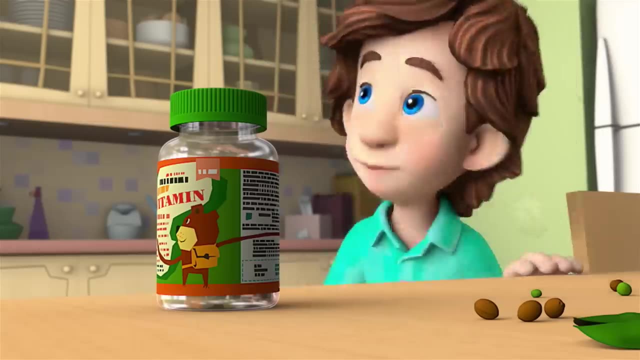 Can I have another one? No, that's enough. You shouldn't take more than one vitamin every day. I remember where I saw this. I saw the same kind of bottle with the green lid over at Katya's. Speaking of memory, let's check your multiplication table. 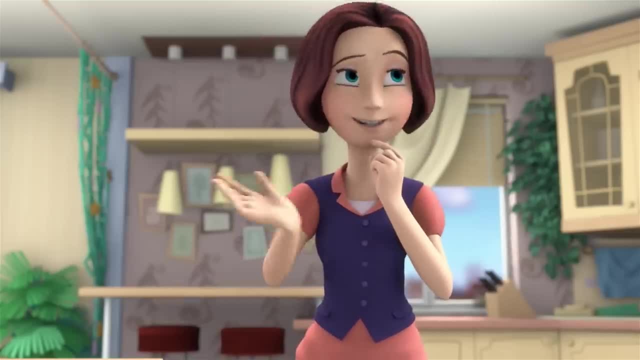 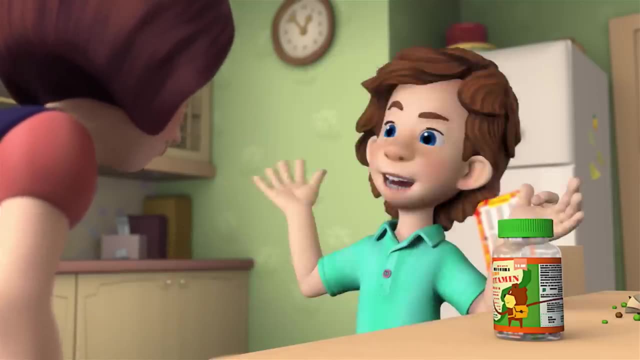 Let's say that. Let's say that you and Katya are each taking one vitamin a day. So how many have you eaten after nine days? The answer is eighteen Ha, Well done, It's getting better. Vitamins really work. 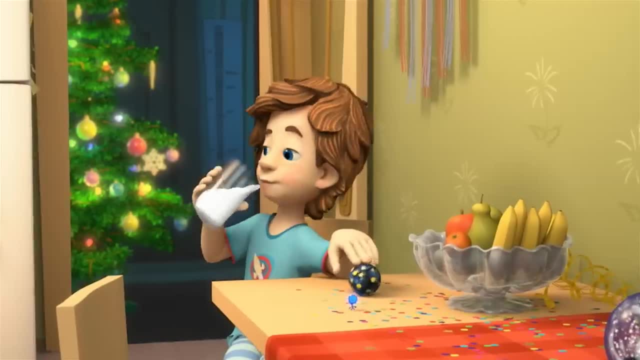 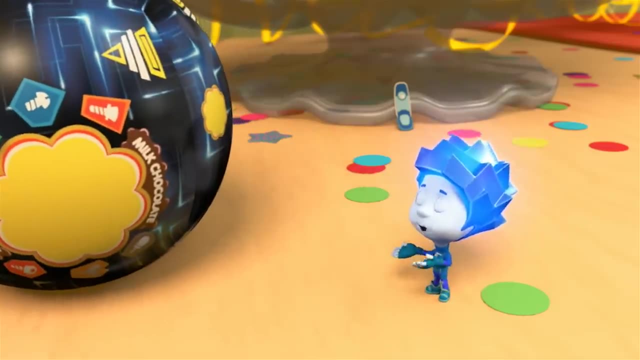 Chocolate, Tom Thomas. unwrap it already In the morning, Nolik. I really want to see the toy that's inside. Be patient, Nolik. That's all. I'm going to bed. Please don't touch it, okay. 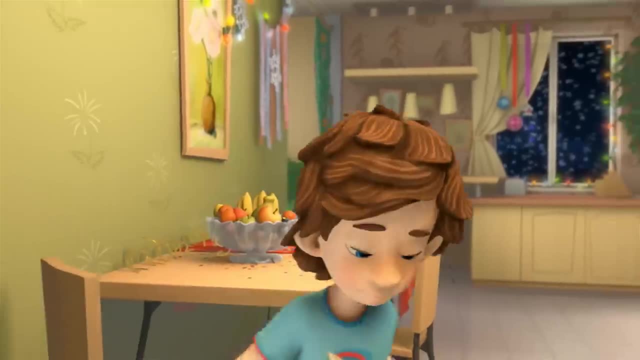 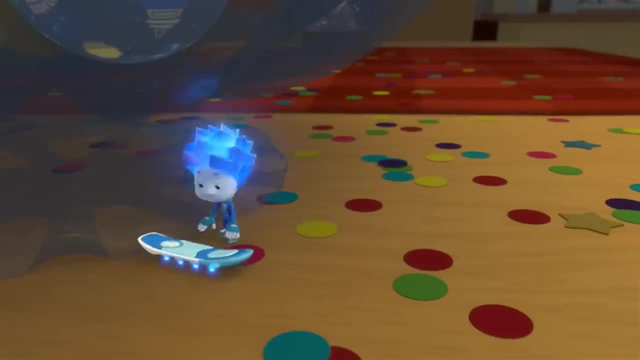 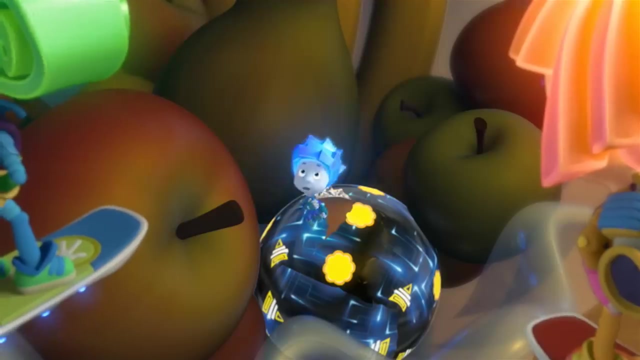 And you won't open it without me, right? That's the deal. Good night, Nolik. Uh-huh, And what are you doing in here, Me? Well, I was. Oh, it's a chocolate ball with a toy inside. 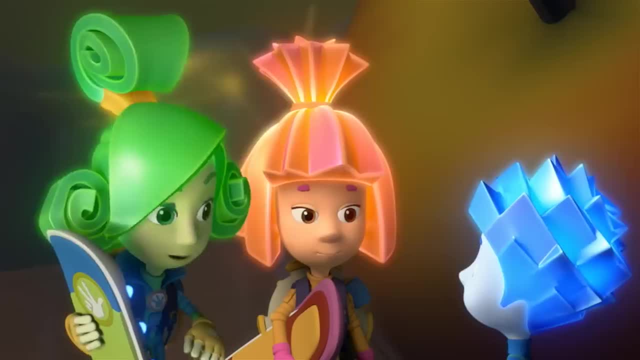 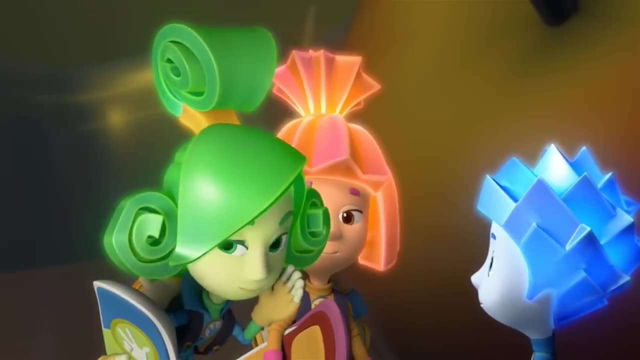 How interesting. Yeah, totally. Let's unwrap it and take a look. We can't Not until Tom Thomas comes in the morning, But if we're real careful he won't notice. A chocolate confection- Ew, A piece of perfection. 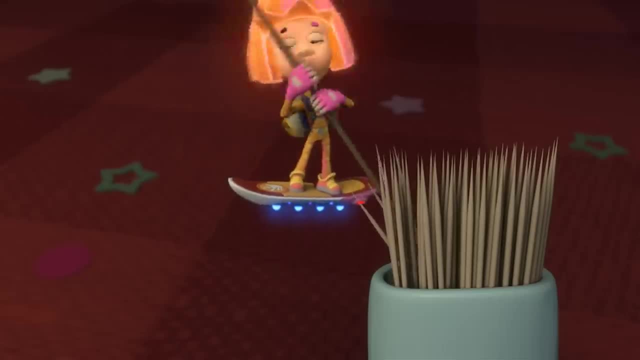 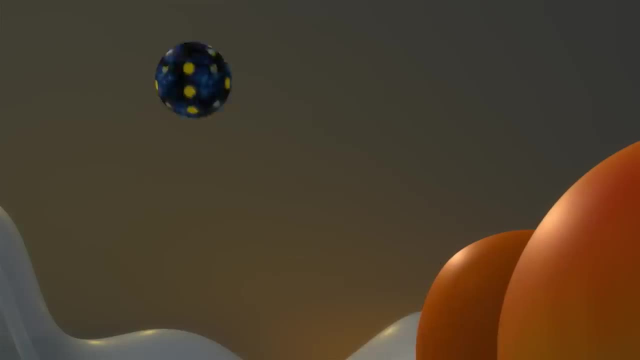 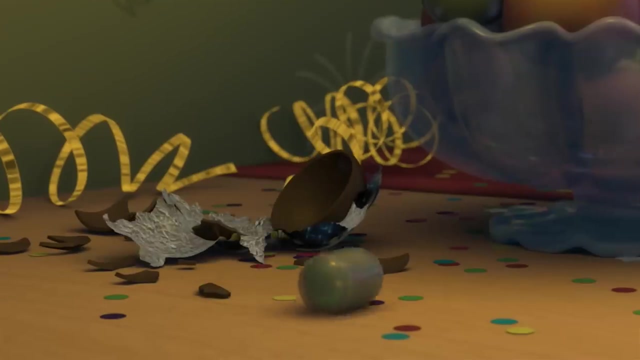 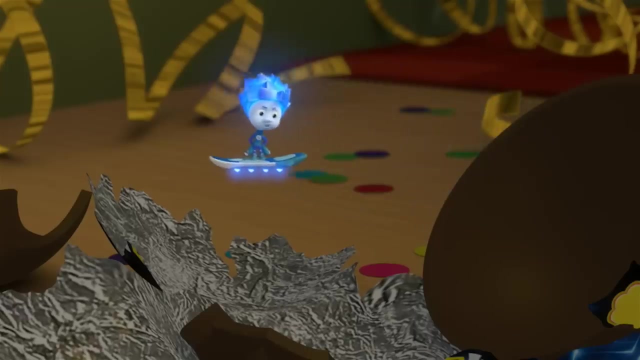 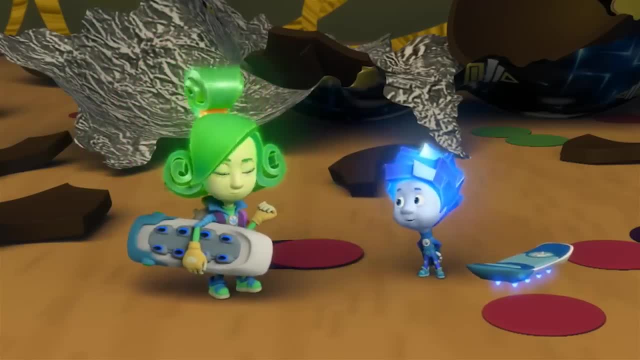 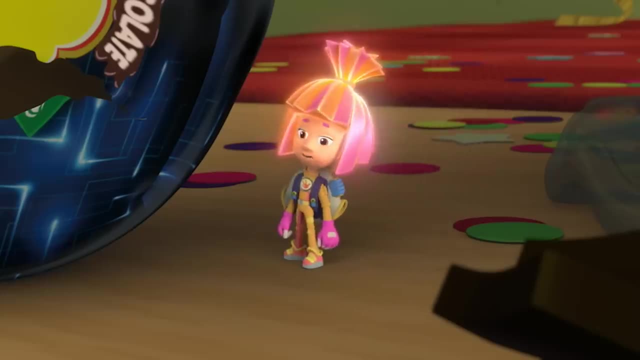 when he finds out you touched the chocolate ball And you Like you didn't touch it, I didn't. Oh then what's that? Nolik Chocolate? Absolutely, It's 100% natural milk chocolate. It says so right here. 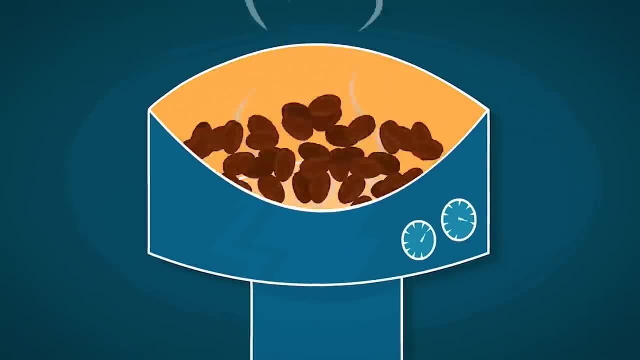 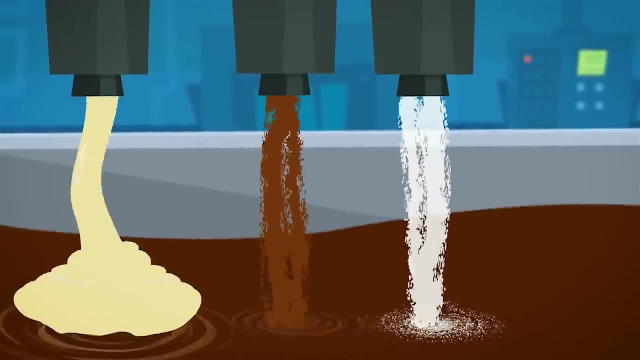 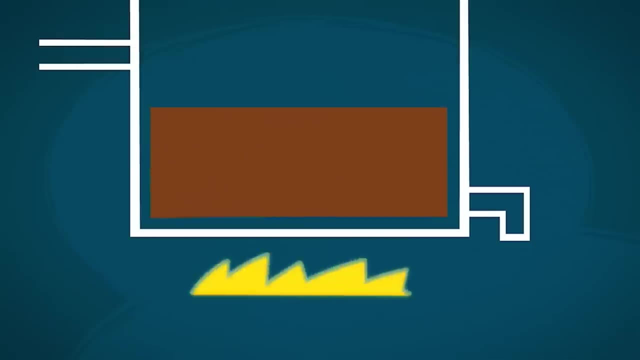 Wh-what? Wait, They are roasted, crushed and ground. After that, the ground beans are pressed to extract the oil from them. If you mix butter, cocoa and sugar, you'll get dark chocolate, And if you add some milk to it, then you'll get milk chocolate. 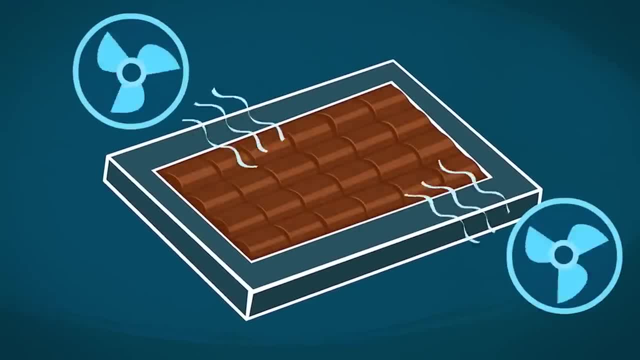 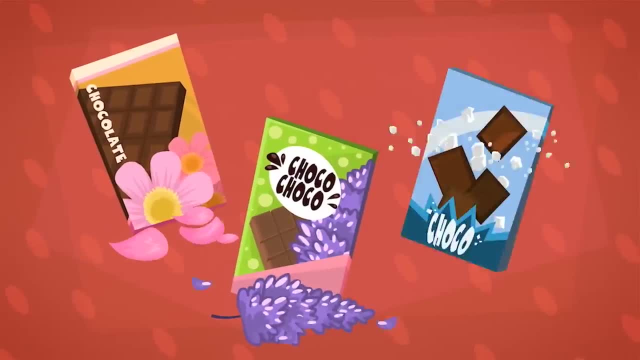 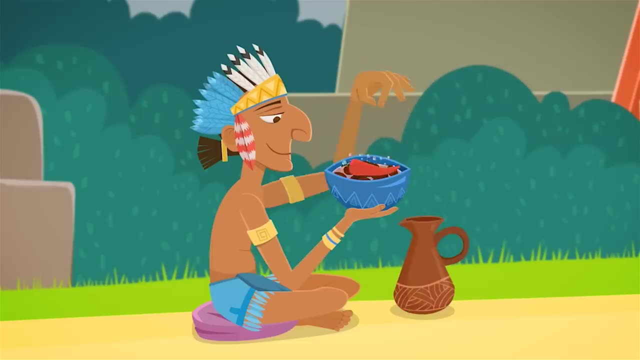 Then you just warm it up, pour it into molds and cool it down. You can add raisins or nuts into chocolate. Sometimes chocolate is even made with flavors like flowers or salt. Chocolate wasn't originally for eating. It was used in a drink made by mixing roasted beans with water and then adding hot peppers. 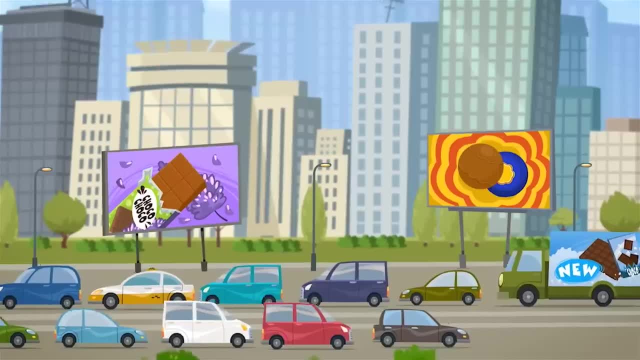 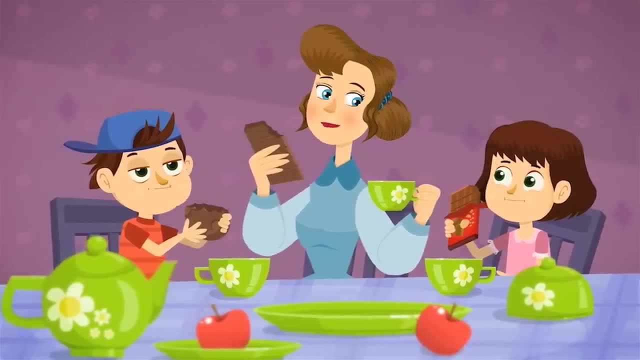 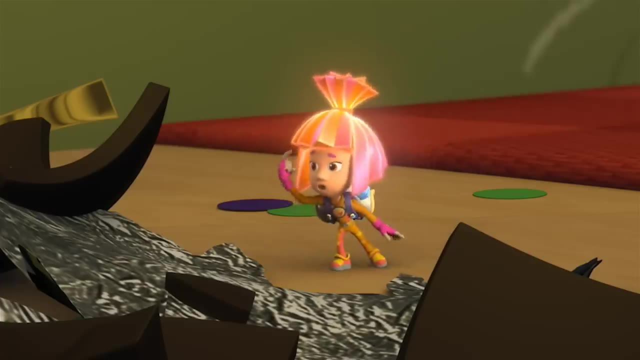 Not every adult could drink it, let alone a child. Today, chocolate is a favorite treat the world over, for children and adults alike. How can we put it back together? How about Scotch Tape? Come on, We'll start by warming up the chocolate so it softens up, and then use that to make a new ball. 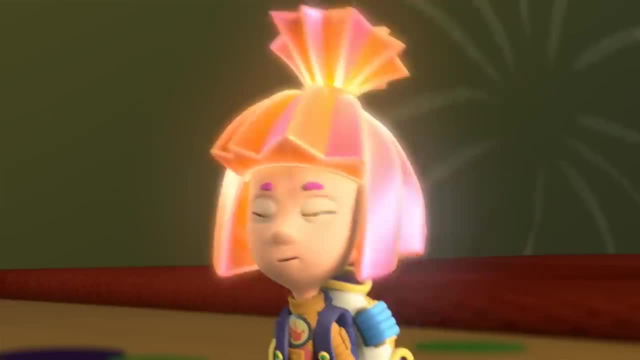 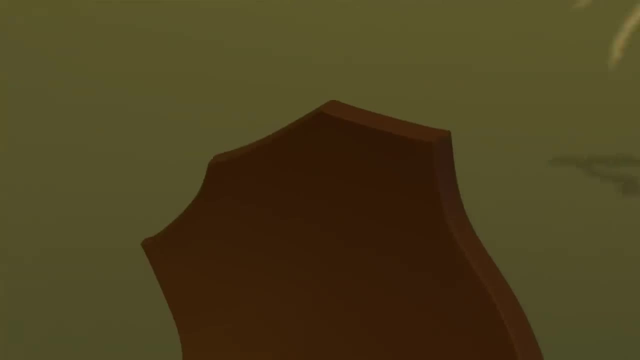 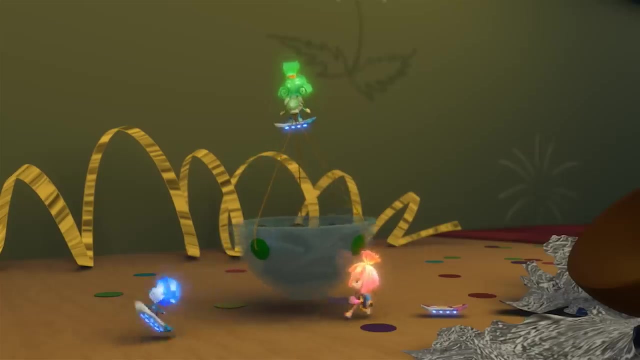 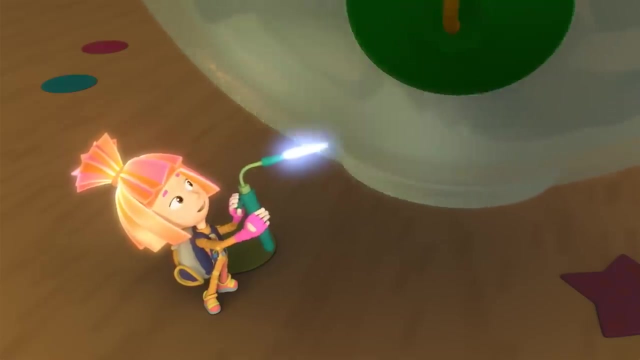 And then We're meant to make it hard again. Yeah, we just cool it off. My chocolate confection has gotten imperfection. Half of it's gone into thin air, But this is expected When chocolate goes unprotected. first, you have got it. 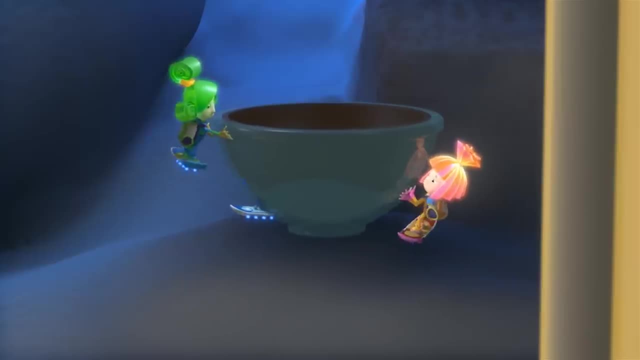 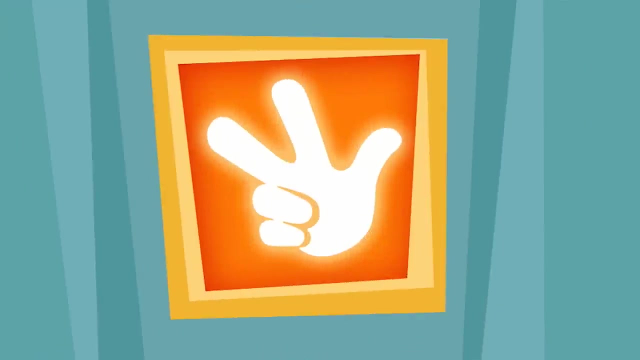 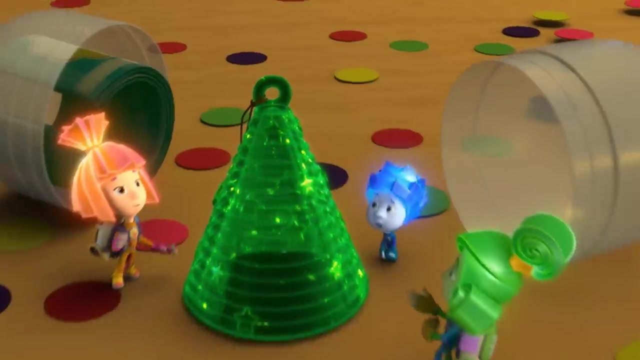 Because that chip's not there, Not there, Not there. Tideesh Done, Let's put in the toy. But we haven't even looked at it yet. Oh, it's so pretty. Tom Thomas is gonna love it. Oh wait. 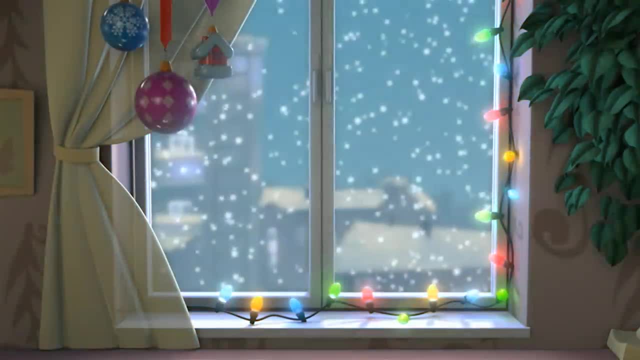 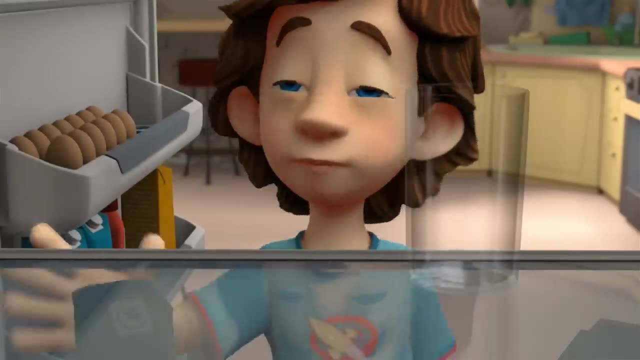 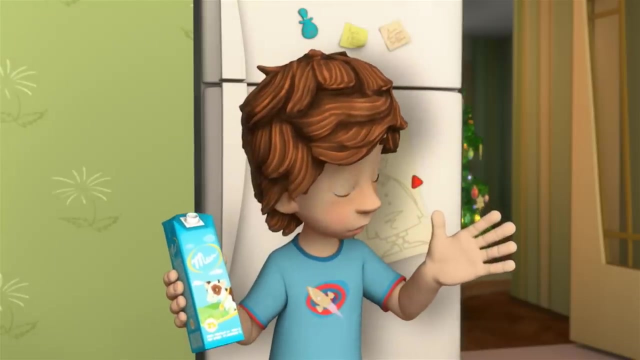 Oh, what do you think of this idea? I've got a new confection Of chocolate: perfection, Safe in his wrapper, shining bright. Oh what perfection. My brand new chocolate confecting. I'll try my best not to take a bite, Hi there. 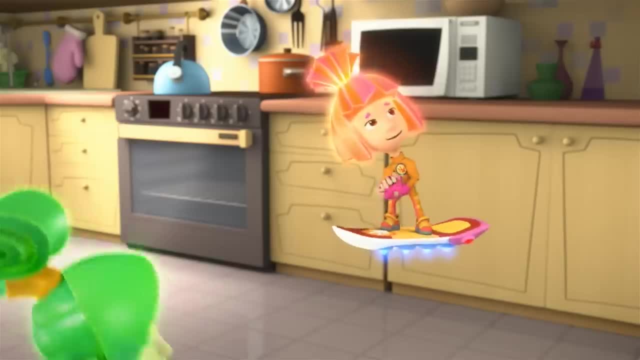 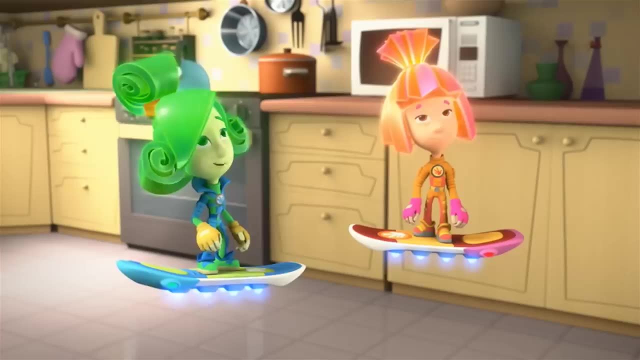 Oh, what's that? A chocolate ball. You're lucky Could there be a toy inside, Mm-hmm. But I can't take off the wrapper without Nolik. You really can't do it without him. I can't. I told Nolik I wouldn't. 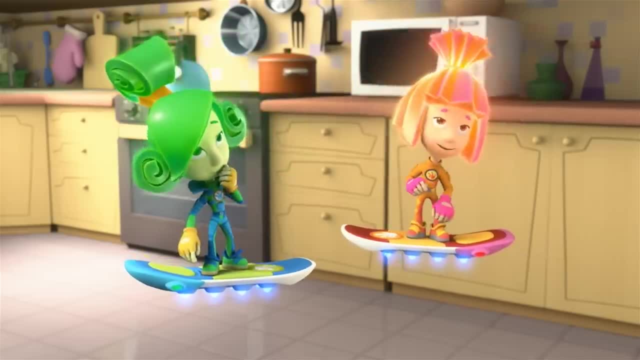 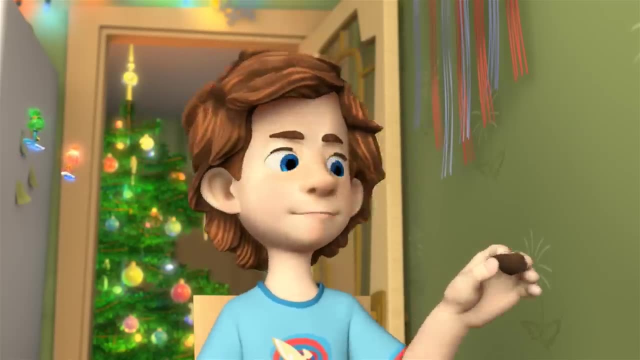 Mm, your chocolate is going to be delicious. Go on, you can eat a little? Hmm, if you say so, I'll eat the chocolate, but we won't open the toy without Nolik Mm. good chocolate. 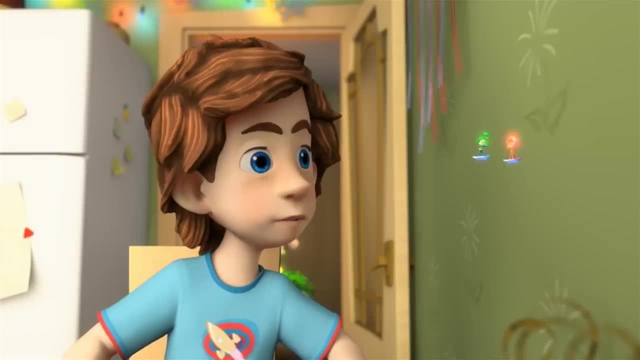 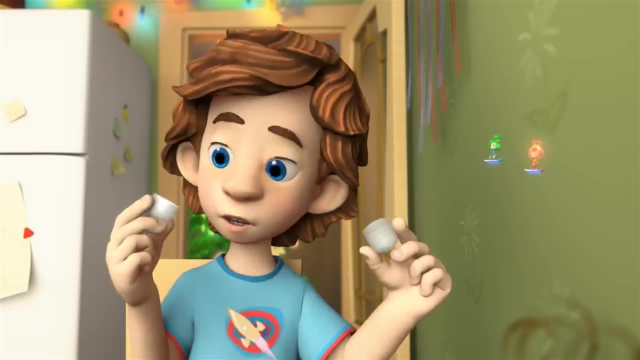 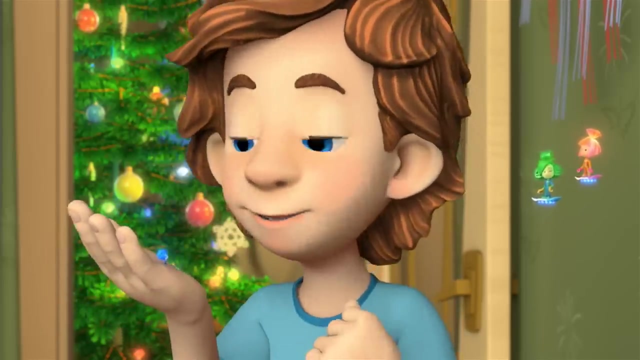 Come on, don't you want to know what the toy is? We won't tell. All right, just a peek and we'll close it right up. OK, Here's the treasure. Nolik, what is this for Teej? 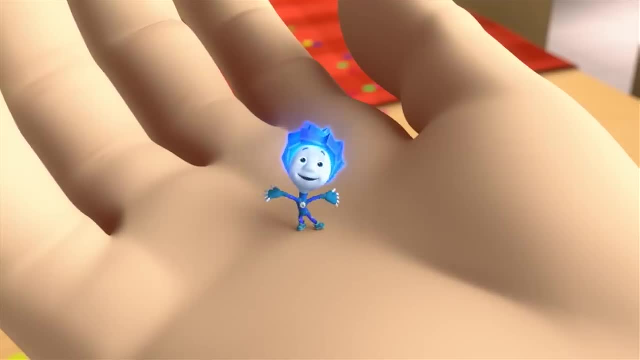 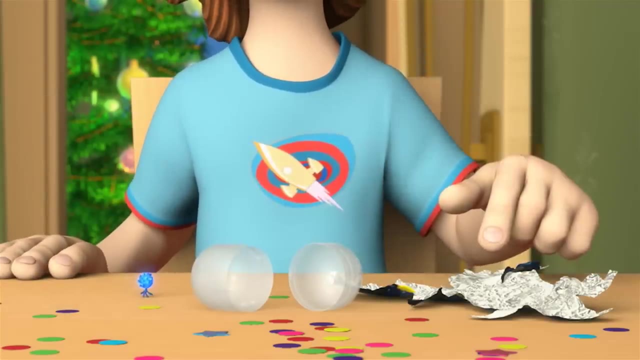 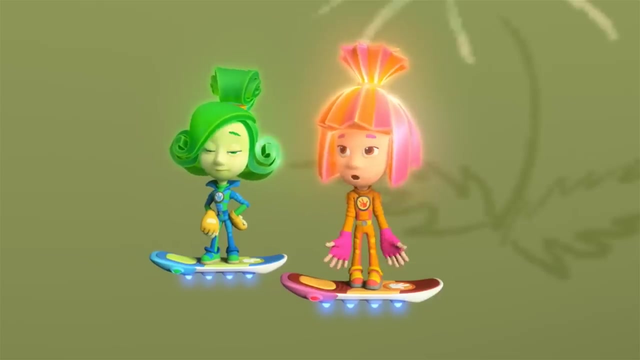 Nolik, Really, How did you get in there? Surprise, Hmm, you were in the container. the container was in the chocolate ball and the ball, Yep, That's just impossible. Ah, he went and got you two to help. 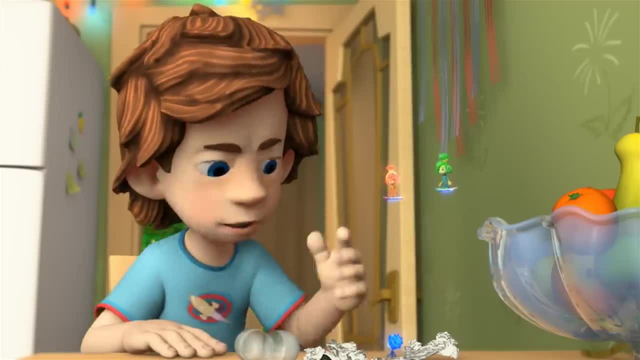 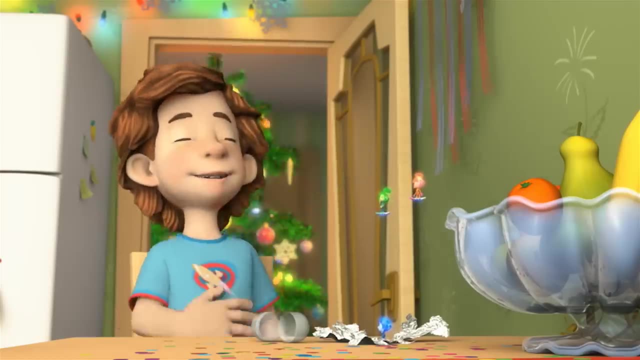 We helped a little. Hang on, Nolik. I promise not to touch the chocolate till morning And you promise not to open the toy without me right All on the bench time. My friend loves chocolate. Make the next pitch. 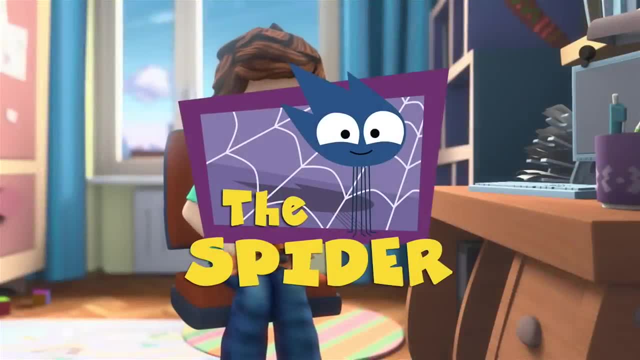 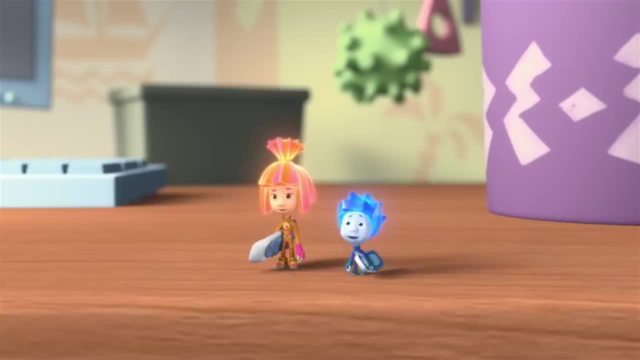 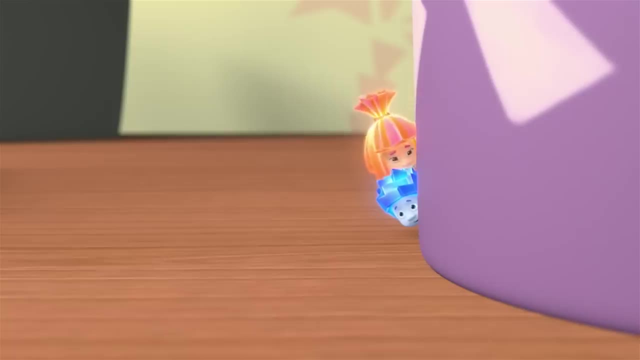 I'll try with my best friend, The spider: Chewsocka, Chewsocka. Tom Thomas, what are you doing? I'm petting Chewsocka- How come? Huh, Because it makes her feel good. Just don't rub her fur off. 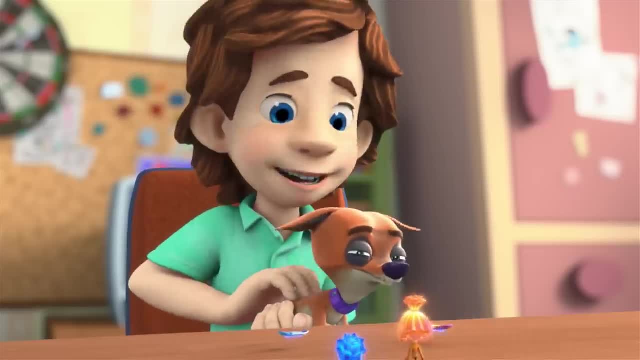 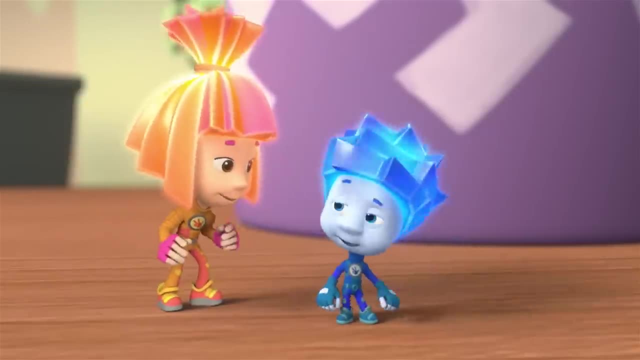 You're just jealous, guys, because you don't have any pets of your own. What do you mean? We've got a pet, Yoo-hoo Buggy Buggy. She was in the vent the last time I saw her. 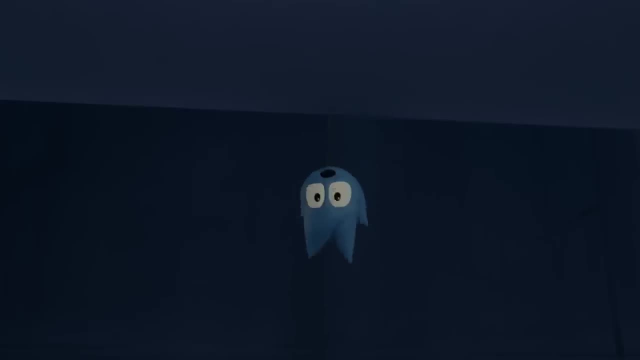 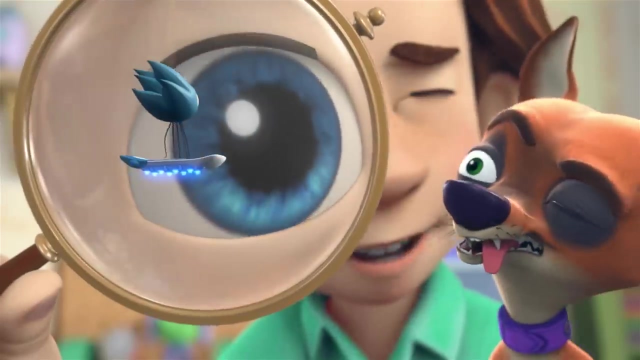 Buggy, Come on out, We need to talk Here. this is our friend Buggy. Wait, This insect is really your pet. Ha, What a joke. Buggy's a spider. She's not an insect at all. 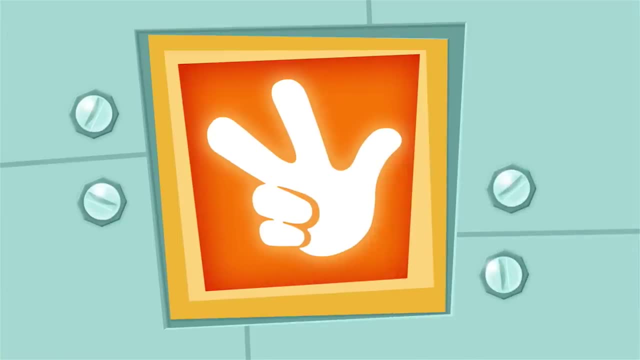 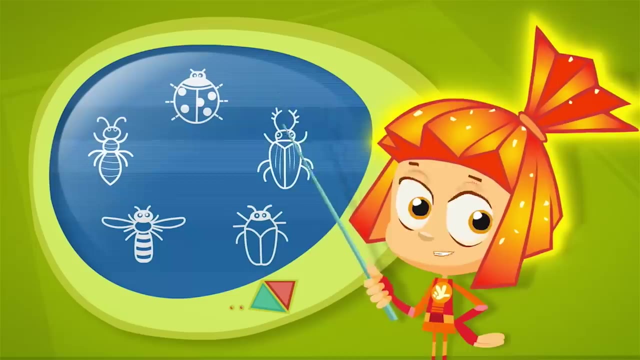 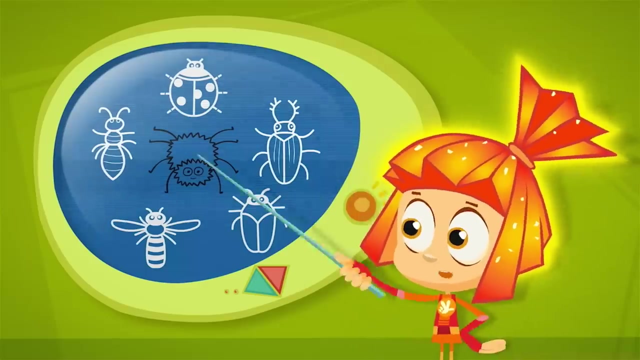 But isn't a spider, a kind of insect? Insect is the term used for mosquitoes, flies, beetles, dragonflies, butterflies, ants and many others. Spiders certainly look a lot like insects. They have very similar legs, But spiders aren't insects. 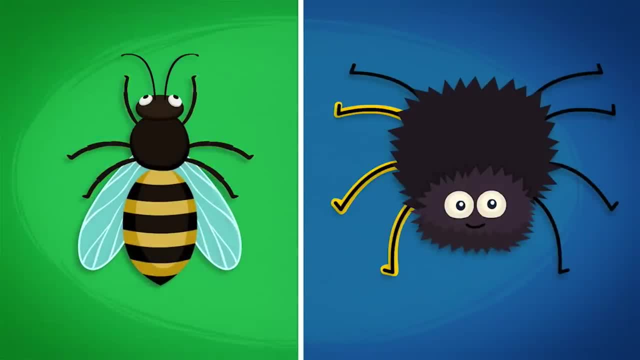 They're arachnids. Insects have six legs, while spiders have eight of them. Many insects can fly, but spiders can't. But spiders can move spider webs. They may look beautiful, but really they are traps for hunting insects. 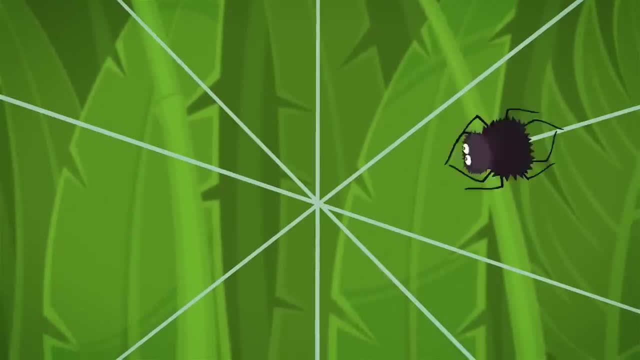 How come your Buggy has five legs instead of eight of them? I don't know. She lost them somehow. Anyhow, she can do lots of tricks. Hello Buggy, How do you do? We know how to do that trick. 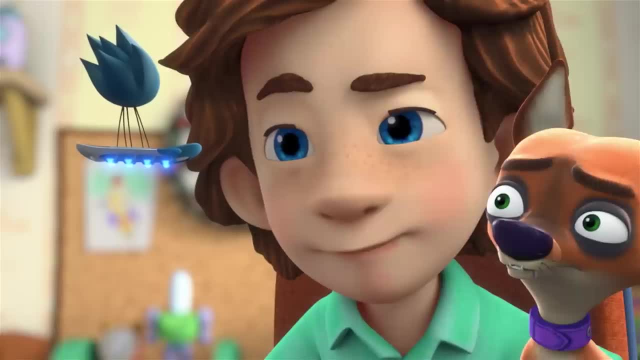 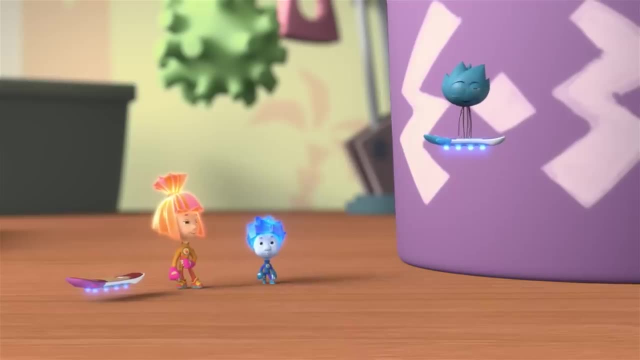 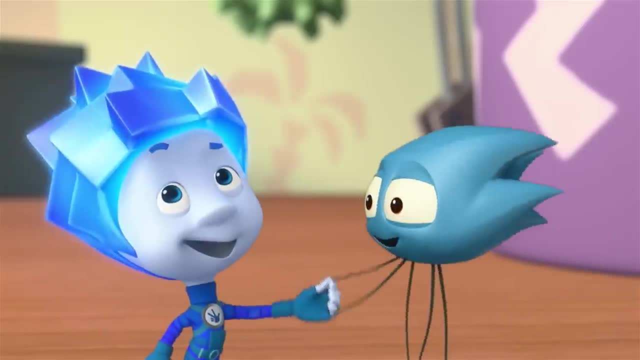 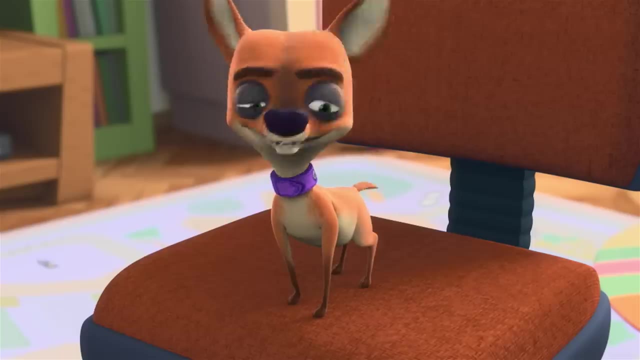 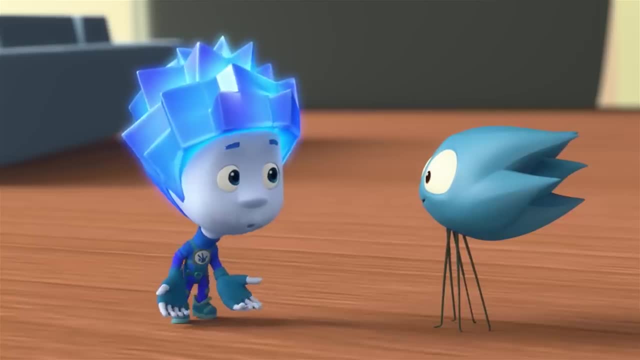 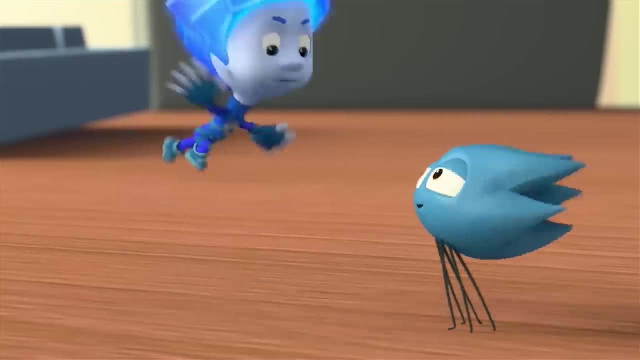 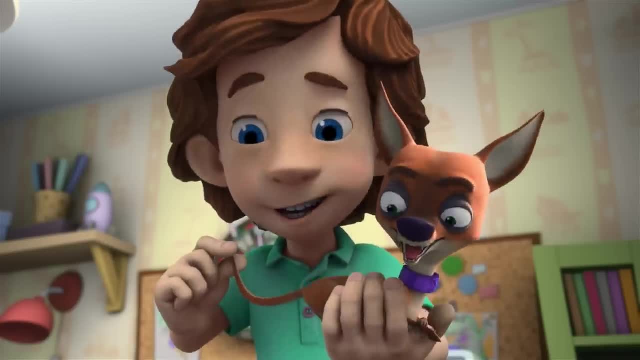 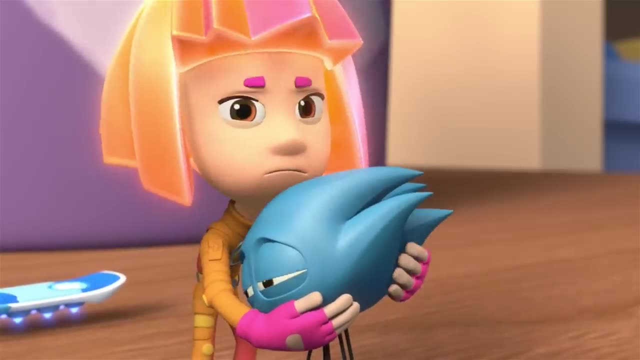 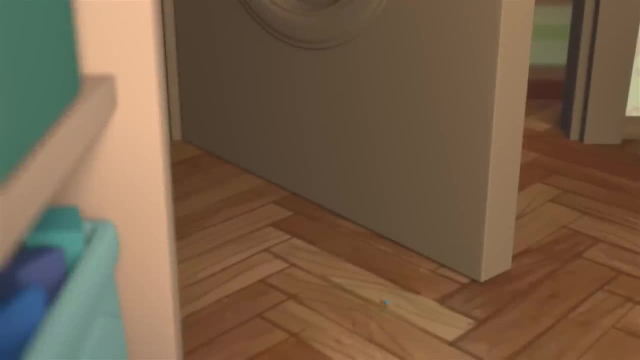 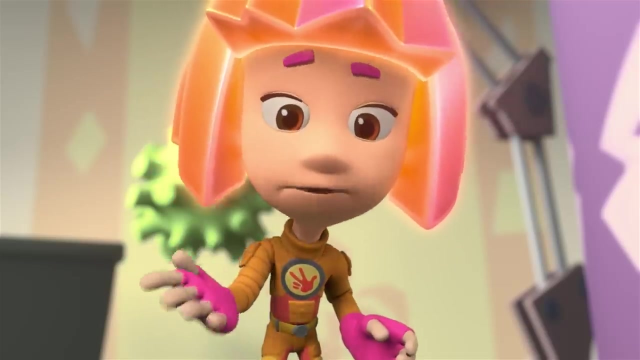 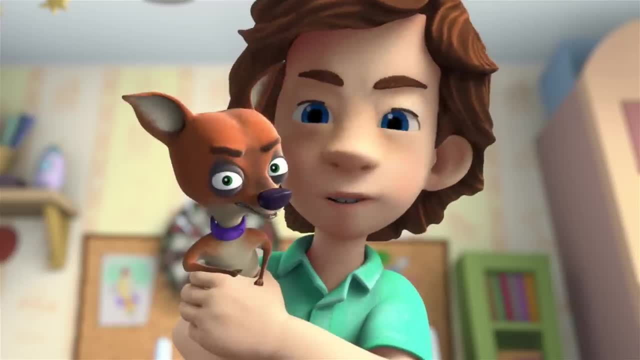 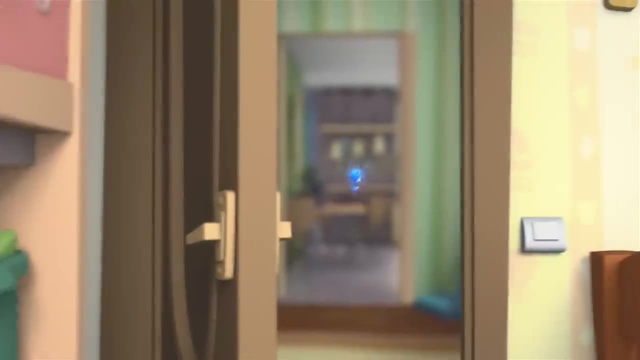 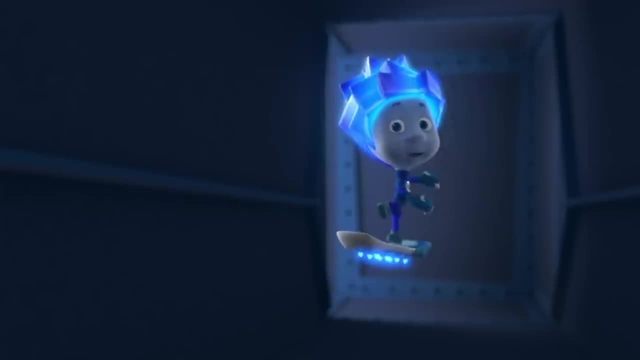 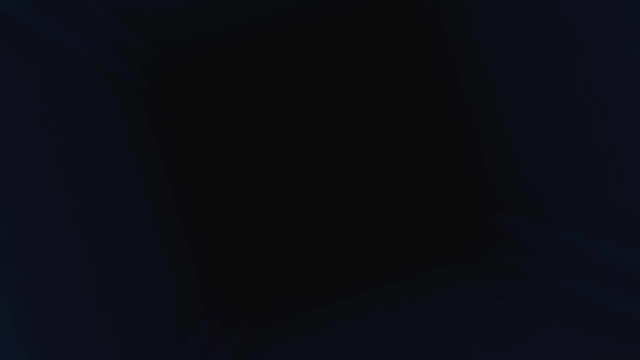 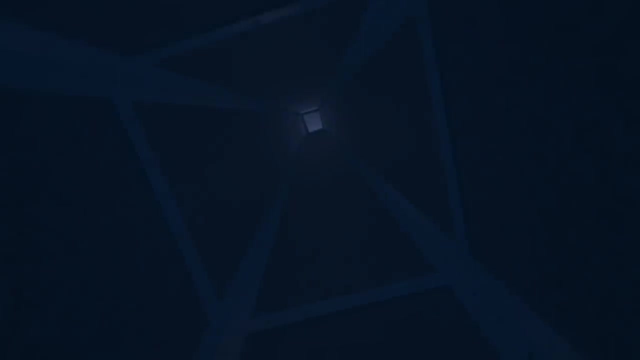 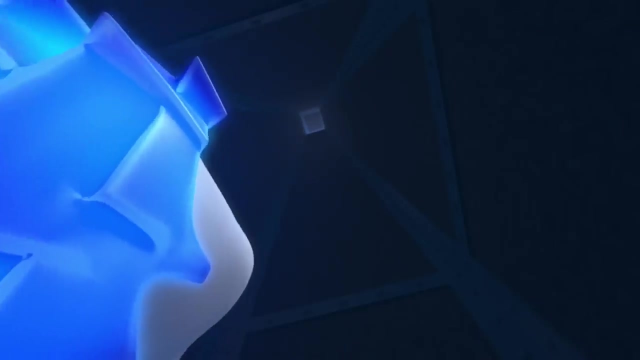 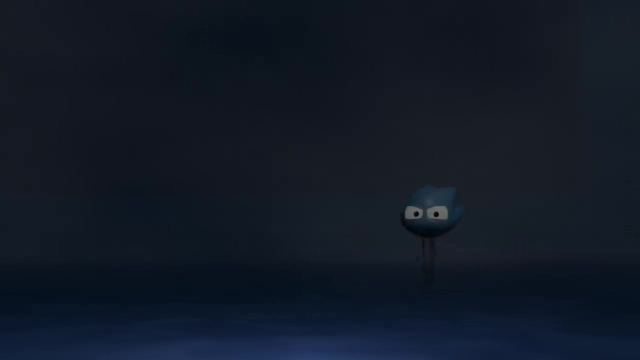 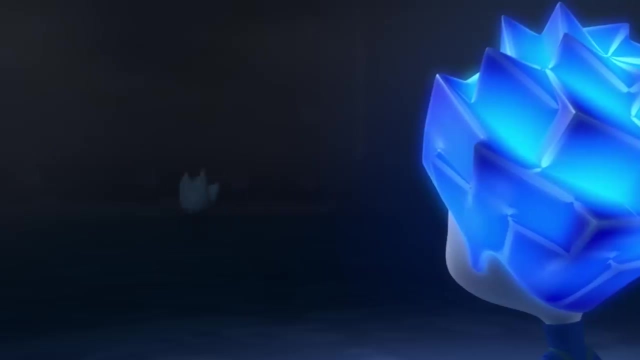 Oh buggy, Oh buggy, Oh buggy- Is that you? I think I broke my leg. Could you help me out? buggy, You don't want to help me. You're right. I don't deserve it, Because I've been a really bad friend. 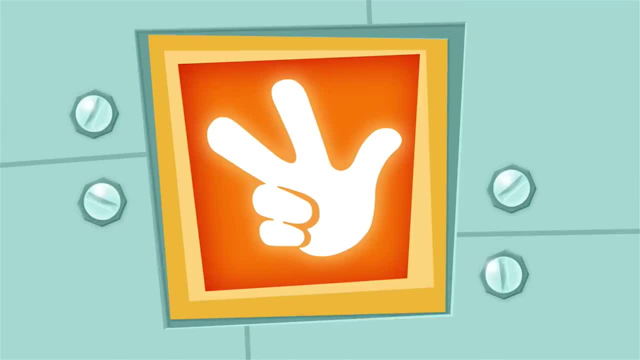 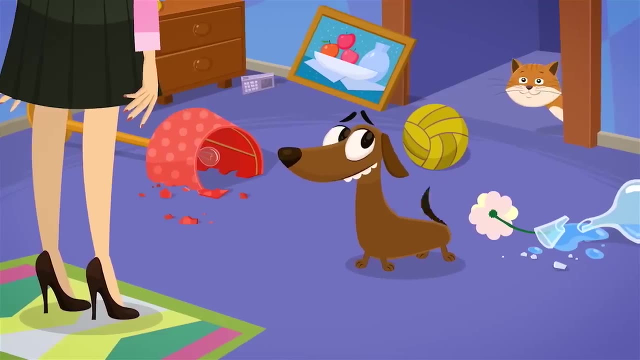 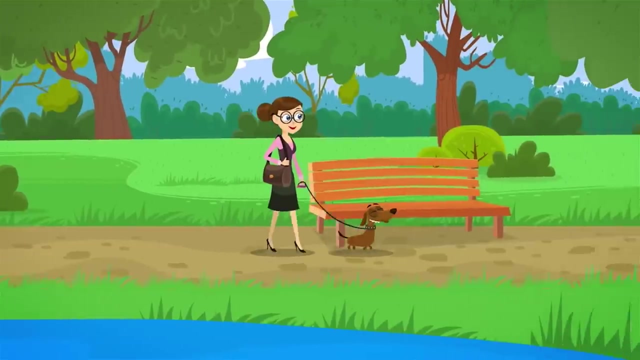 People like having pets to live with them in their homes: Dogs, cats, hamsters, parrots, fish, turtles. Some folks even get crocodiles, And the bigger the animal, the more people they get They love it, the more work it takes to take proper care of it. 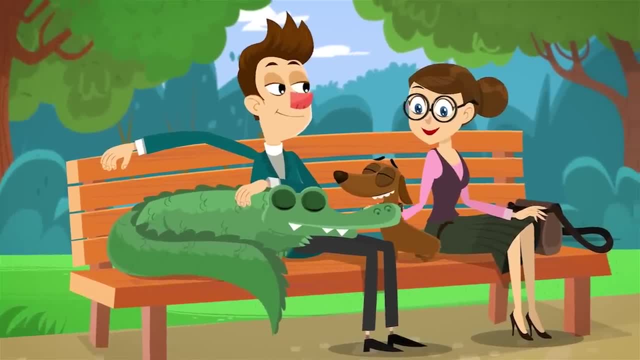 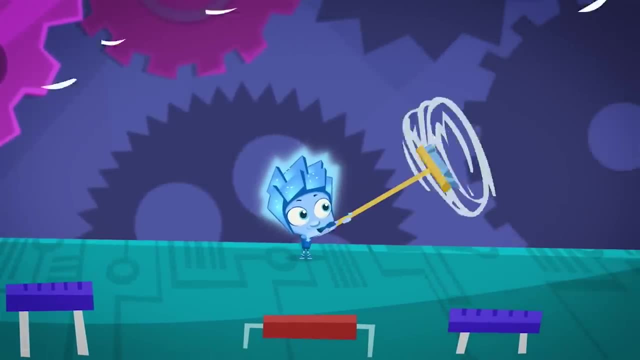 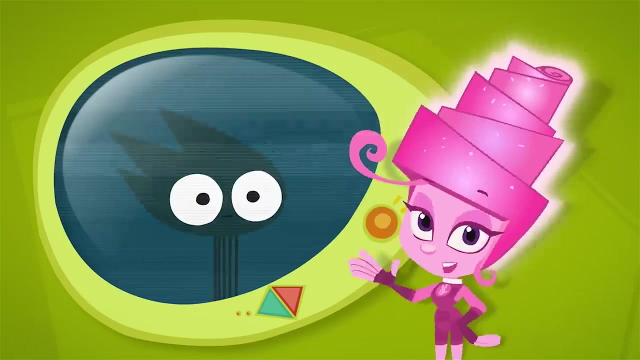 But every pet needs love and care, no matter what size it is. Fixies like to have pets too. All sorts of little bugs, spiders and flies. Fixies treat them as friends and take care of them. Of course, a little spider isn't as smart as a dog, but they also can be trained. 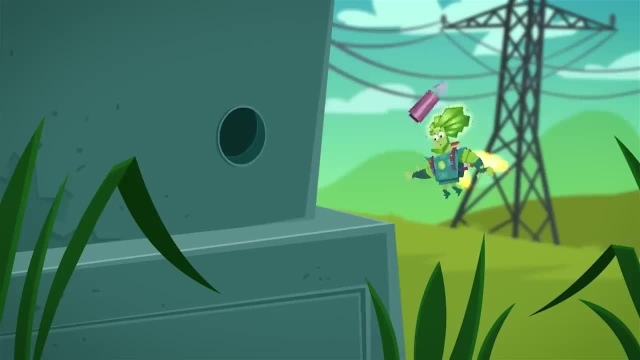 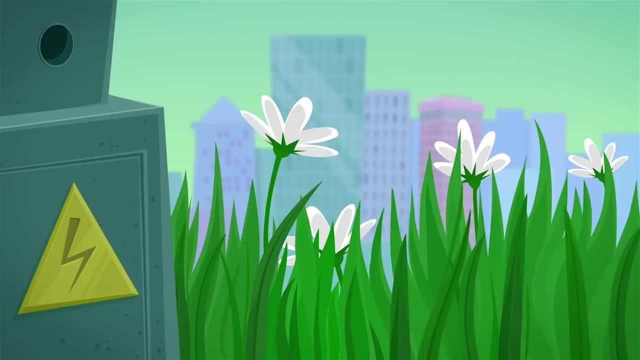 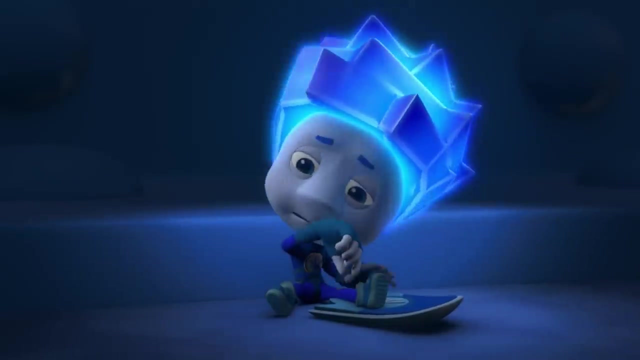 There are some Fixies who have managed to domesticate such big insects as bees, beetles and dragonflies. Fixies fly on their backs and use them to carry heavy loads. That's it. I'm stuck all alone in here Forever. 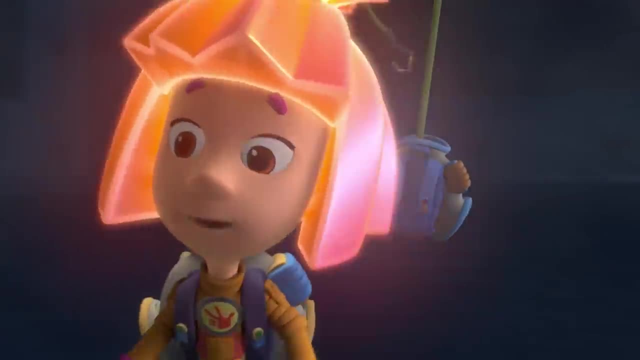 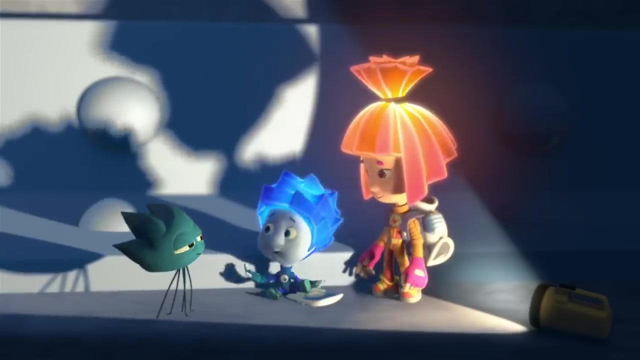 Simka: Oh, how did you find me? Buggy led me down here. Buggy, you didn't ditch me. I'm sorry. I'm sorry. I promise I'll never, ever yell at you again. Ow, my leg. 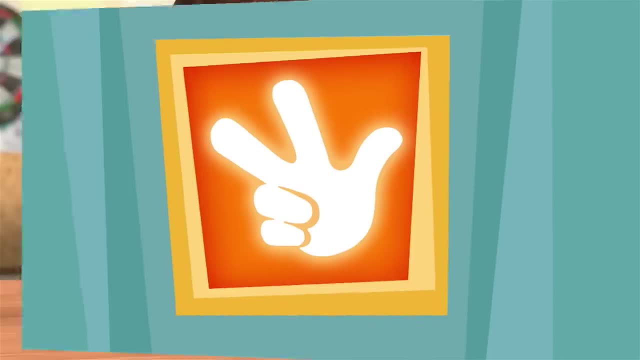 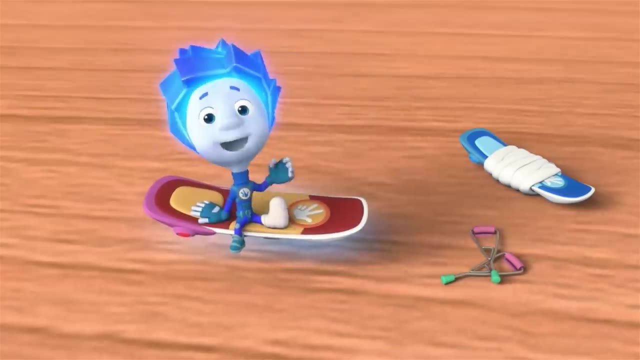 Hang in there, Nolik, We'll get you out. It was so scary You could have died down there. Yeah, I almost died, But you know what Buggy saved me? Yeah, that's cooler than learning how to shake hands. 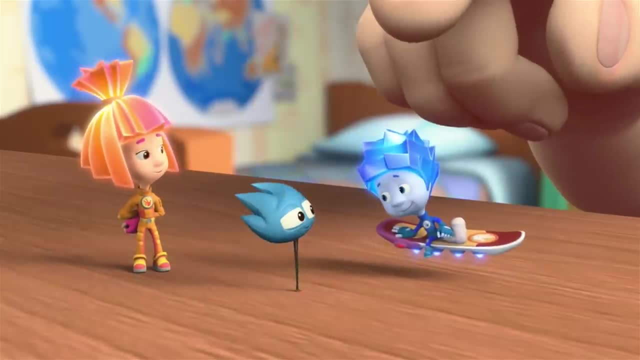 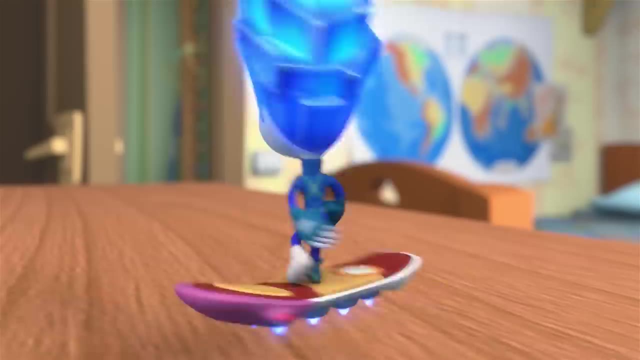 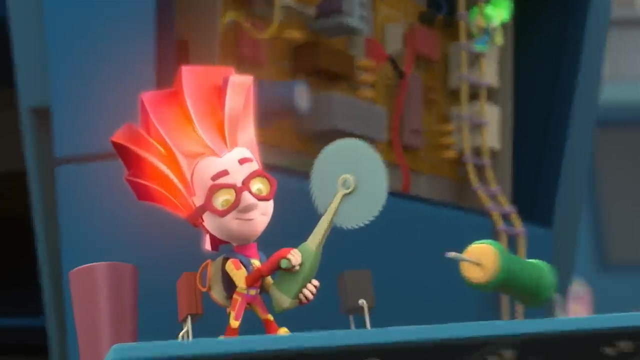 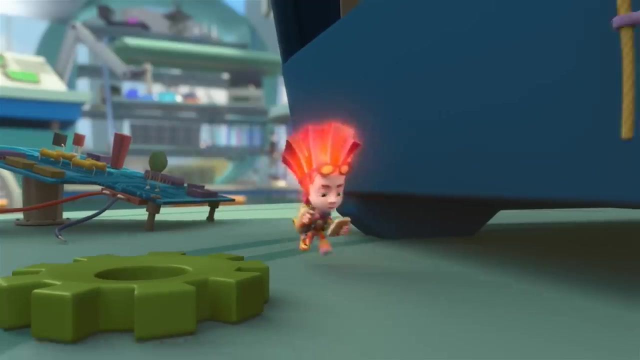 Buggy sure is a true friend indeed. Does your leg really hurt a lot? Ah Ooh, Nah, it doesn't really hurt, I'm fine, I was just joking Money. Hello, Uh-huh Fire, can you help me please? 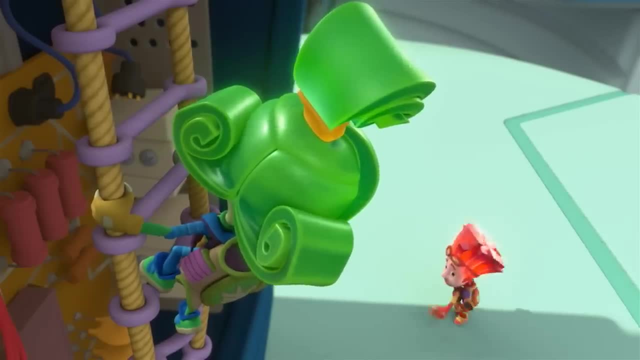 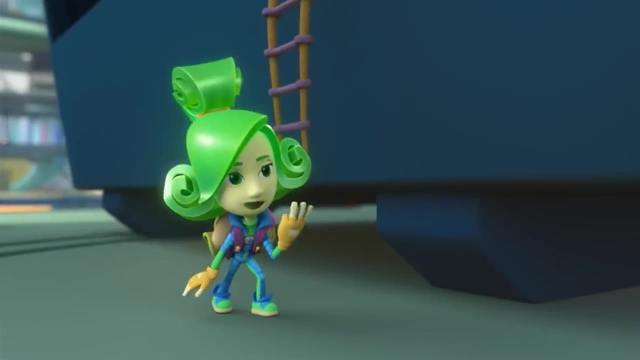 Sorry, Verda, I need to go to uh, the warehouse Right away. But I helped you yesterday, didn't I? Well, I helped you the day before that, Yeah, well, what about last week? I helped you three times, remember. 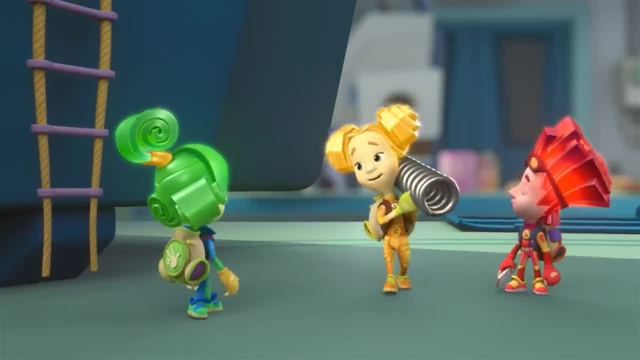 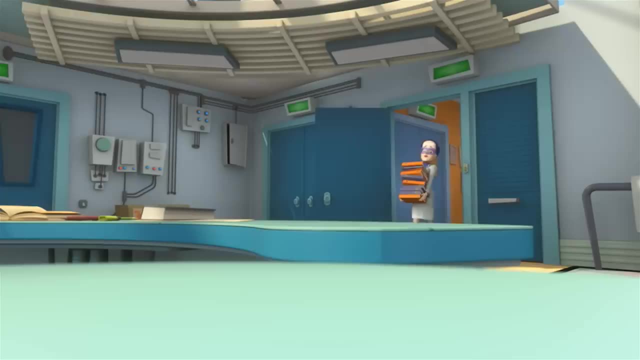 Well, I, You helped one another when it was time to. I don't see why you have to count, Course not. Tula, You ask for the most help from all of us. I do not, Verda. Look how Elisa helps Professor Eugenius, And she doesn't argue with him. 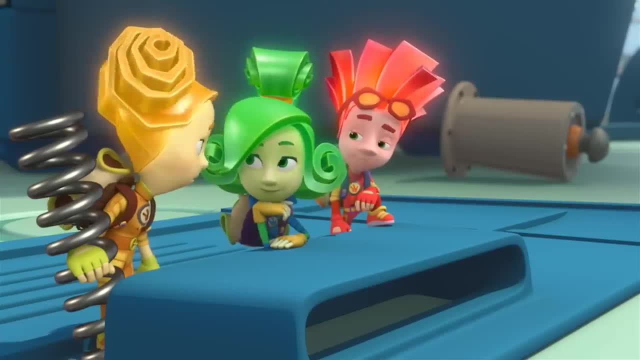 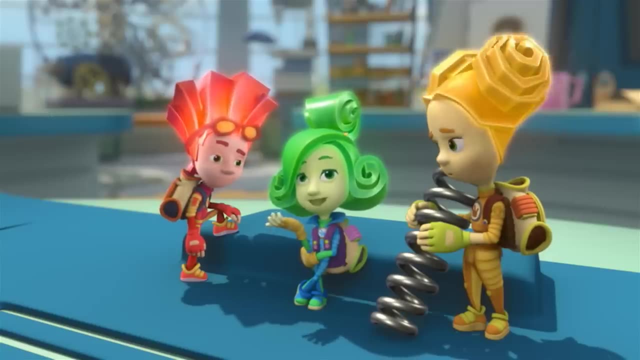 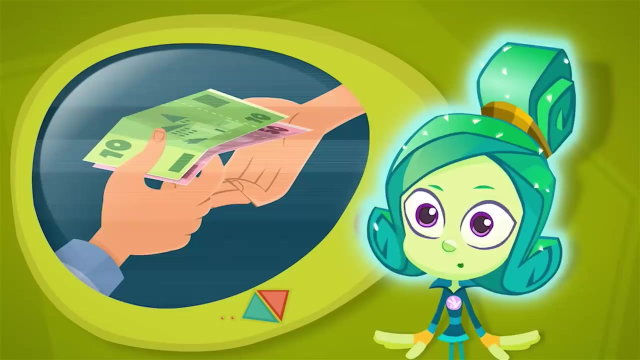 Of course not. She's in love with the professor. Actually, it's her job, And for helping the professor she gets money. Hmm, money, That's a smart idea. Money constantly moves from one hand to another. A person does his job at work and in exchange, he gets money for it. 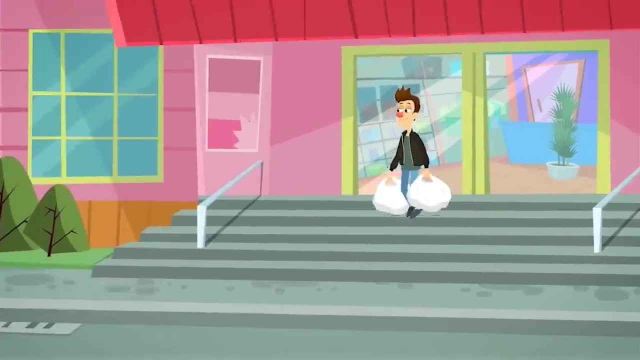 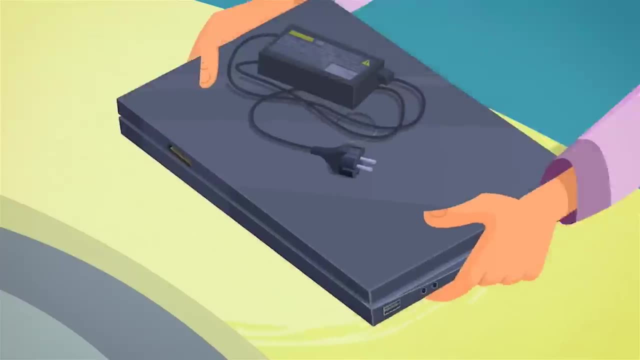 He can use the money to buy things he wants, like clothing or food, Or he can pay somebody else for their work, like getting a ride from a taxi driver, a haircut from a hairdresser or a computer repaired by a technician. 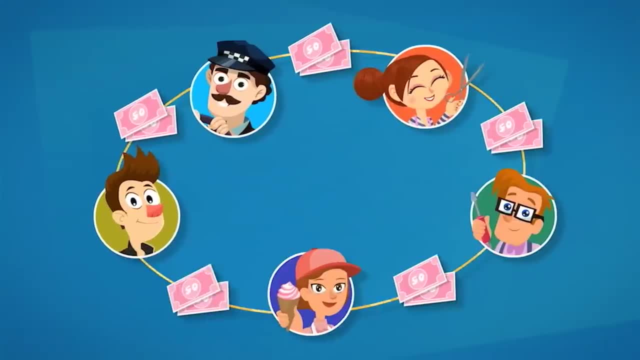 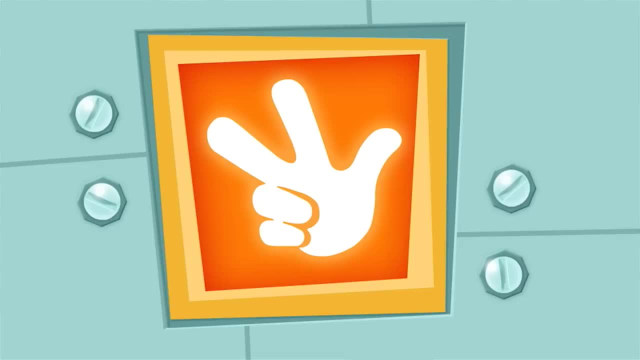 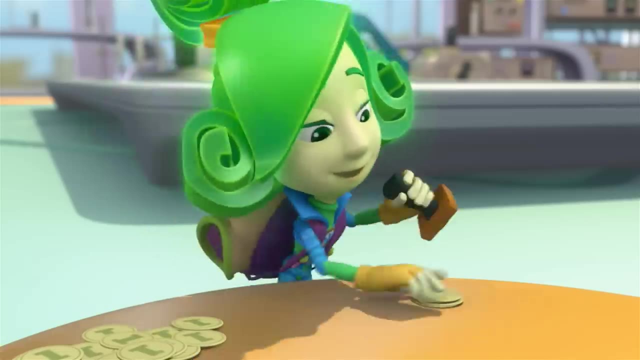 All people take part in this circular situation of money, But, unlike people, Fixies don't use any money. We do just fine without it. From now on, we'll do it like people do it. If you work for somebody, they give you money for it. 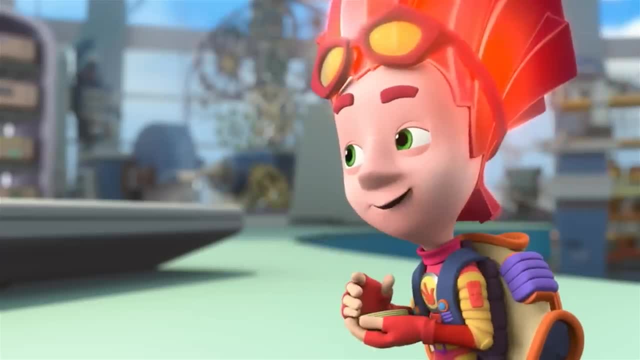 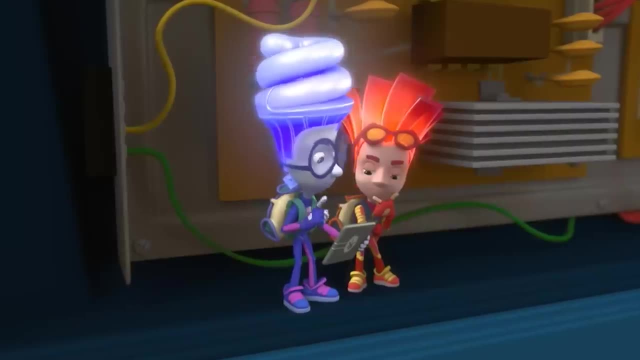 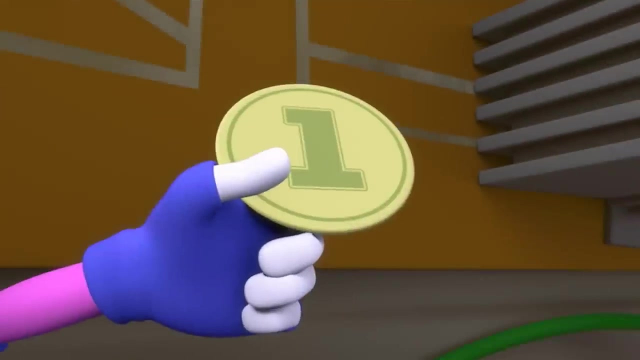 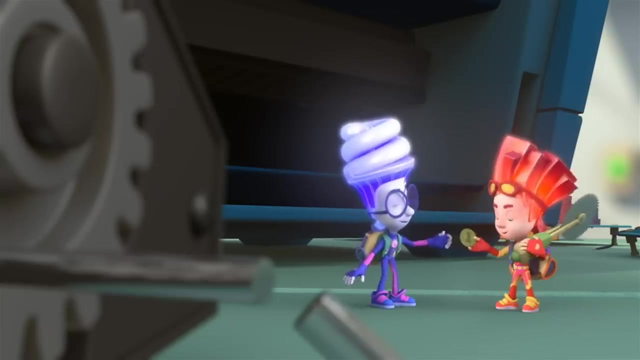 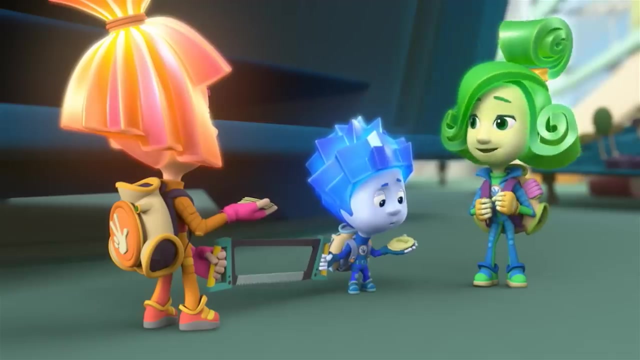 And if you need some help then you pay, And that'll stop the arguing And all the false accusations. And those are for Simka and Dole. And now it's all fair. What is this Money? What are we supposed to do with it? 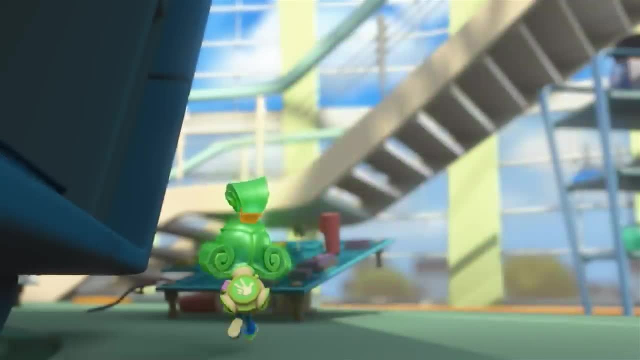 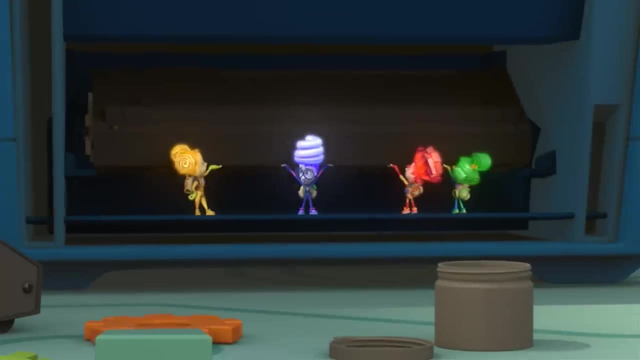 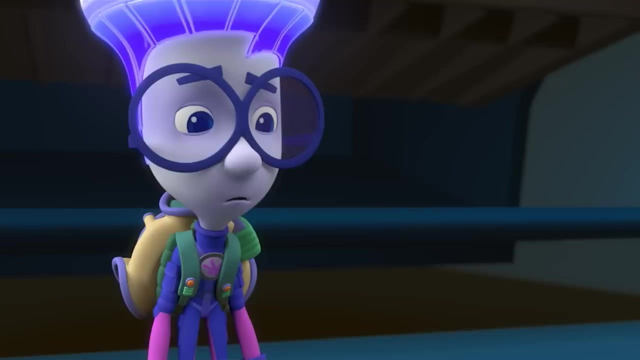 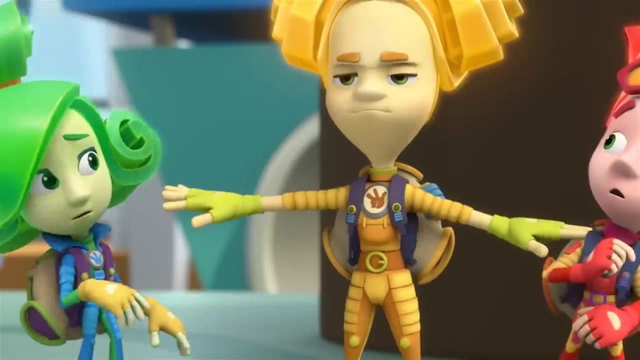 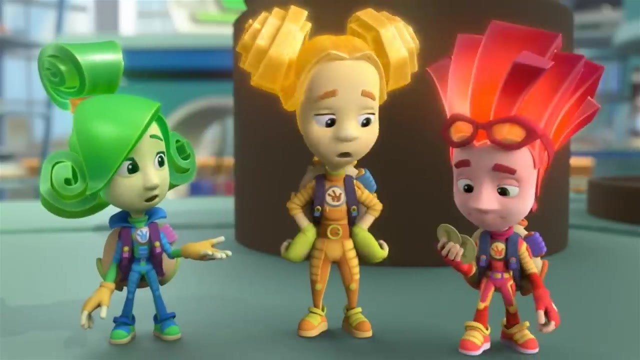 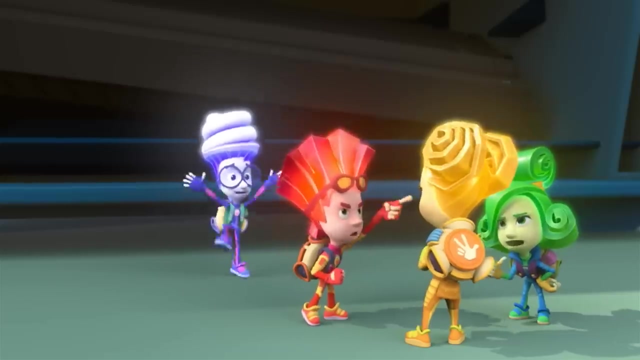 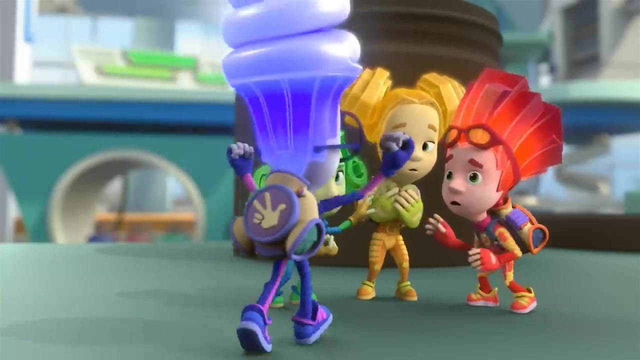 You don't know, You pay for someone to help you. I don't like this new idea At all, At all, At all. We gotta give them some money, That's right. Maybe we should give them our money so they'll stop arguing. 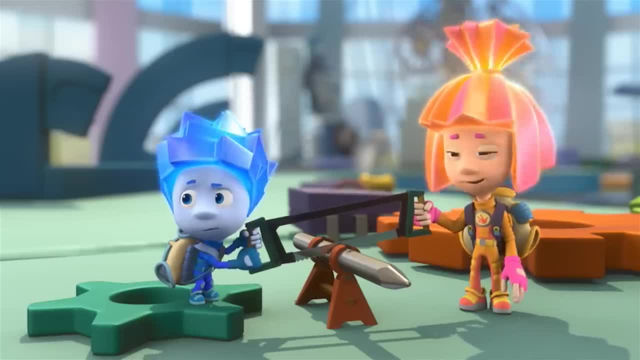 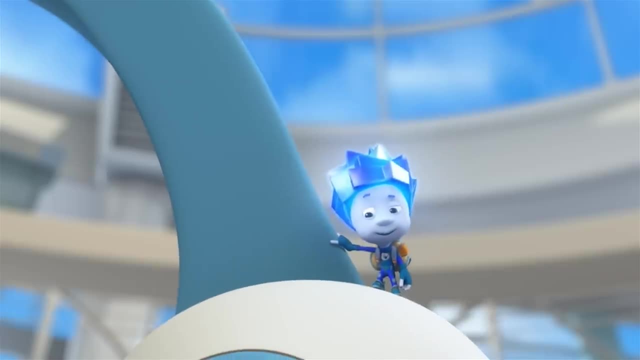 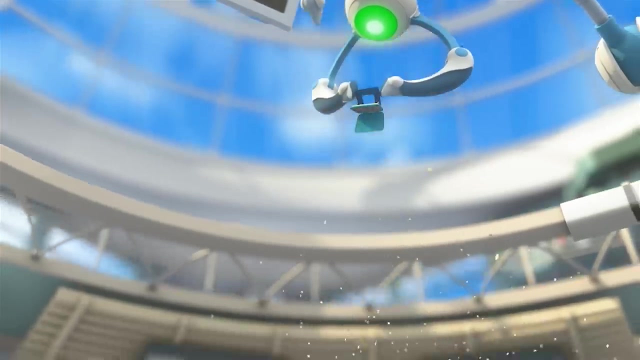 So they'll stop arguing. I've got a cooler idea. Hey, Who needs money around here? Because we've got a bank or something? Because we've got it Now, there's enough for everybody. Where are you? We're in here. 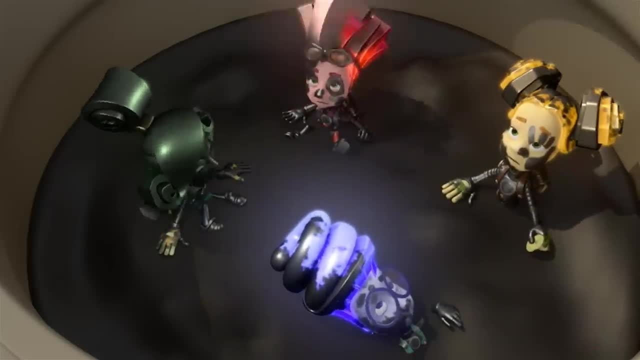 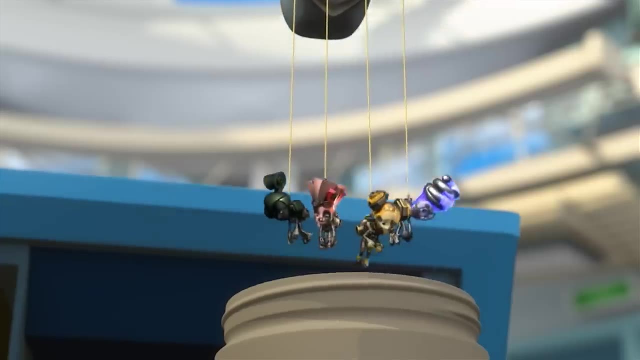 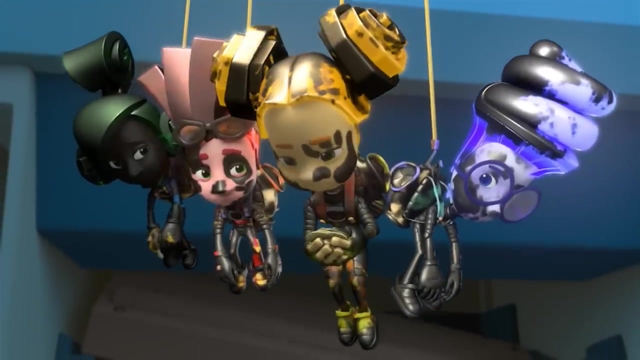 This is all your fault, Fire, And your fault. No, it's the money. That's whose fault it is? He's right. That's why we were fighting. We didn't even fix the printer. Money is nothing more than just paper. 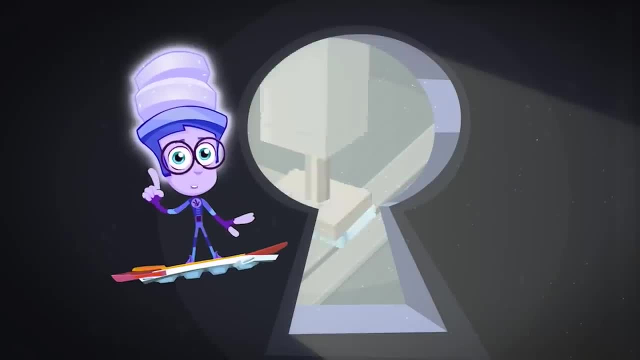 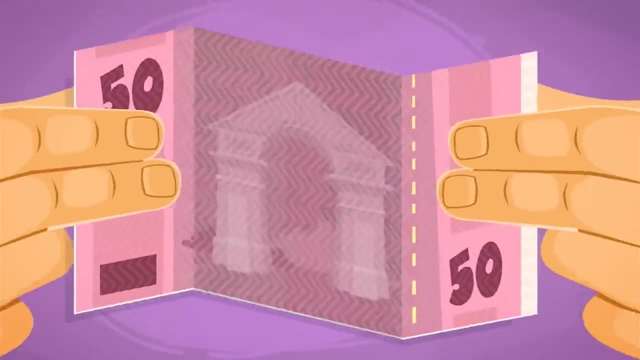 Although money is printed in strict secrecy, we still know something about the process. The paper used for money is made out of cotton and linen. It's stronger than normal paper made out of wood, which means it doesn't rip as easily, even if you fold it thousands of times. 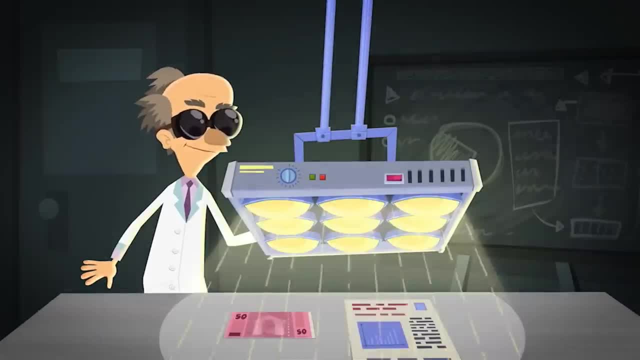 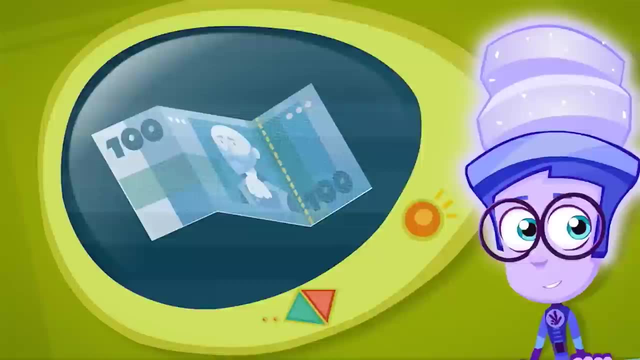 The ink used for printing money is special too. It won't rub off, It won't pop off the paper or fade in the sun. And that's not all. The ink has secret additives that can only be seen if you look at the money under a special light. 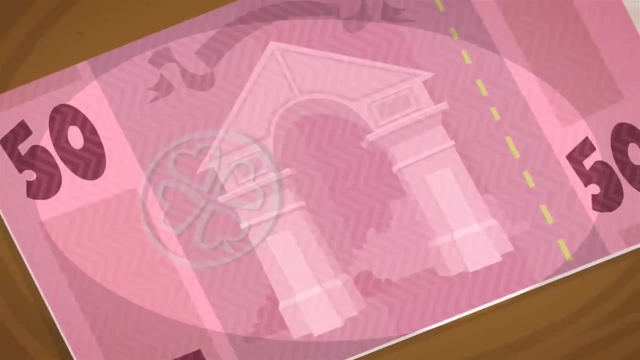 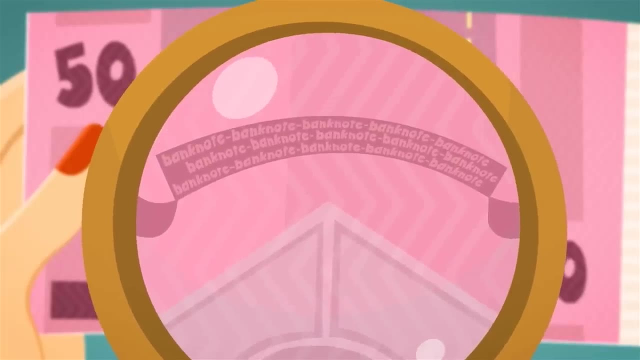 This helps protect people from fake money. It is for the same reason that watermarks, metal strings and teeny-tiny writing is also used on money. This writing's very hard to read, unless you happen to be a fixie. I hope I didn't say more than I should have. 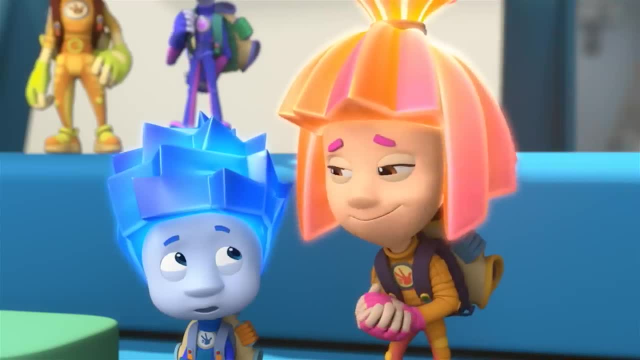 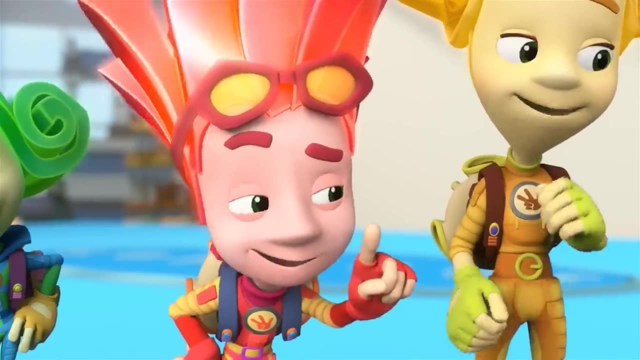 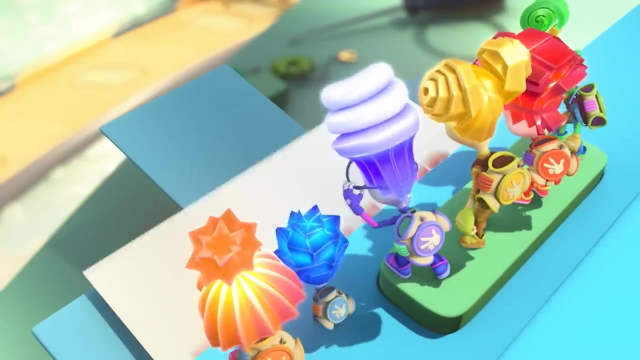 Well, all done, It's time for a test. But what are we going to print? A word with real value? Yeah, something really precious. No, it's not money, Right, it's so much better: Friendship Tideesh. 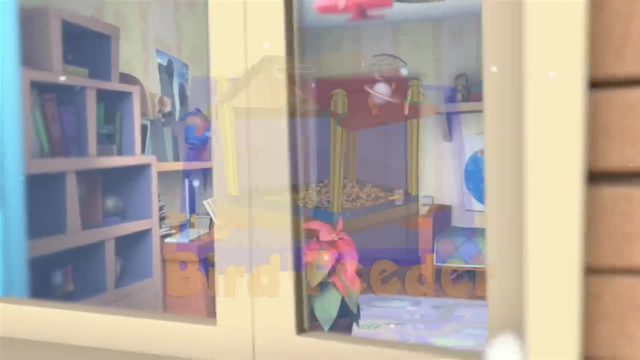 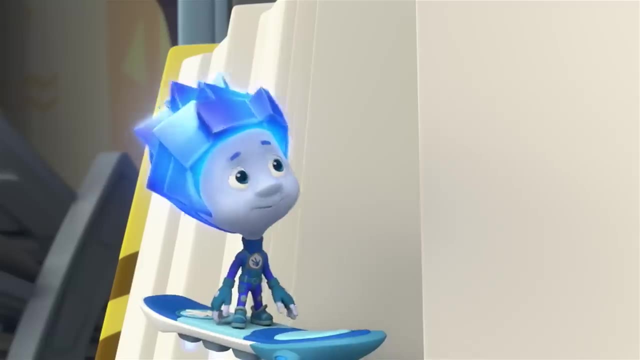 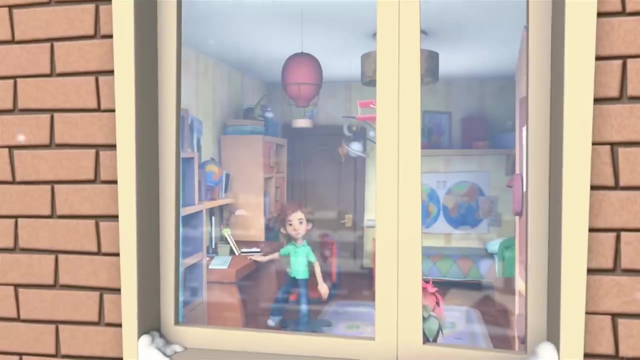 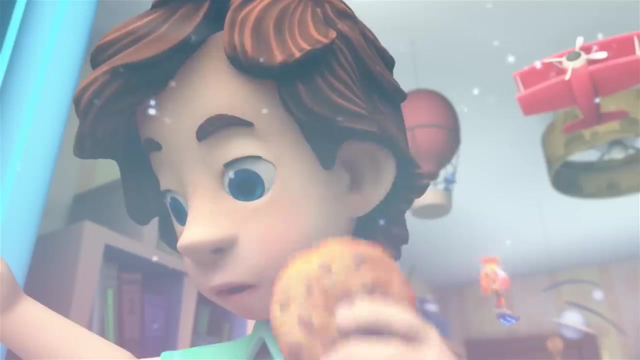 The Bird Feeder, Mm-hmm, Did you hear that? What? Oh, again Outside the window, There, Huh, a little bird. He's beautiful, Uh-huh, Only he looks sad. Just wait till he sees what I'm going to do. 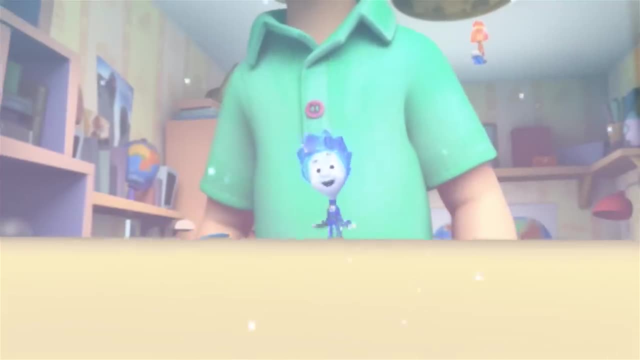 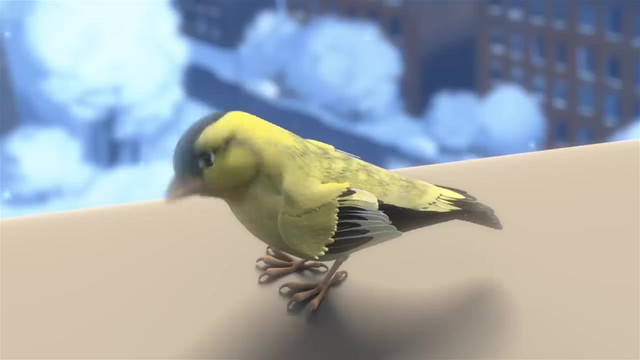 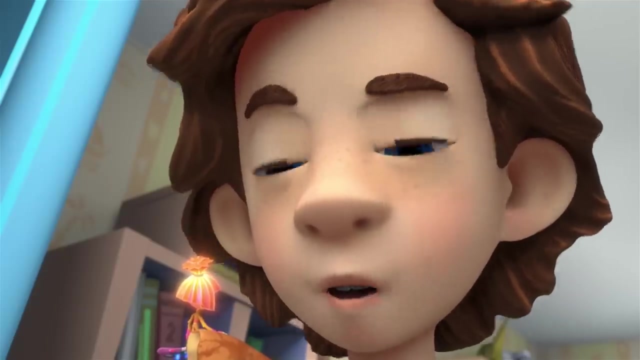 I guess he doesn't think you're funny. That's because he's cold out there. He wants to eat, that's all. Maybe we should make a feeder for the poor bird. Do you know how to make a bird feeder? No, 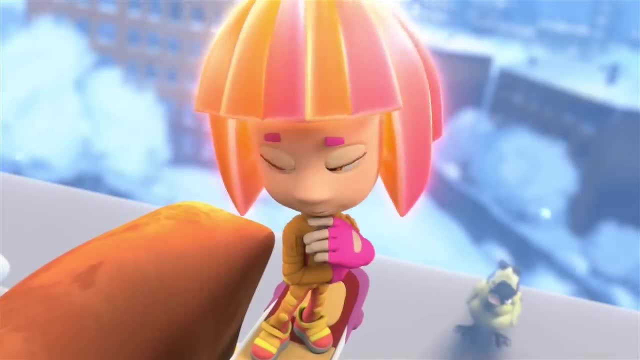 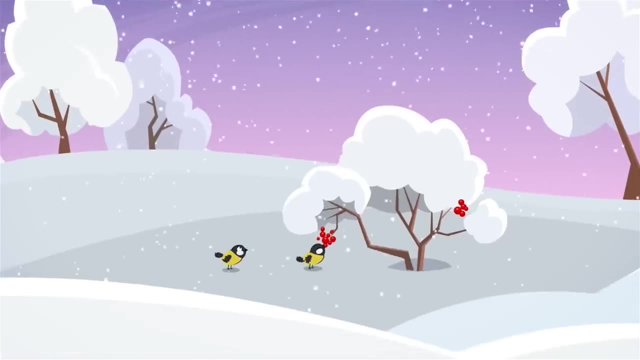 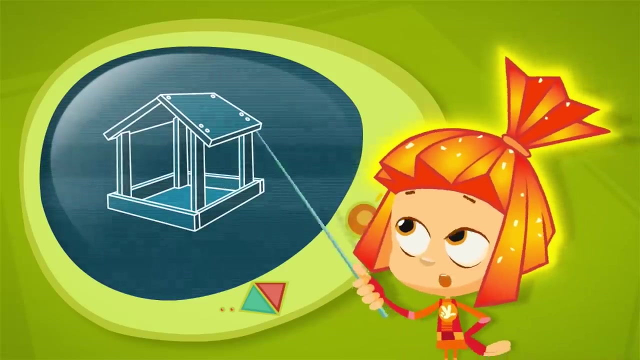 But we both know someone who knows everything In the winter. it's not easy for birds to find food under the snow. Luckily, many people come to the rescue. They build little houses for the birds, designed to hold food. The name for these houses are naturally bird feeders. 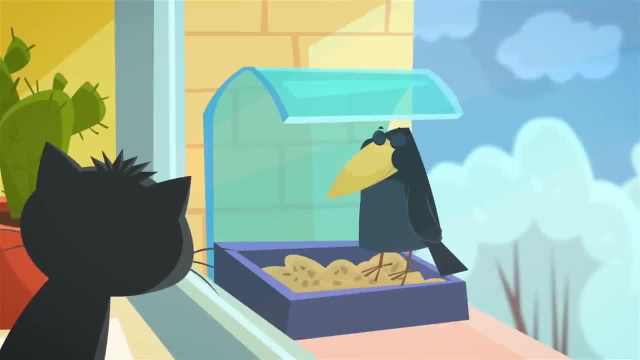 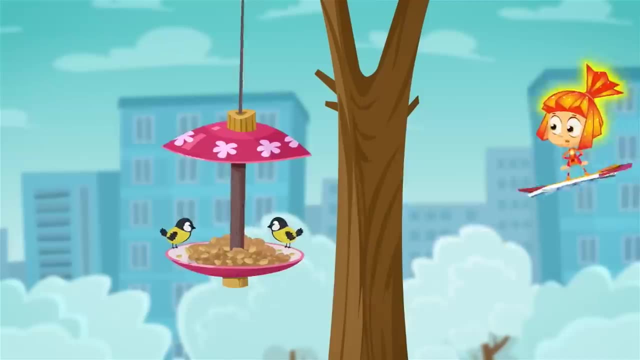 Bird feeders can be made out of wood, plastic or even something as simple as a milk or juice carton. Building a bird feeder by hand isn't hard to do at all, But building it is only one part of the work. What's most important is remembering to keep it filled with food. 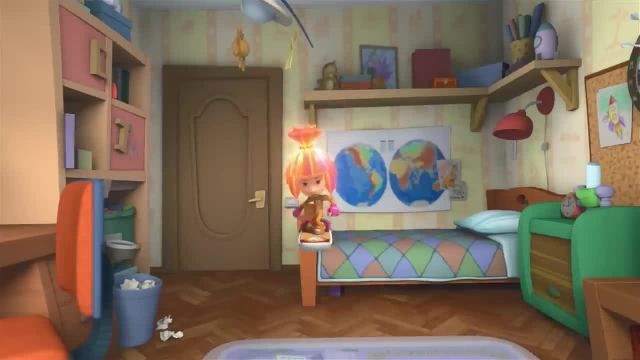 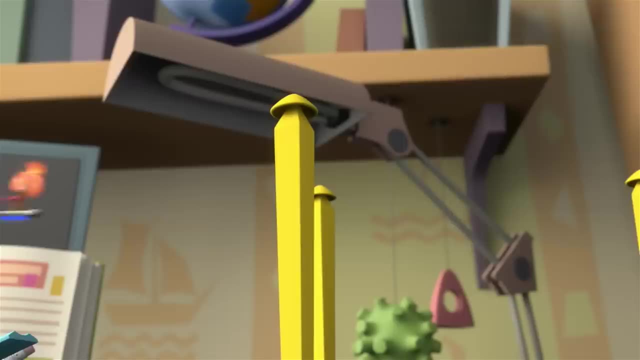 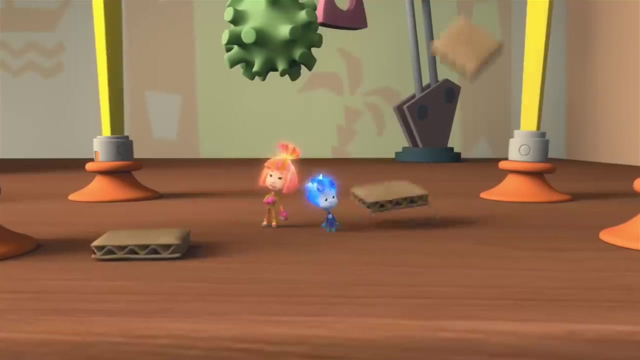 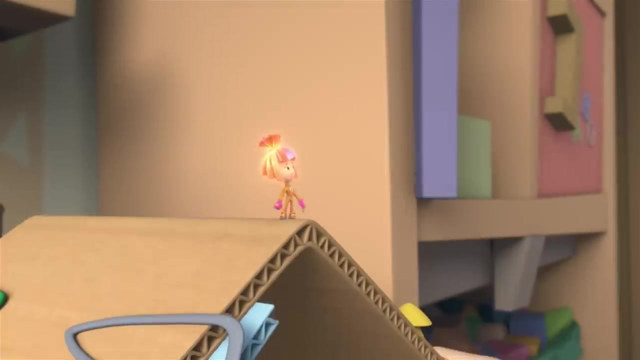 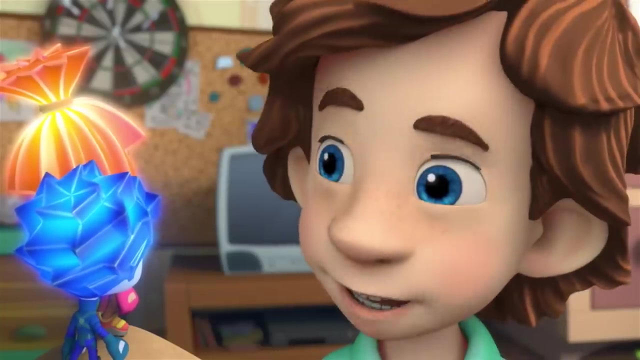 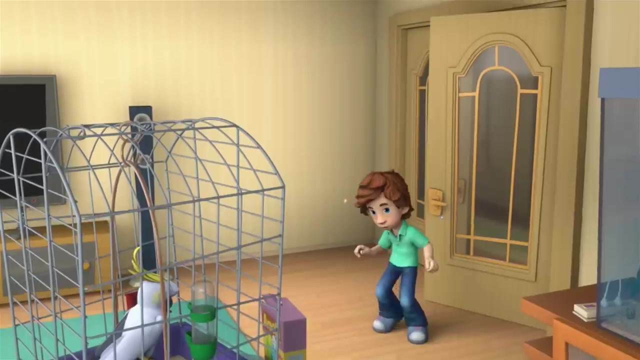 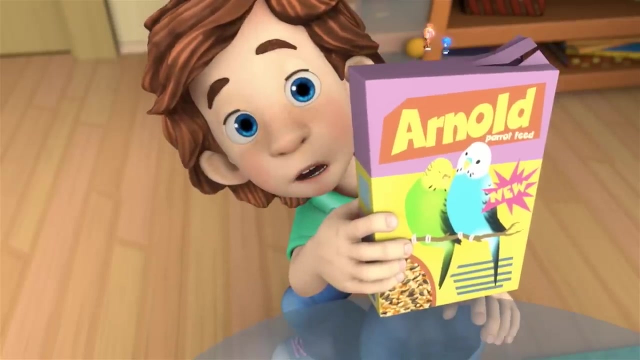 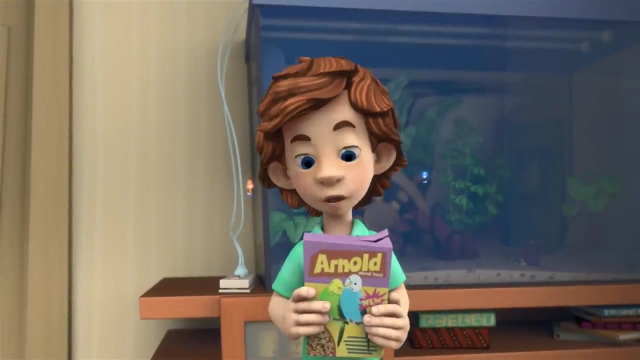 Well, shall we start? The bird feeder is ready, And what are we going to put in it? I got an idea. Adisa, I need some of your food for a little bird. You aren't greedy Greedy, Greedy Greedy. 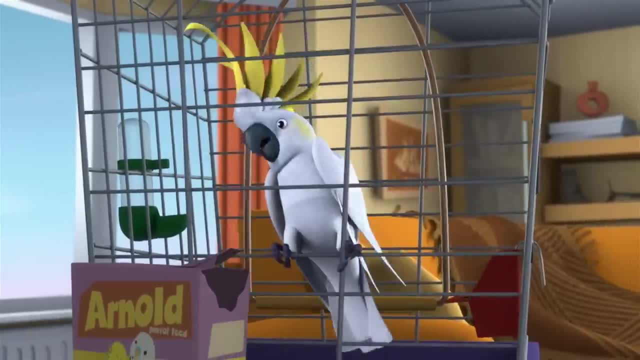 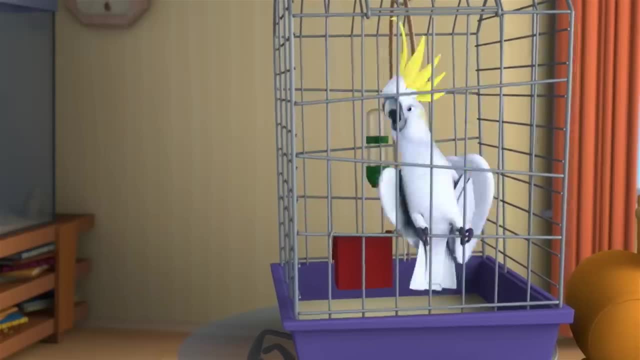 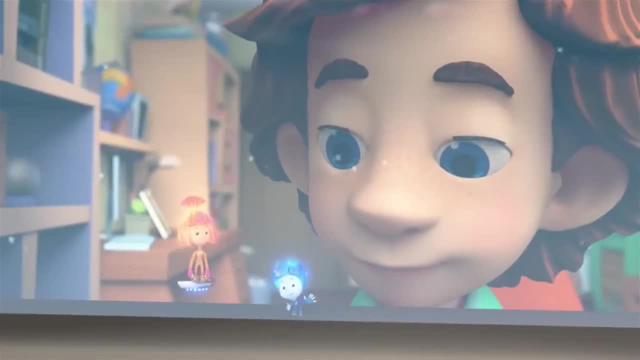 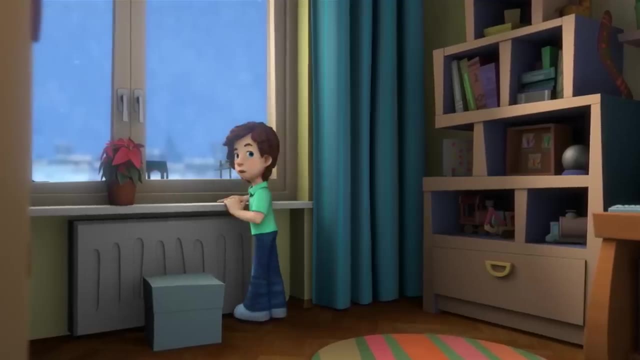 Wow, Now there's two of them out there Eats. There's enough food for everybody. Poor Adisa, Poor Adisa. Let's bring them in here. We can open a restaurant for birds. Adisa's a poor little bird. 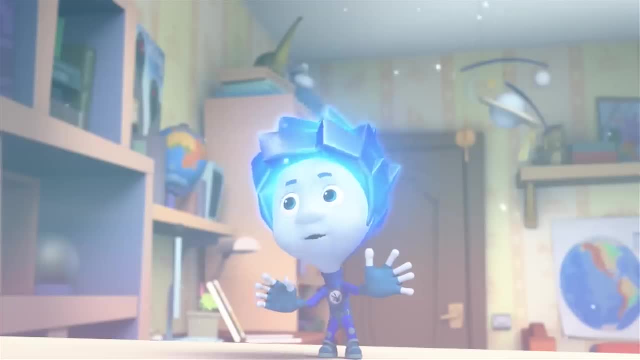 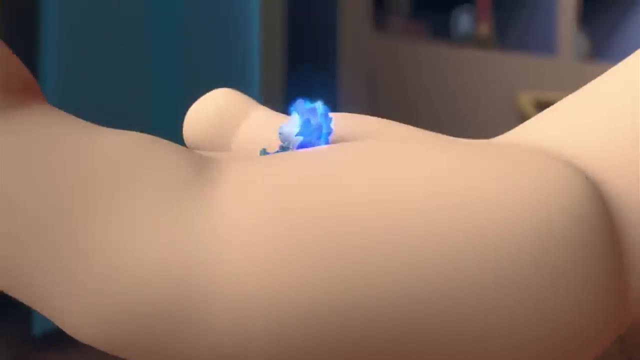 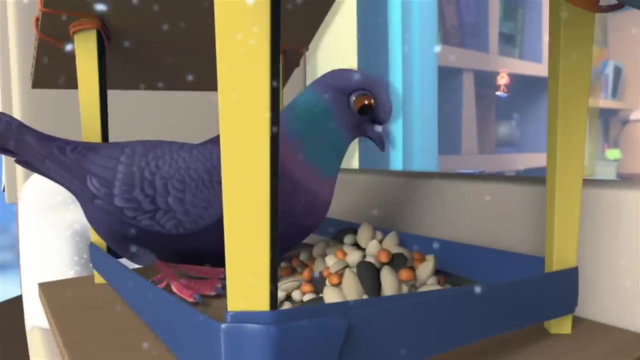 Why did you scare the little birds away? That feeder's for them, Get it, Just fly away, Shoot, He's bullying our friends. Hey, you leave, Leave. You'll never chase him away. now We'll see about that. 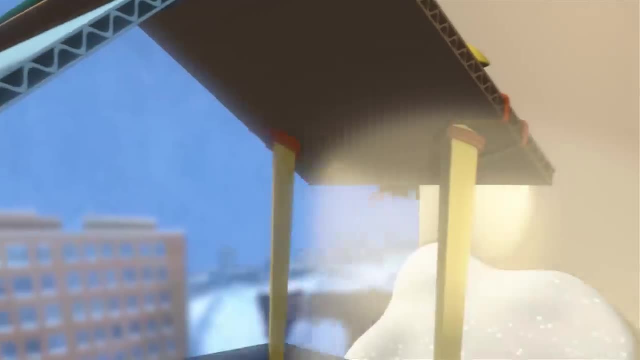 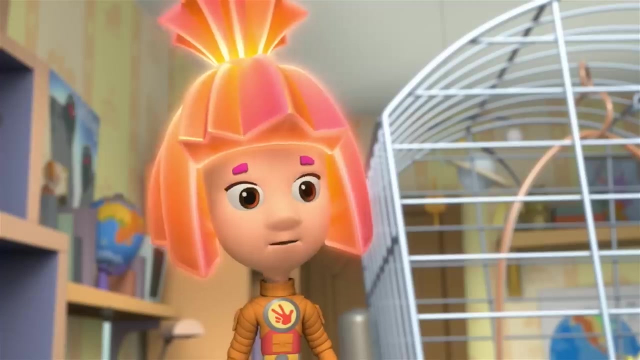 Aha, Serves you right, Pigeon. It's not nice to bully little guys. Yeah, and how about big guys? It's all right to bully them. The poor pigeon also wants some food, Food, Food, You sure. 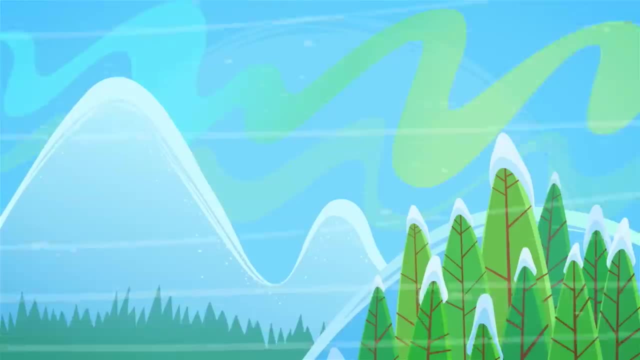 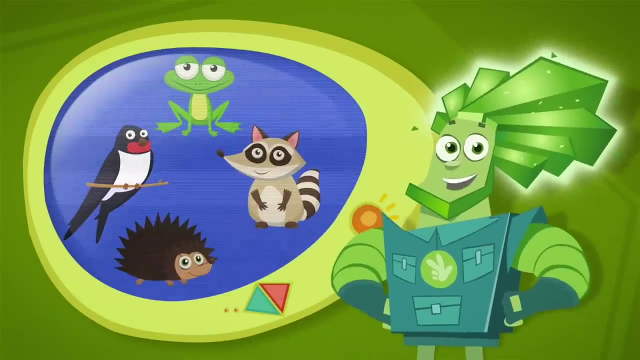 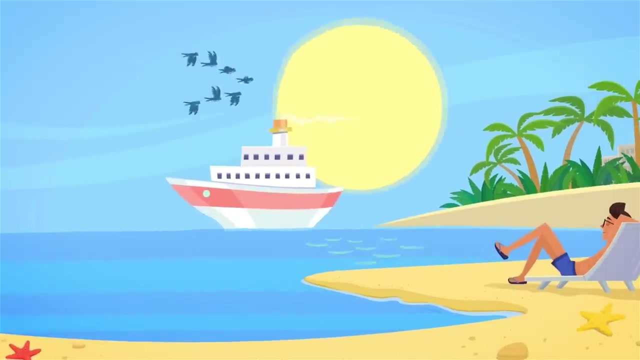 Sure Winter can be beautiful, but also very cold. Animals have different ways to prepare for when the weather gets cold. Some birds gather into flocks and migrate to where it's warmer. You could almost say they're flying to a resort. Squirrels, hamsters and chipmunks collect and store nuts, mushrooms and pine cones. 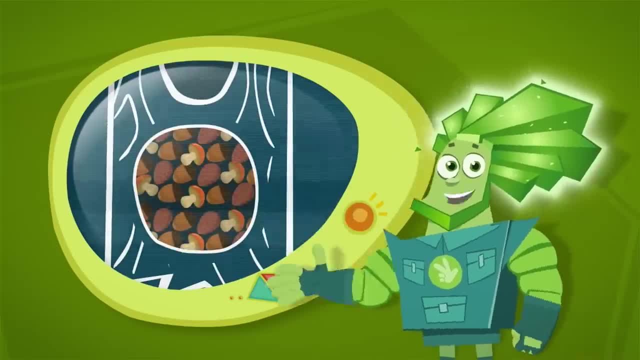 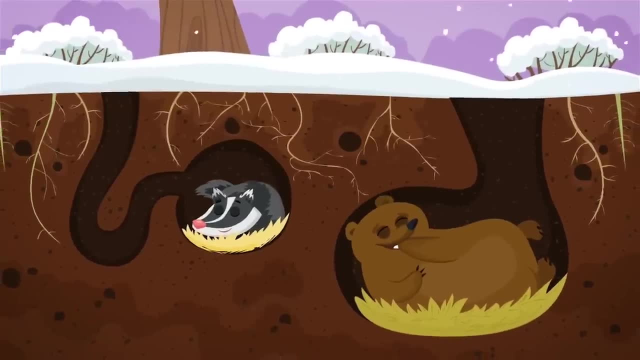 There are many people who don't have pantries that are as well stocked. Badgers and bears eat a lot of extra food in the fall and then go to sleep in their dens and burrows for the whole winter. Fish also sleep in the winter, only they're at the bottom of rivers and lakes. 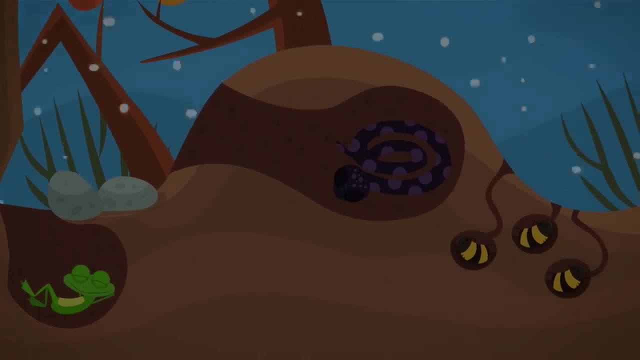 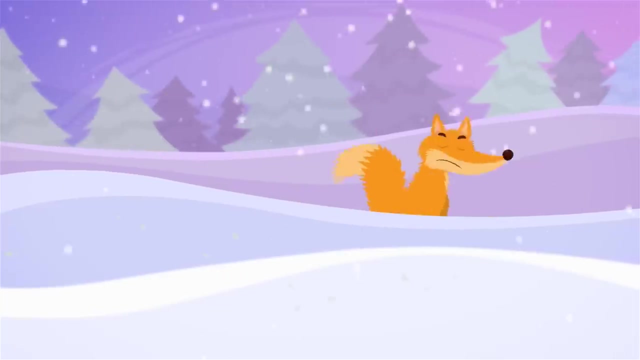 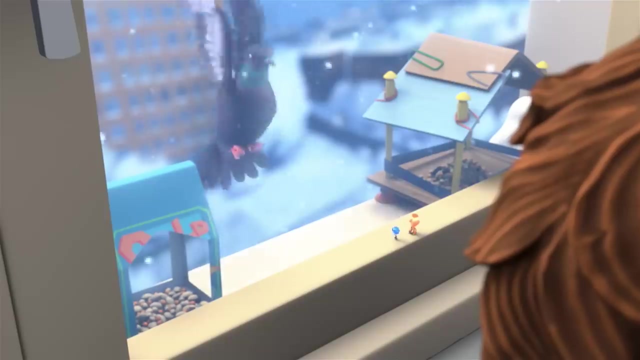 Frogs, snakes and even wasps burrow in the ground while hares, foxes and wolves grow thick coats that protect them from the freezing cold, Although it isn't easy for them to find food, So that will be your feeder. 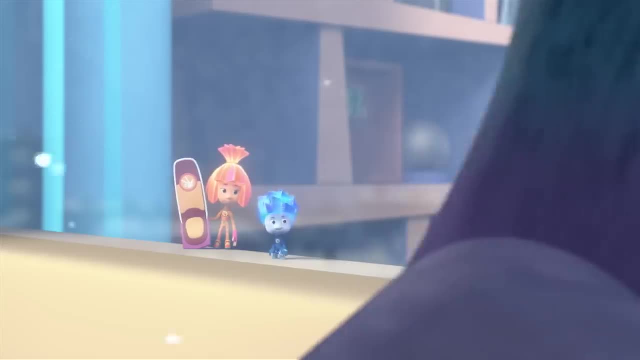 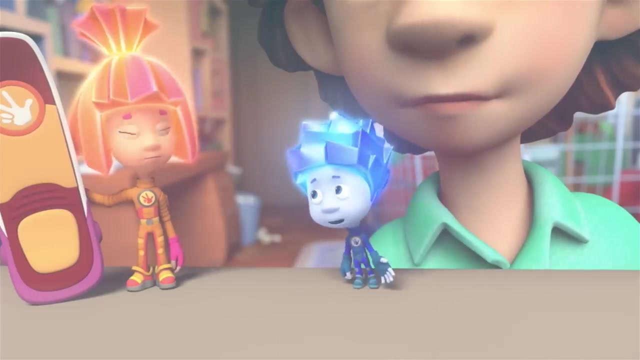 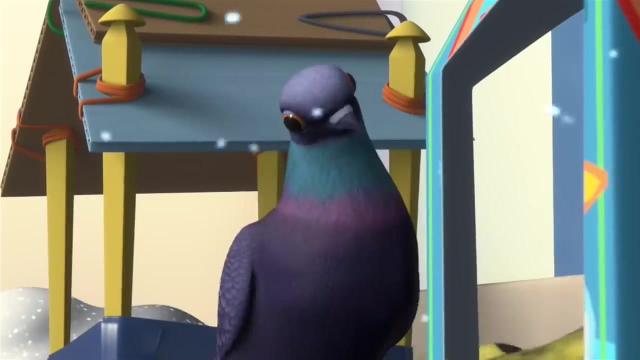 And that new one will be for the little birds. Hey, are you taking their food again? There you go, But those little birds, they'll probably never come back here. Look, Nolik, They came back. They're actually going to eat some more. 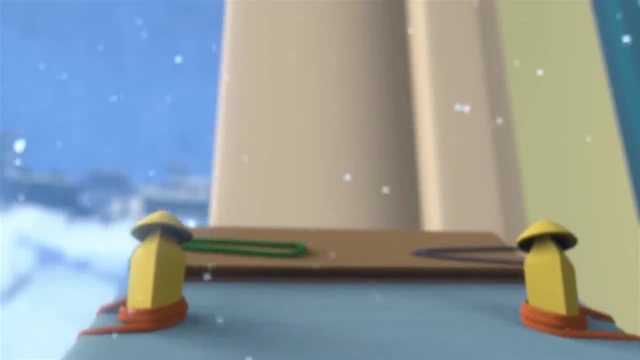 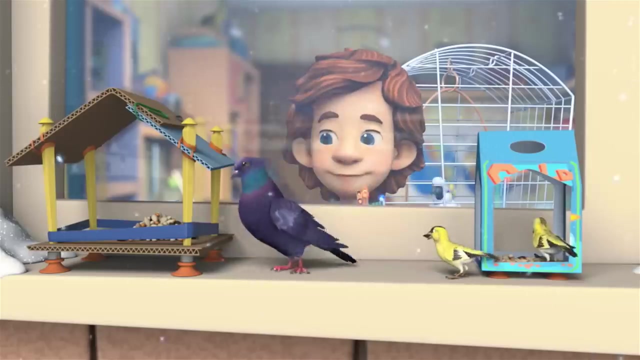 Oh, I see, Oh my gosh, And we'll soon have a big one. I'm waiting for those birds to come back. Oh, they're here, They're here, They're here. These are the little birds. They are here. 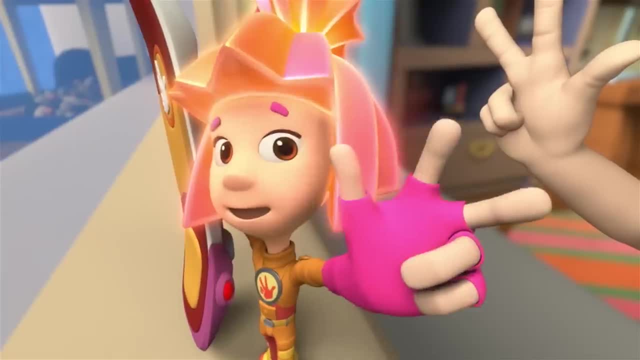 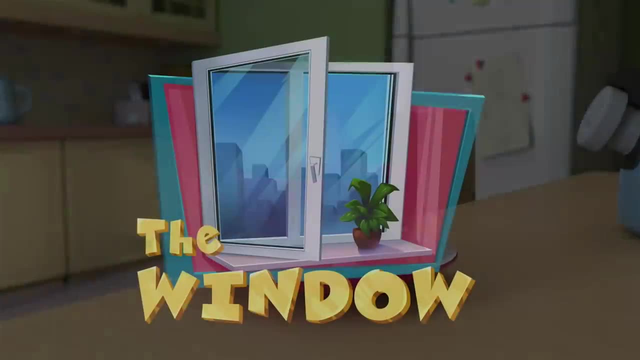 They're here. They're here. Wow, they're here. We're going to have a fun time. I'm so excited. Bye-bye, Nolik and I, Bye-bye. Bye-bye, The little birds. Bye-bye. 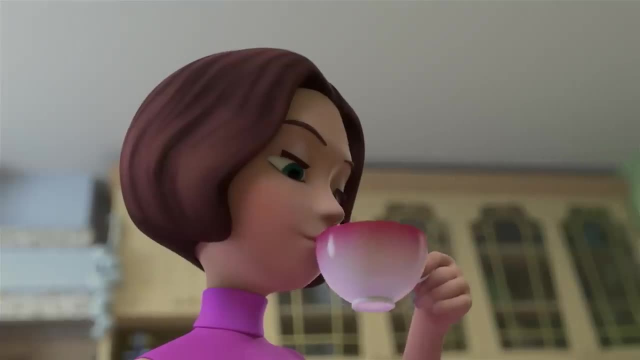 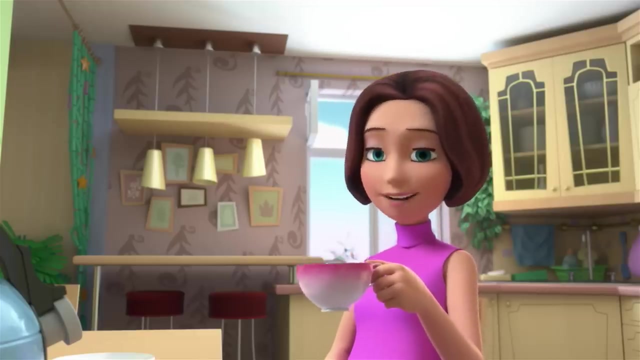 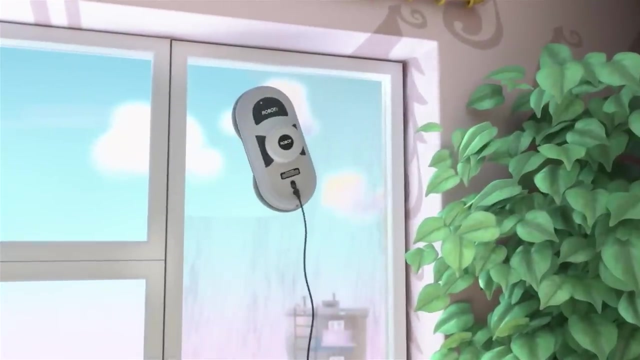 Bye-bye The little birds. Bye-bye, Bye-bye. Oh hi, there We're all up. What are you doing? I'm washing our windows. Uh, it looks like that thing's doing the washing. You guessed it: It's a window-washing robot. 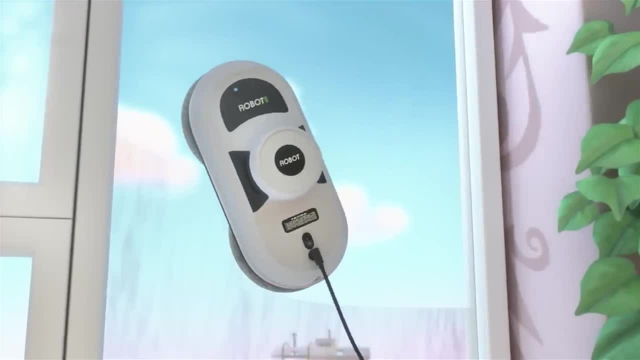 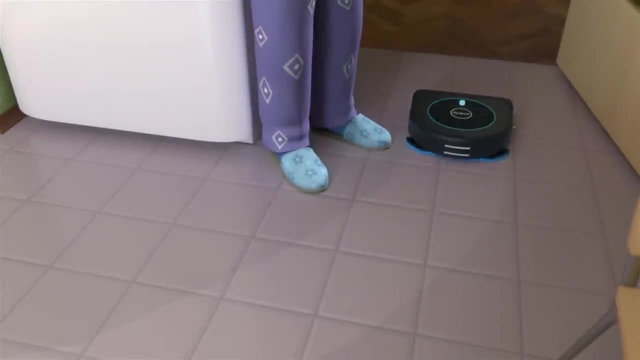 I borrowed it from a neighbor to try it out. We should buy one for ourselves. I don't get it. We've already got one robot. Uh, I mean uh robot. So we'll have two, One for the floors and one for windows. 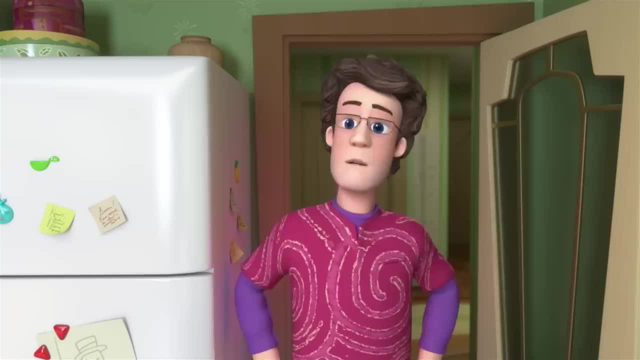 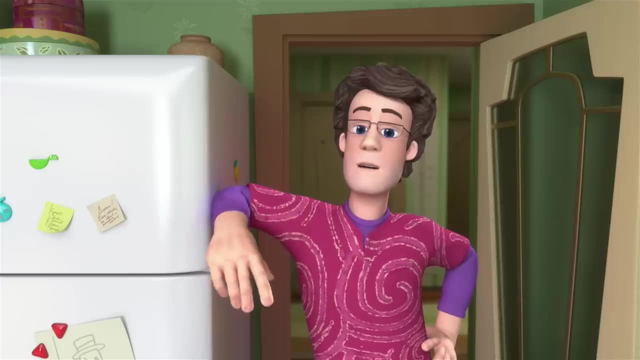 I can clean the windows, But it can be dangerous work. What's so dangerous about it? I'll just go and wash them right now, And instead of a robot we'll buy something uh useful Like a skateboard for a boy. 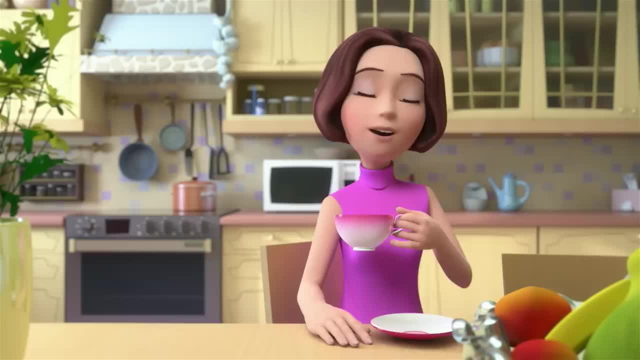 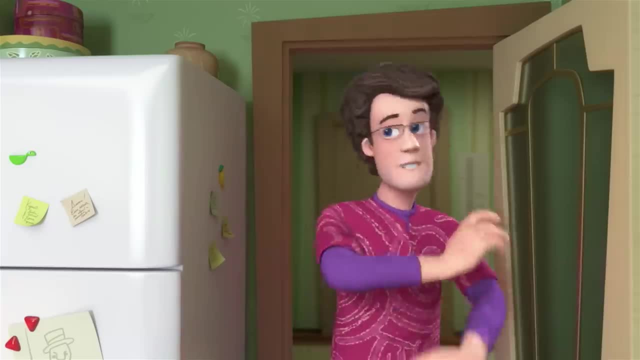 I've already got one, So you'll have two Clats. Uh-huh, If you say so, There just so happens to be a dirty window in your office. Let's see how you do it. Consider it done, Mm-hmm, And we'll clean the tiles with the robot. 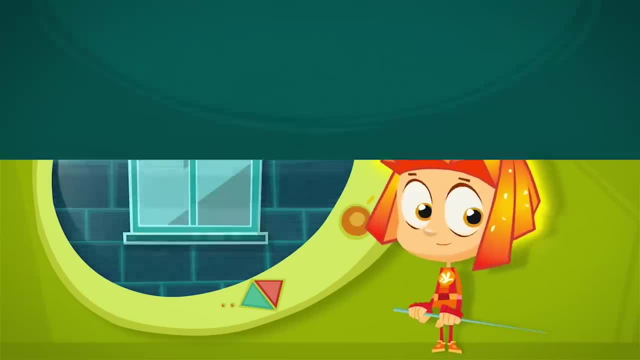 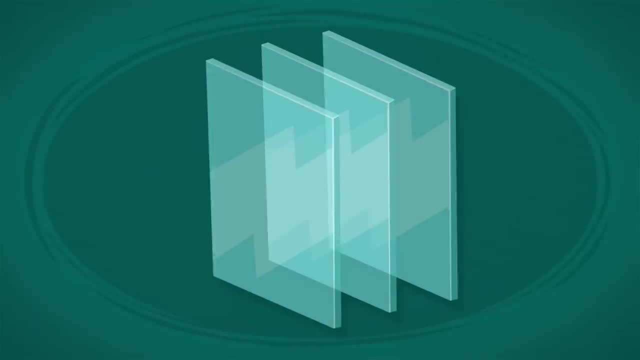 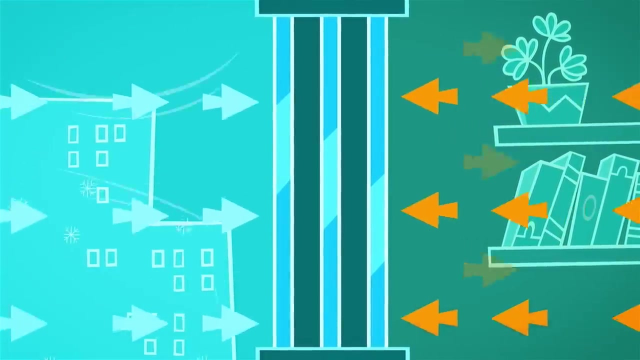 A window is much more than just a hole in the wall. Windows provide houses with light, ventilation and views to the world outside. Modern windows are made with several layers of glass. Between each layer is a space that's filled with air. The air works as insulation to keep heat from escaping. 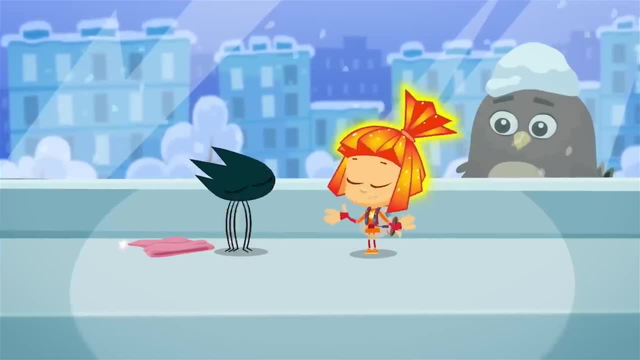 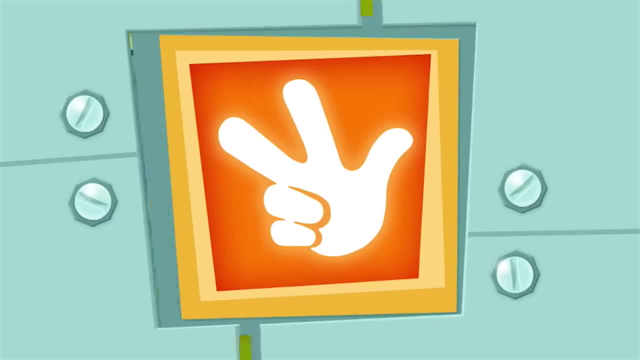 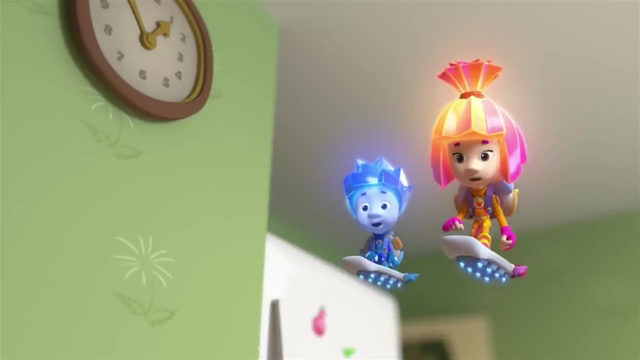 And when you're outside, do you know how to tell how many layers of glass your window has? Just shine a flashlight at it. The number of reflections tells you the number of layers. Whoa, What an amazing appliance. Let's go and take a closer look. 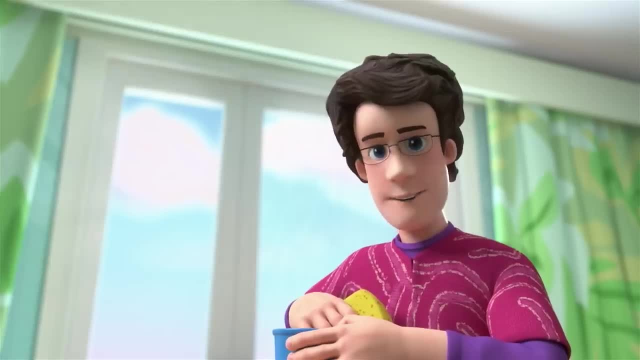 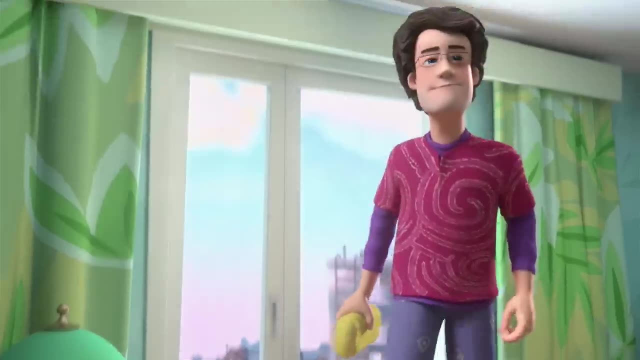 You'll really buy me a new skateboard, Dad. That's what I said, But first I've got a window to wipe. All right, Robot, We'll show ya. Tom Thomas. Dad can show him himself. We really live on a super high floor. 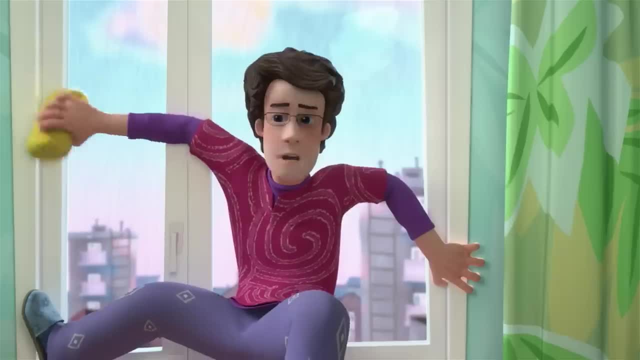 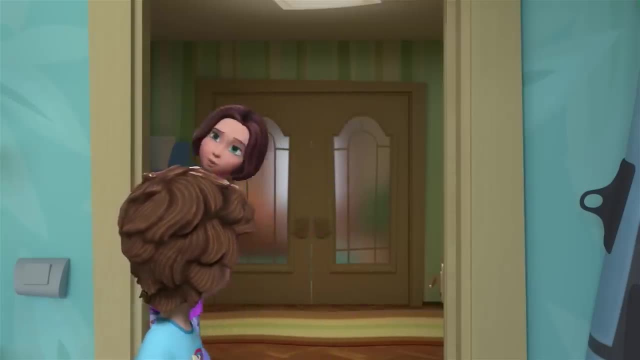 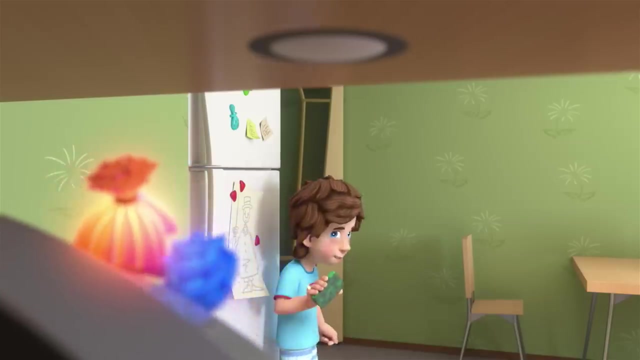 Yeah, but the robot isn't afraid of heights. I'll start from this corner. It'll take you forever that way. Admit it, the robot works better. We won't. We're gonna win this thing. Hey, what is he doing? 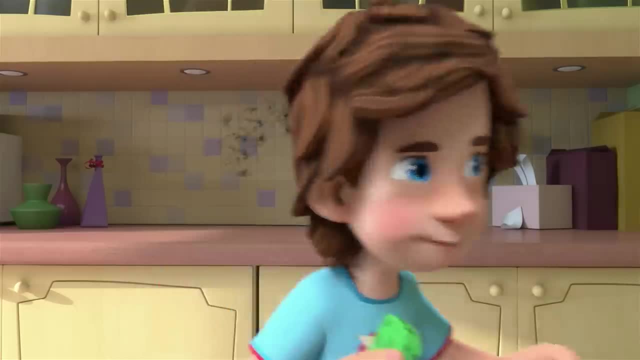 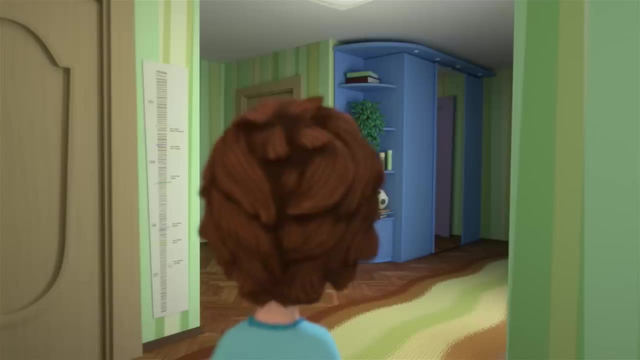 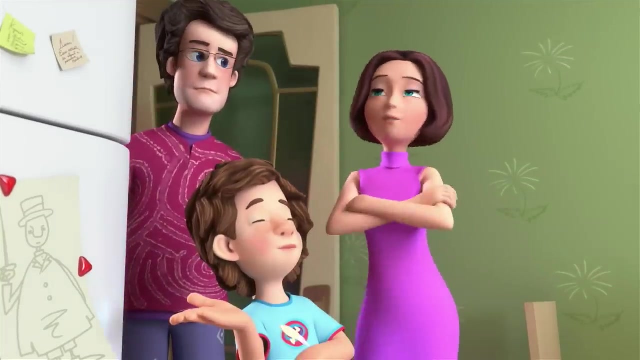 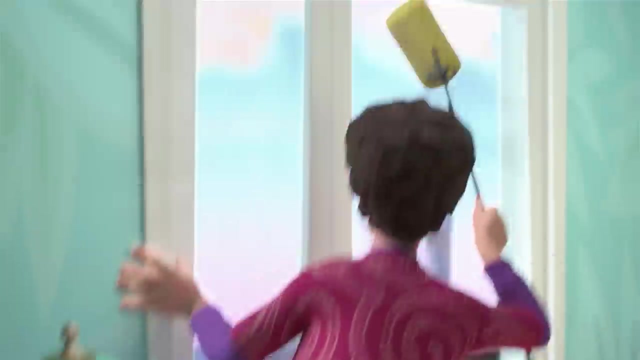 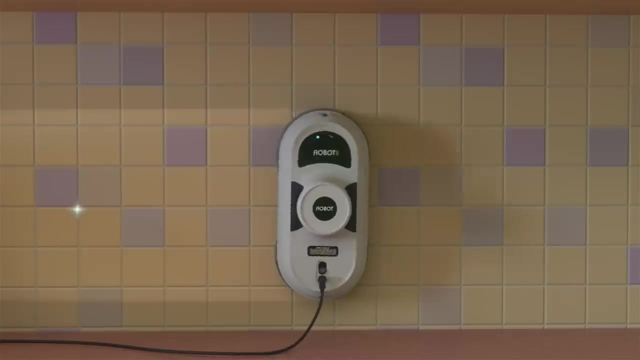 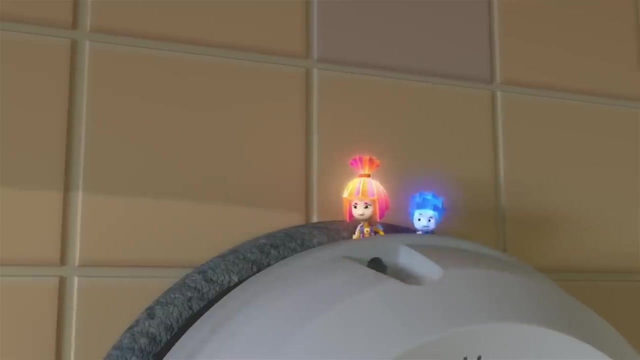 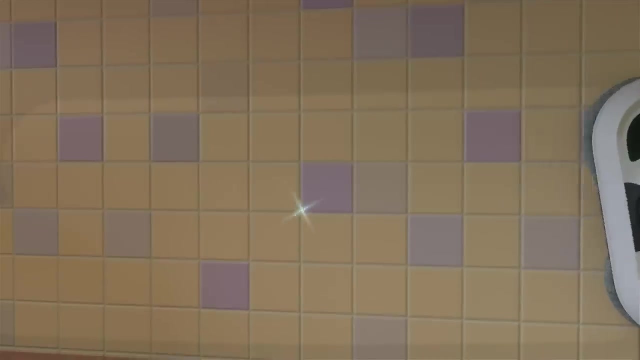 I'm not sure. Huh, Mom, Mom, The robot made such a mess in there. It's impossible. Look Good joke. Just wait, I don't get how you're cleaning it. Easy, You can talk. You gotta be kidding. 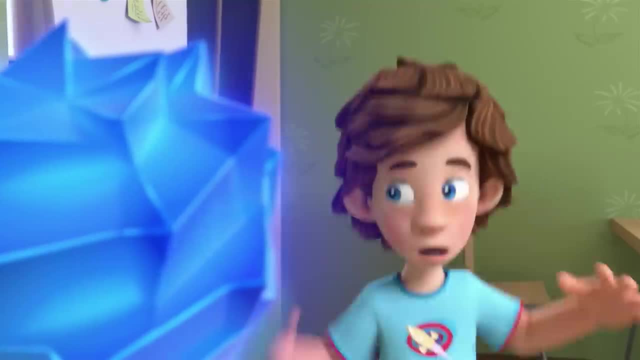 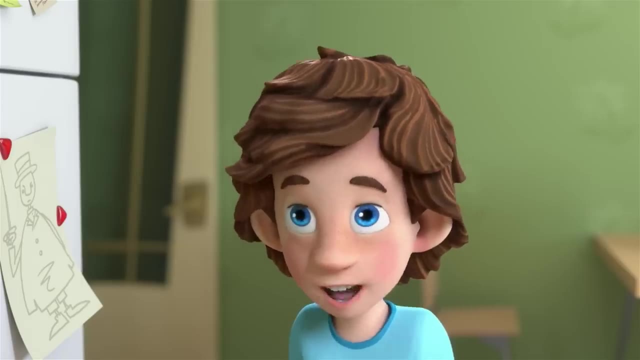 And you were misbehaving. You guys, You're the ones trying to stop me. I tried to make the robot look bad, so we had to defend it. It's only because my dad told me I'd get a skateboard. Yeah, For doing a bad thing. 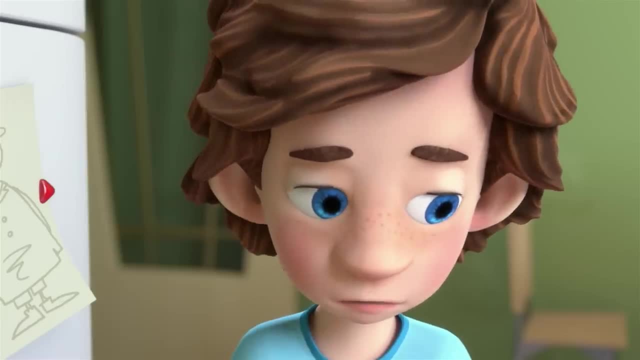 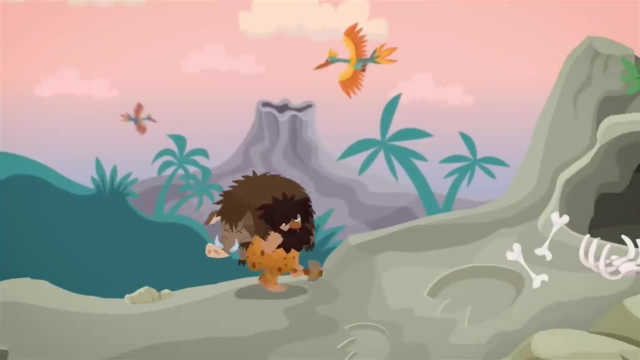 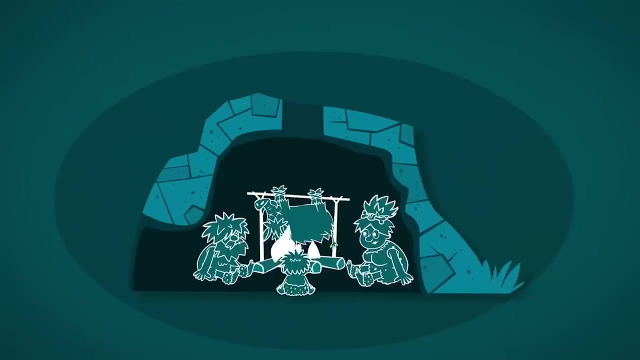 Aren't you ashamed of yourself? I am. You learned your lesson And don't forget Fixies. look out for appliances. The dwellings of most ancient people had basically no windows at all. There may have been a hole up above for letting out smoke from a fire, but that was it. 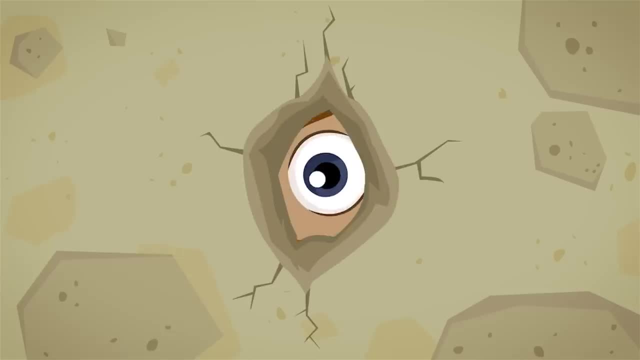 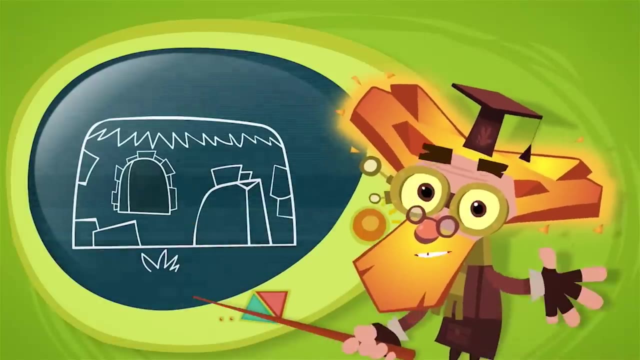 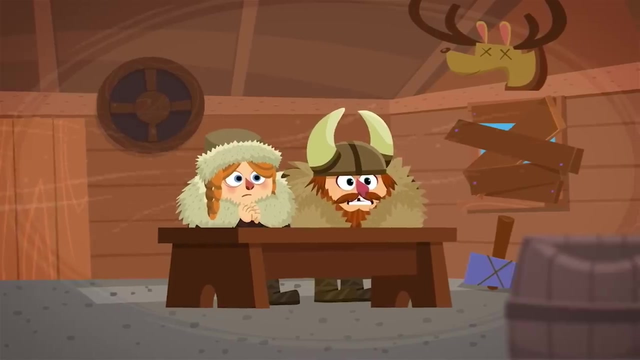 Later people started splitting open their walls, but the openings were so small that very little light would ever get inside. The size of windows grew quite a bit over time. People would cover them with animal skins, fabric, paper or wooden planks to protect themselves from the cold and the wind. 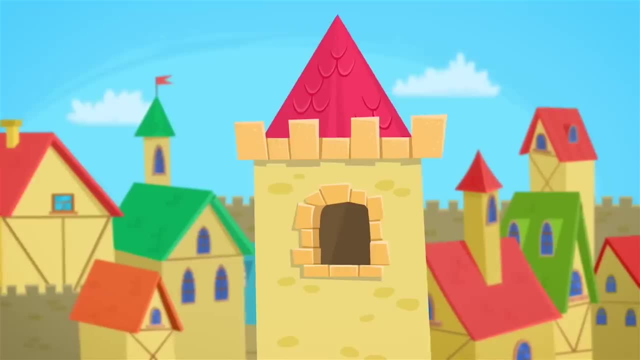 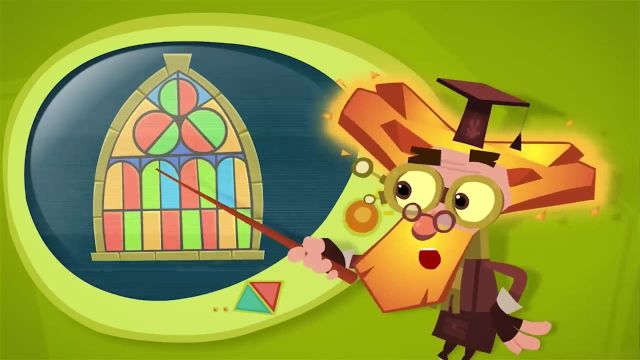 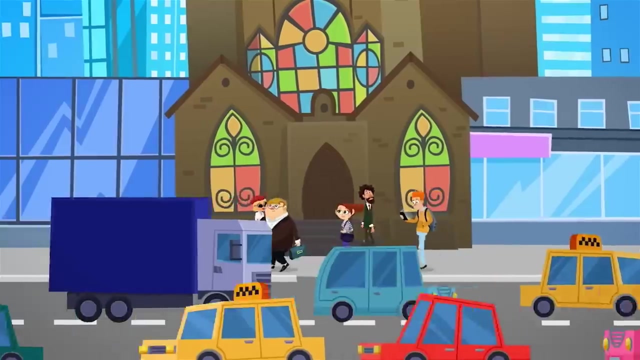 When people learned how to mine valuable minerals, they began to cover window openings with thin sheets of a mineral called mica. Windows made of glass were very expensive And only the richest people could afford them for their homes, But today it's hard to imagine a window anywhere not covered in glass. 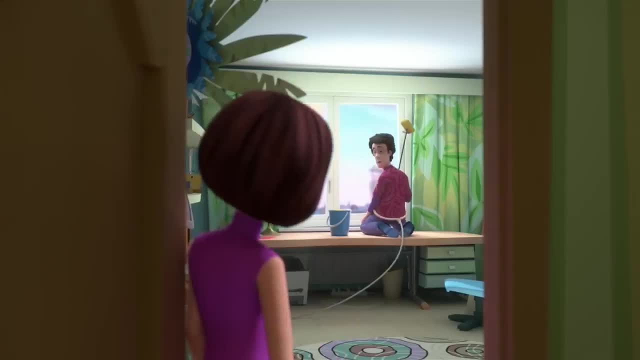 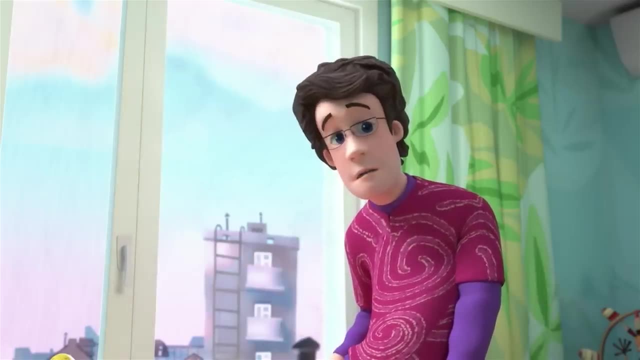 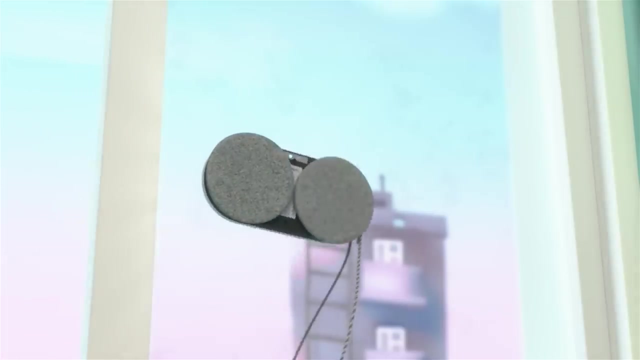 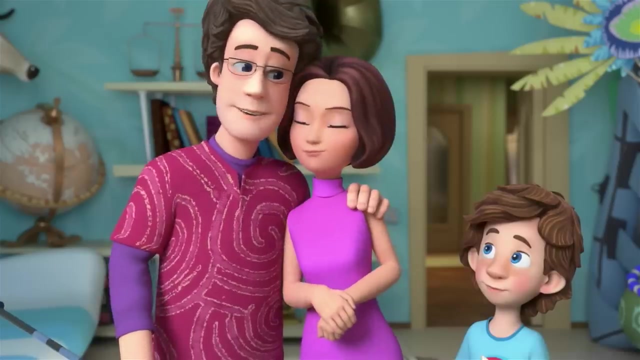 Everything's washed. And what about the outside? Forget it. I I quit. Would you wash the back with the robot? Yeah, consider it done. Yeah, you're right, I see It really is a great appliance, And that washer's defender is even better. 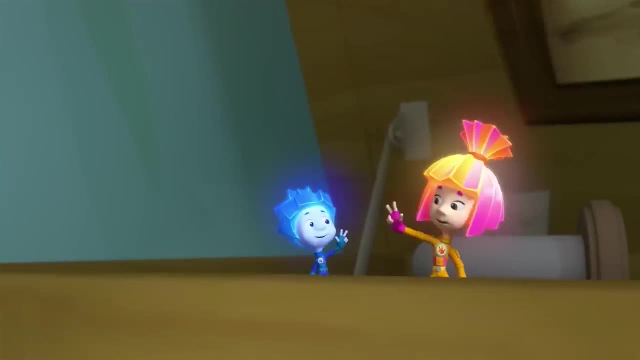 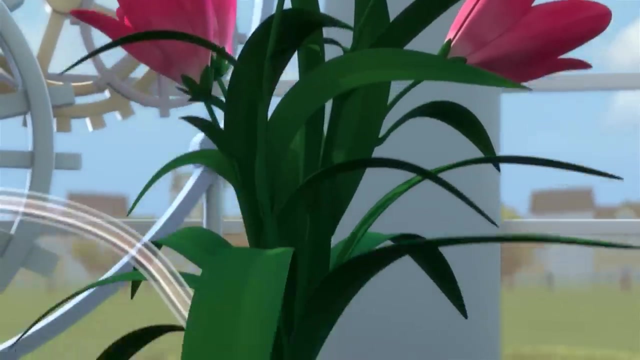 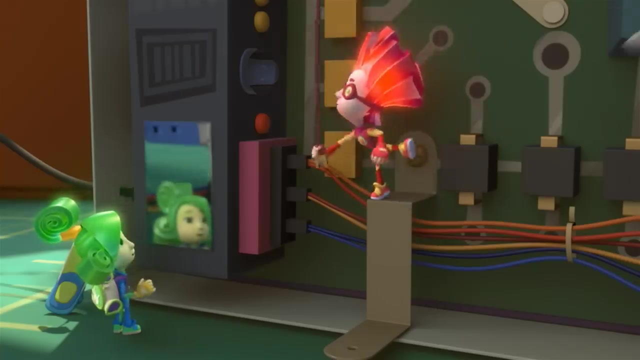 You're right about that, Tideesh. Oh wow. What kind of device is that? Maybe an alarm clock? No, This is a time machine. Beep, beep, beep, beep, beep. Time machines, They don't exist. 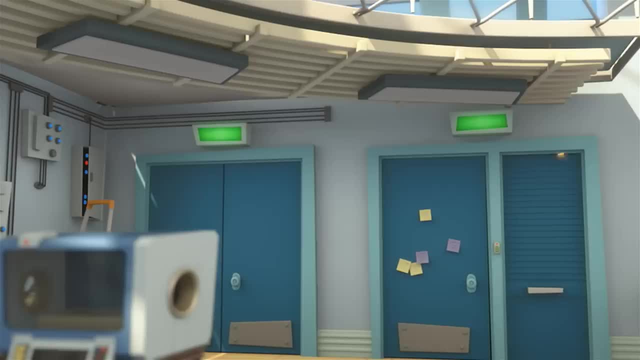 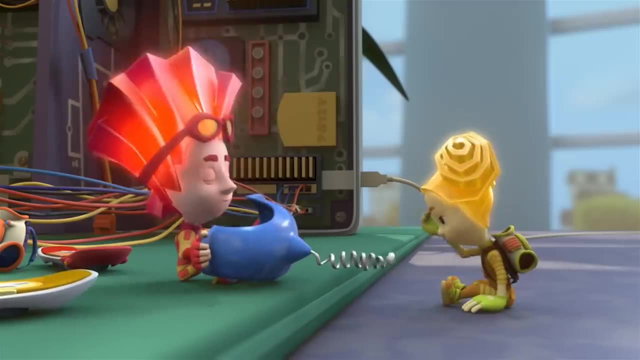 Whoa, What a shame. I learned that, Studied that. Well done, Toola. Whoa, What did I just bump into? What do you mean what? Into a time machine. But I thought, time machines aren't for real. 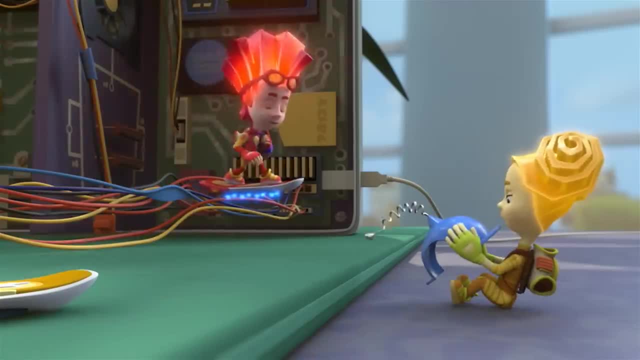 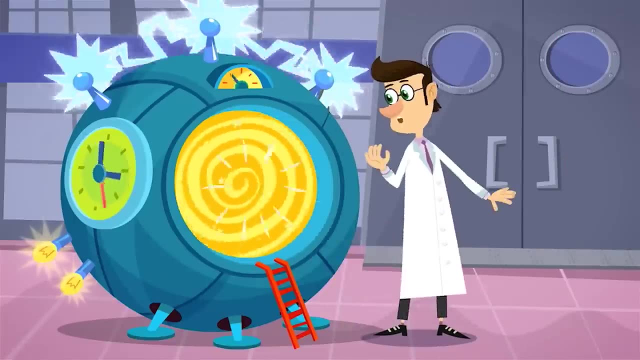 Of course they are. You get in and take off for the future Or the past. Splendid Tideesh, Tideesh, Tideesh, Tideesh, Tideesh. I could still learn how to travel in a time machine, Maybe to go back in time and fix a bad grade. 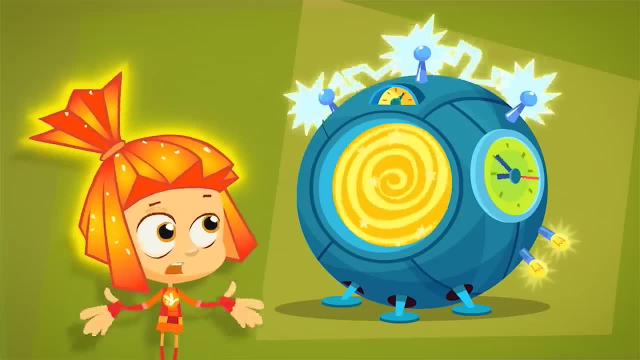 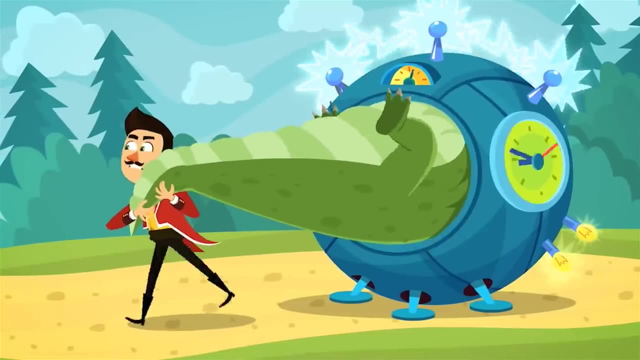 or to get a peek into the future. Of course it would be interesting, but time travel isn't possible, and thank goodness. Just imagine how mixed up everything could get. Someone brings back a dinosaur from the past, while someone else brings aliens from the future. 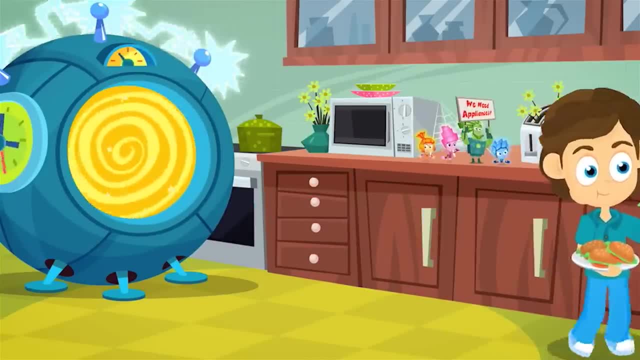 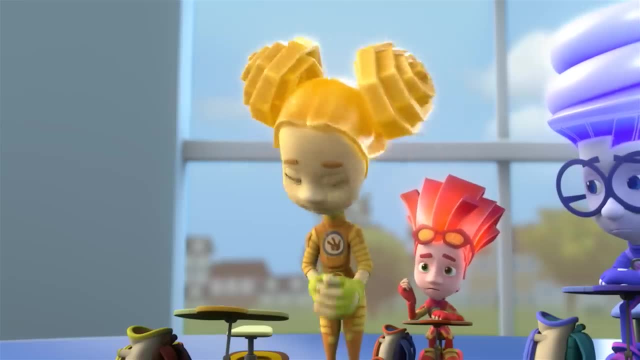 No one would need to invent anything, Appliances would sit unused and Fixies would have no work to do. It's awful. So you've got no idea of the answer, But I don't remember Too bad, because tomorrow we've got a hard test. 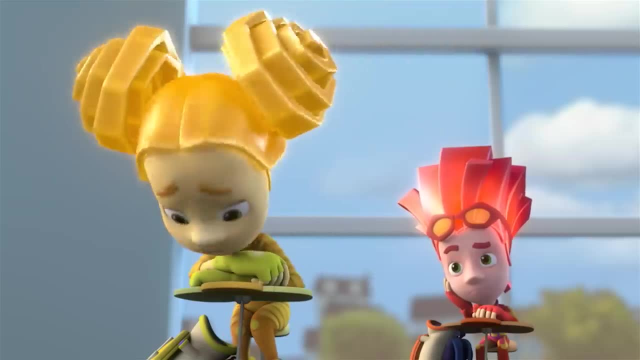 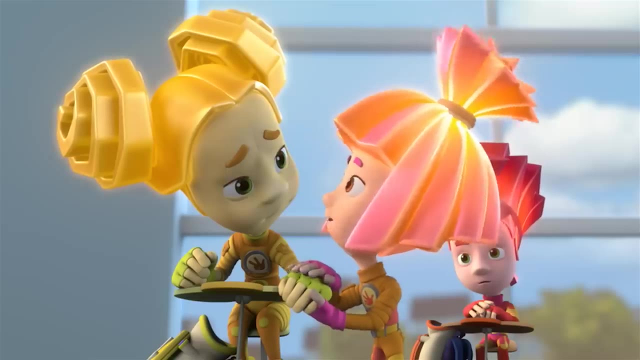 Make sure you're prepared. I'm sure I'm gonna fail. You're gonna pass. You studied all of this right, So So you just need to stop worrying so much. that's all I wish I could, Poor girl. 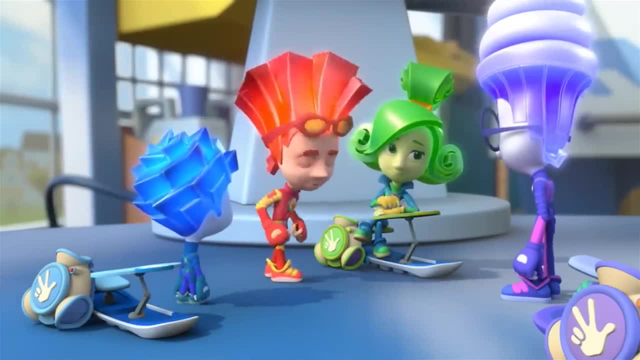 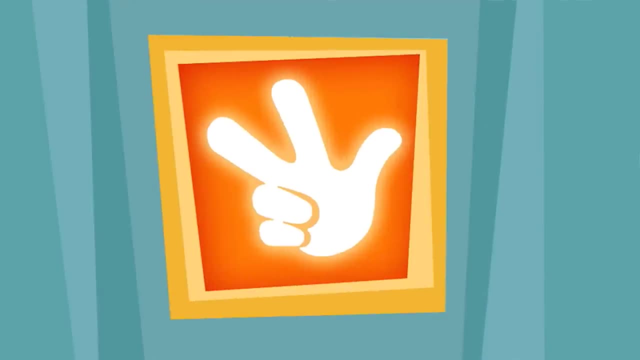 How can we help her? Hey, I know how This morning Toola believed that that thing over there is a real time machine. Sounds like an anti-scientific plan. Stop worrying, It's simple, We'll send you two tomorrow. 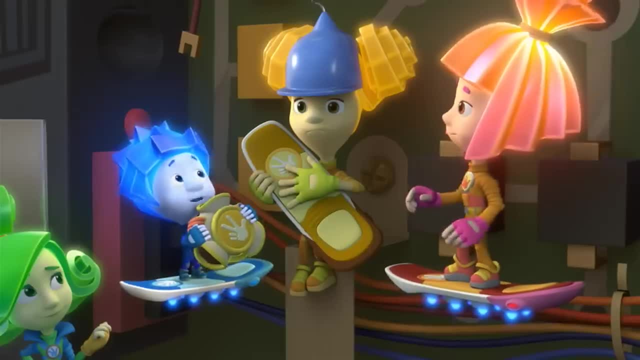 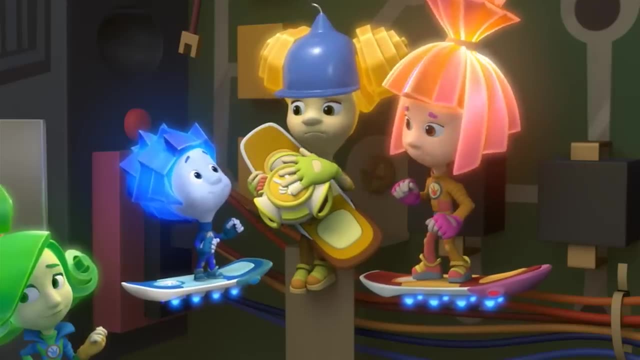 you'll sit down, take the test and come right back here. I wish I could go. It's like a dress rehearsal: The main things not to worry. Then what do I do? You just pull on that wire and you'll get them back. 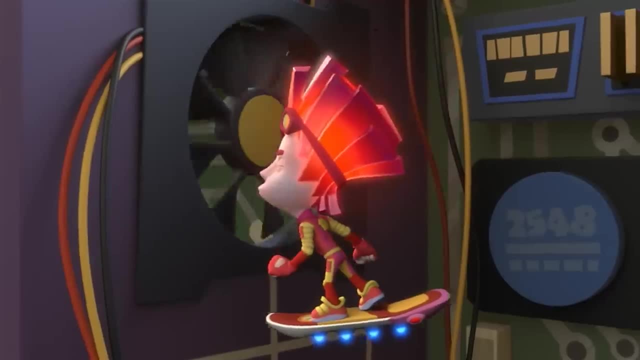 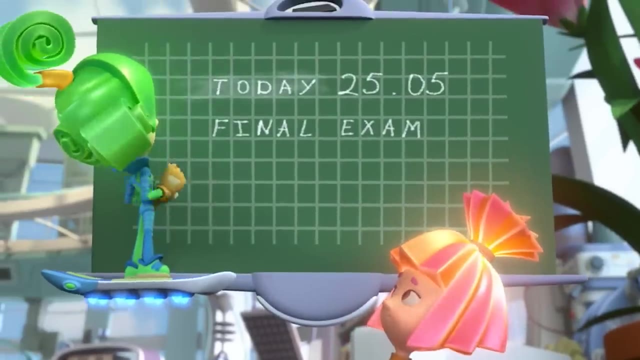 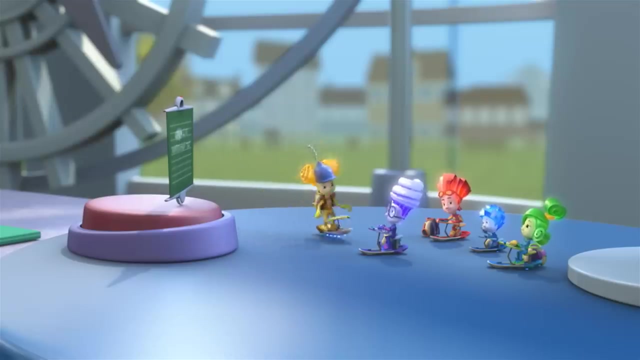 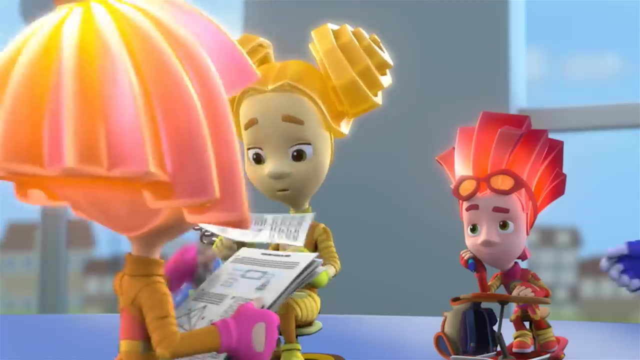 Well, time to go. Wow, it's tomorrow. Hi there, Are you ready? Uh-huh, Grandpus got sick, so I'll be giving you your tests. I'm scared, Don't worry, it's just a rehearsal. 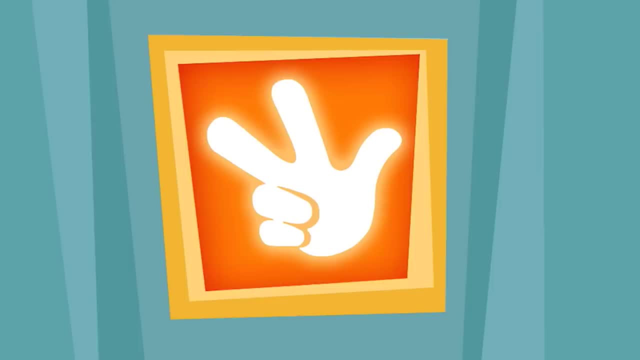 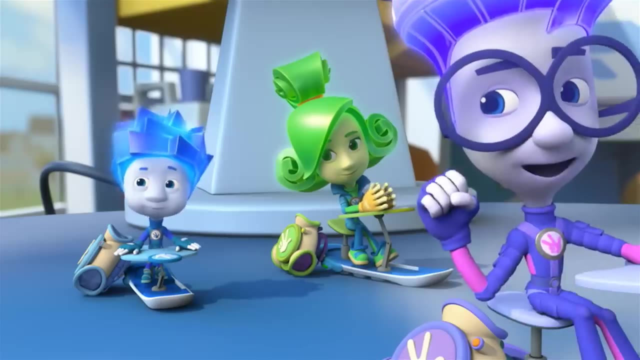 Well then, who had the best test? Congratulations: Toola So cool. I'm so happy, I'm so happy, I'm so happy. Toola So cool, Awesome, That wasn't scary at all. Impressive, By the way. what's wrong with the professor? 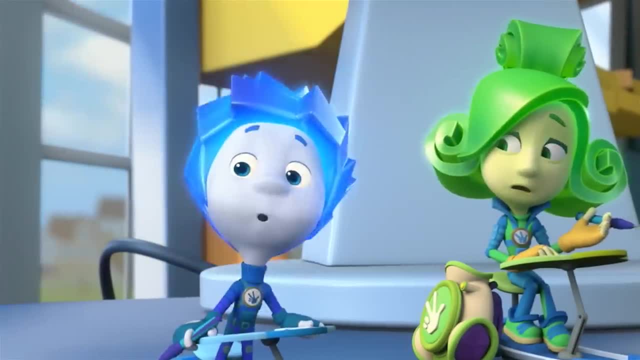 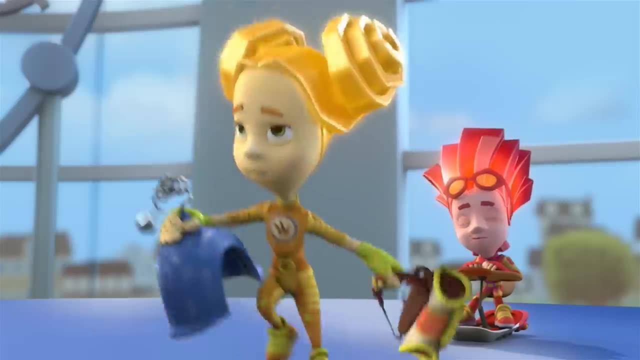 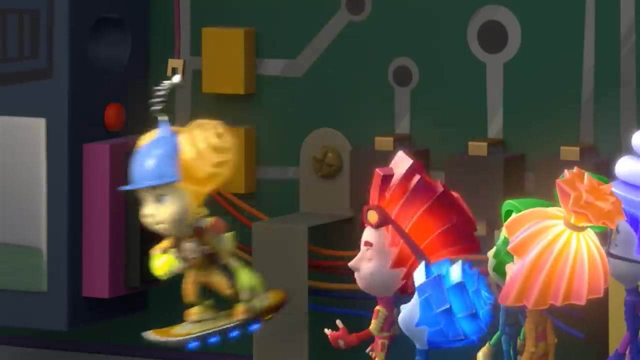 Uh, Grandpus, Uh, you know, don't you? A bolt fell on his head. You dropped it, remember I did Yeah, yesterday. I'm not sure I like this future. Well, how did it go there? 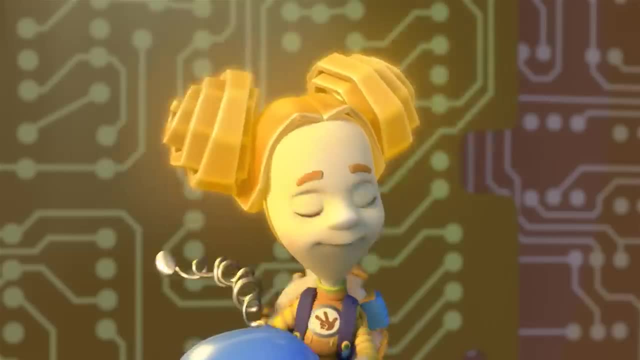 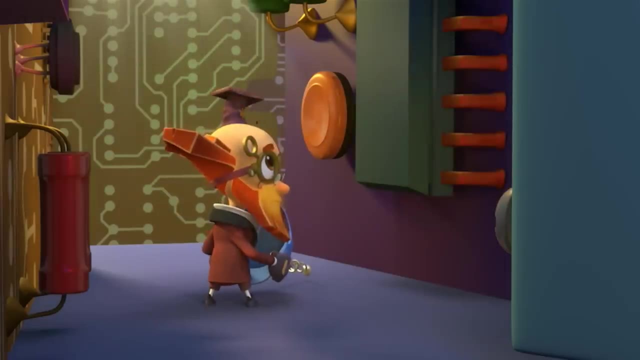 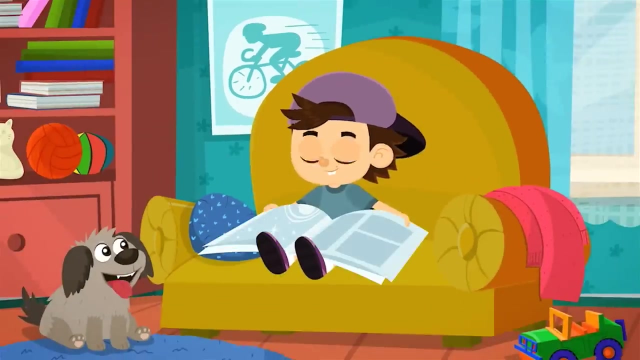 Later. But if you meet a Fixie, please don't let their secret out. Leave this on until tomorrow. What is this? Come back? No, If I do, I could hurt you, Me. What for? Wouldn't it be incredible to travel into the future and see what you'll become? 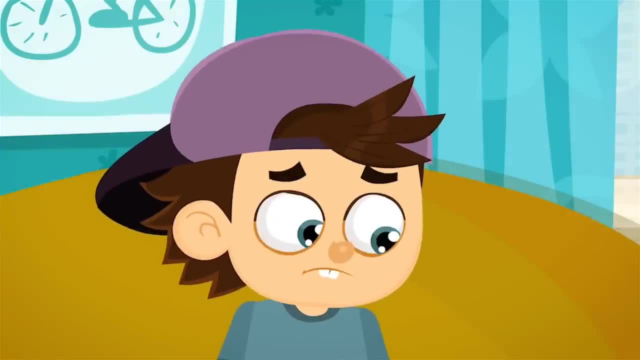 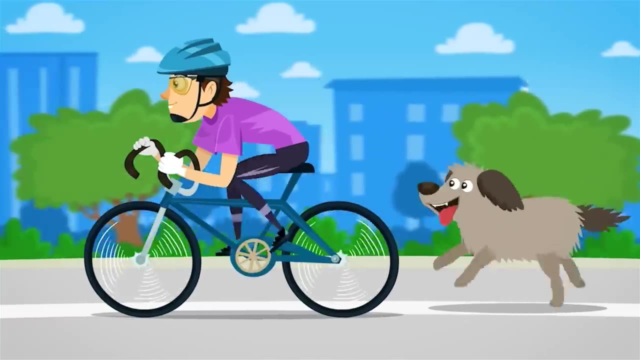 Unfortunately, that's only possible in our dreams. But if you have a dream and aren't afraid of challenges and setbacks, your future can turn out just the way you imagined. Do you want to become a champion? Then you need to start your training. 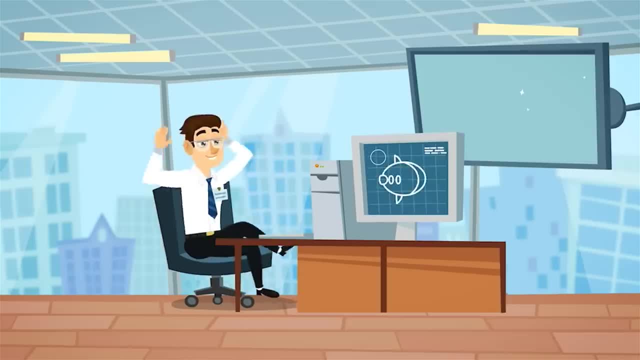 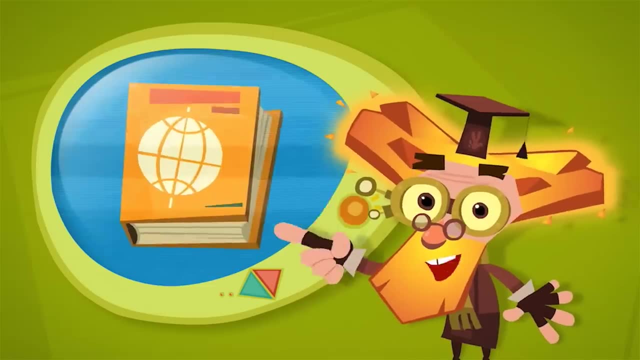 right away. Do you dream of becoming the best programmer in the world? Then first pull up that grade in math class. Do you dream of sailing the oceans? Then you'll need to do a lot of reading, because a captain has so much he needs to learn. 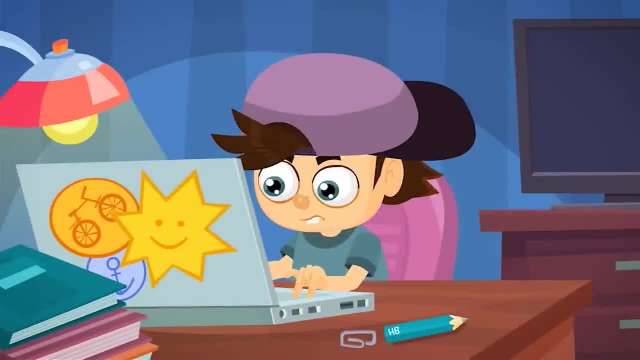 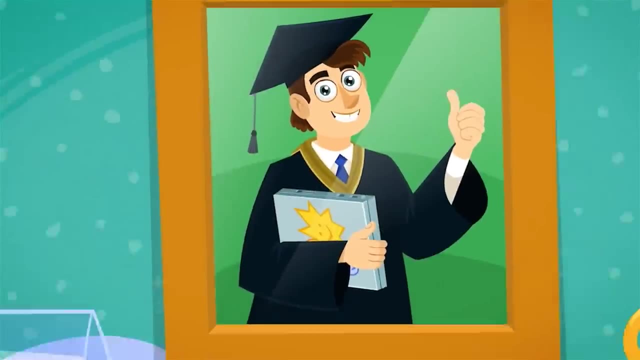 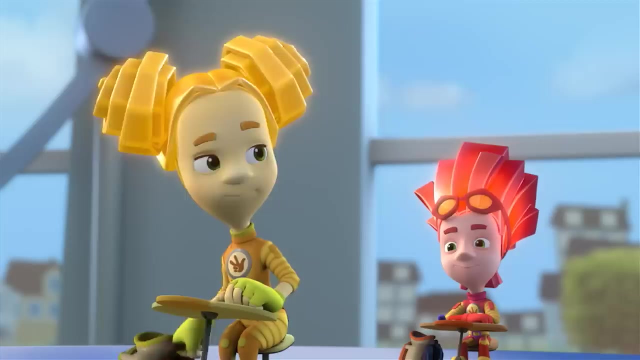 Start creating your future right now, And we Fixies will be right there to help you, making sure the machines you need to reach your dreams will keep on working for years and years to come. Hey there, are you ready? Uh-huh. 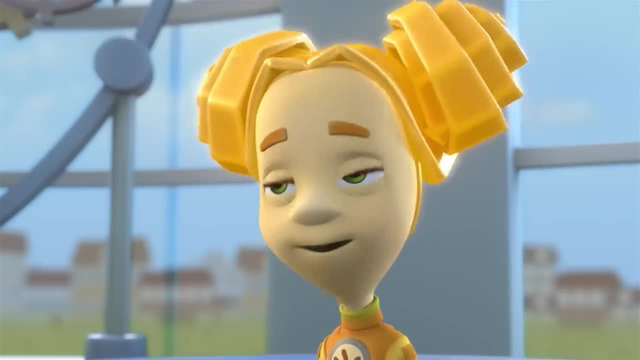 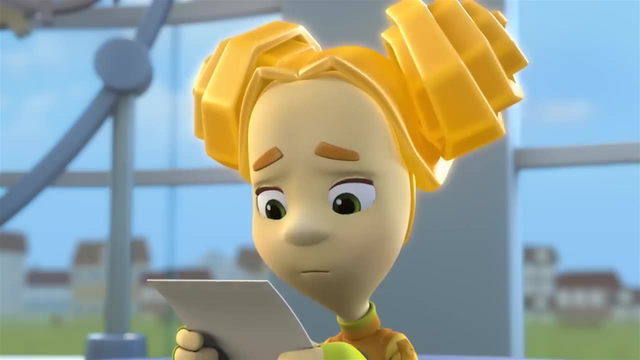 So far, everything's exactly the same. Toola, take this, please- It worked- And pass out the tests. You may begin. These questions are different. Who had the best test? Congratulations, Toola. What am I worried about? 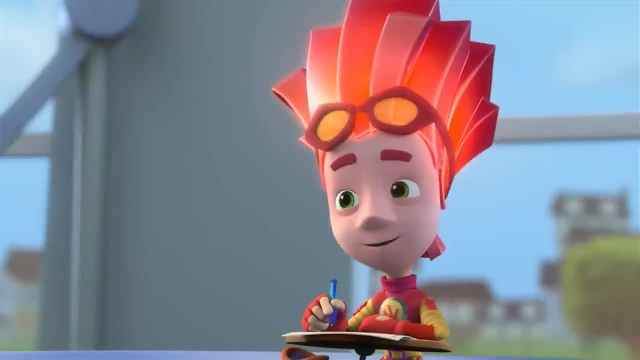 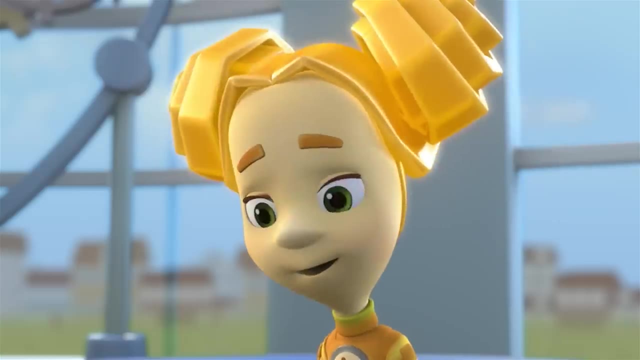 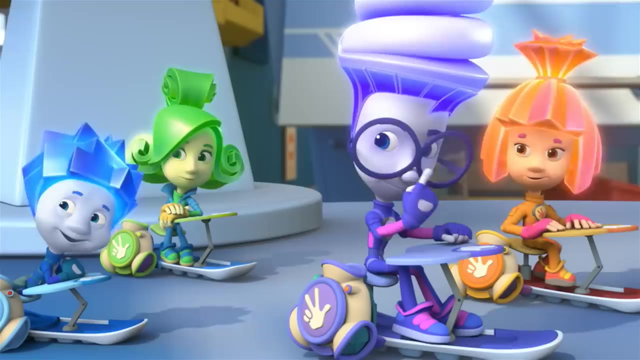 I know everything is going to be fine, Tideesh. Well then, All of your test results are great. Only none of you could guess what this device is. What do you mean? Isn't it a time machine? No, it's from automatically watering plants, that's all. 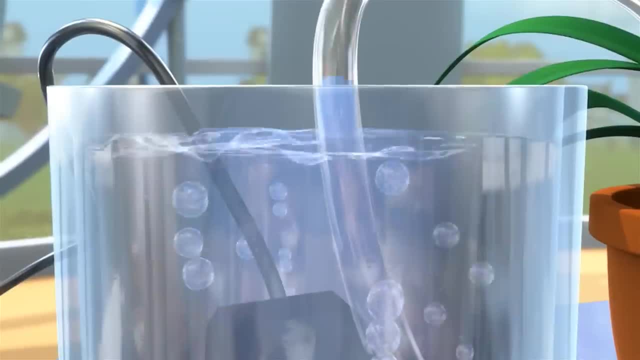 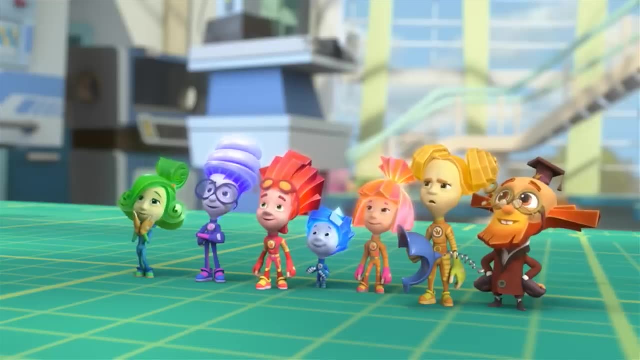 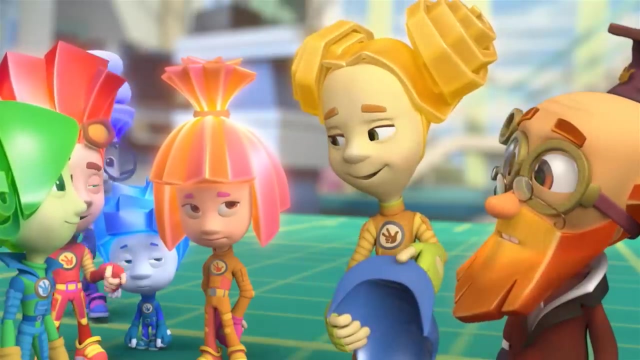 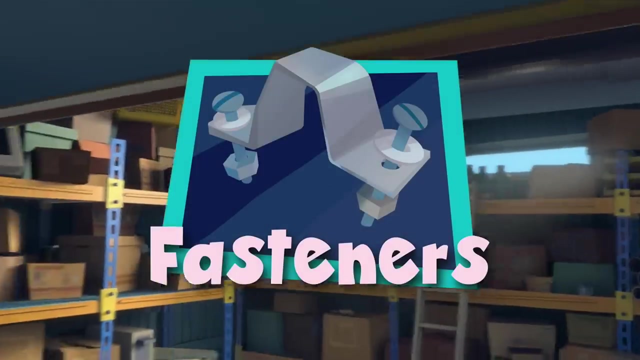 You see, Cool right, Wow, it's fantastic. So hang on. you guys tricked me, But you passed the test, right. Well, all right, Then I forgive you. Fasteners And of course all of the appliance's parts must be fastened good and tight. 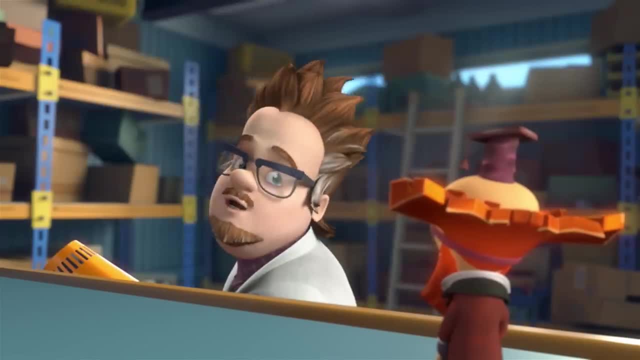 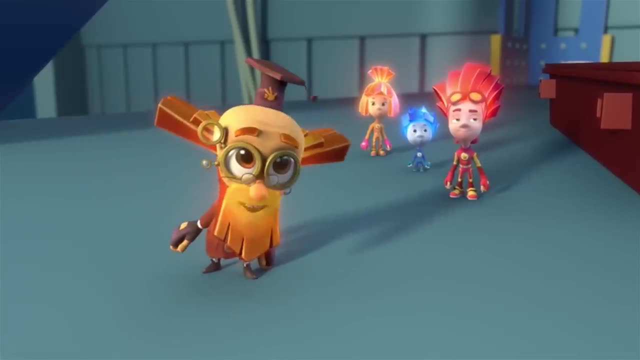 What are you doing, colleague? Today, Lisa is returning from her vacation And so I decided: before she gets back, I'll clean up the laboratory. Quite a noble initiative. Now where was I? You were saying all parts have to be fastened. 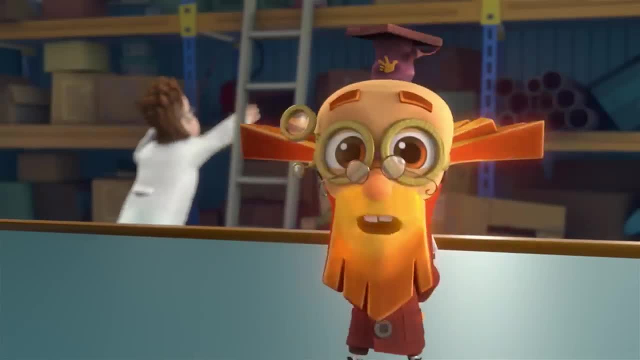 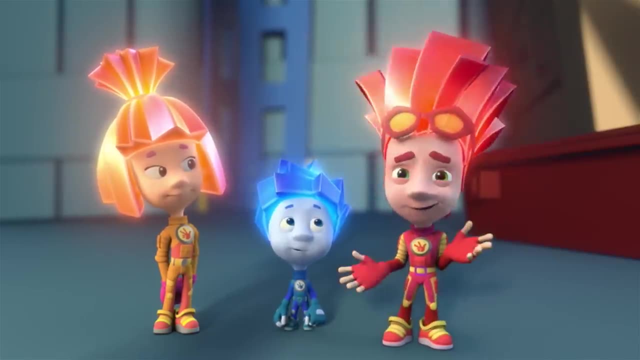 Heh, you're right. And what kinds of fasteners can you name Fire? Uh, a screw, Mm-hmm. And what else? Uh, another screw, Heh, that would make a total of two screws altogether. 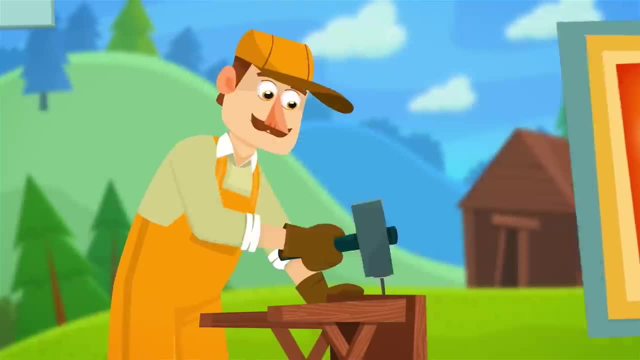 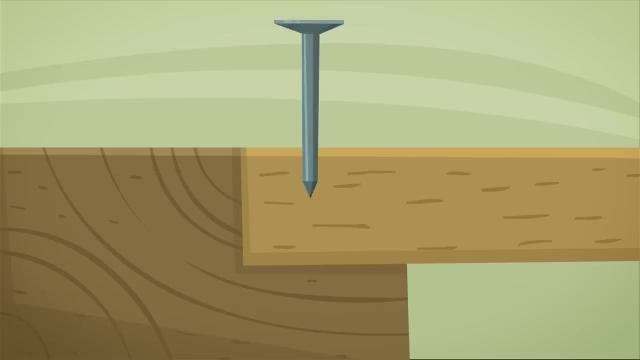 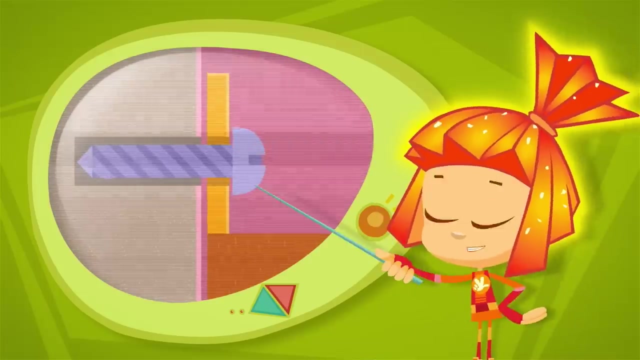 Simka. To fasten wood or plastic parts together you can use nails. Nails are hammered in with a hammer. In metal or stone you need to first drill holes for the screws. To help a screw hold better, it can be inserted into a special fastener called an anchor or wall plug. 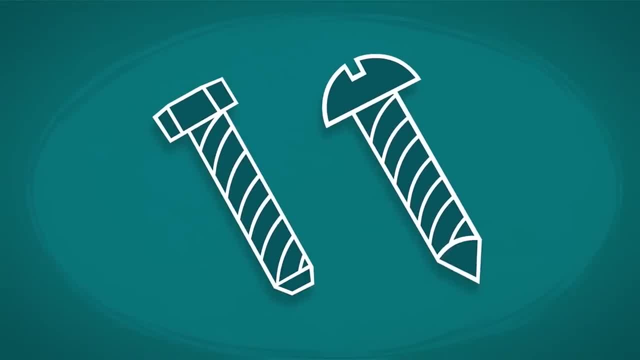 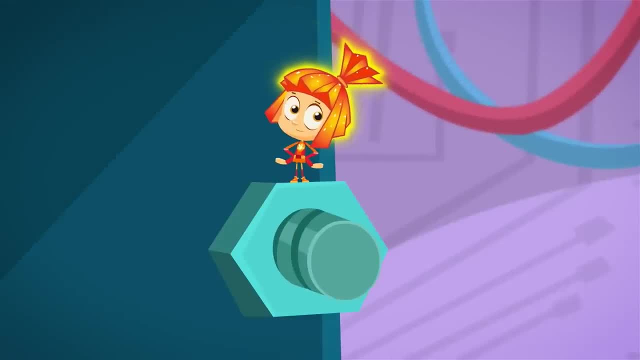 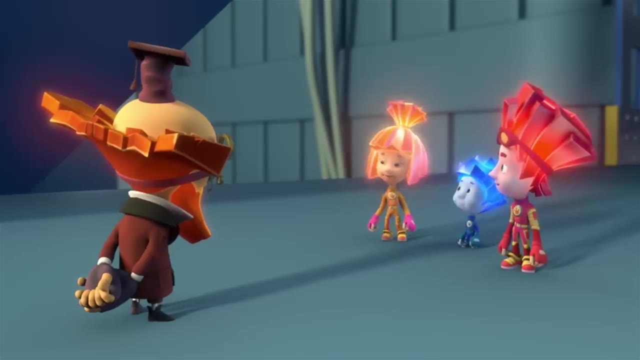 The difference between a machine screw and a wood screw is that wood screws have pointy ends. Machine screws go into holes that already have a thread, Or into a nut. And what if there aren't any screws or nails around? Well then a fixie can turn himself into a screw and screw himself in. 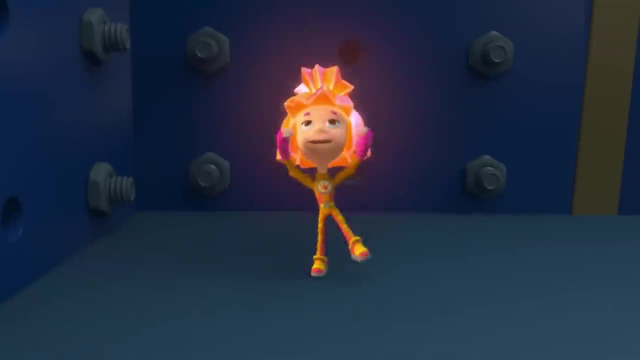 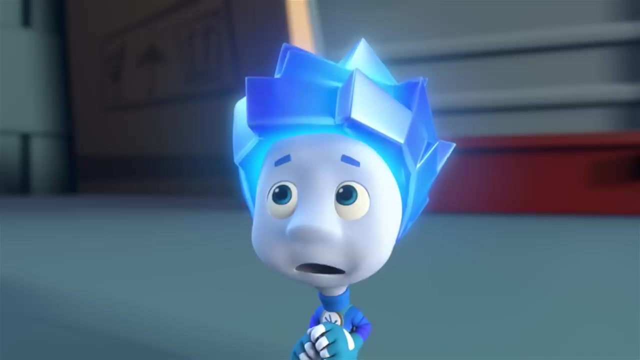 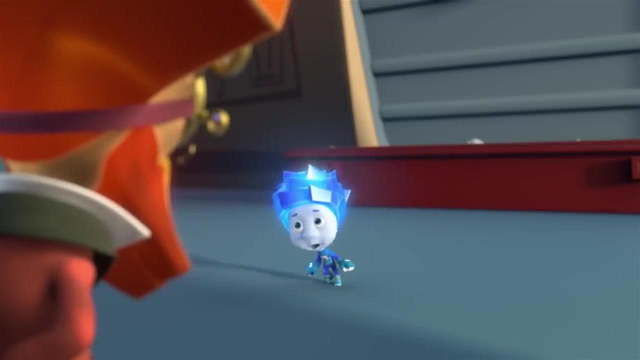 Like this Masterfully done Fire, think you can do it? Of course, Yeah, Nolik, Is it okay if I won't go? What do you mean? you won't go? Wait, I started on the wrong foot. 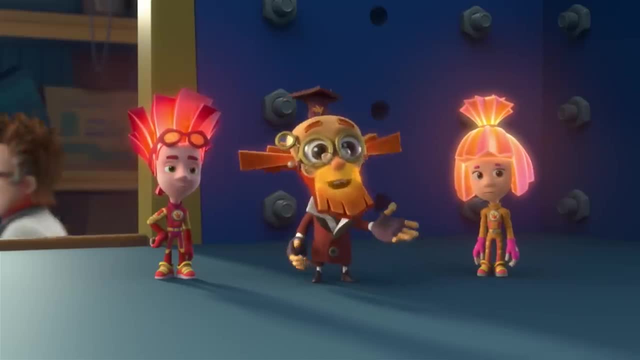 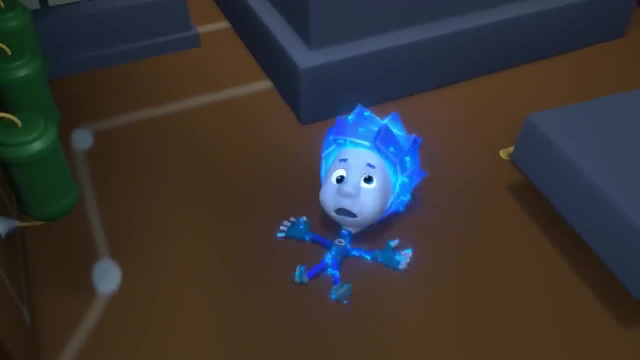 Uh, no, I guess it was the right one. Don't be scared. You've done this a thousand times. Uh-huh, You're right, You had to make sure the appliance was turned off first. Yeah, I should have. 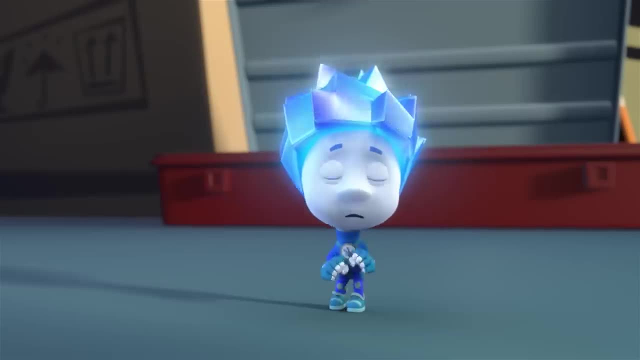 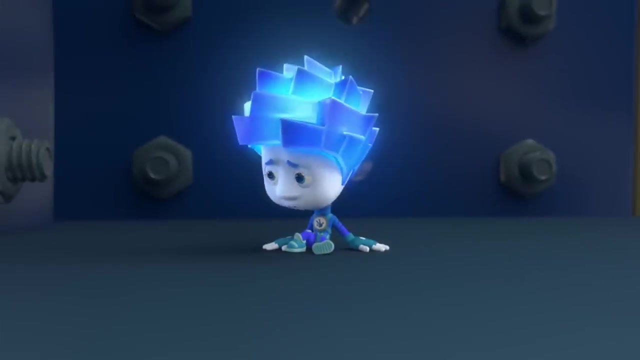 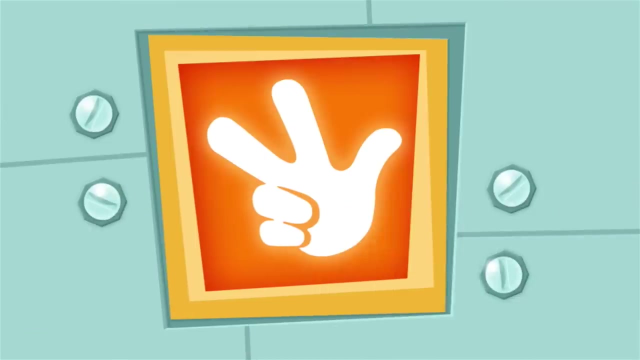 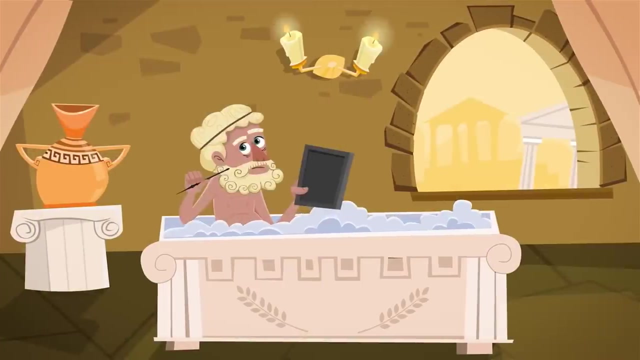 This time it's not going to happen to you, It's all under control. Go on, I'm still scared to do it. How about you try again? And who came up with this dumb screw idea? According to legend, the screw was invented in ancient times by the great Archimedes. 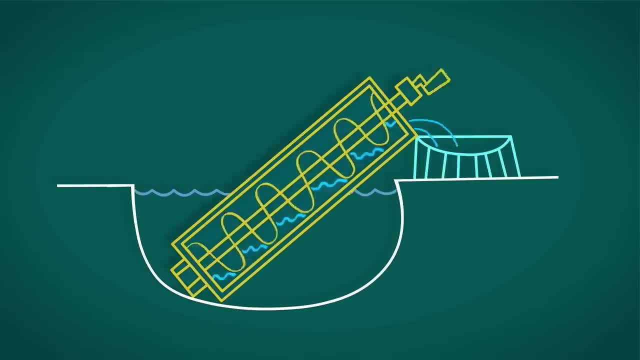 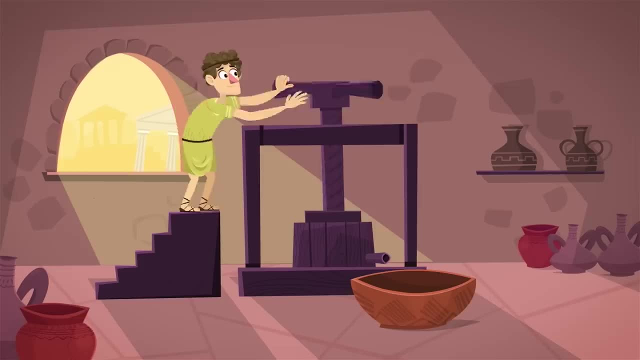 Using his screw-type mechanism, Archimedes built a special machine for getting water out of a canal. In ancient Rome, people used wooden screws and presses to squeeze the olive oil out of olives. Screws were also used as parts of drills or as lifting jacks. 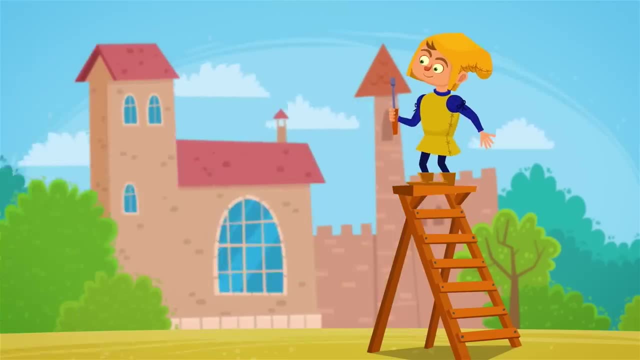 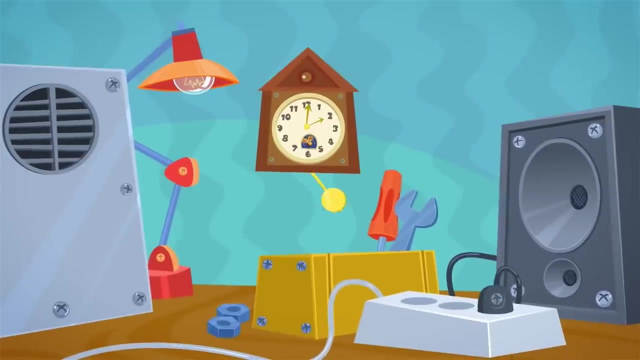 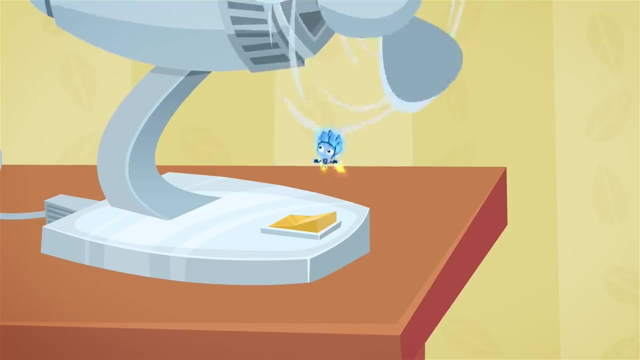 But the use of screws as fasteners did not begin until the 15th century. Soon thereafter, screws became so popular that today it's almost impossible to find an appliance made without one. And if one of these little screws should fall out, we Fixies will come to the rescue. 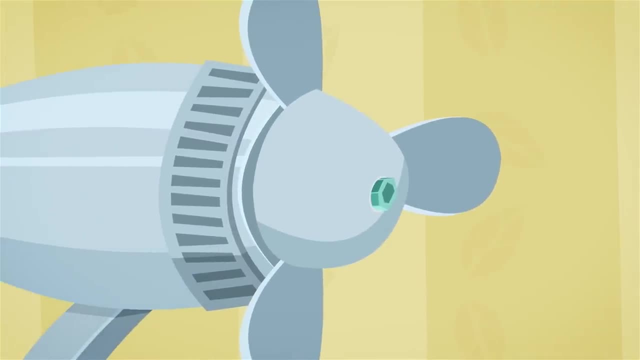 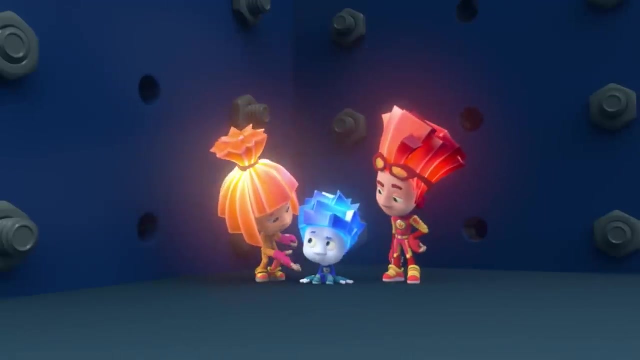 Because we don't just turn into screws. when we need to hide from humans, We're always ready to do it when help is needed. Nolik, let's try it together. Don't be scared, We're here with you, Ready. 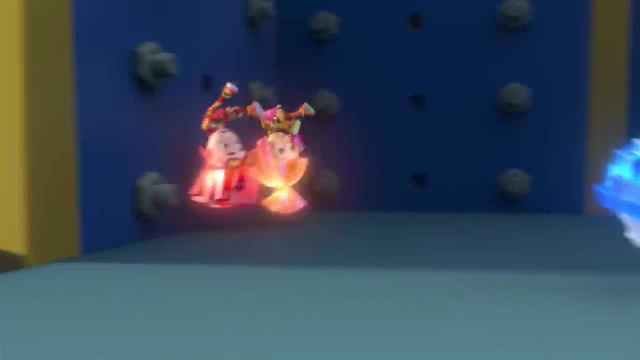 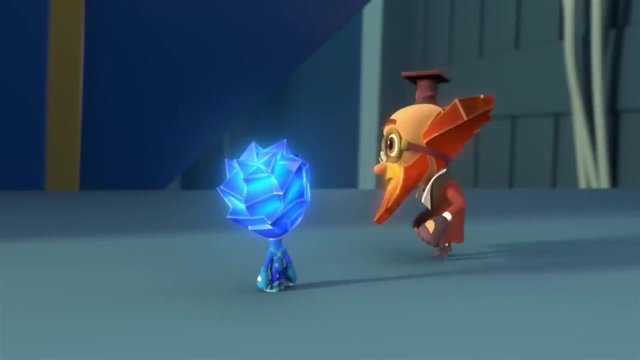 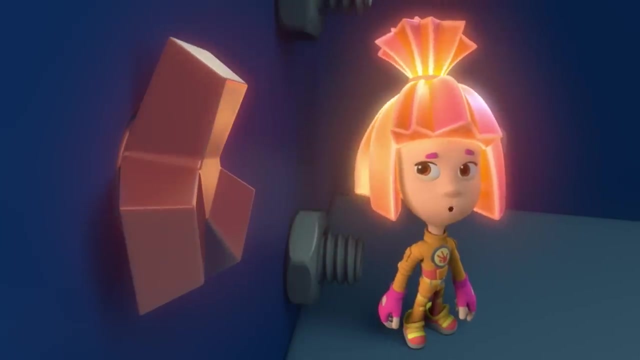 And Go, Nolik, watch me, son. I haven't screwed myself in in over a hundred years, but I'm not scared. Did you see that? It's a piece of cake, Grampus. I'm stuck, It's all my fault. 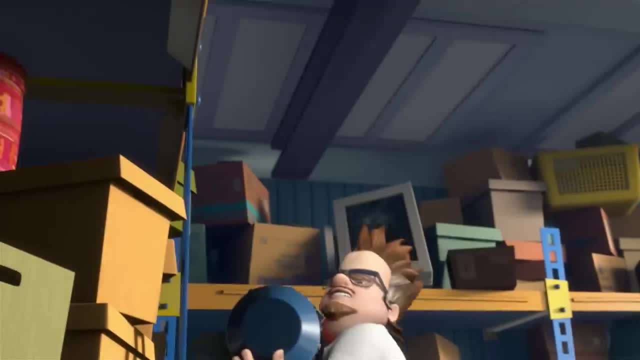 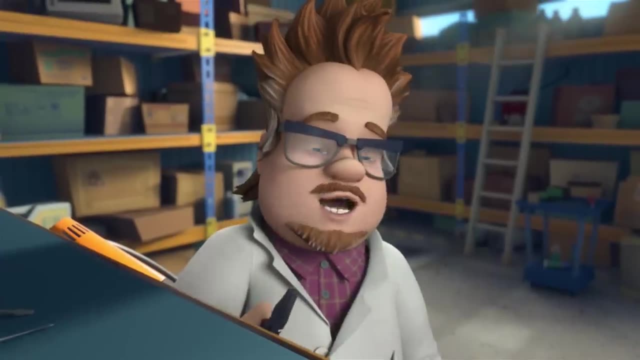 There's no need to worry. Professor Eugenius, can you help us unscrew Grampus? I'll be right with you. It It's got a bit rusty. It's probably old age. I know what will help: A drop of oil. 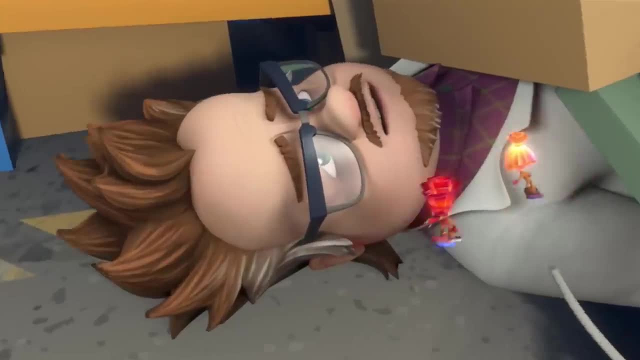 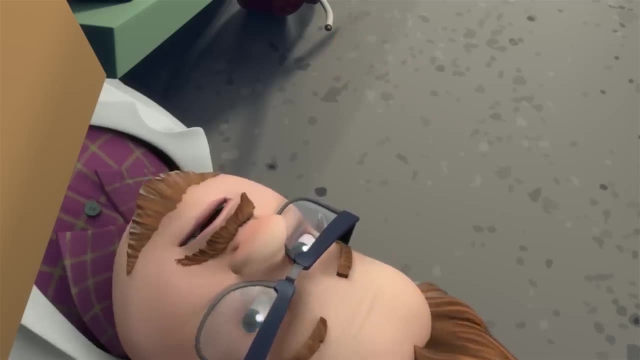 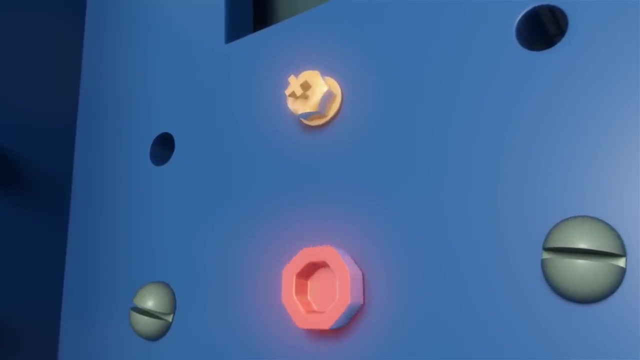 Ow, Professor Eugenius, are you okay? I'm okay. Thank you for asking. Look out, It's going to fall. We need to fasten the shelf to the wall. Nolik help, We can't do this without you. 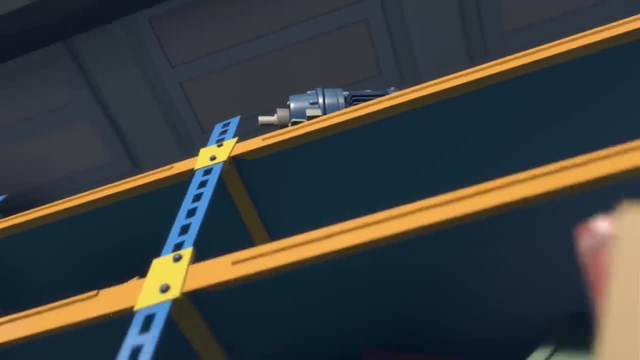 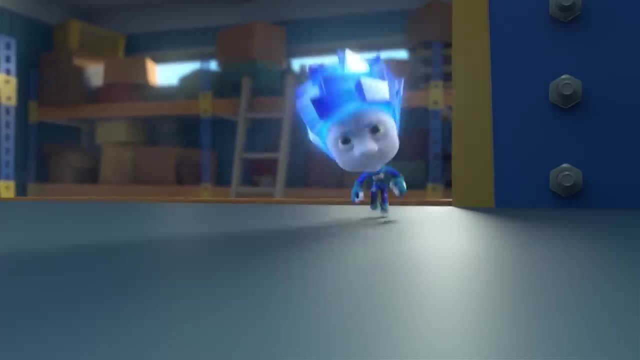 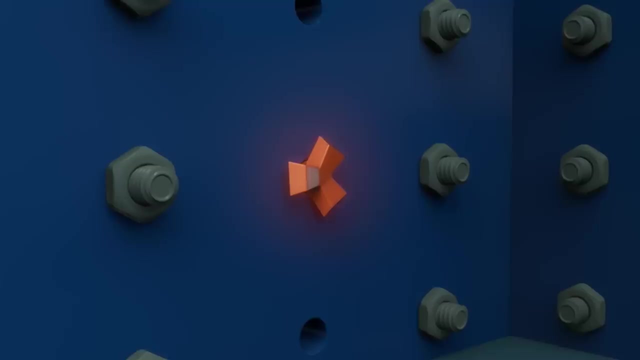 Simka, I'm scared too. Nolik, save me. What's going on out there? No big deal, colleague, I just got a little bit buried. Will anyone unscrew me? I wish I could, And we're holding up the shelves. 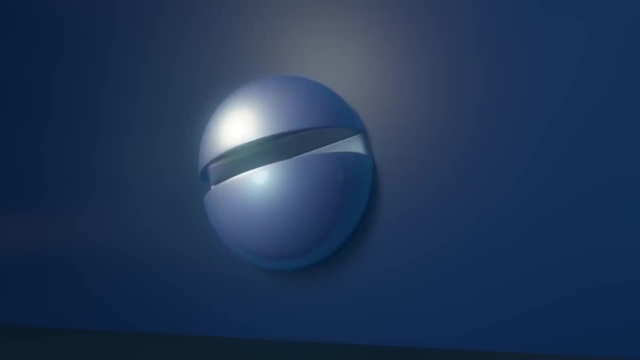 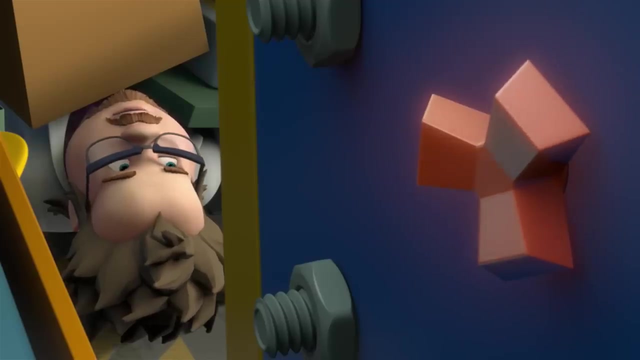 And Nolik, Me too. I did it, I screwed myself in. Well done, Nolik, I knew you could. And who's going to help us now? Elisa will get here shortly. All right, We'll wait for Elisa. 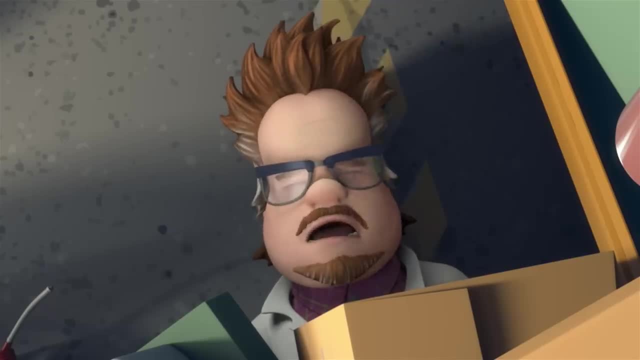 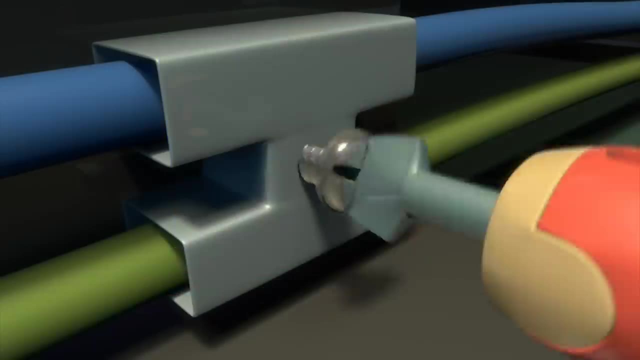 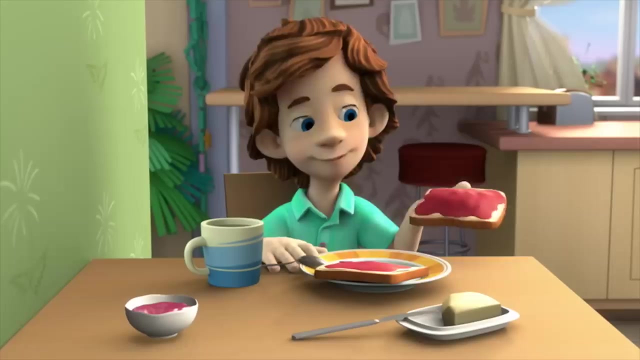 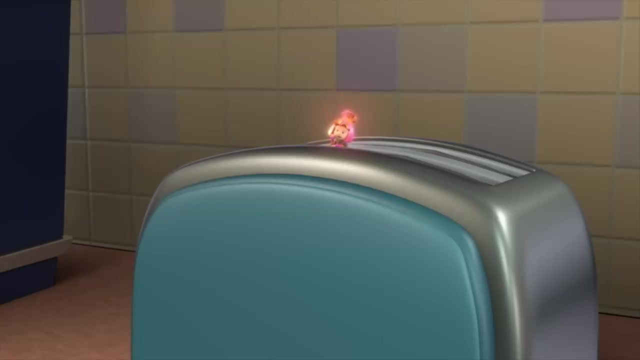 Yeah, just as long as her return flight isn't delayed. The Coffee Maker, Tideesh, Hi there. Tom Thomas, Are you ready for school? Uh-huh, And you, I'm helping Masiya today for school. Three more patients. 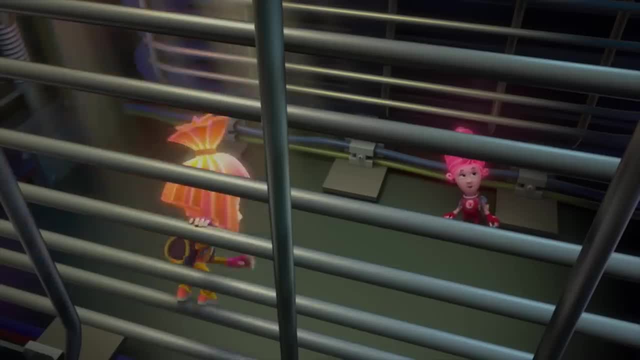 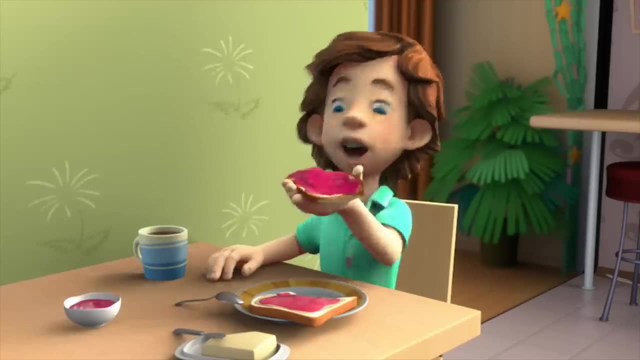 How in the world can I do it all? I have that new equipment being delivered and I'm leading this week's case presentations. Oh well, somehow I'll have to figure out how to do it. Um, Good morning, Yeah, just great, huh. 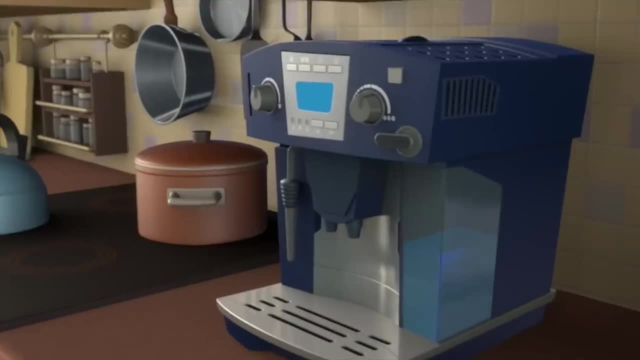 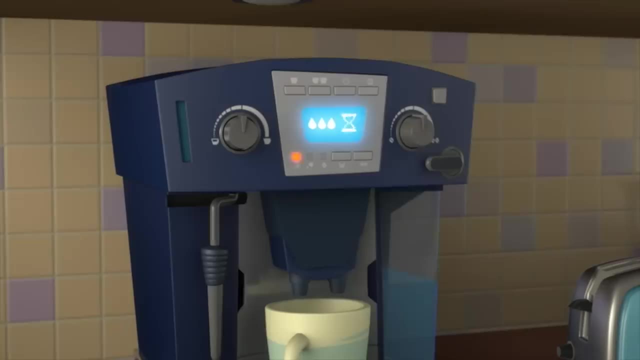 I got work piled up to the ceiling. Okay, a cup of coffee is the only thing that can save me today. Now what The last thing I need is to be late. The Coffee Maker started its cleaning cycle. She'll have to wait. 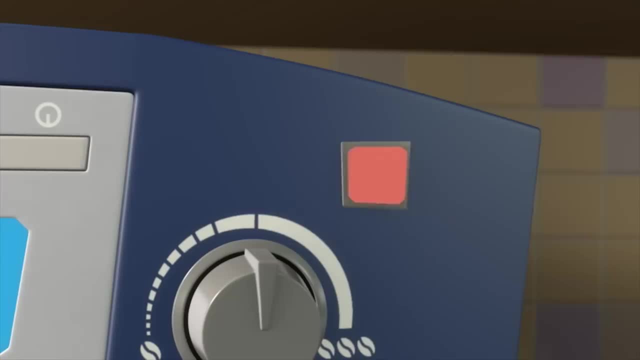 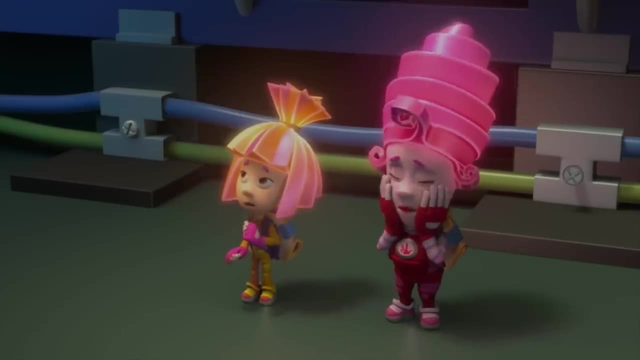 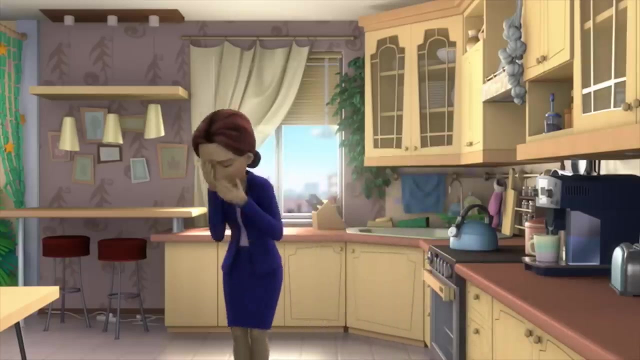 What's the problem? Why don't you work? Are you going to work or what? Oh, the poor Coffee Maker, Tom Thomas' poor mother. That's enough Work already. What is going on today? Hey Mom, come on. 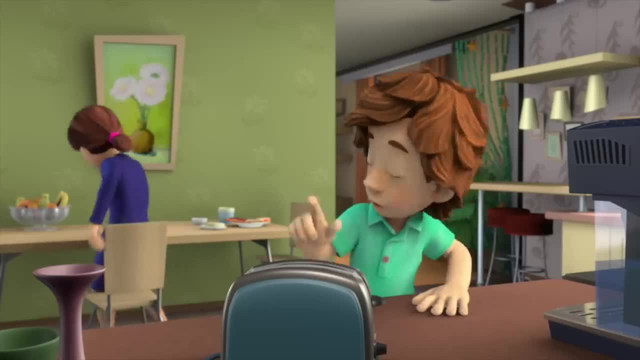 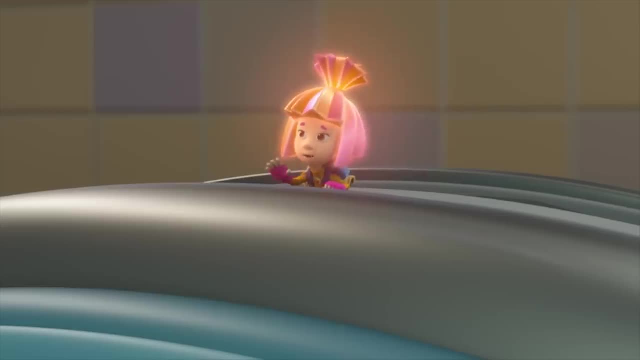 Let me give it a try. I can't take any more of this. We've got to help her. I really hope nothing broke in there. Don't worry, we'll get it working. Just distract your mom, Mom. and what if the Coffee Maker just started working again right now? Would that save your day? you think, Mm-hmm. Early Coffee Makers would do nothing more than heat up the water and force it through the ground coffee. Today's generation of devices are often called coffee machines. They can do so much more, and even remove the mineral deposits themselves. 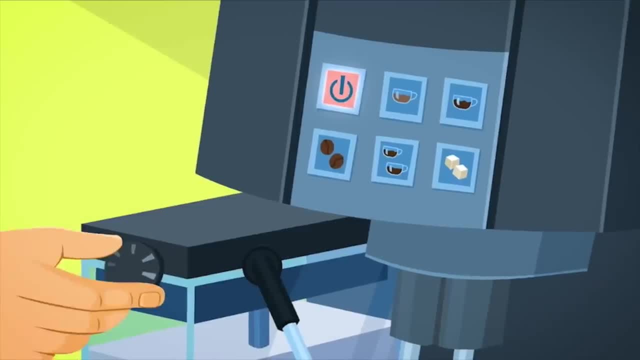 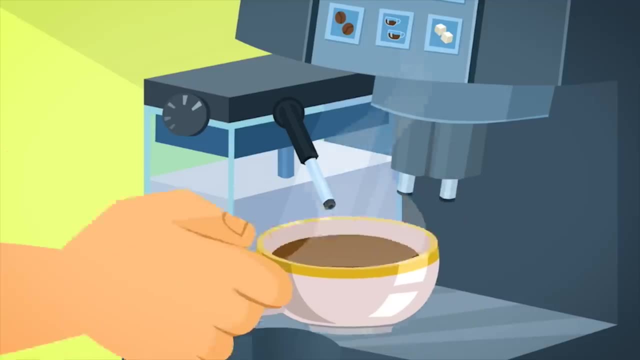 These machines can make your coffee any strength and add milk and sugar if that's how you like it. And most conveniently, they can grind the coffee beans right before brewing. Just press the button and the fresh cup of coffee is ready. And that aroma. The main thing with any coffee maker is to be nice to it. Then you just give it some time and it starts working by itself. That is just absurd. Restarting it is the first step. Simka, get over there and open and close that contact. 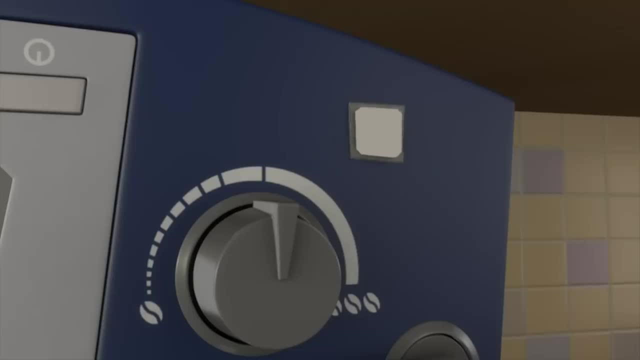 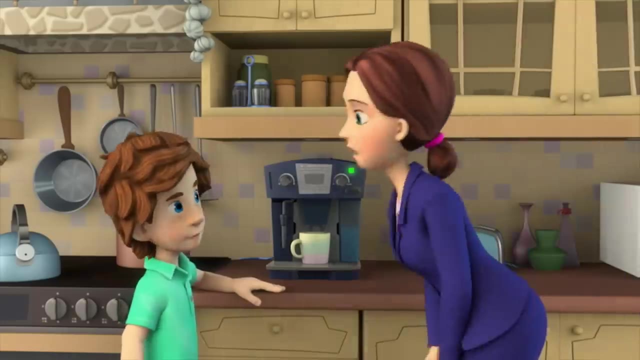 Mm-hmm, You see, That's what I was talking about. A coffee maker isn't alive, it's a machine, that's all. Then how come you hit it like you did? Hmm, But if you're really nice to it and you pet it…. 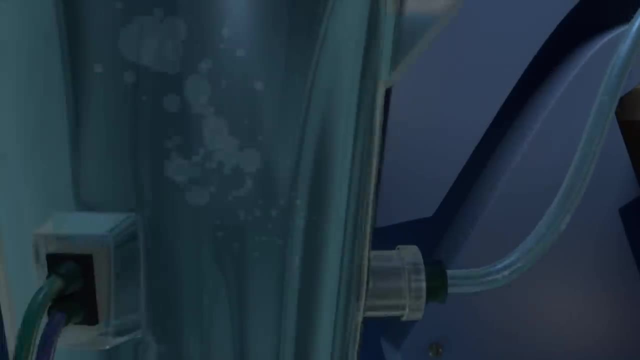 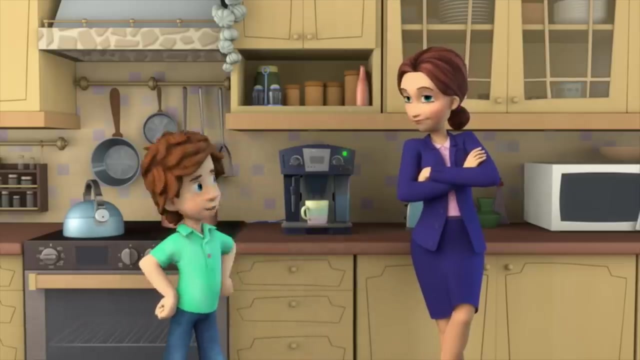 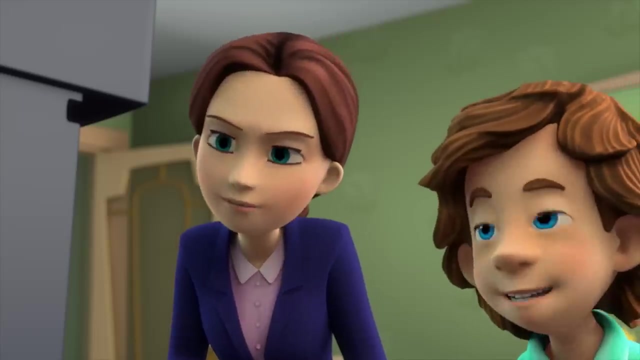 Then she'll purr. Hear that It liked that a lot. Coffee Maker. blink to us when you're ready to start working, Turn on the display. Mm-hmm, See that It answered us. It behaves like it's really alive. 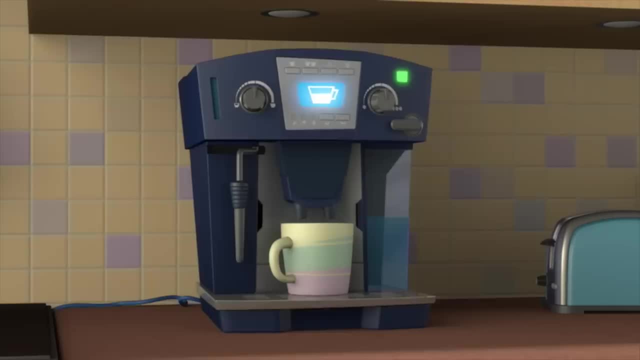 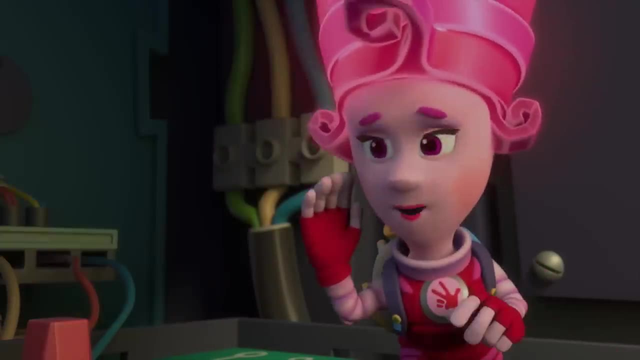 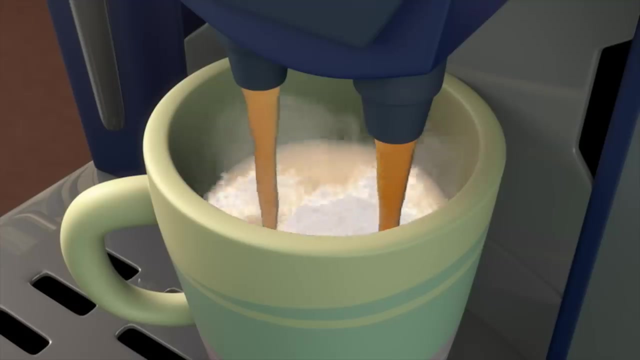 Well, Coffee Maker, make coffee. It's impossible. Tideesh Time for a little surprise. Just don't give up our secret. You fixed it somehow. What's your secret? It's simple: If you handle appliances with care, then they'll take care of you. 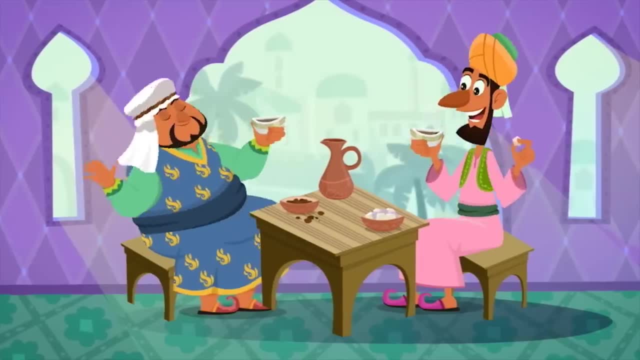 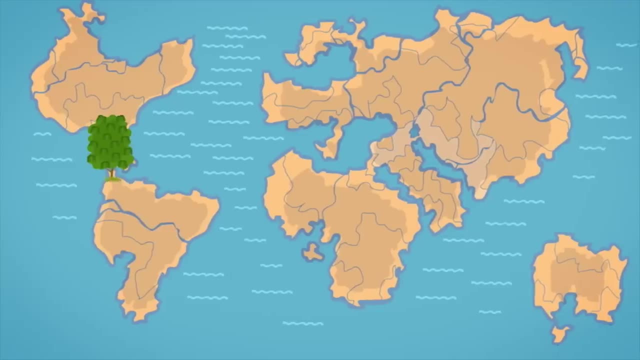 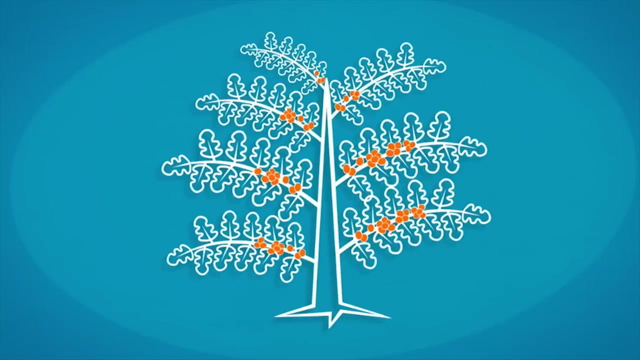 The magic taste of coffee was first appreciated in Arabia, And that's why the most well-known variety of coffee is called Arabica. Coffee trees grow throughout the world. in mountain regions where the weather is warm and humid, The branches of coffee trees get covered with coffee berries. 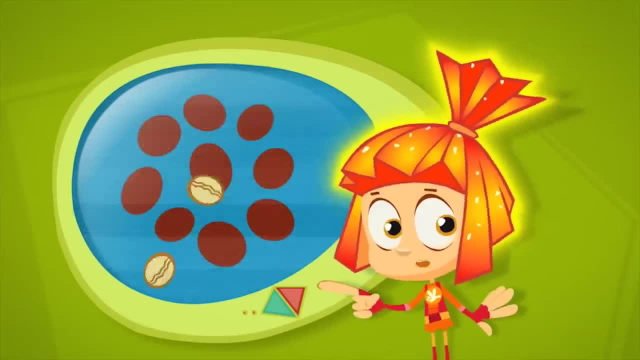 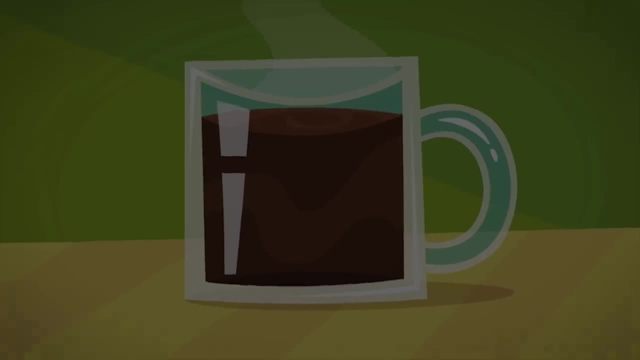 But to make the coffee drink we don't need the berries, just the seeds inside. After the coffee beans are roasted and then ground, hot water is added. Different cultures serve coffee differently. Some serve it hot, some cold, With sugar, with milk, with ice cream. 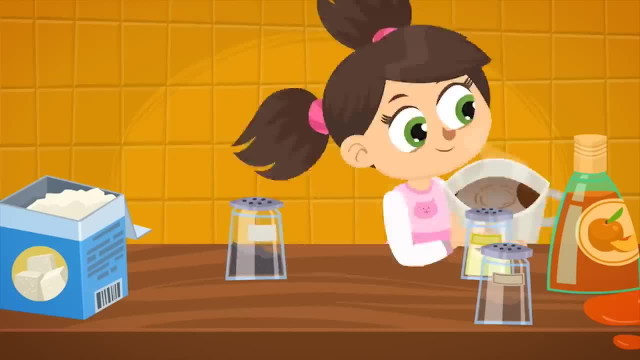 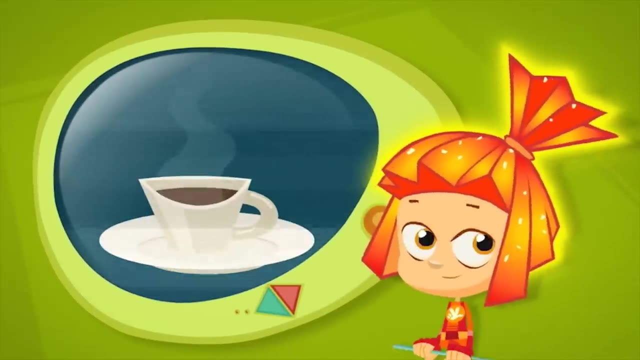 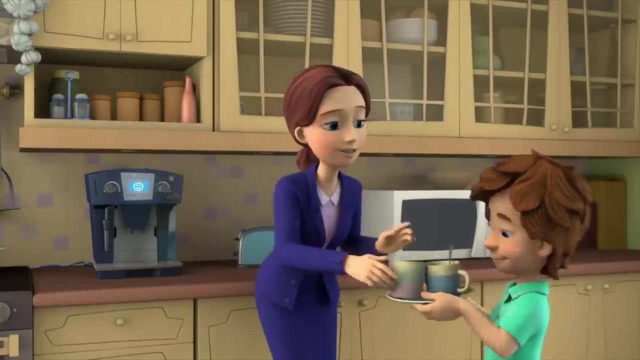 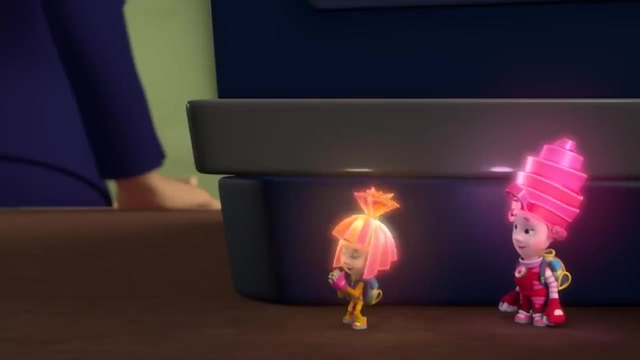 with cinnamon, with ginger and even with salt and pepper. They say that coffee gives people energy and helps them from feeling tired, But it's important not to drink too much. Tom Thomas, you're a powerful wizard. She believes it. It's remarkable. 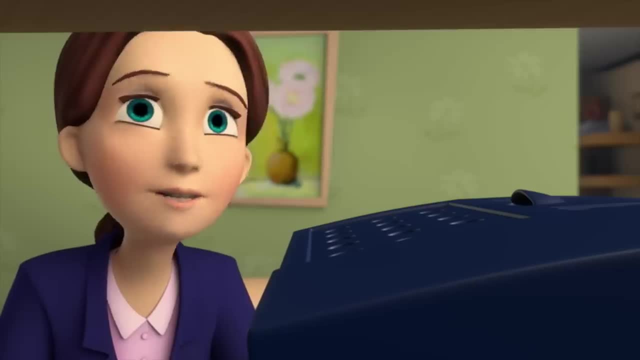 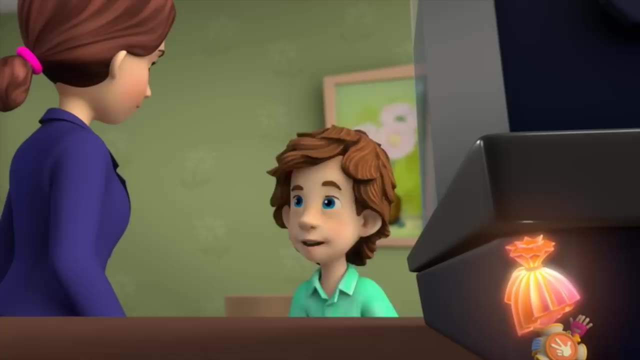 I can't believe an ordinary coffee maker can be so emotional. Poor thing, Forgive me, huh. And that's not all. If you take care of your coffee maker and you're nice to it, it can even. it can even sing a song. 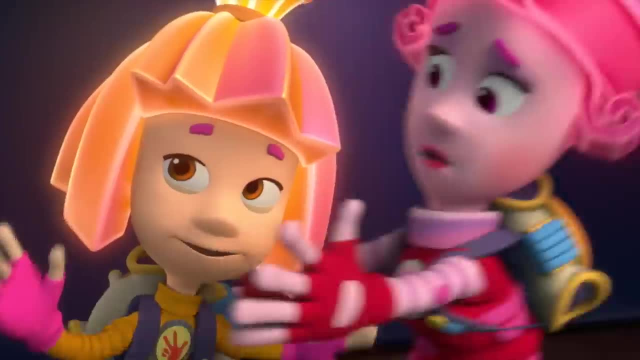 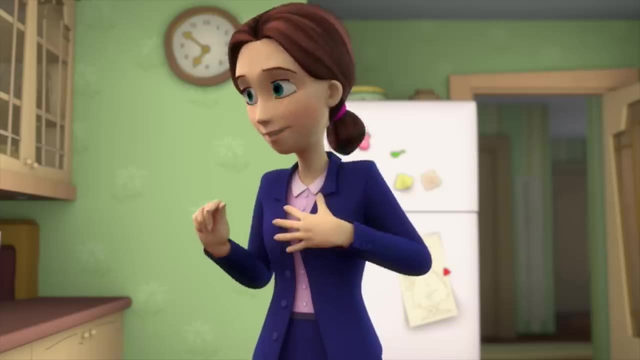 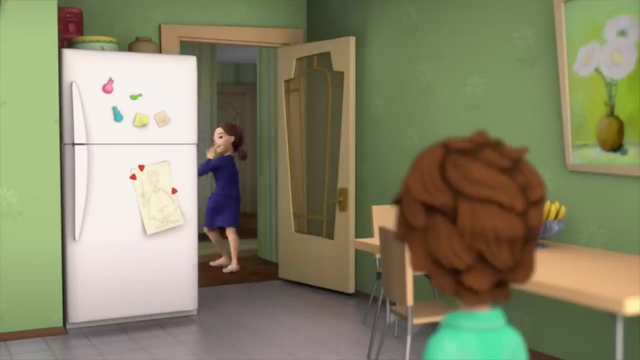 Oh, my dear Augustine, Augustine, Augustine, I've got to be hearing things. You've got me under your spell. Tom Thomas, Time to go, Augustine. Oh my dear Augustine, Augustine, Why did you start singing? Sorry, I got carried away. 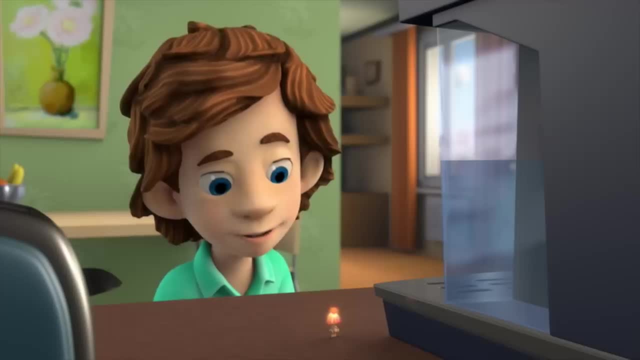 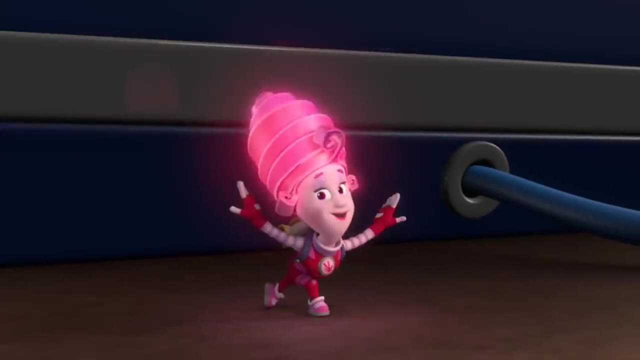 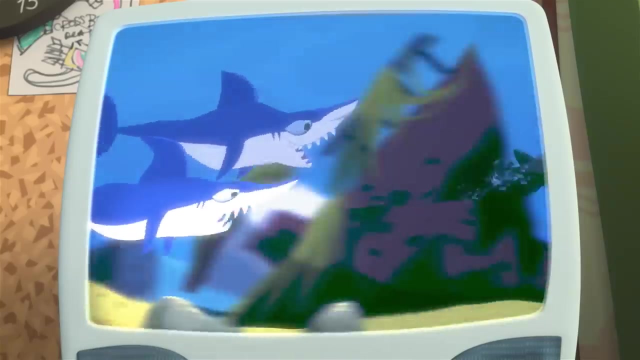 And I got carried away. Sing me that song again, will you? Oh, my dear Augustine, Augustine, Augustine, Oh my dear Augustine, everything's gone. The Submarine And the submarine disappeared into the ocean deep, leaving the vicious sharks high and dry. 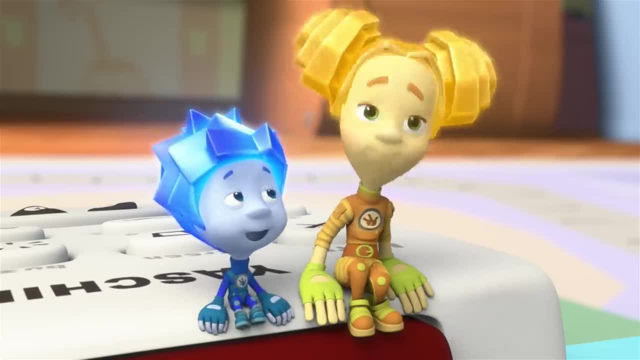 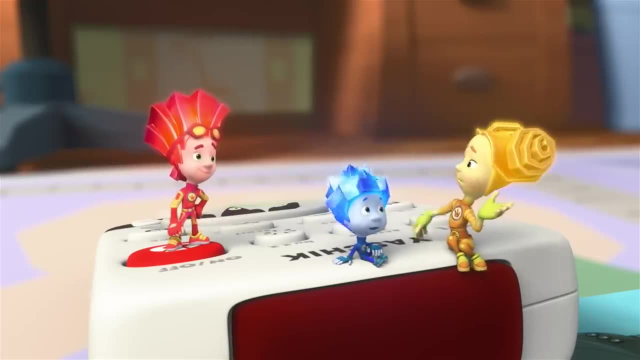 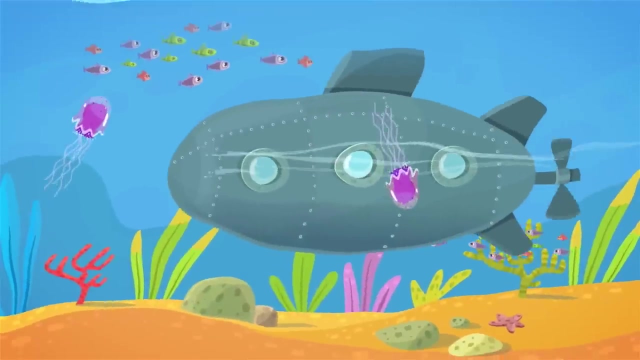 That cartoon was super Class Splendid. I wish we had a submarine too. What do you say? we make one, But we don't know anything about building a submarine. What makes you say that The most important thing for a submarine is to be airtight? 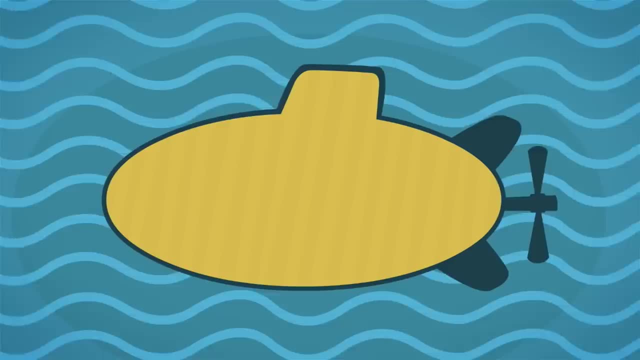 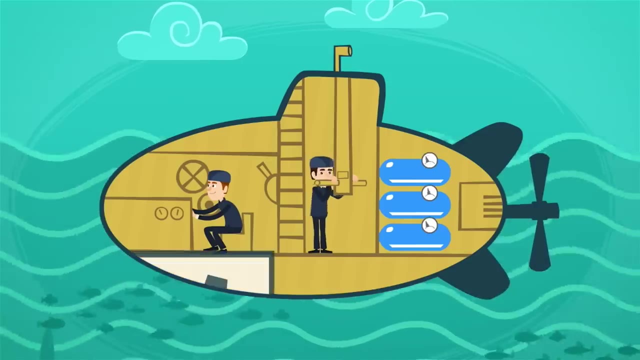 so that it's impossible for water to leak in from outside And inside. there needs to be a reserve of air for breathing. For a submarine to go underwater, it uses special containers. When the containers are filled with water, the submarine becomes heavy and starts submerging. 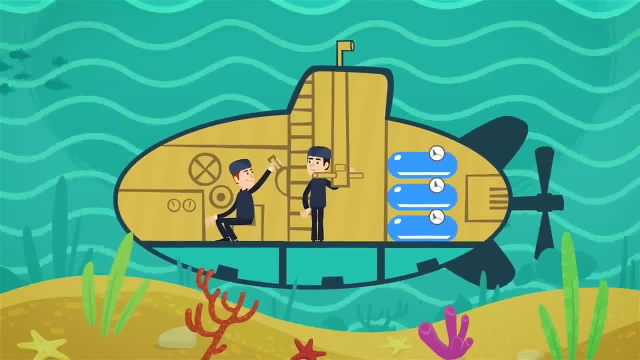 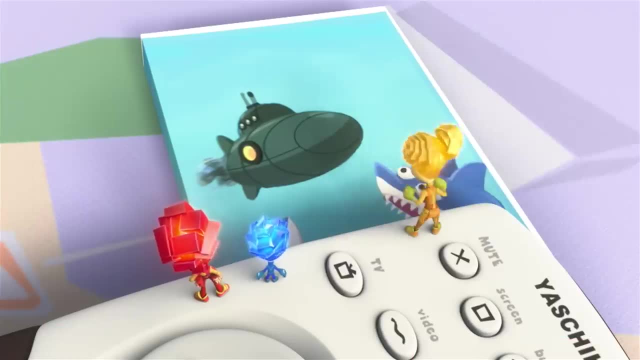 When it's time to take the submarine back up to the surface, the water in the containers is switched back for air and the light submarine clings. And what are we going to make it out of, Out of uh broken toys? 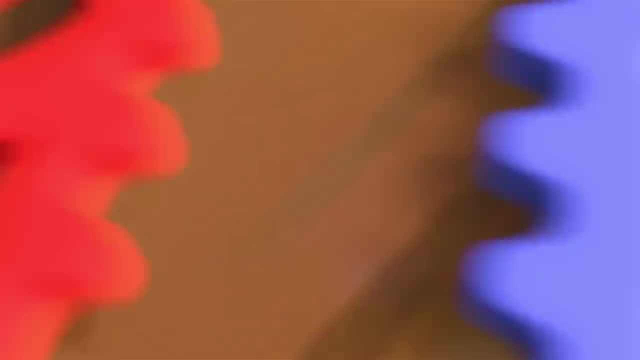 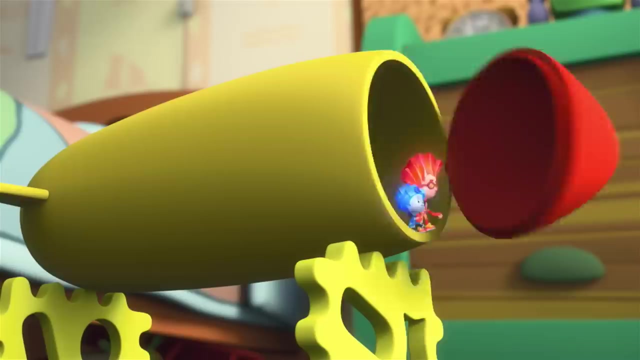 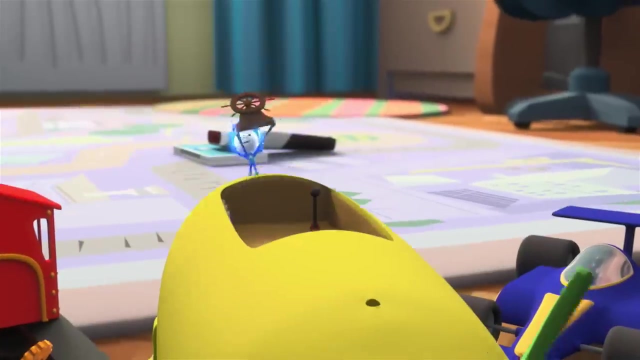 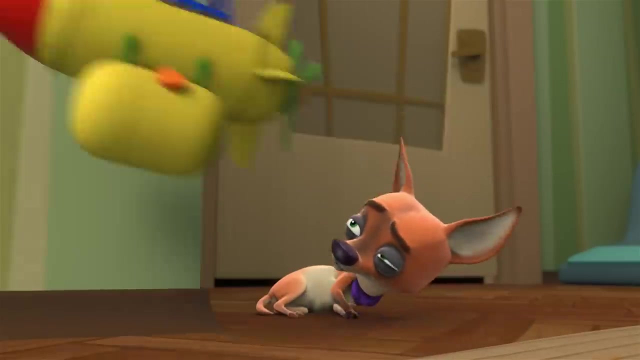 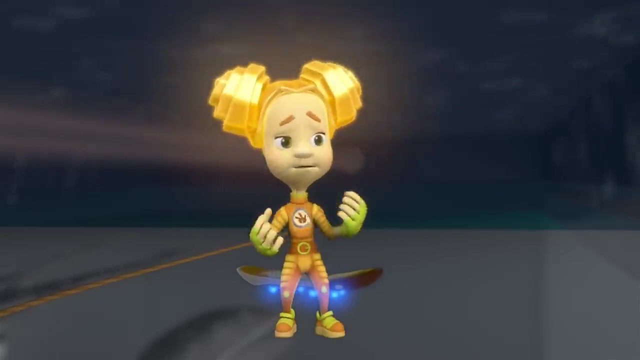 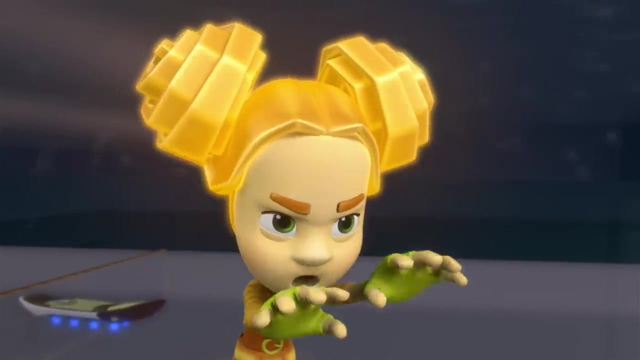 And where are we going to sail her? In the aquarium. Mm-mmm. Tola, aren't you going with us? I'm afraid to. How come? What if water fills up the submarine and then we drown or those huge fish gobble us up? 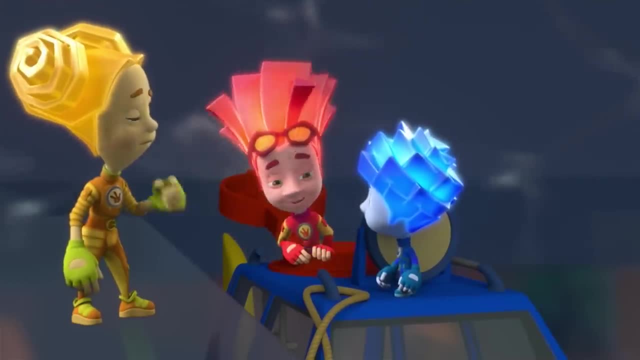 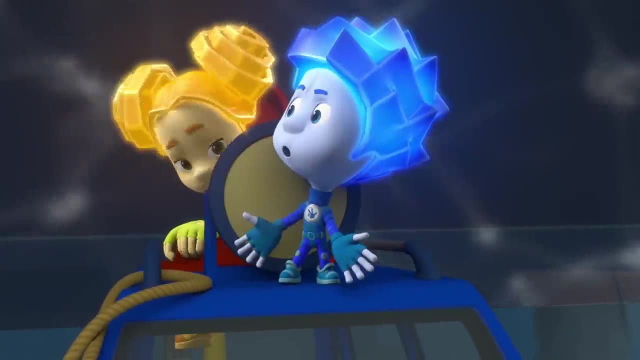 Come on, Toola, That's silly, Nolik's little and he's not scared of this. Yeah Well, all right, Cast off the lines. The who Unhook the rope. it means, Ah, You should have just said that. 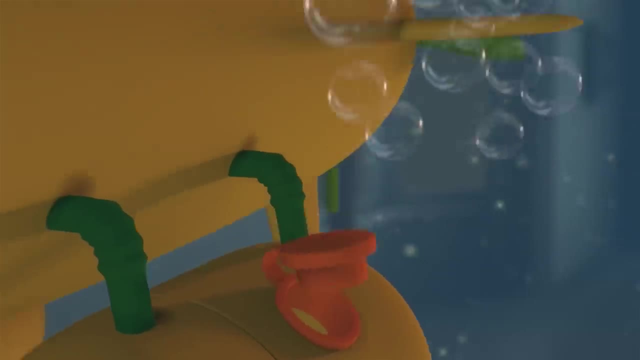 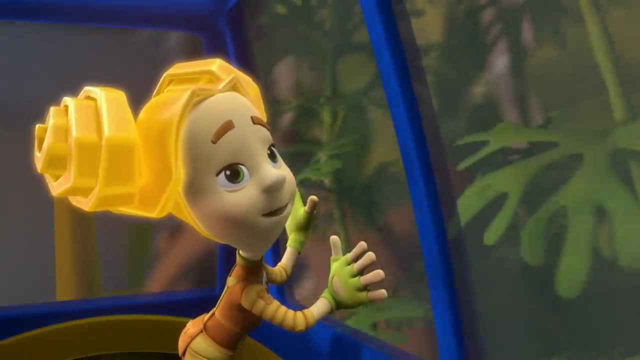 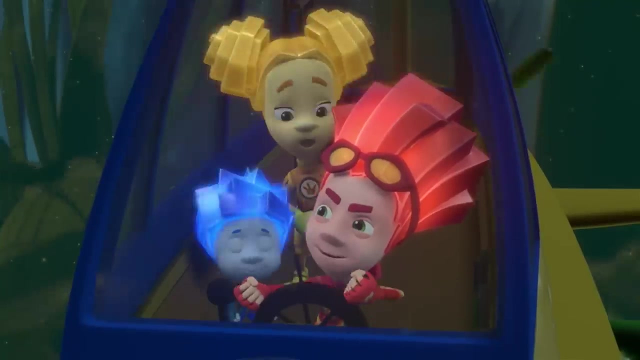 Are you ready? Time to take her down? Hooray, We're sailing. It's just beautiful in here. There they are, The fish and sharks. Time to scare them Turning right. Go after that one. You can't escape from us. 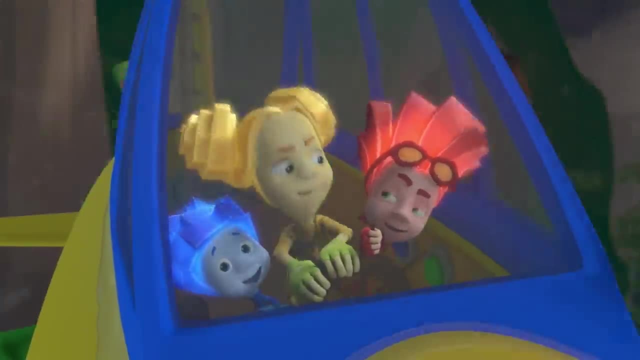 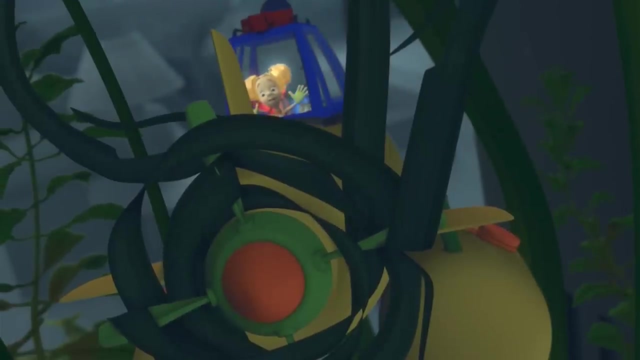 Please stop it. Come on, come on, come on, Stop torturing the fish. It's terrible. What, Oh no, I don't know. There's algae wrapped around the propeller. I want my mom to see us. 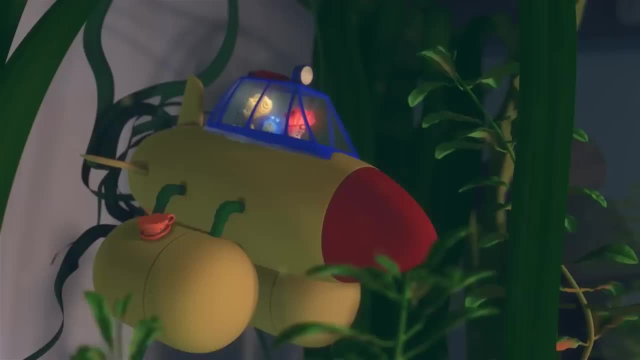 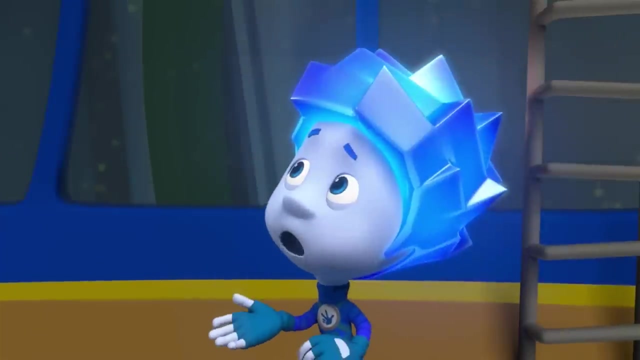 Just be calm, There's no need to panic. Let's try taking her up. It's not working, Of course. No wonder I was scared. And so what do we do now? How about we open the hatch door? No, we can't. 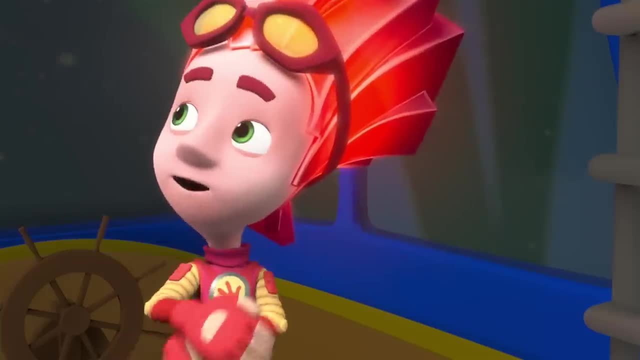 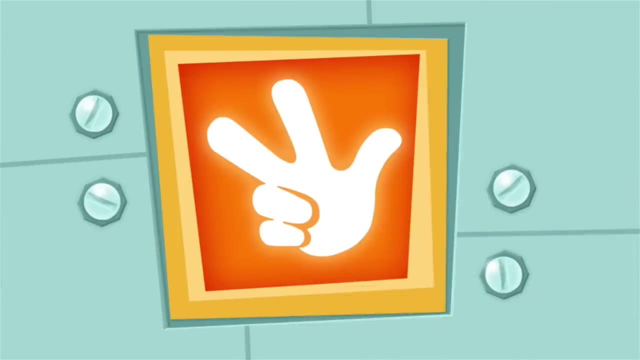 The water would pour into here and then we would all drown. Well, in that case I don't know. I need to come up with a plan. Yeah, The world's first practical submarine was built almost 400 years ago in England. 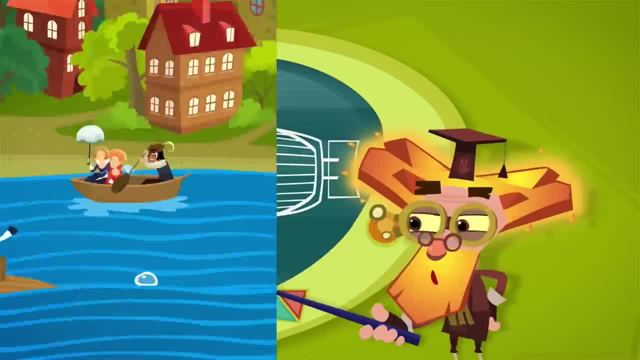 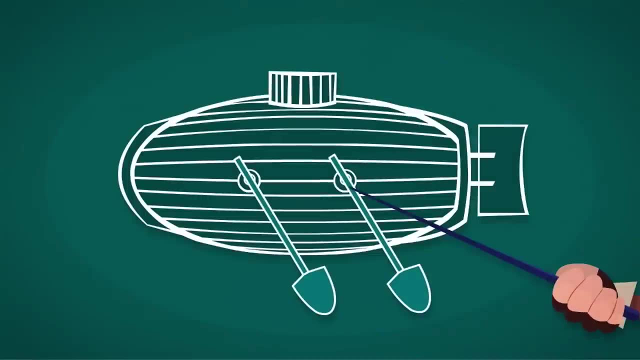 It was made out of wood and couldn't dive very deep at all. Inside the vessel, rowers sat with oars, So it couldn't move very quickly either. About 200 years later, the oars were replaced with a propeller. 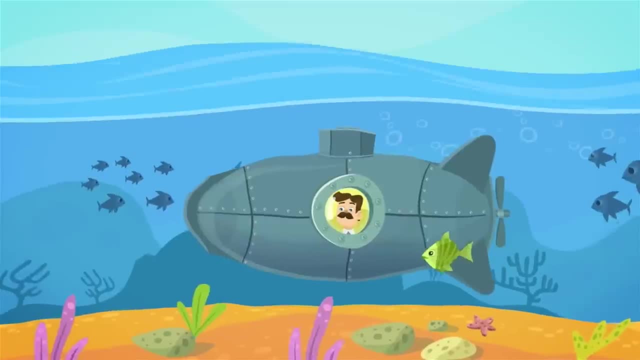 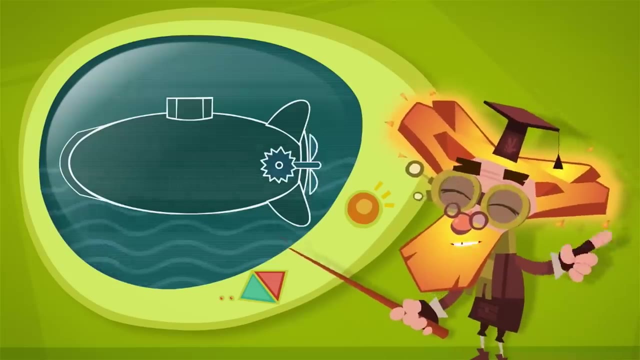 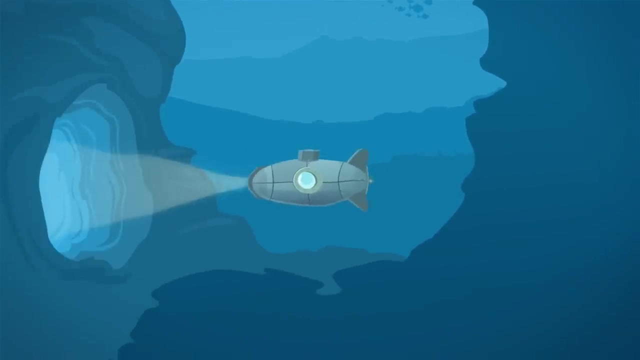 But the propeller on that submarine could only be turned by hand, making it a slow submarine as well. Any good swimmer could easily outrace it. It was only with the appearance of electric motors that submarines started submerging to great depths and moving through the water at very high speeds. 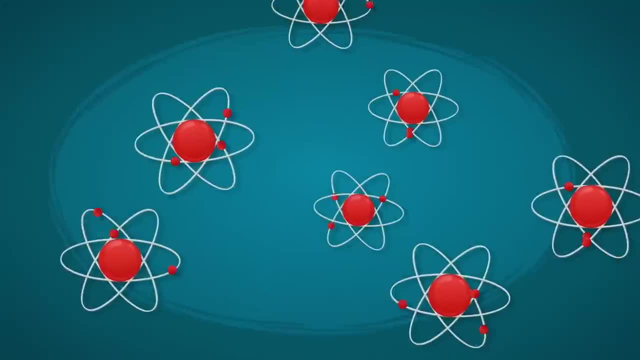 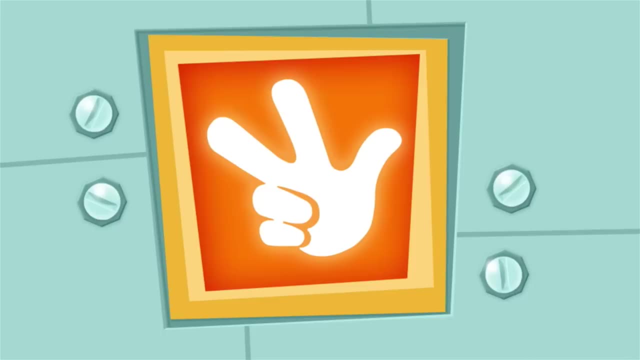 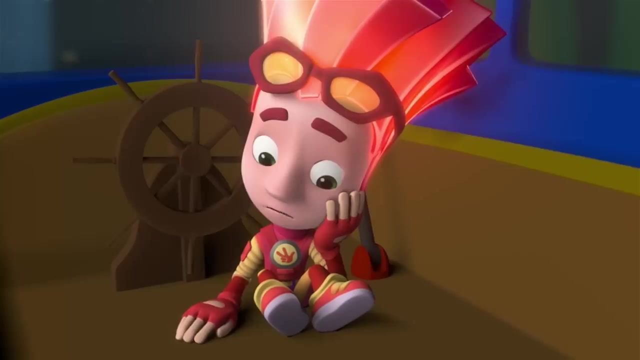 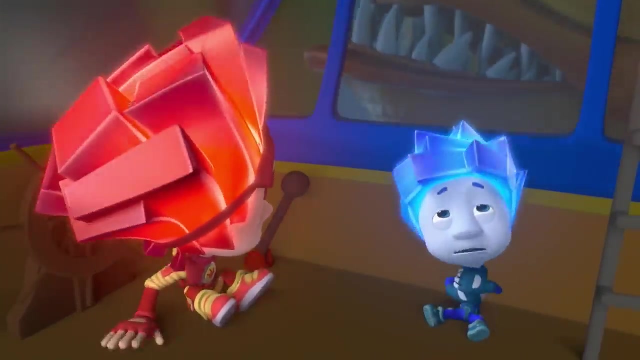 Today's modern military submarines use nuclear reactors for power. These submarines can stay underwater for months without resurfacing Fire. can you come up with your plan quicker, Because we're running out of air Fire, we're going to suffocate. 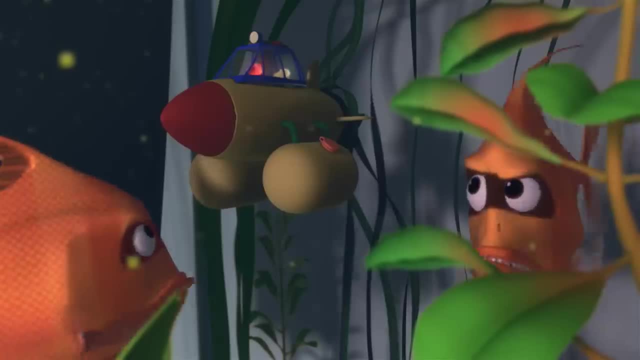 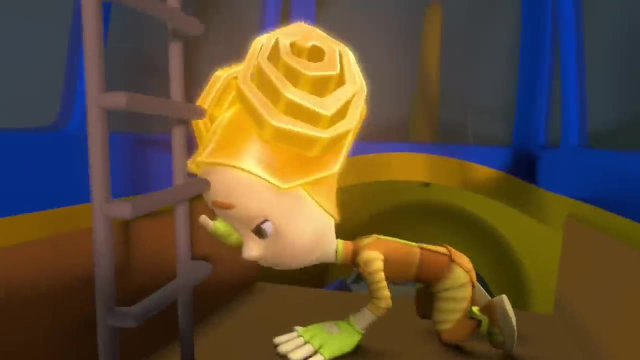 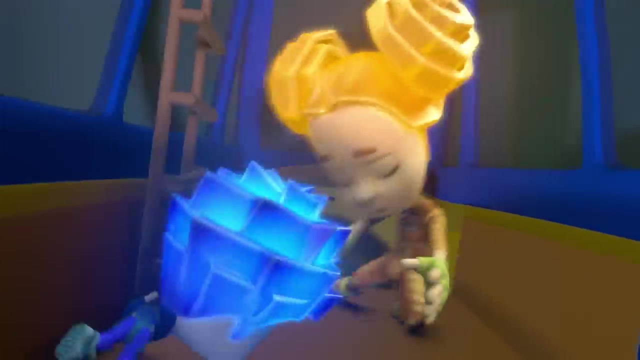 No, we won't mate. The chances are better, the fish will eat us. You never should have teased them. Yeah, we're in trouble. Didn't I warn you, didn't I? And you wouldn't listen? You did everything, just the opposite. 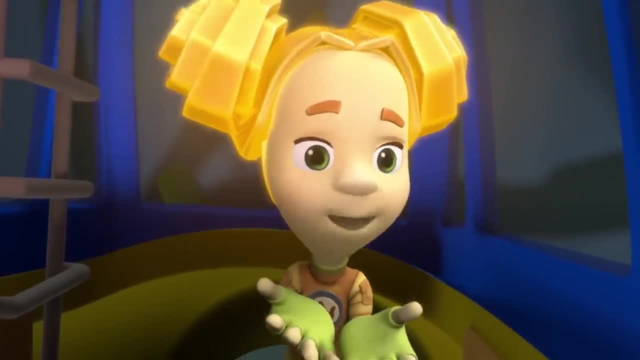 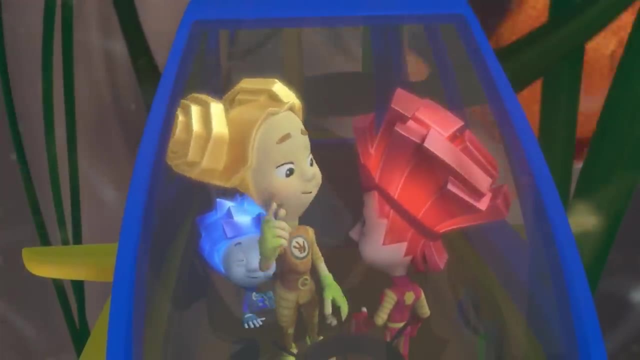 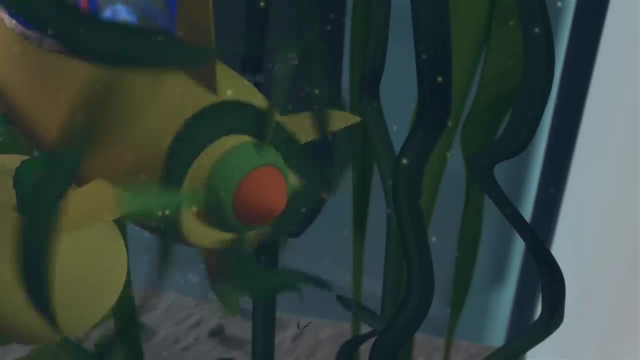 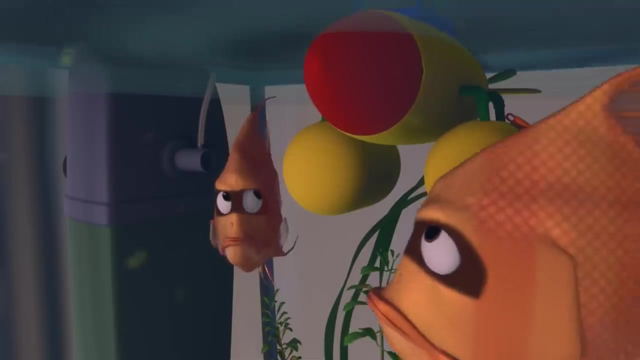 Wait, it might work. Let's rewire the battery the opposite way. We should switch the plus and minus. How come? Because then the motor will start to turn the other way, forcing the algae to unwind. That's what we call a. 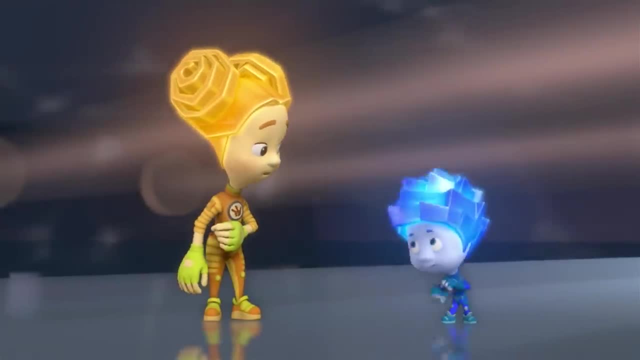 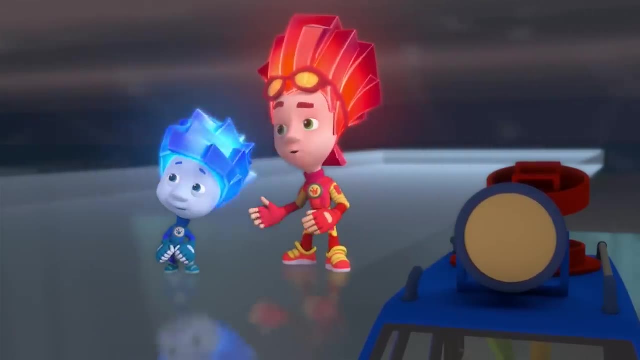 We won't bother you anymore. all right, Peace. Thank you so much, Toola. You really saved us. It's just because I was the one that was most frightened? No, it's because, when things got really scary, you kept your cool about you. 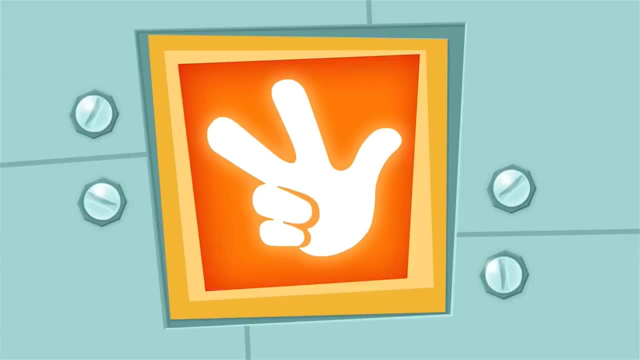 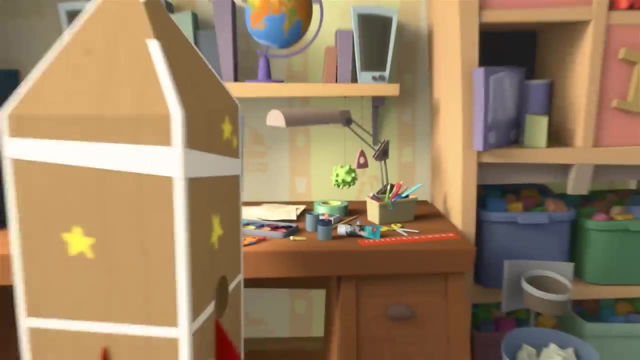 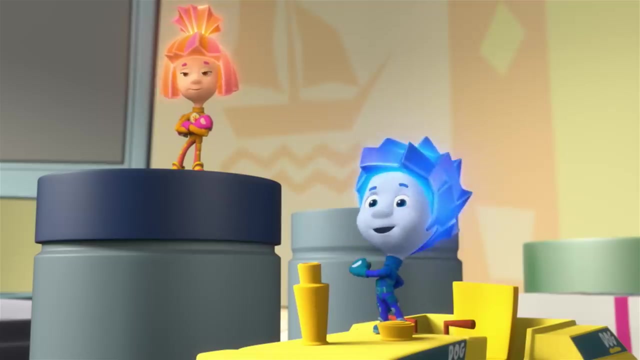 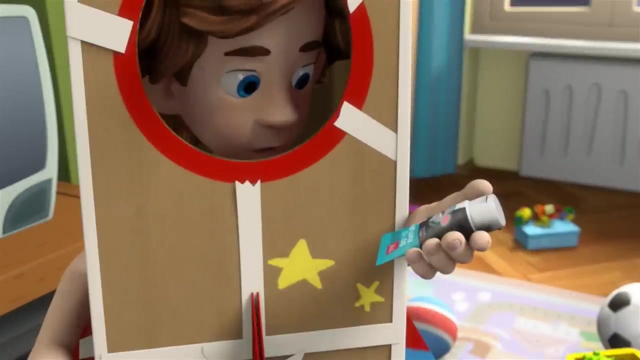 Next time we built a helicopter, The Toothpaste, Astrodot, food Ready, Rocket ready. And who's flying to the sun? Me, I'm ready. A real hero, Tom Thomas, Did you see? There it is. You nearly spoiled a vital experiment. 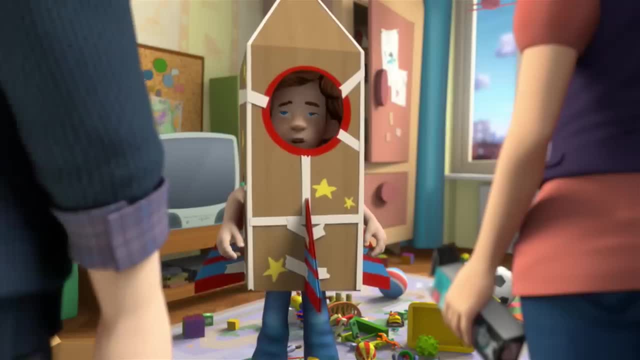 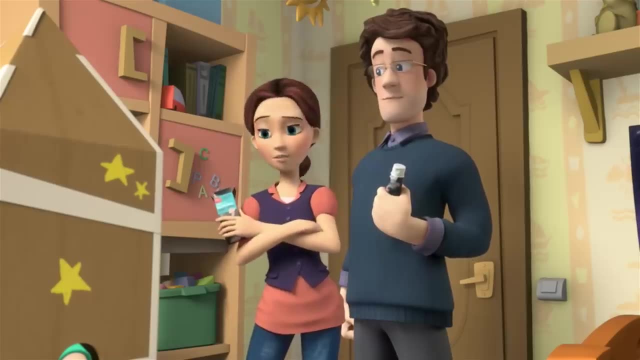 Of global Interplanetary Significance, Spoiled what Our scientific testing of the latest toothpaste formula. I will brush my teeth with it And I, as Chief Dentist, will be monitoring the testing, And so I don't want you even touching it. 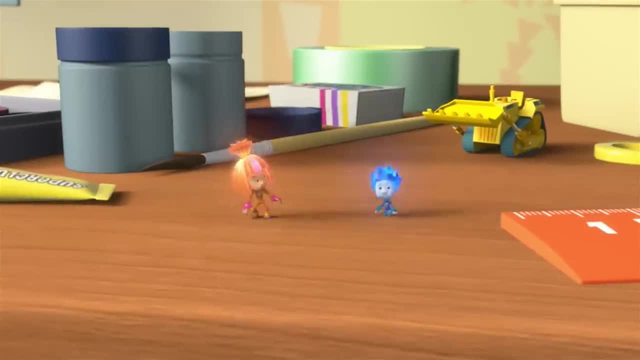 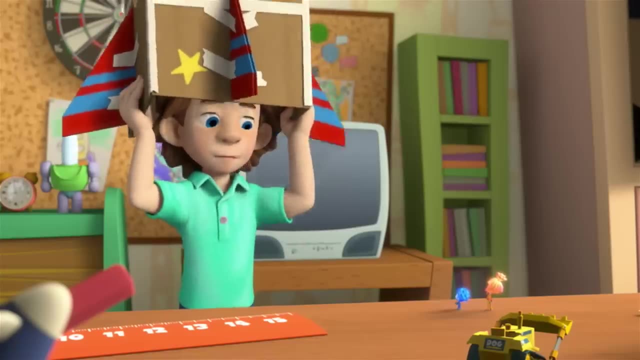 Great. How am I supposed to fly to the sun now? Strange, They make that toothpaste for kids. So Then why is your mom using your dad then? That's right, I'm gonna go tell her Mom that new toothpaste. 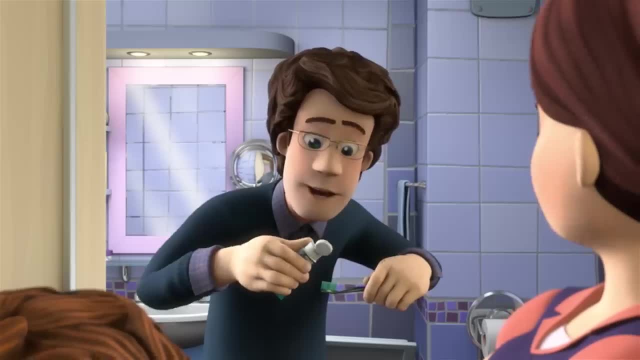 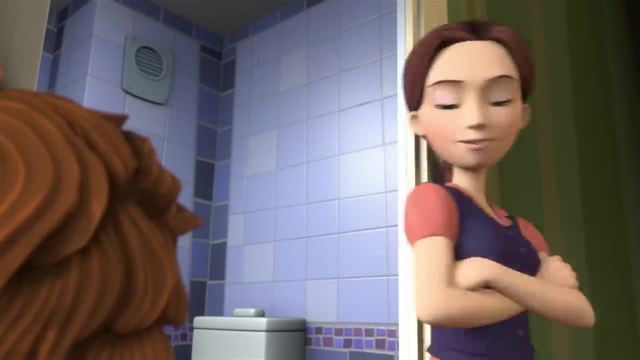 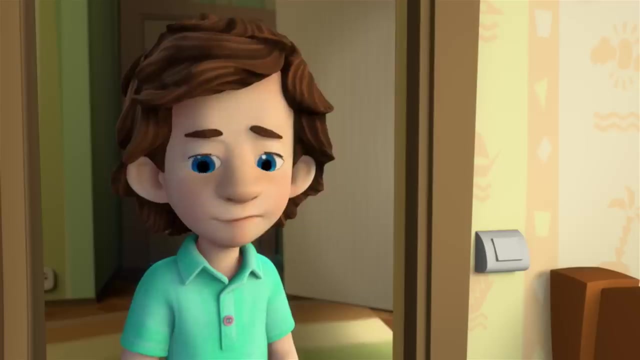 I should test it. No, I'm using your dad Because he's a responsible person And so am I. I'm very responsible. Who knew Your room's a total mess? I had no time to clean it. You didn't water the plant. 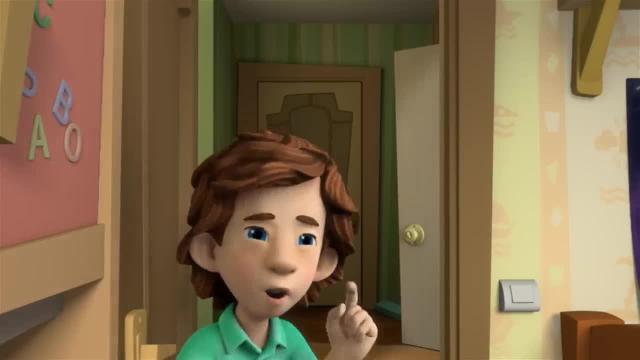 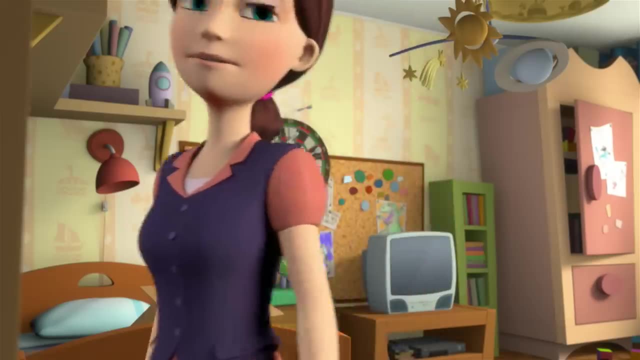 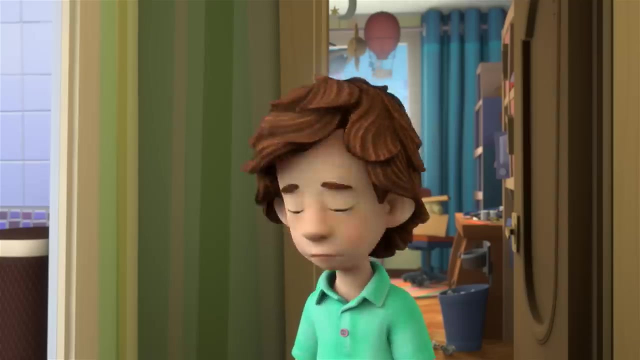 I forgot. Did you brush your teeth? Yeah, For a whole minute too. You're supposed to brush your teeth for two minutes In the morning and at night. Sorry, I'm sorry, honey, Great toothpaste, honey, If you don't want to get a toothache. 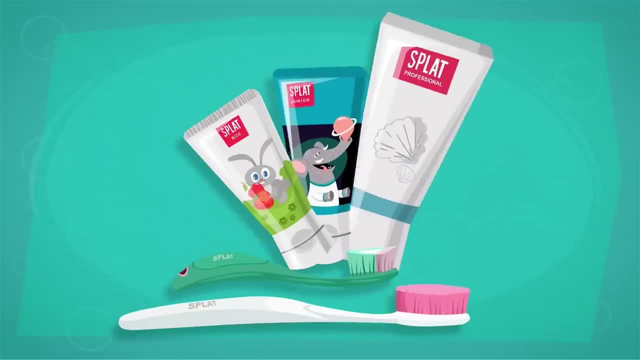 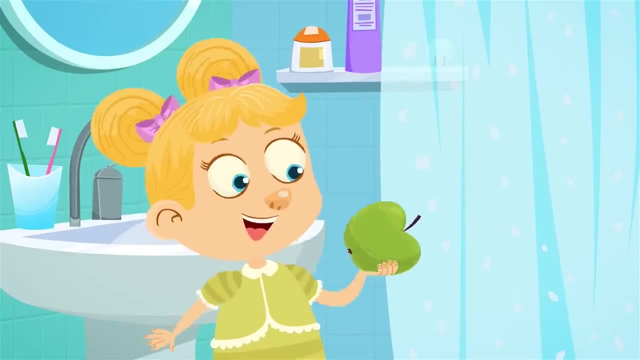 you need to take good care of your teeth by brushing them with a toothbrush and toothpaste. Toothpaste helps remove food that's stuck on your teeth, kills harmful bacteria and keeps your teeth strong, healthy and beautiful. Toothpaste should be in every house. 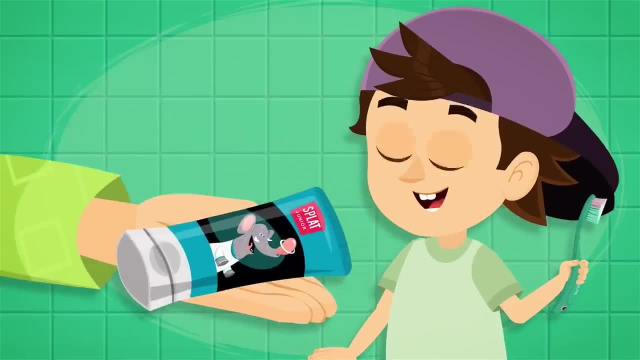 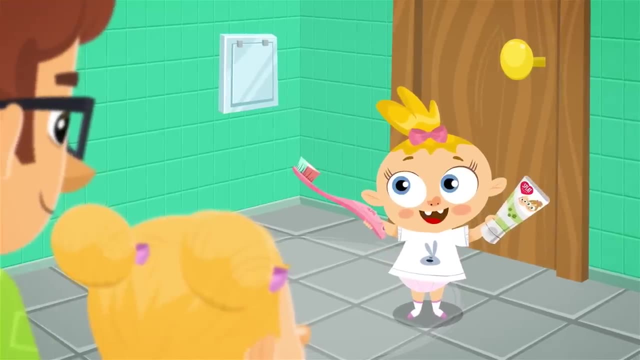 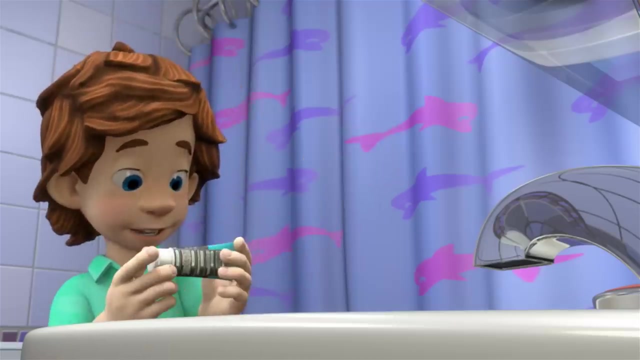 Adults should use toothpaste made for adults, And kids should use toothpaste that is healthy and safe for younger teeth, It's important to make sure you're using a toothpaste that's right for your age. Tom Thomas, don't touch it. 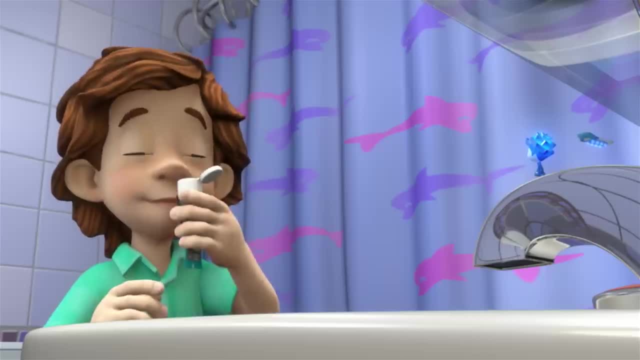 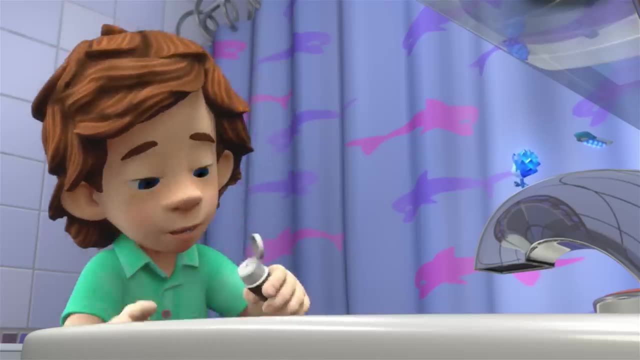 It's for the experiment. I'm just going to smell it, Don't worry. Well, It smells like bubble gum. Hey, Just a peek at the collar, That's all. Come on, Do you want to spoil the experiment? Now put that toothpaste right back. 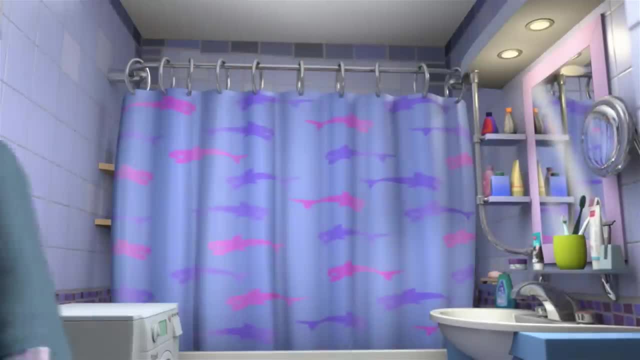 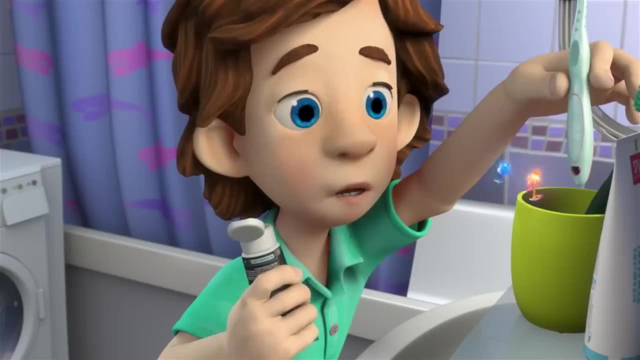 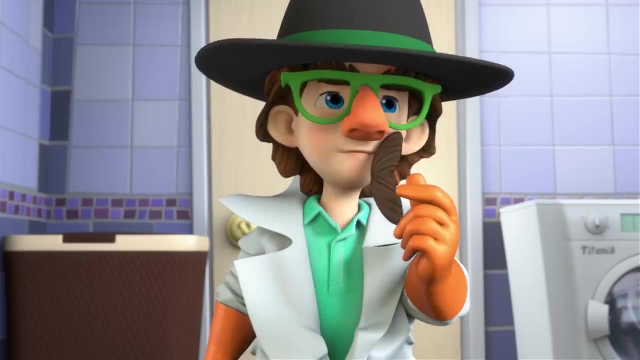 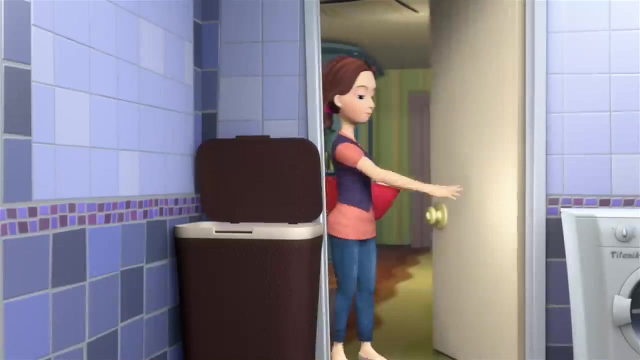 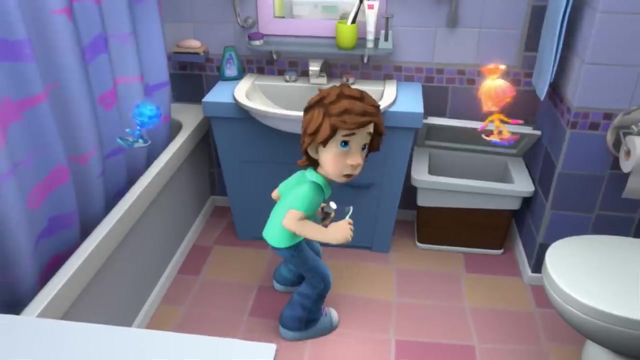 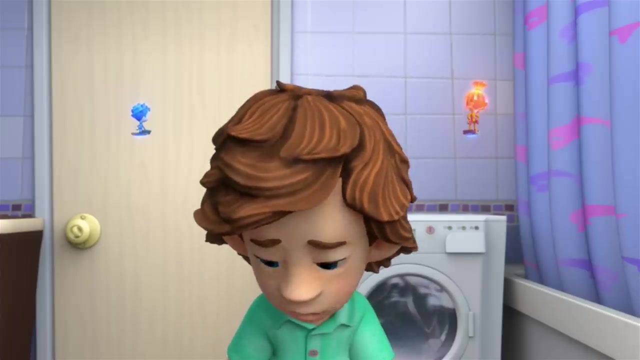 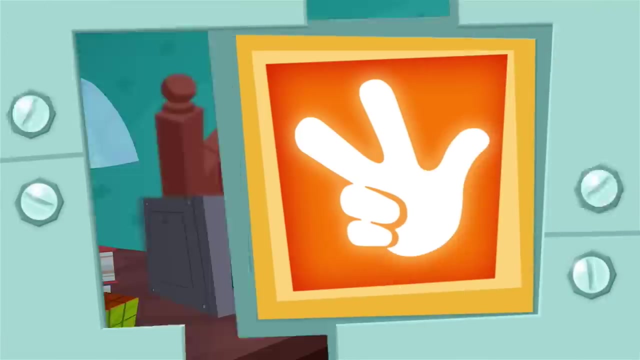 Hmm, Again USB. Well now, So we caught you again. I want to try this toothpaste. so bad, but how Well? what if you? um, Do you know how to brush your teeth correctly? Let's check. 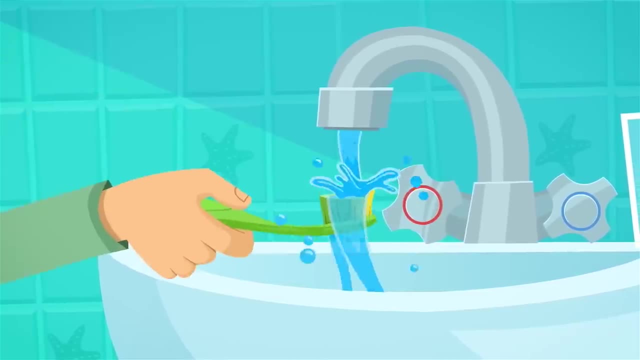 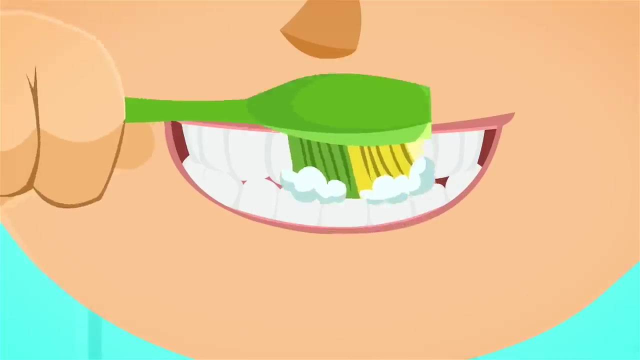 First take your toothpaste, your toothbrush, and rinse it with water. Then squeeze on a bit of toothpaste. A small pea-sized drop is all that you'll need Now. one: brush the outside of your front teeth up and down. Two: 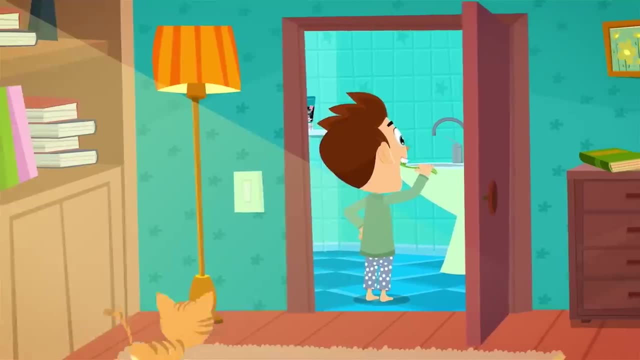 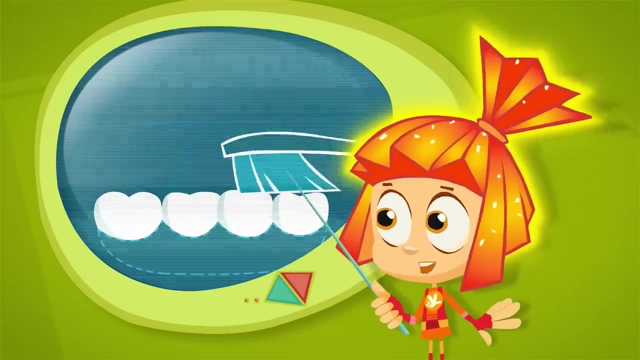 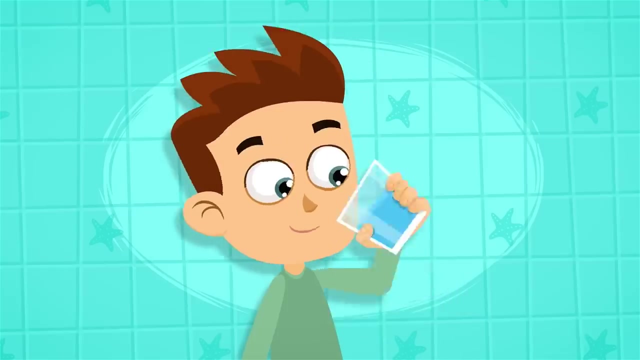 brush the backs of those teeth, from the gums on down Three. open your mouth real wide and brush the teeth in the back. These are the teeth that you use for chewing. Go back and forth, over and over. You should brush a full two minutes, no less. Now it's time to rinse out the toothpaste from. 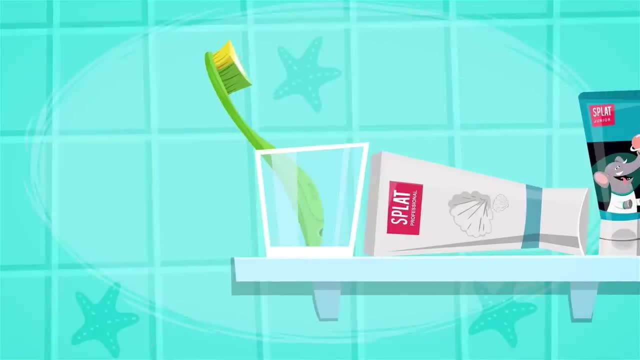 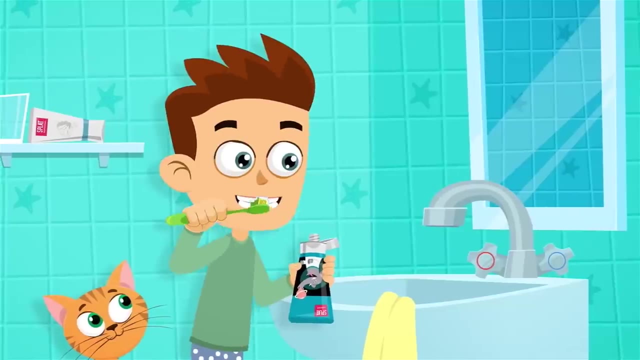 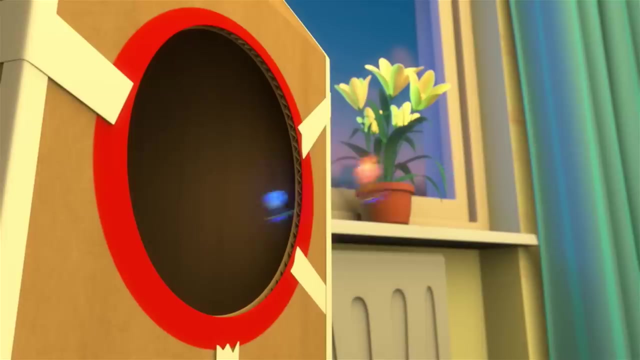 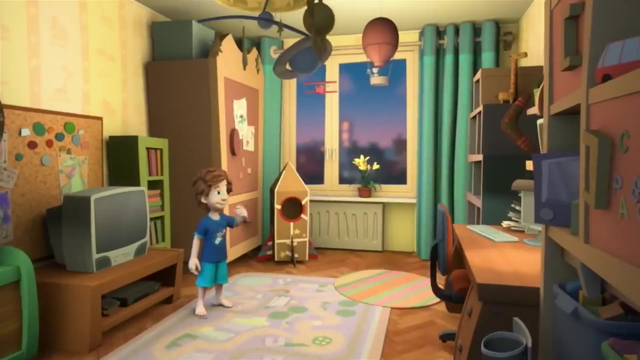 your mouth and clean the brush. That's right. the brush needs to be clean too, And please don't be lazy. If you brush your teeth two times a day, they'll stay in great shape for many years to come. Mom, Dad, see, I've done everything Well done, And I promise that I'm going to brush. 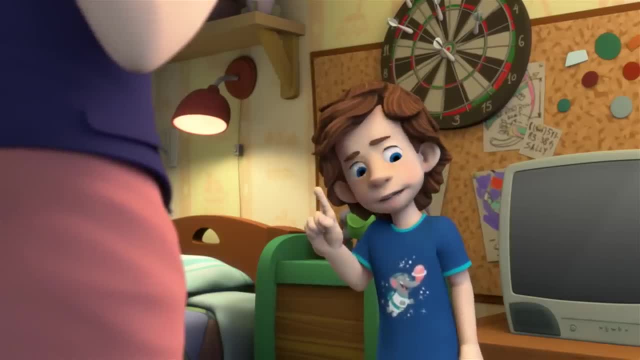 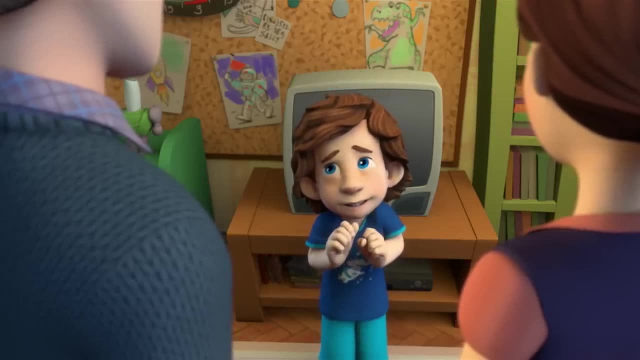 my teeth the right way, as long as I need to, and And twice a day Only. let me be a part of your awesome experiment, please, would ya? Well, I don't know, I think we could try it. Oh What? 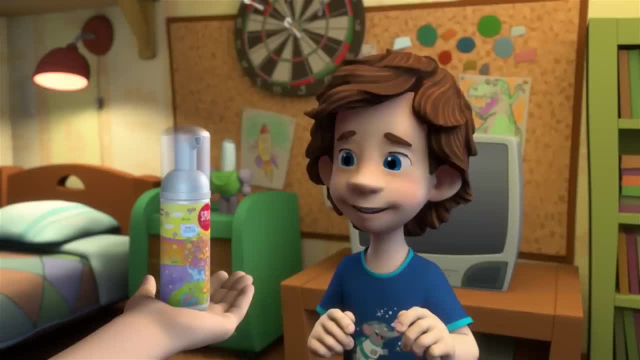 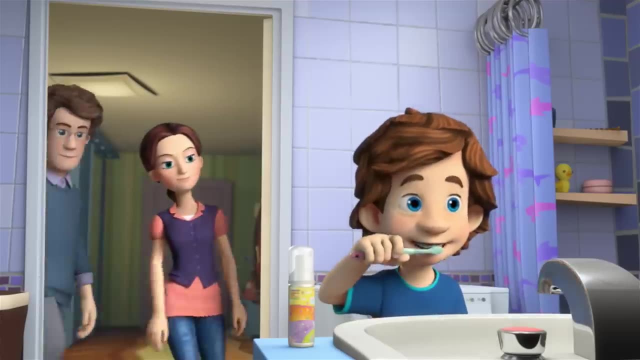 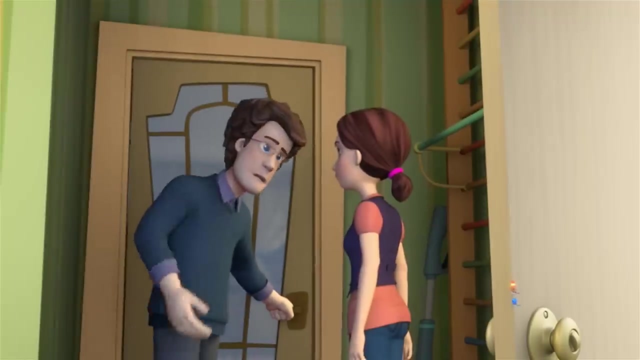 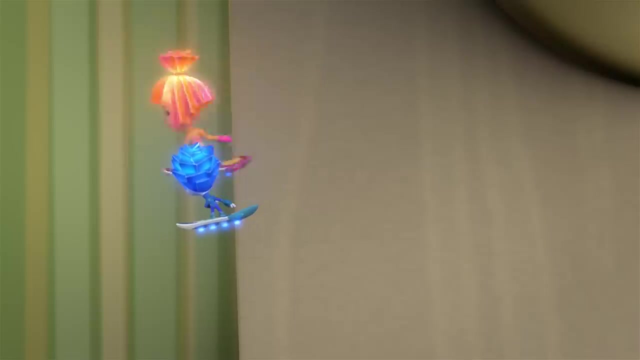 Well, we also have this foam for teeth. Who's going to test that Me? A real hero. How many ways did we try to get him to brush his teeth before? that didn't work? We never sparked his imagination before. Your idea about the experiment was brilliant, Simka. 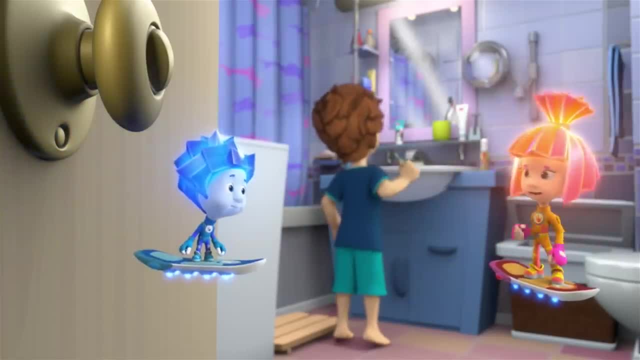 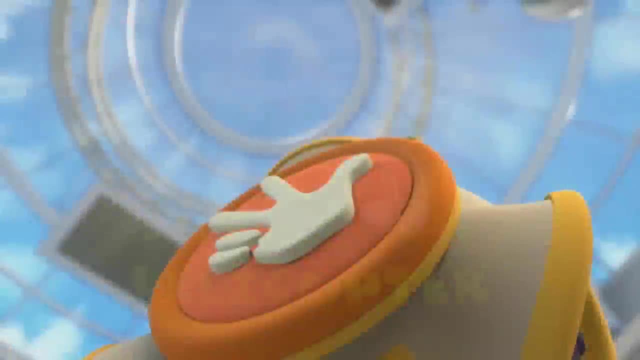 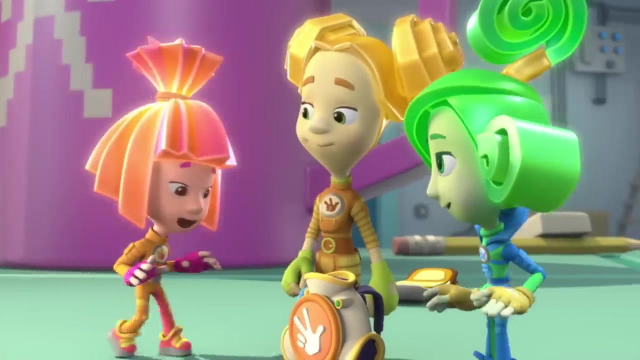 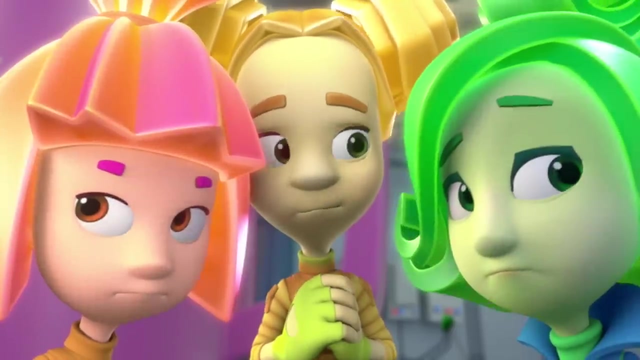 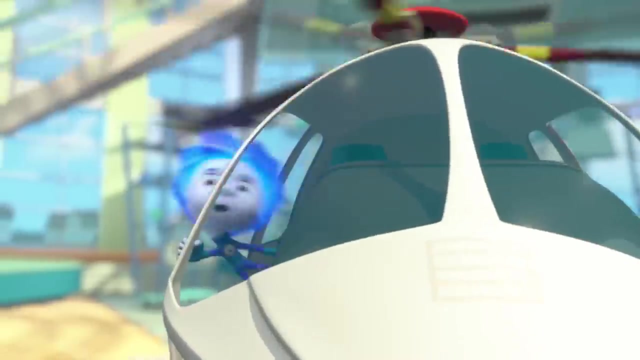 do you think we should tell him? The answer is no. We can't disrupt the experiment, The Helicopter. It's very important and I need your advice. Sorry I'm late. Oh girls, I can hardly wait to see this. Here it goes. Hey there, Where did you get a helicopter, Professor Eugenius? 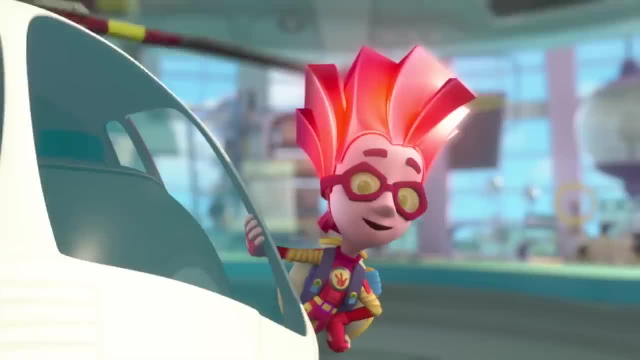 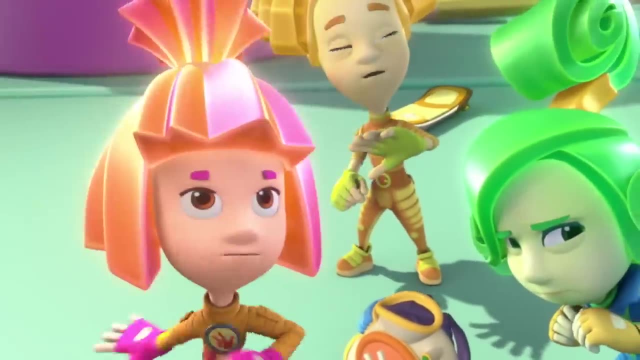 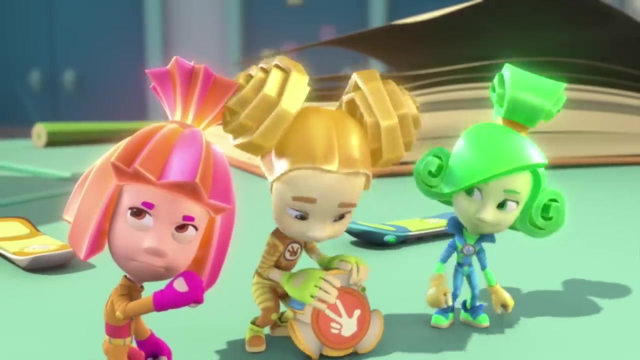 threw it away, but we we fixed it. Come fly with us. Hop in. There's no way We're busy Doing what Something important. Go find somewhere else to fly. You got it, No problem. Now back to work. 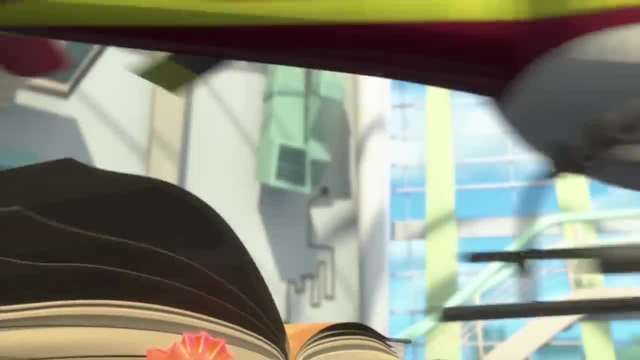 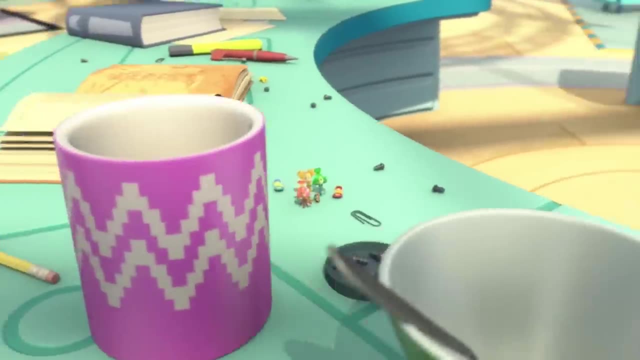 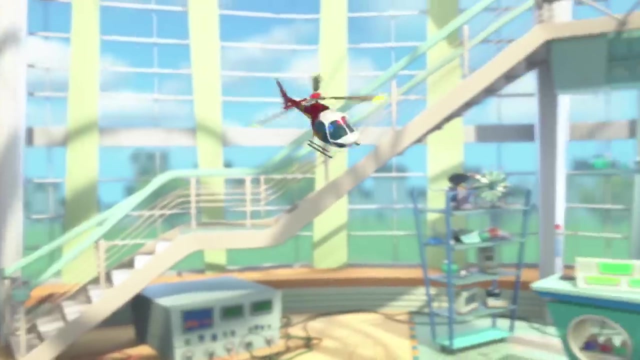 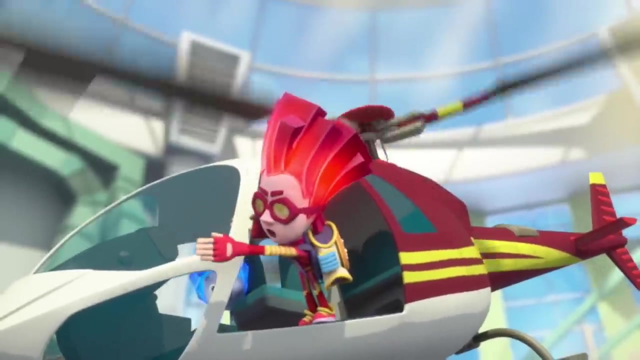 Stop it. right now You're bothering us And and you're going to fall, Land that helicopter. We can't do it, But you're flying it. Why can't you land it? Because there's the controller, Digit's our pilot, Digit, fly on. 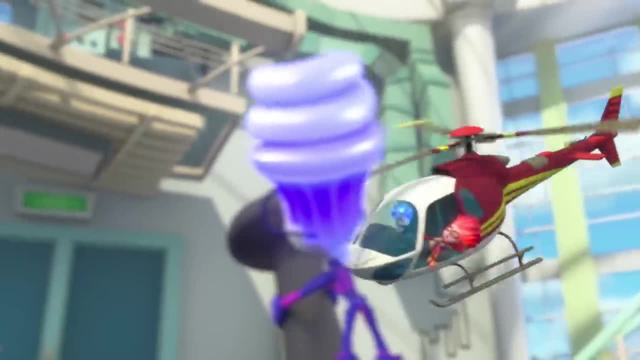 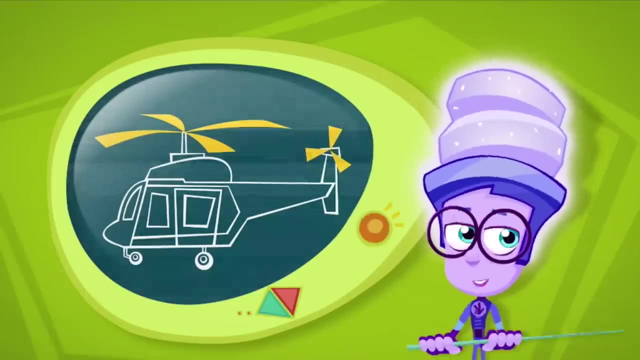 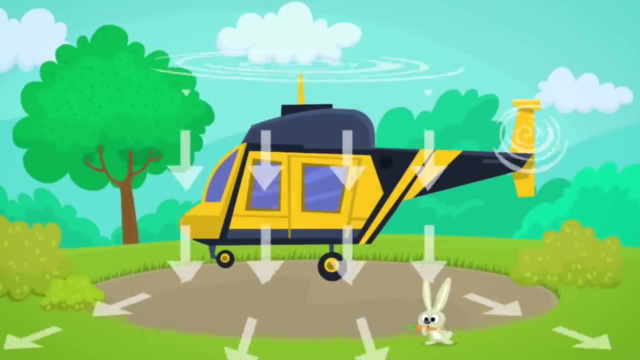 Ehh-hhhh, Ah. Helicopters fly with the help of propellers. The biggest one is called the main rotor blade. When the engine turns it, the rotor pushes the air with such a powerful force that it lifts the helicopter up off the ground. Of course, helicopters can't fly as fast as air. 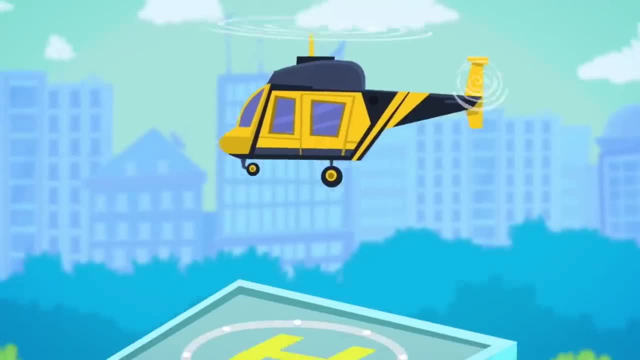 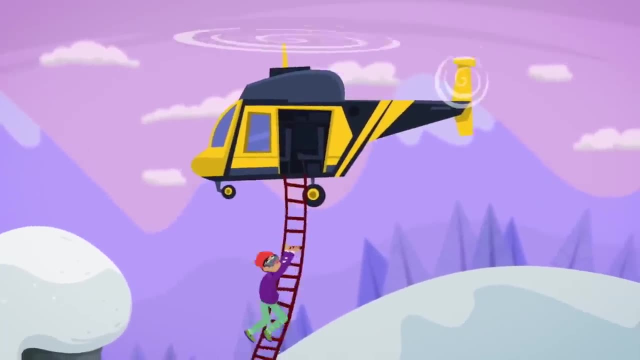 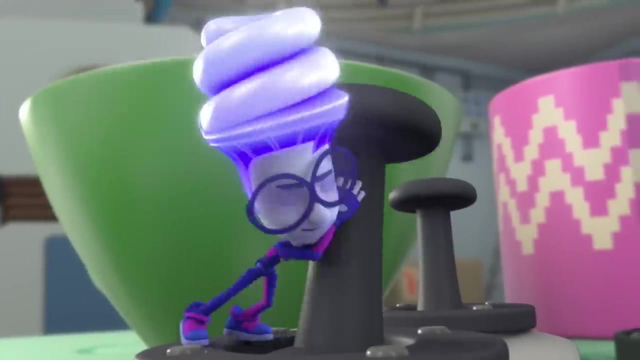 planes, but they have the ability to easily land on a small patch of ground and on a And, unlike airplanes, helicopters can hover in the air for a long time and even fly backwards. Digit, turn us to the left. No, Turn right. 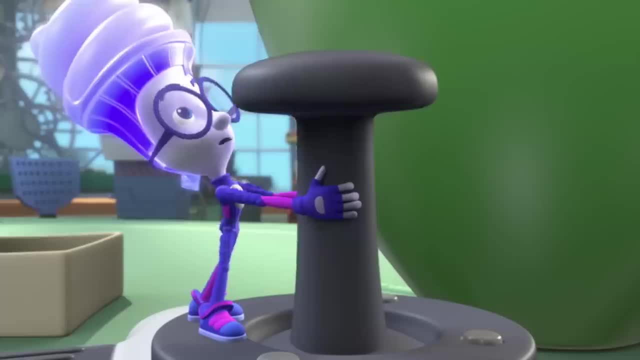 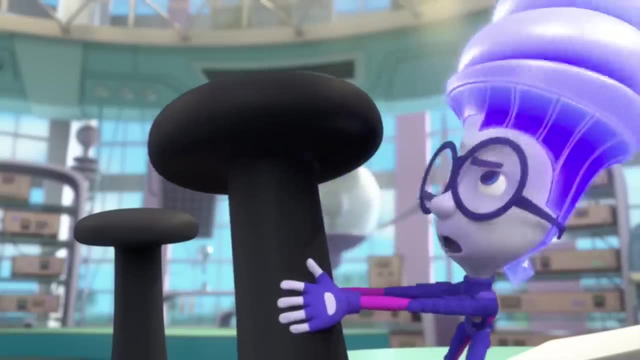 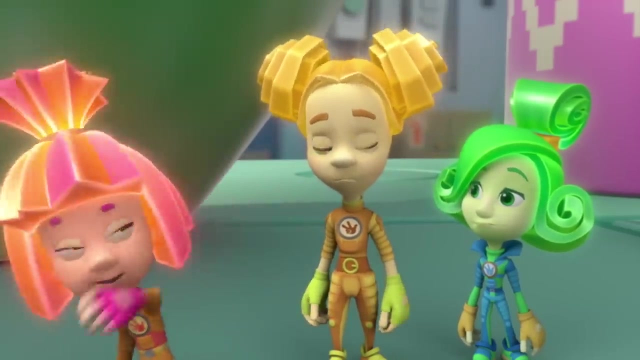 And higher Digit. Fire and Nolik are being dopey, but you're smart enough to know it's dangerous. Just land it. Hang on, hang on. This is one amazing rotor-driven machine. Leonardo da Vinci himself had it designed for one. 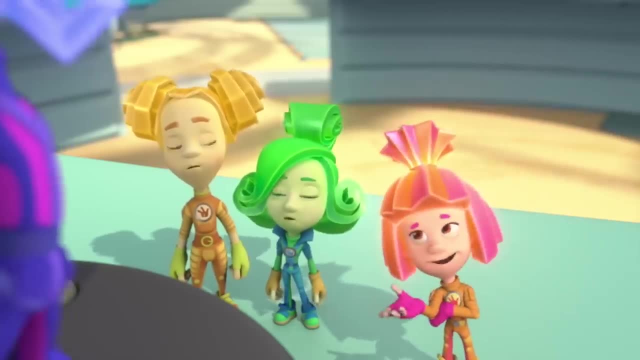 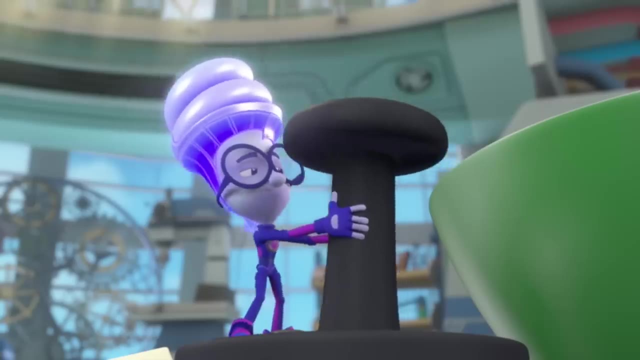 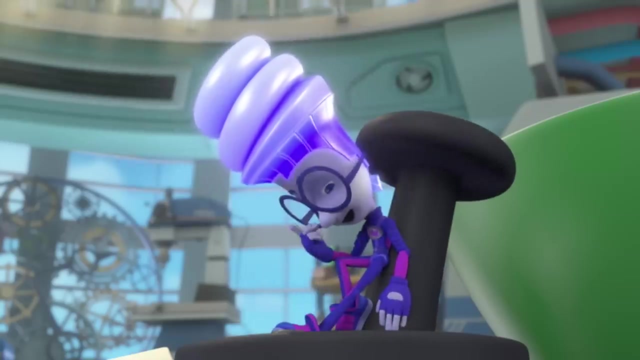 And now look who's controlling it. It really is impressive. You're a total ace on that controller And so smart And brave. The girls really like boys like that. That's how I roll. Sure, yeah, you're great. 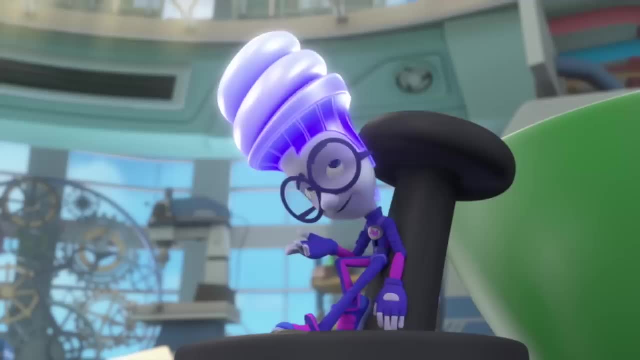 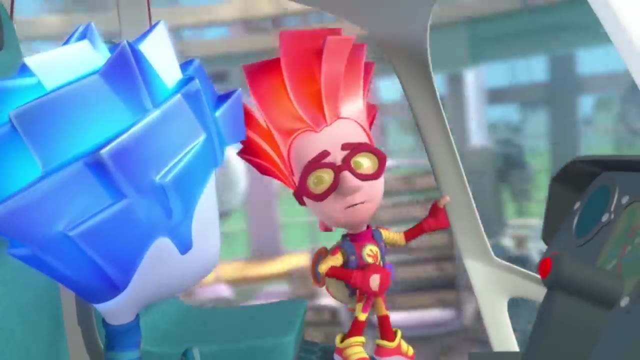 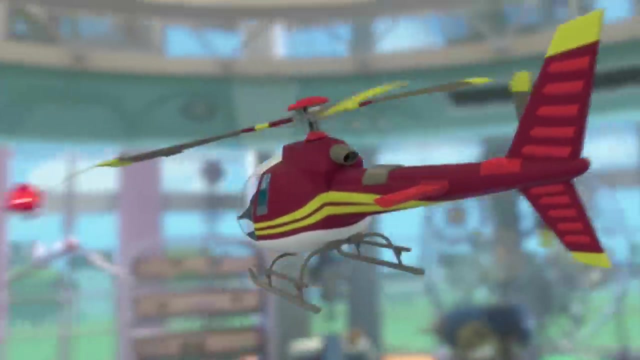 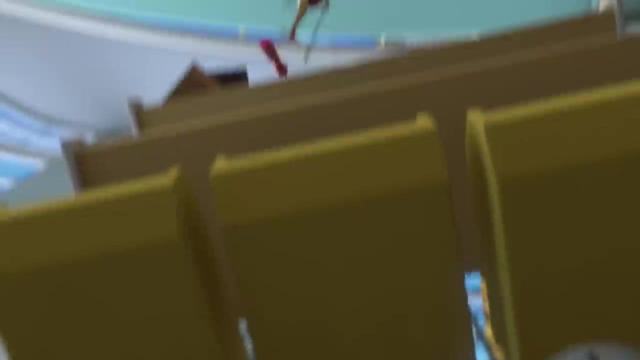 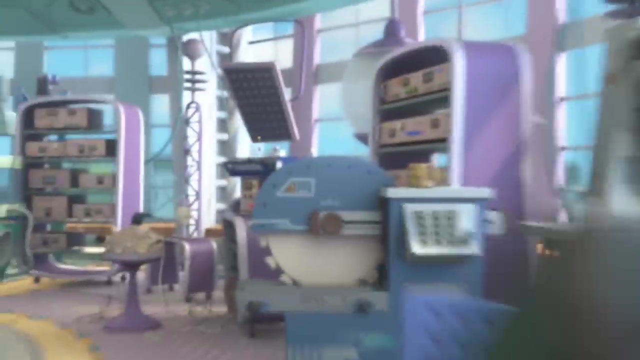 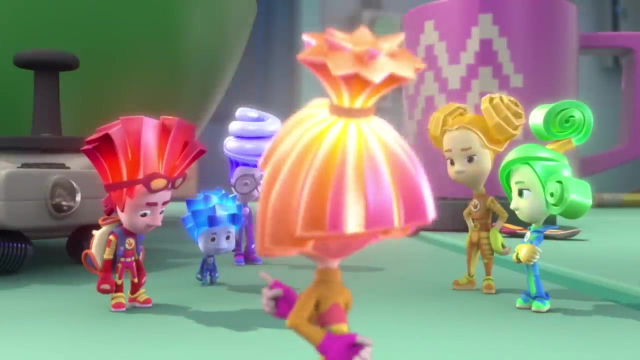 Now land it, Digit The wall. Nolik, don't panic, We're gonna have to jump. What about me? Where's Fire Here? You could have crashed, And if it wasn't for us… If it wasn't for you distracting our pilot, everything would have been OK. 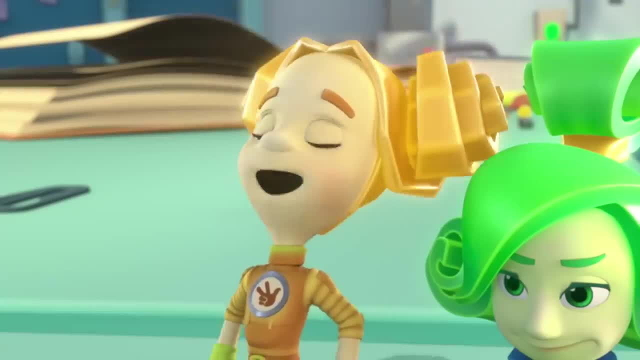 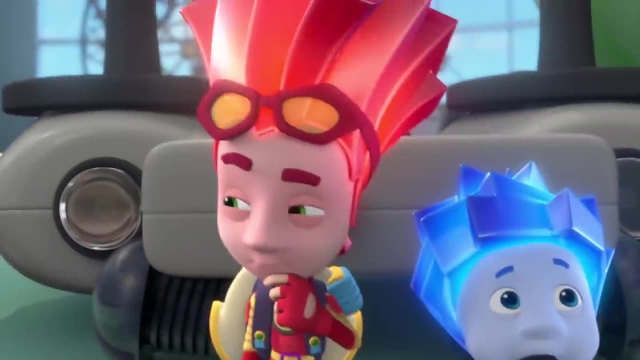 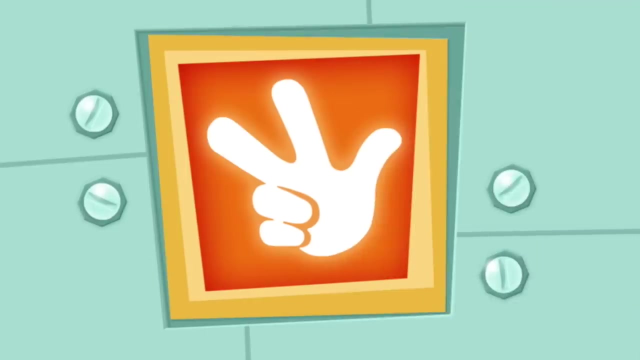 A real pilot, you know, shouldn't get distracted, And first he has to learn how to fly on a simulator. Right Digit, Uh-huh, That's true, But we don't have one, Don't go anywhere. Airplanes, helicopters, trains and even cars. 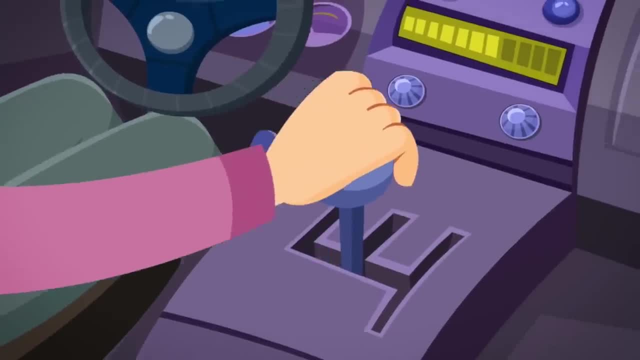 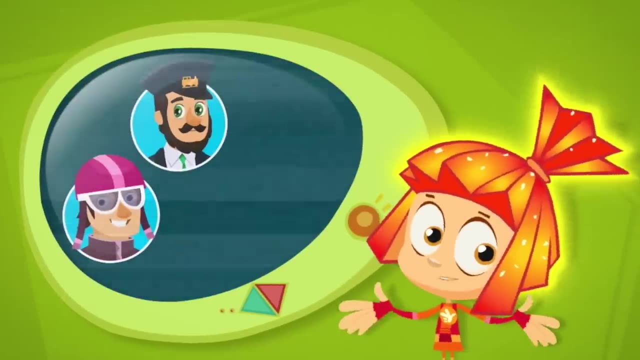 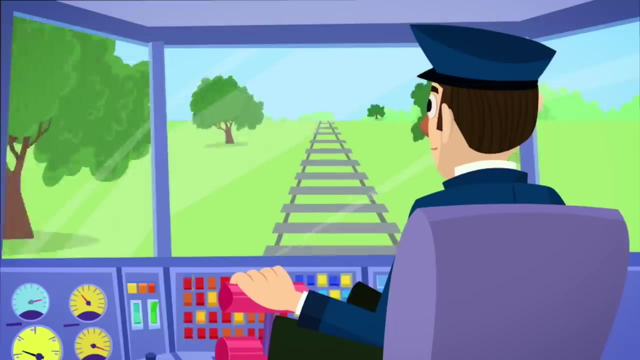 are complicated machines that can be a challenge to navigate, And if you don't watch what you're doing, you can easily end up having an accident. That's why future pilots, train operators and drivers all take comprehensive training classes that include learning how to fly a plane or drive a train using simulators. 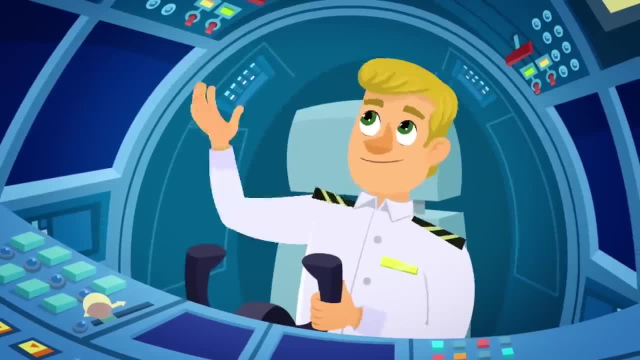 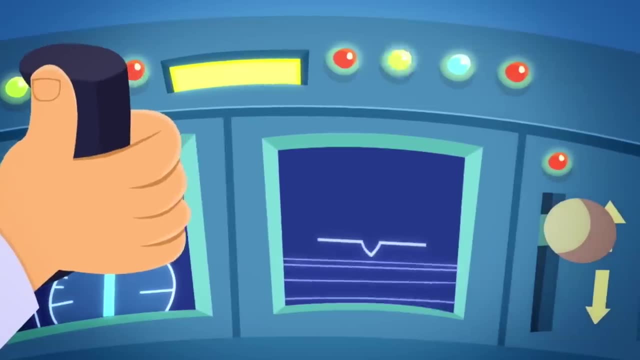 This, for instance, is an exact copy of a cockpit, only without wings and with screens for windows. You pull the controller and the cabin moves the way it would if you were actually taking off, And on the screens the Earth is racing under the clouds. 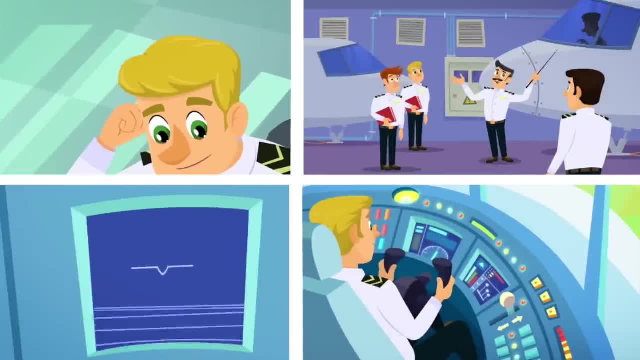 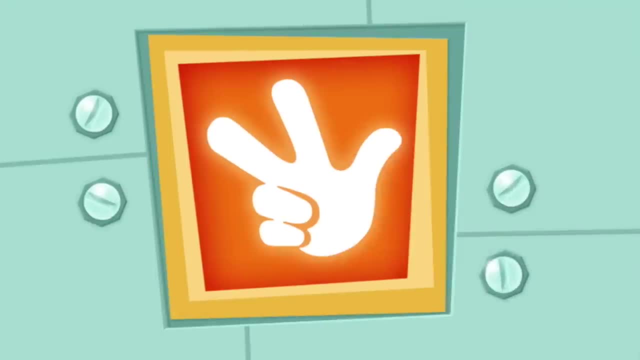 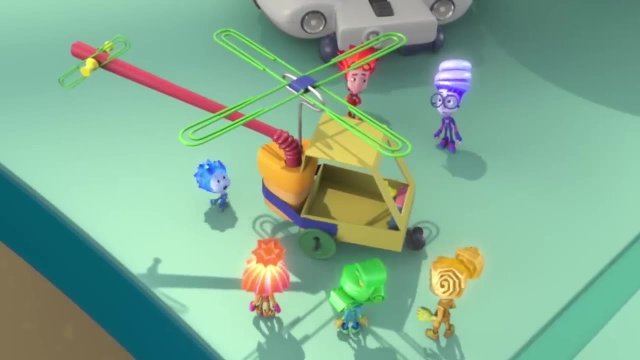 It takes your breath away. Commercial pilots are required to take part in many simulations like this before they're allowed to pilot a real airplane. Our pilot simulator is ready to go, Oh wow, And I'll be the first one to try it. 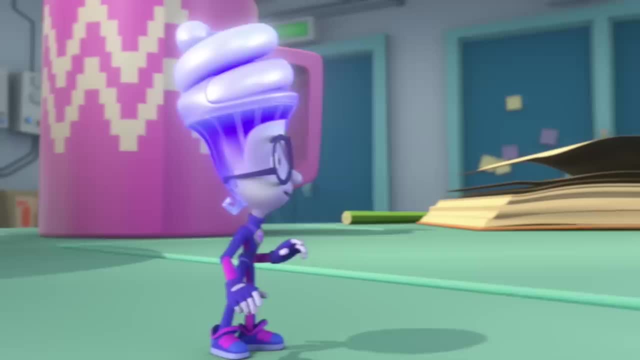 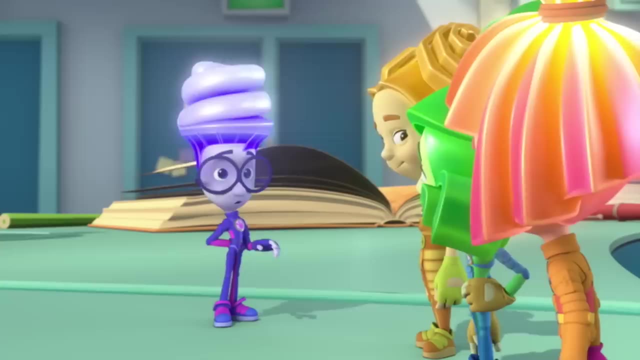 Here we go. Kids Right Digit. I'm only going over there just to take a look. You know how those two can behave, I'll just watch them. It's my turn again. Hey, wait, It's my turn now. 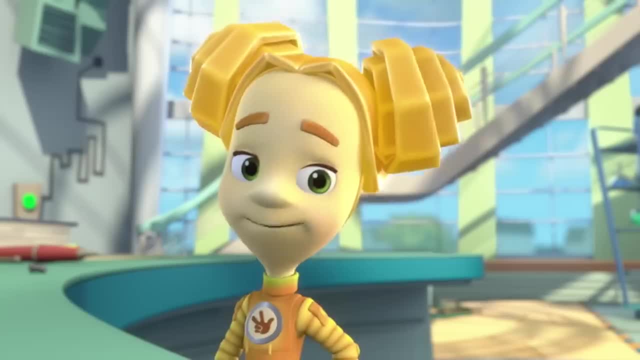 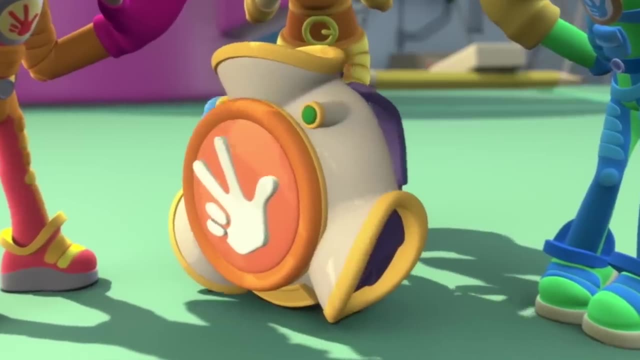 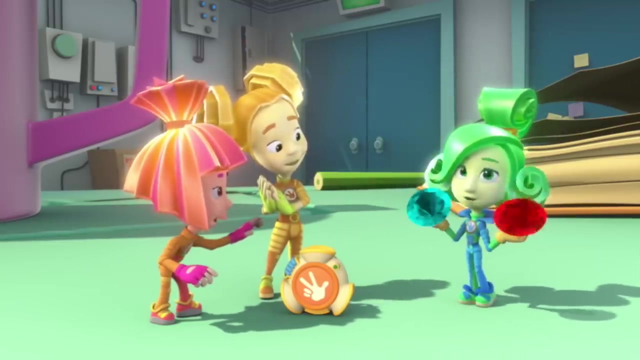 Boys are just silly. They're never serious, They just joke around. Speaking of serious, we have some important business to take care of. You're right. I can't figure out where I should put them. What about on the pack-o-mat? 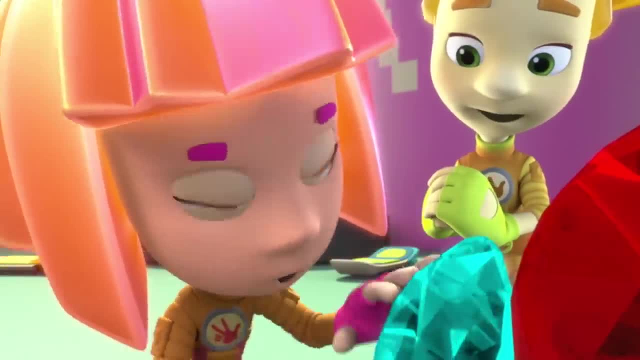 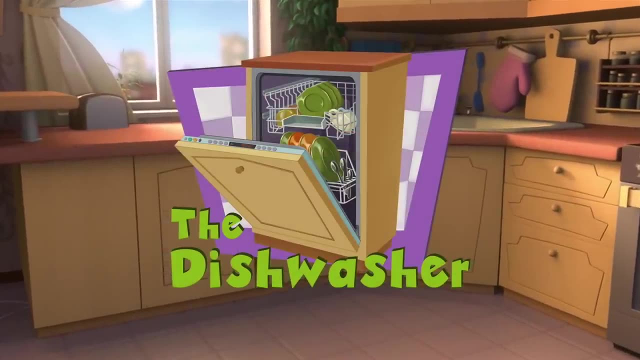 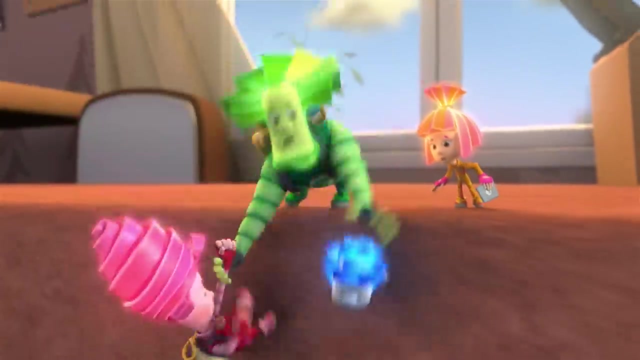 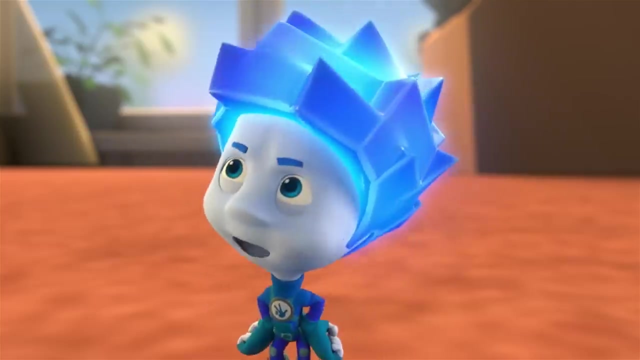 Oh, that's a very serious problem. Yeah, This is really important, Not something silly like those boys are doing. Can't catch me, You won't catch me Enjoying yourself Without a care in the world. What No more cares and bows at you together. 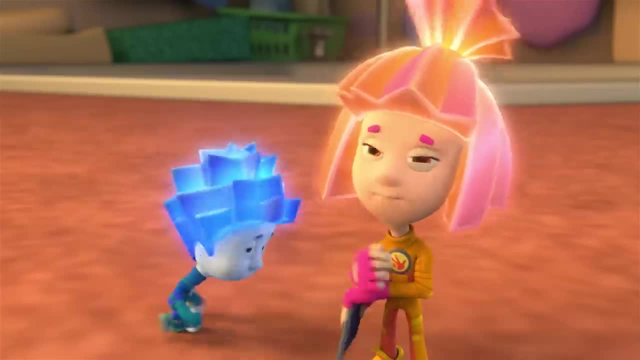 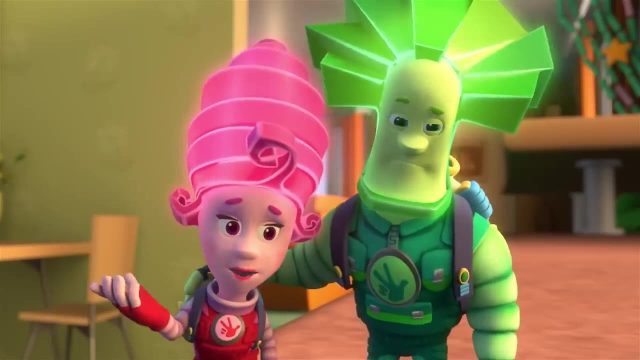 Yeah, anyone can see that. Wanna bet me, How about we try doing your job and you try doing ours, And whoever loses has gotta grant the other's wish? We have a dishwasher here in the kitchen that isn't working and you're distracting us with your nonsense. 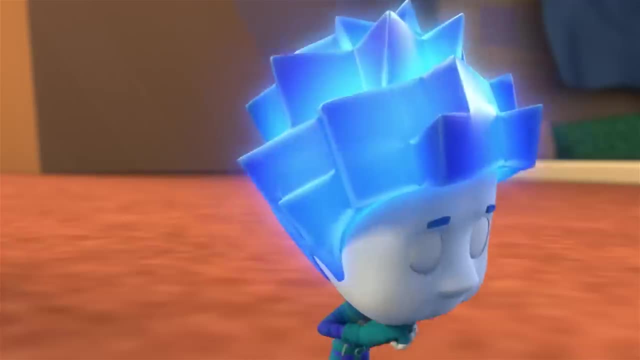 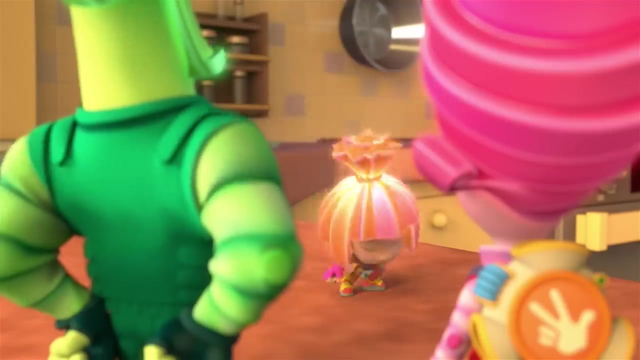 Wait a sec, Let's do it. Find the broken part, Good as done. But where You're, the adults now Go and find it. Just look out for yourselves And you kids. time for school. And I better not hear you. 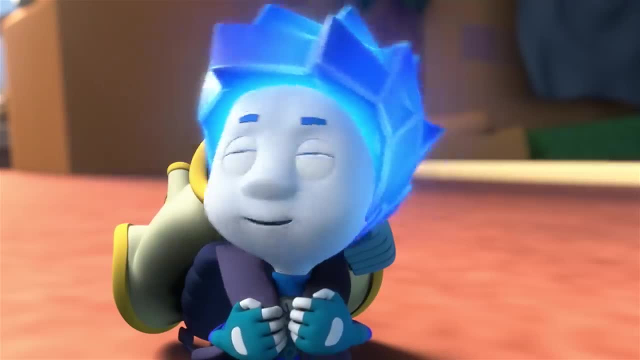 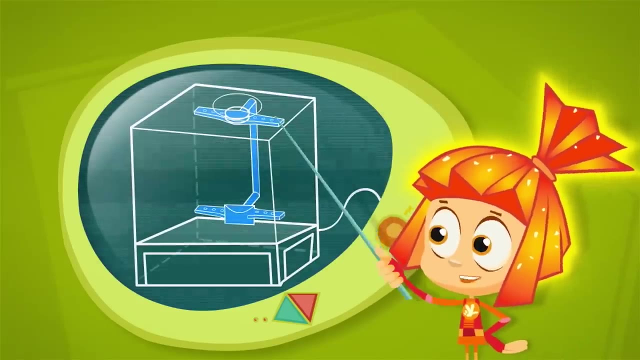 And I better not hear that you were misbehaving. Was I there when they taught us about dishwashers at school? The main element of a dishwashing machine is this part called the sprayer, which looks like a propeller After the dishwasher's pump delivers water. 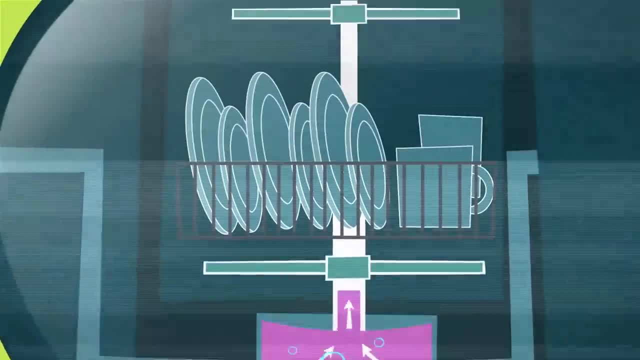 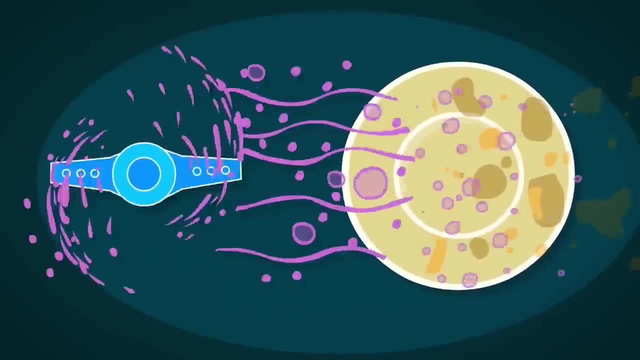 it is warmed, mixed with detergent and then pushed up with high pressure. That makes the propeller spin very quickly so it can shoot out the water with a force strong enough to wash all of the dirt off the plates and glasses. But it does it carefully so that dishes not only come out sparkling. 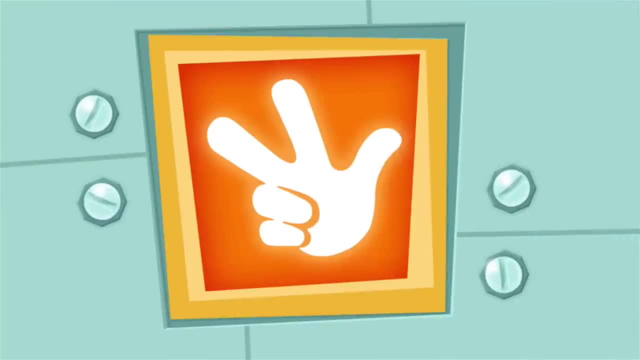 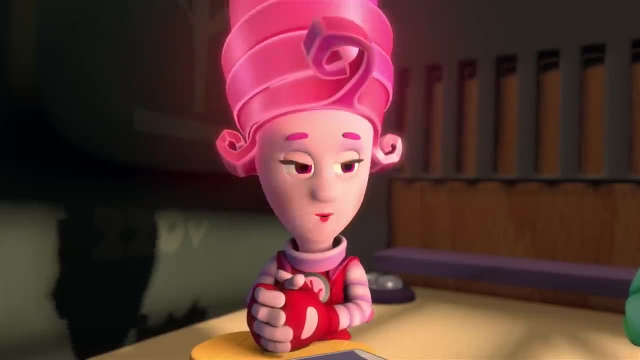 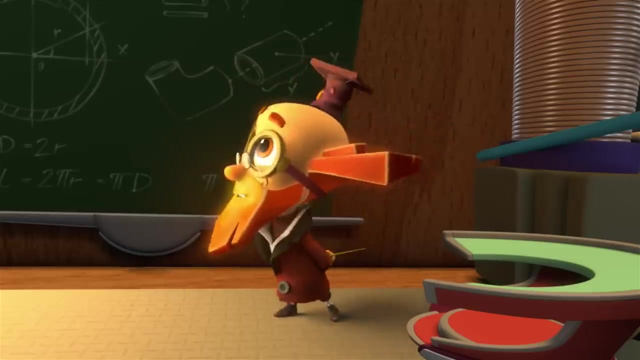 but unbroken as well. Is this a parent-teacher conference? It's not. It's an experiment For today. I'm Simca And I'm Nolik, All right, Who's ready to tell the rest of the class what we studied yesterday? 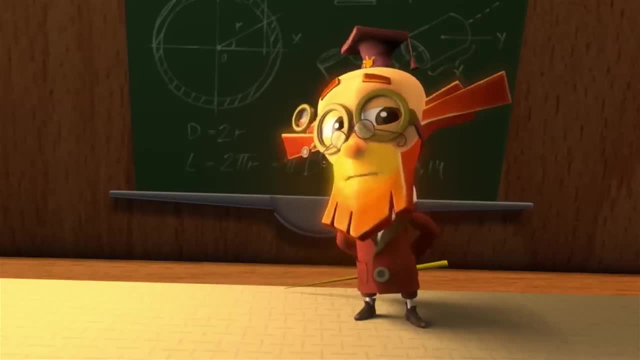 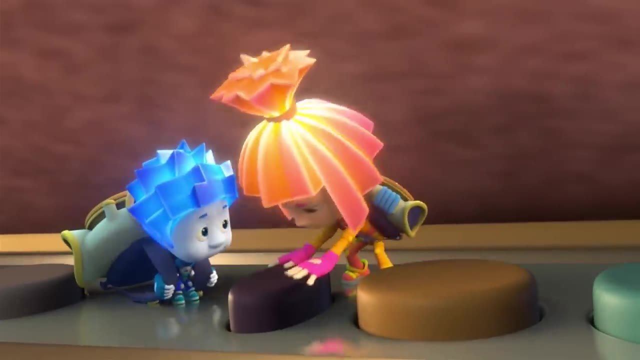 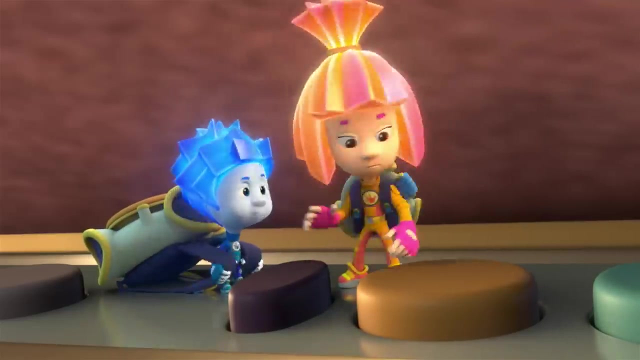 Simca Yesterday. Oh, You forgot Be seated. That's an F, Mm-hmm, I think the problem is in the control panel. I wonder if the dishwasher ran out of water. Ugh, Papus, don't argue with your wife. 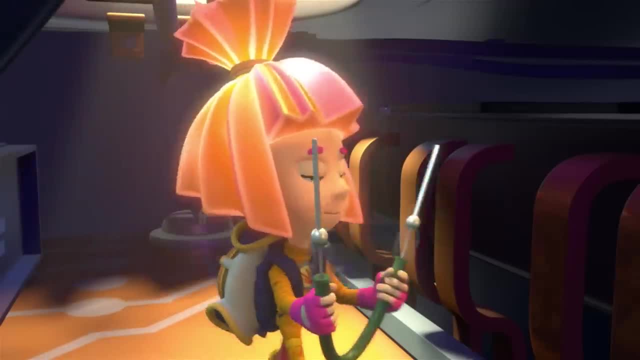 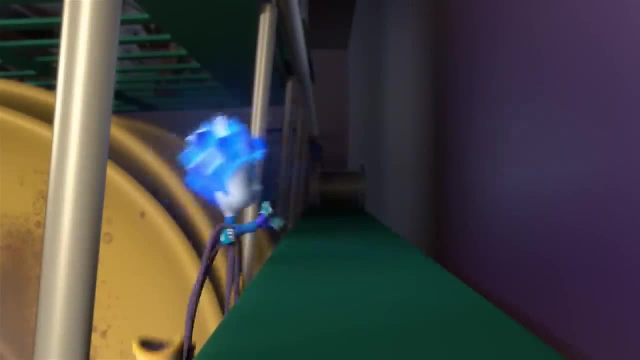 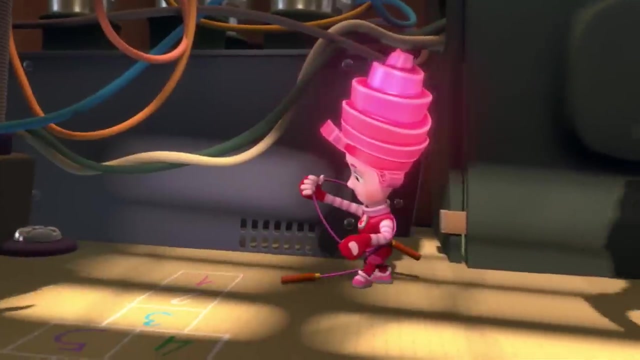 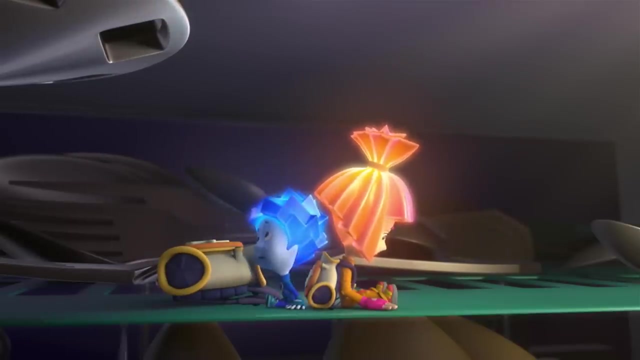 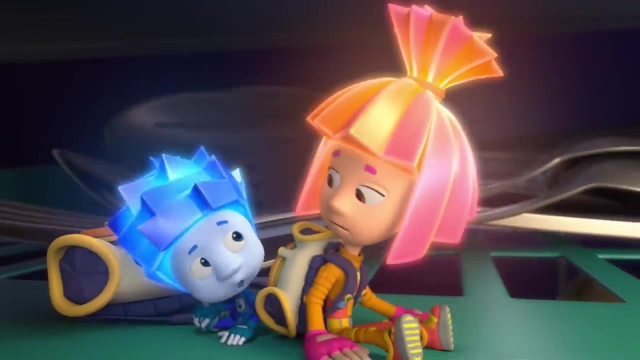 Yipe, This one is working, And so is this. You know what? Why don't we just wash those dishes? But that would be cheating. No one will find out. The dishes will all be nice and clean And bam, We're the winners. 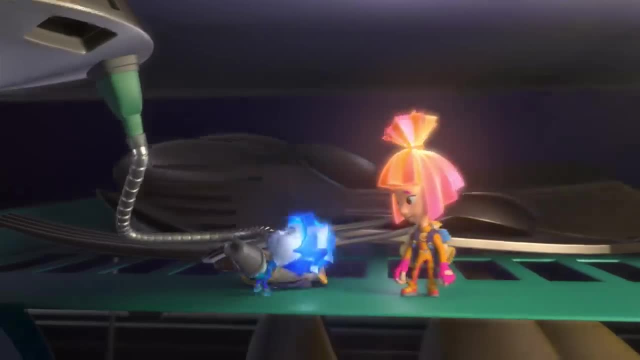 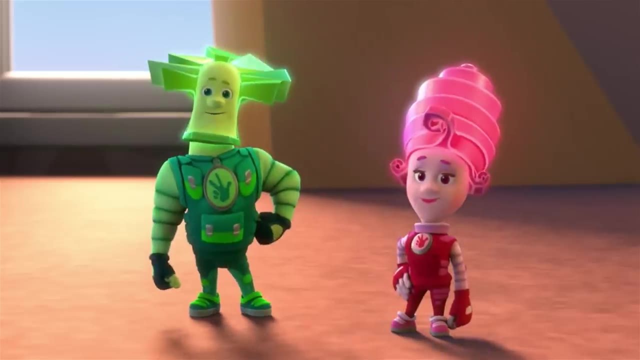 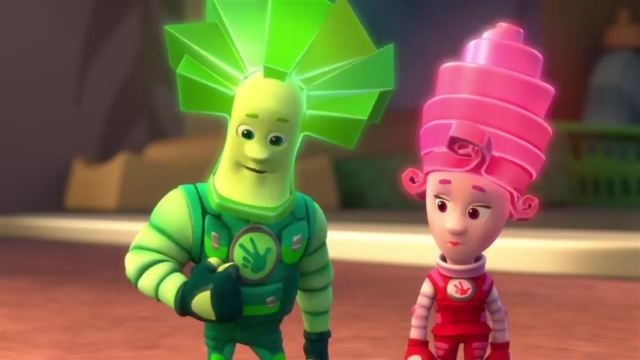 Captions by GetTranscribedcom. Captions by GetTranscribedcom. Captions by GetTranscribedcom. Check it out, We are all done. How come the indicators aren't lit? Fixies have to fix things, And what do you call this? 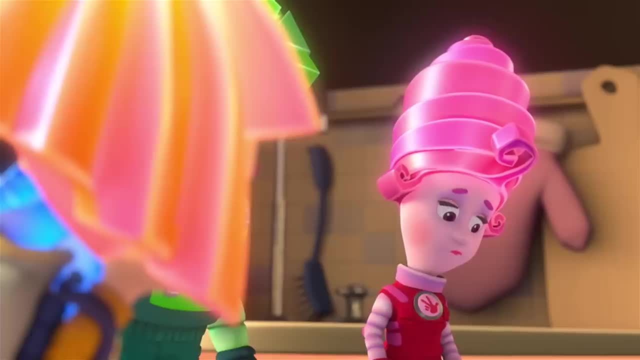 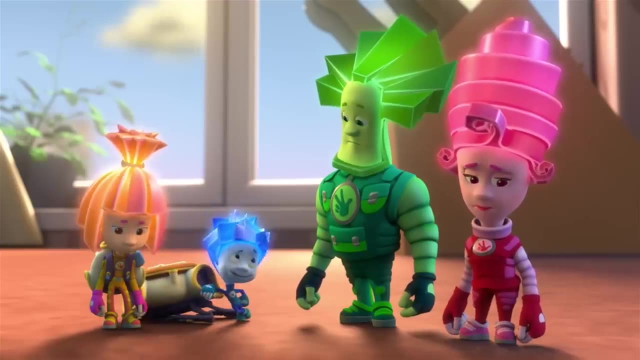 And you? did you both go to school today? Of course we did. I, I mean, Simka got an F for her answer. Well, thanks, Marcia. And did you play with Tom Thomas? You know that we don't show ourselves to people. 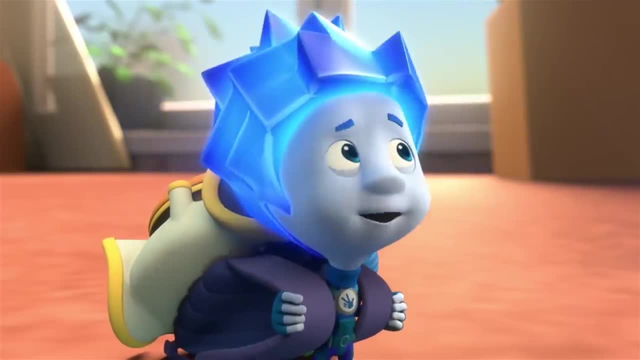 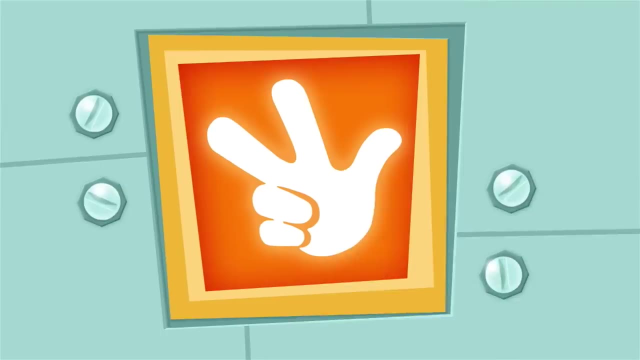 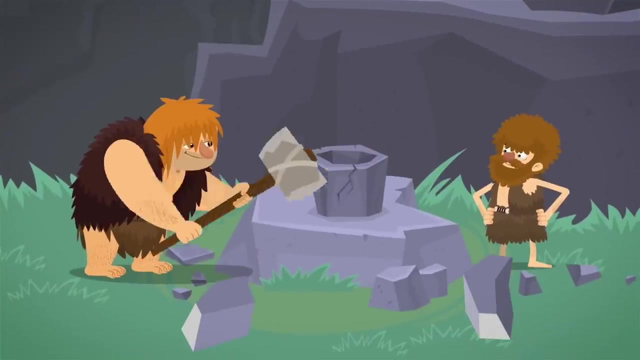 Tom Thomas isn't any human. He's our friend. Either you play with him or you both lose, just like we did. No way, We'll play another round. The earliest kitchenware appeared about 7,000 years ago. Early people made these containers from stone or wood. 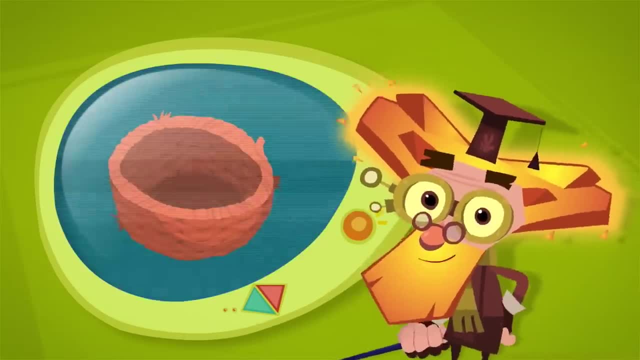 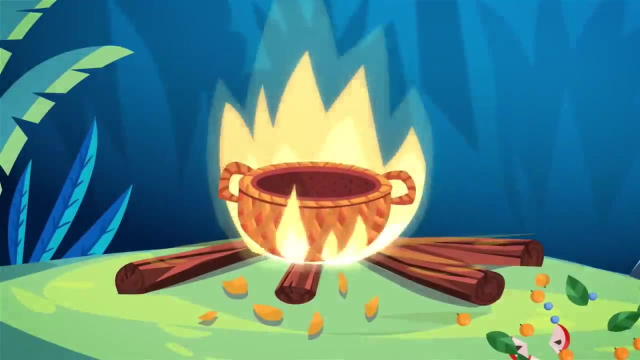 Another kind of container for holding food was woven baskets. The baskets would be lined with clay for durability. Once one of these baskets fell into a bonfire, and lo and behold, the wood on the outside burned away, while the clay was now hard as a rock. 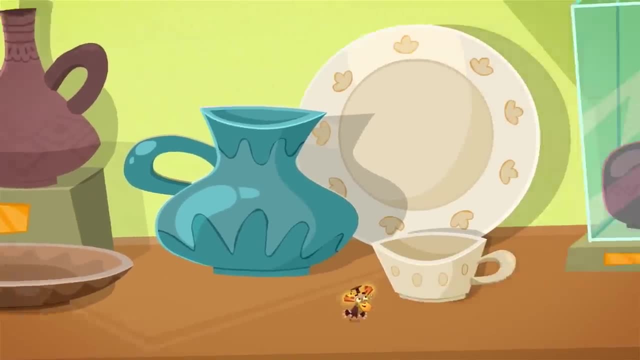 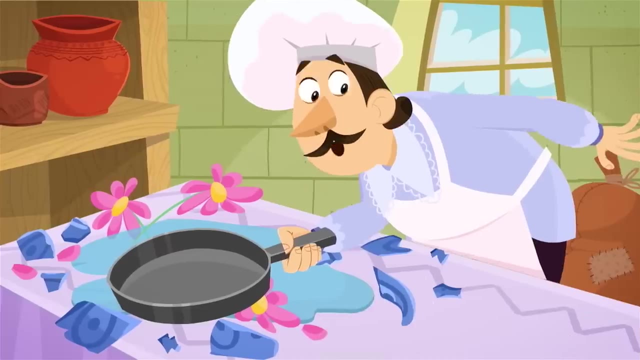 That discovery led to the invention of clay pottery that is still in use to this very day. Later on came the development of glass, metal and cast iron cookware. The world's richest people can even have food served to them on dishes of silver or gold. 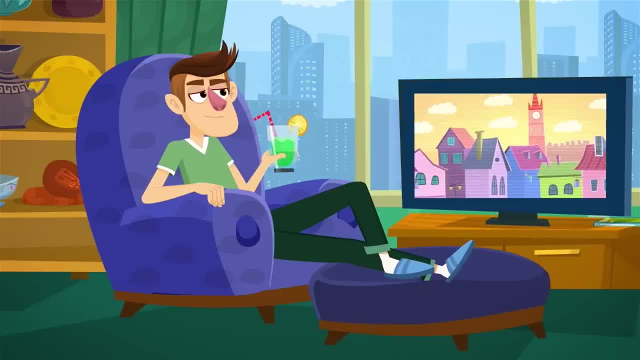 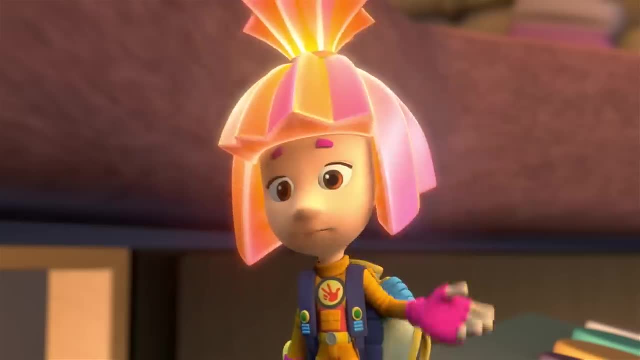 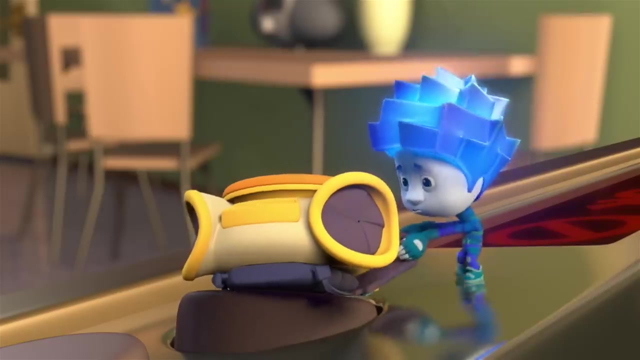 Today, kitchenware is not only a practical convenience, but it can decorate any home as well. Forget it. This is impossible. Let's just tell them we give up. Simka, how come this button is crooked and not sticking out? 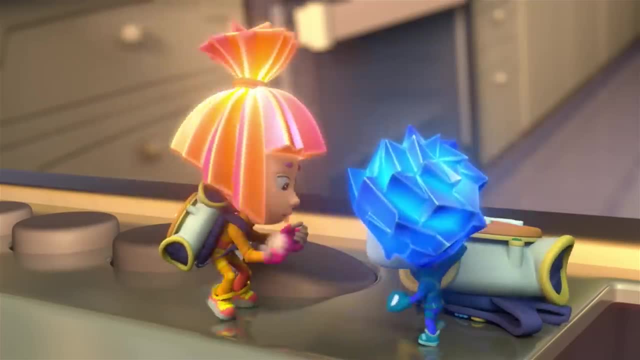 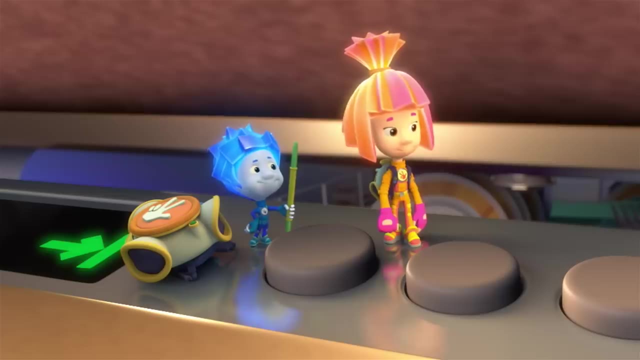 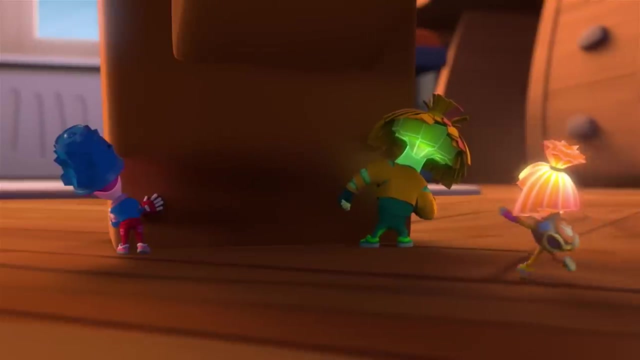 Because the button got jammed. Yeah, Nolik, you figured out what was wrong. I'm glad I kept dragging this around. Tideesh One, Papus, we fixed everything. Shhh, Really, Does this mean you're playing with him? 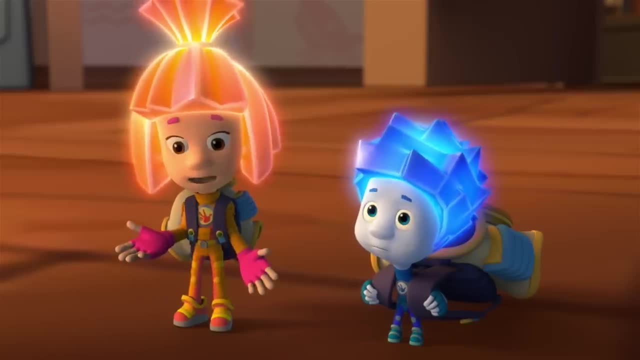 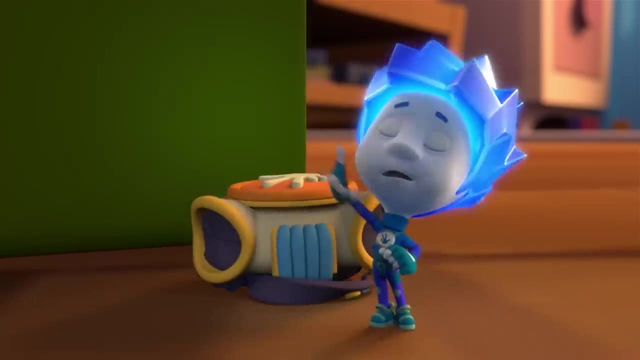 What You think. we're some quitters. Ha Fine, Then, which one of us is the winner? Ready or not? here I come. Let's call it a draw. Each team gets one wish. Our team wants you to fix my ass.